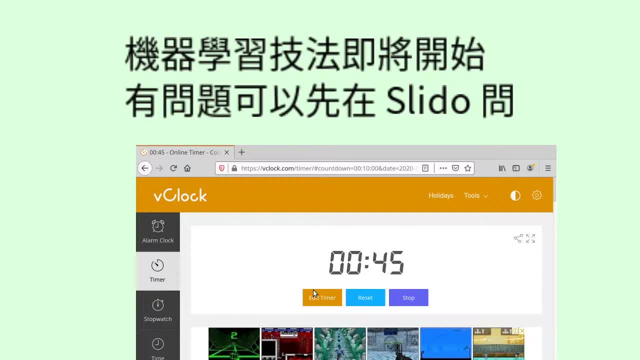 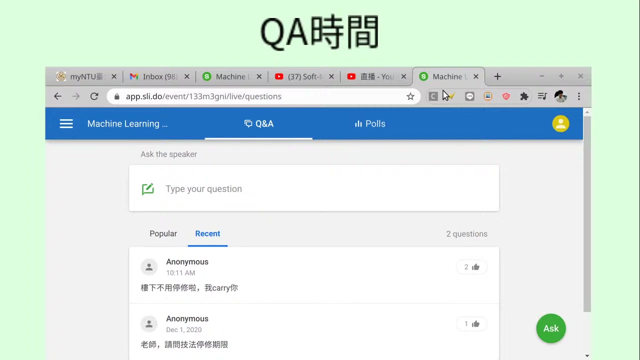 Thank you, Thank you, Thank you, 大家好大家好歡迎來到今天的機器學習技法的課程。. 天下下雨現場同學比較少一點。. 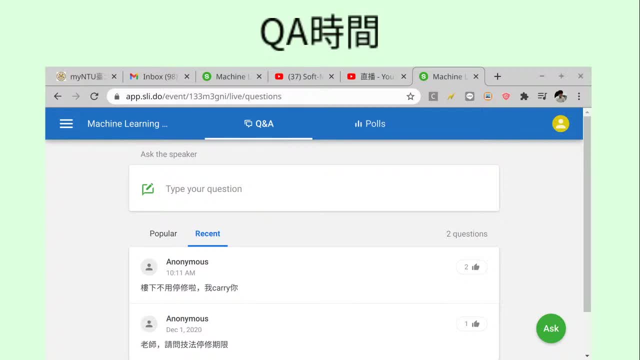 感謝下雨的天氣還願意來到這邊的同學們。 如果你不方便過來沒關係線上的同學們我們一樣聽一樣討論。. 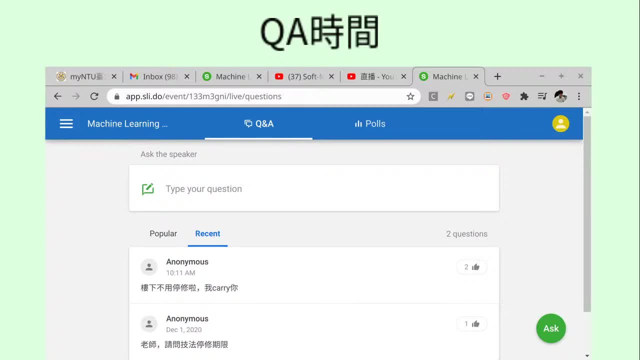 幾件事情第一個是我們今天大概就會把所謂的 support record machine- 我們預計想要教的部分結束掉或至少告一個段落。. 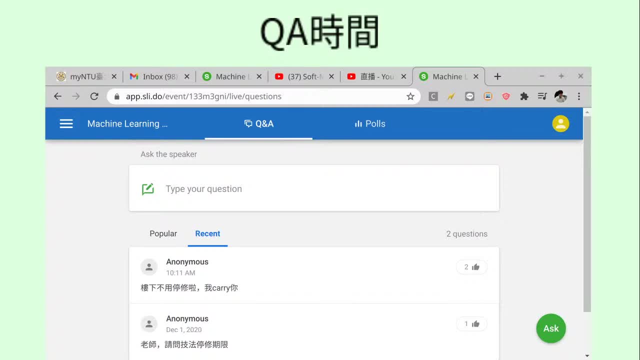 那告一個段落的原因會是我這個禮拜會用一點點時間. 我們先教所謂的推薦系統。. 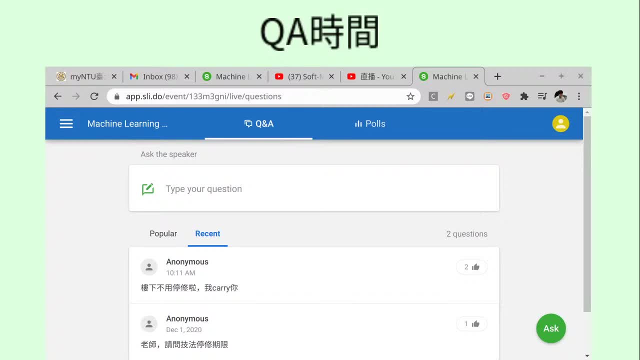 本來在機器學習技法的錄影課程裡面是在非常後面的部分。 但是我們之所以要先教這個是因為下星期二的課程. 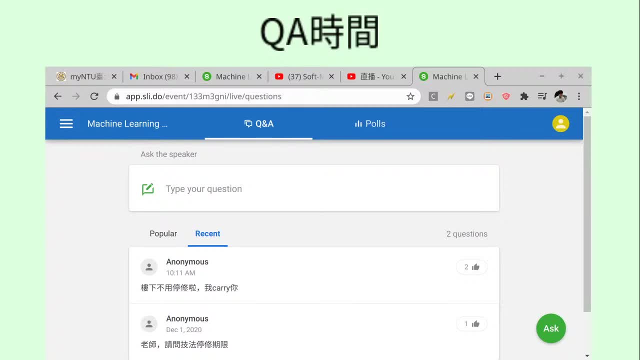 我們會請到一位 guest speaker 來跟我們分享他的經驗。. 然後我們會請到一位 guest speaker 來跟我們分享他的經驗。. 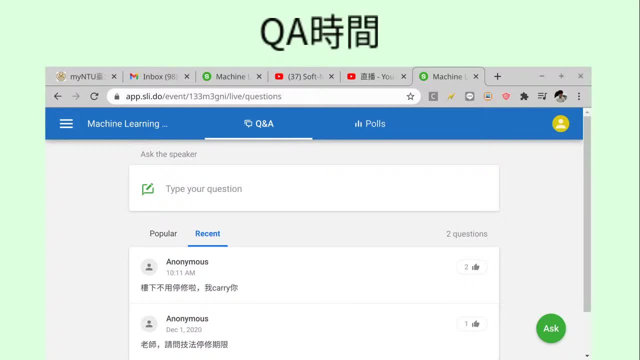 然後他之前跟我說他的課程裡面可能會講到推薦系統。 因為推薦系統畢竟是在業界裡面非常廣為被使用的一個機器學習的工具。. 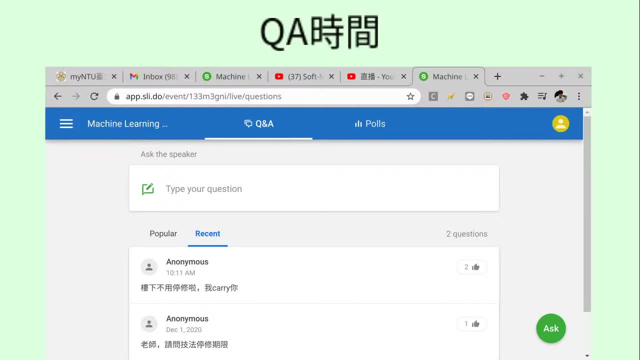 然後所以我就想先把那個部分先講。. 講完之後下禮拜的課程一我們請 guest speaker 來演講。. 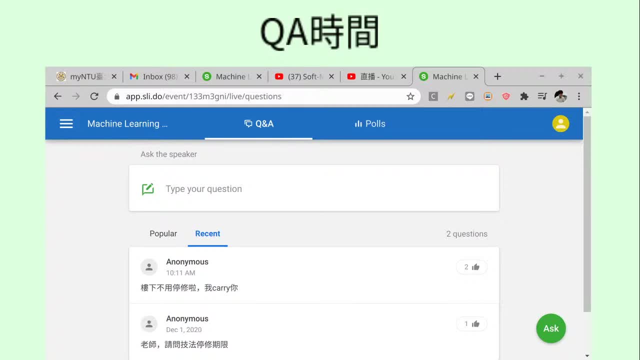 那下禮拜五的課程不是這個禮拜五下個禮拜五的課程我們會停課因為我在國際會議。. 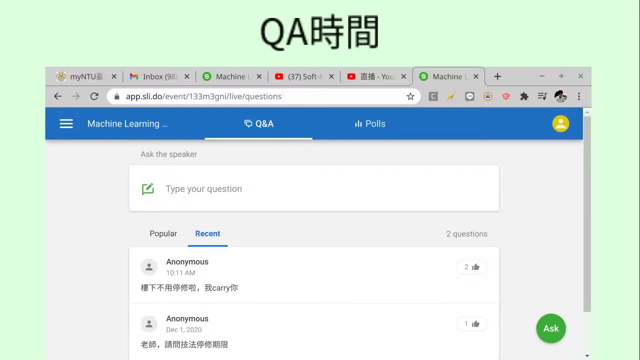 然後那在下禮拜我們才開始 resume 我們機器學習技法其他的課程。 所以我們的SVN大概今天會稍微告一個段落。. 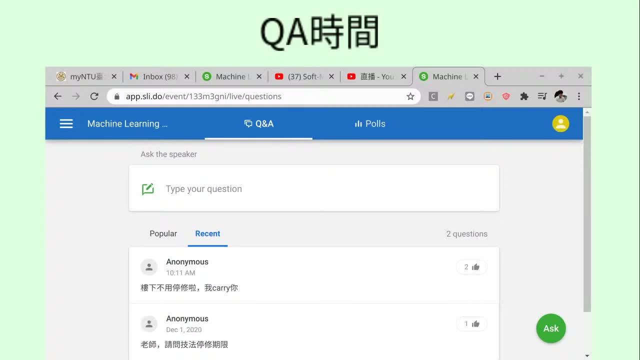 那如果這個等於是下禮拜的一個短暫的休息回來之後我們還有時間的話SVN其實還有一些內容是我們可以上的。. 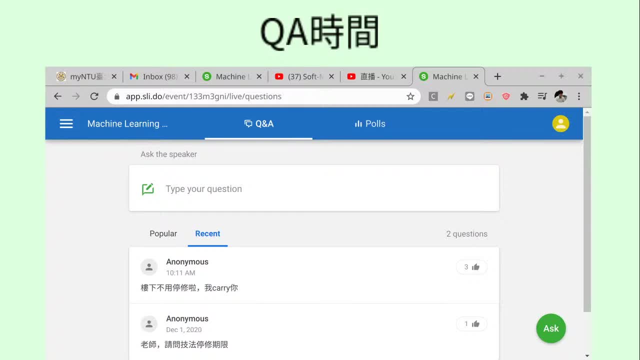 那我們再看看課程進行的方式因為後面的包括deep learning包括SVN其實我們都是選擇性的上。. 然後我們還有一些有趣的課程進行的方式因為後面的包括deep learning包括SVN其實我們都是選擇性的上。. 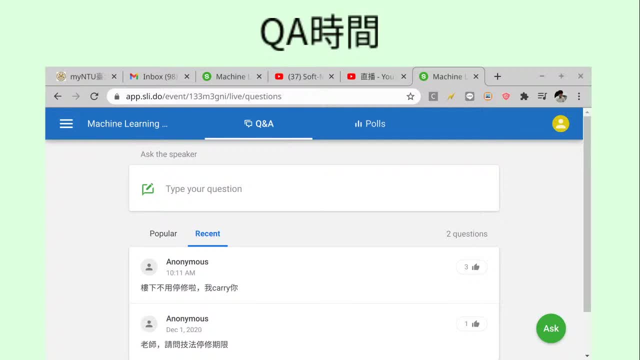 那所以這大概是我們課程的安排。 那一個要跟大家講的尤其現在在聽直播和看錄影的同學們就是我們下個禮拜二的那個 guest lecture我們不會有錄影也不會有直播。. 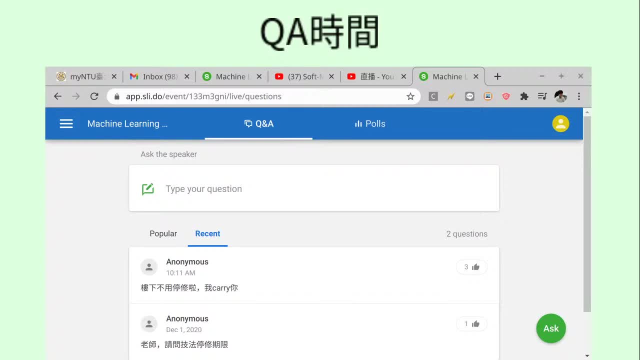 那最重要的原因是. speaker 說如果沒有錄影沒有直播的話可以講的範圍應該會比較廣一點大家的收穫可能會比較多一點。. 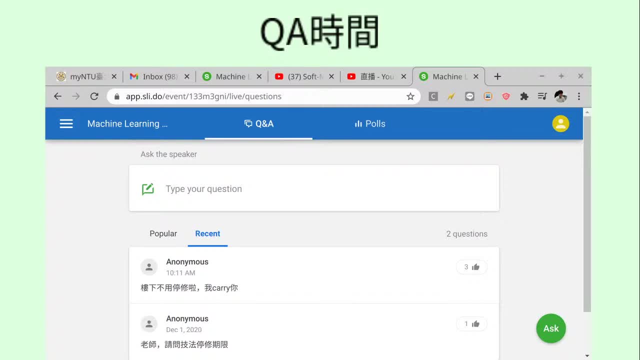 所以這個下禮拜我們是特殊的課程所以我們沒有這個錄影或直播。 那如果你真的很想要來聽 speaker 的經驗分享的話那請你務必要來到現場。. 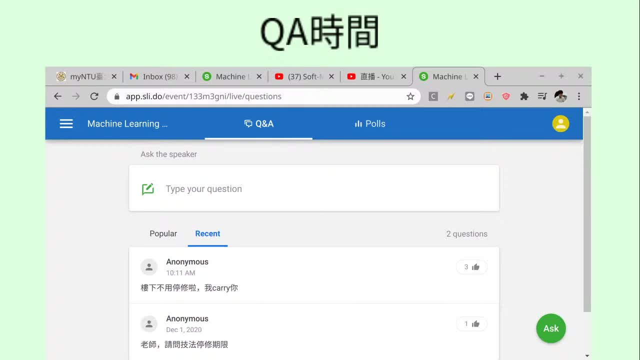 我還沒有講下禮拜的那個演講大概是什麼樣的內容。 我們請來的 speaker 是這個我在加州理工學院的同窗他是台大電機系畢業然後去加州理工學院念了 signal processing 的博士。 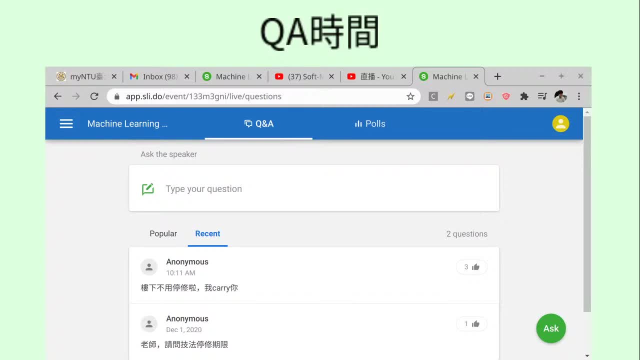 那念了博士之後他加入 Facebook當年是 Facebook 還剛起飛的年代。. 在他加入 Facebook 的前一年我其實去過 Facebook 面試然後那個時候其實 Facebook 不像大家現在看到的這麼大的公司已經開始向上了。. 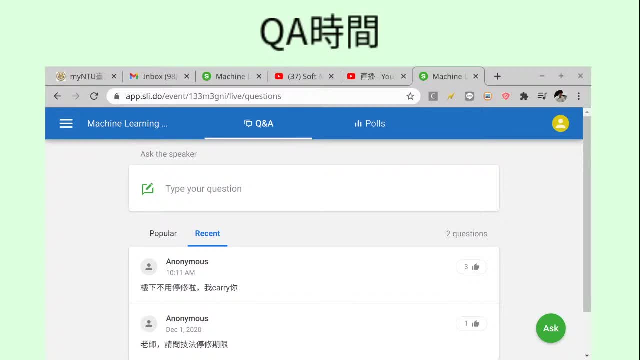 但是其實還有很多的瓶頸舉例來說我去面試那一年那時候 Facebook 推出了他當時的. 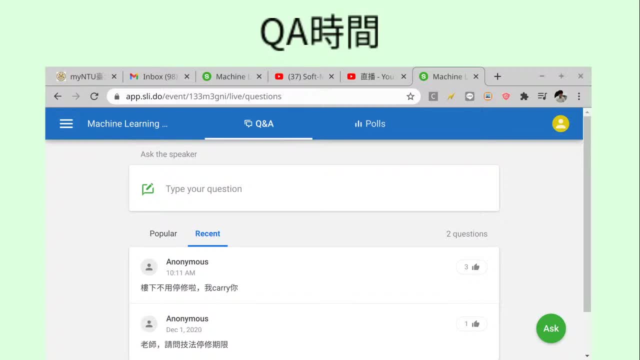 他當時所想像的社群網路裡面的廣告系統但是那個廣告系統遭受到很大的批評。. 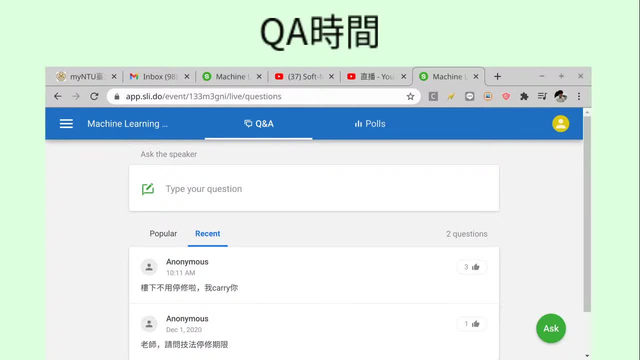 因為那時候 Facebook 想做的事情 roughly 是這樣就是 OK. 如果我今天喜歡某個東西例如說我買 Nike 球鞋好了. 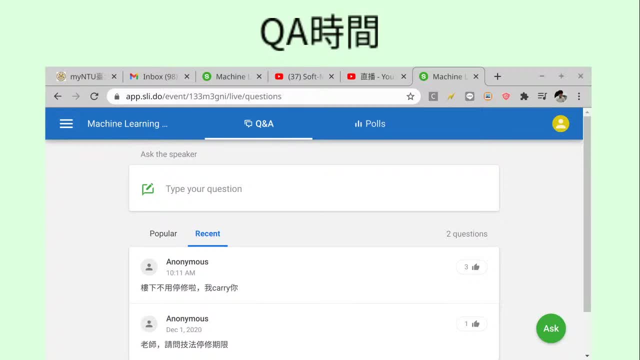 那麼這樣的話如果我朋友知道我買了 Nike 球鞋他覺得很好用那麼他們應該也會想要買 Nike 球鞋。. 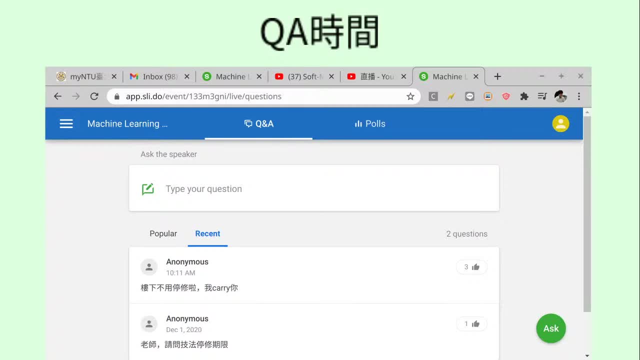 這當然是個很大的假設。 就是說, 興趣這件事情是可以在社群網路之上做傳播的。. 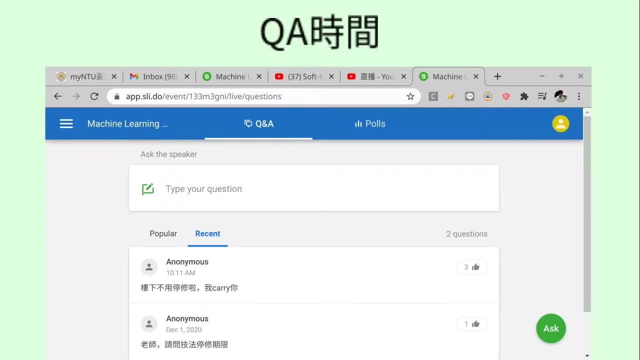 但是也衍生了很多其他的問題。 例如說, Nike 球鞋這種東西我可能沒有太不想讓朋友知道我買但是有一些我買的東西搞不好不想讓我的朋友知道。. 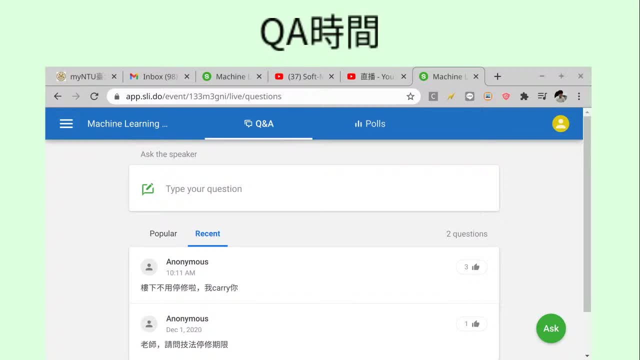 於是就有很多包括隱私權保護等等的問題。 所以那個 Facebook 第一代的廣告系統其實是沒有太成功的。. 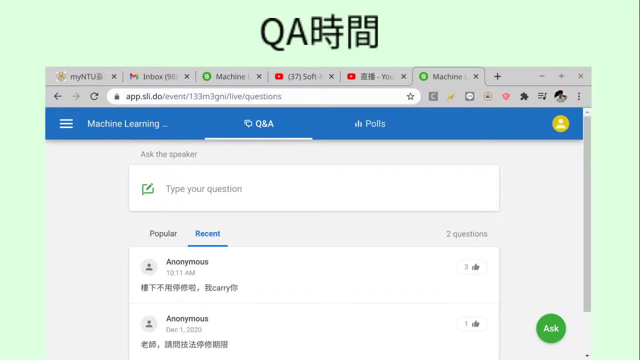 然後經過了很多不同的發展也許才像大家現在看到的 Facebook 系統一樣。 好那我那位朋友呢他就加入了 Facebook然後跟著 Facebook 一路一起起飛。. 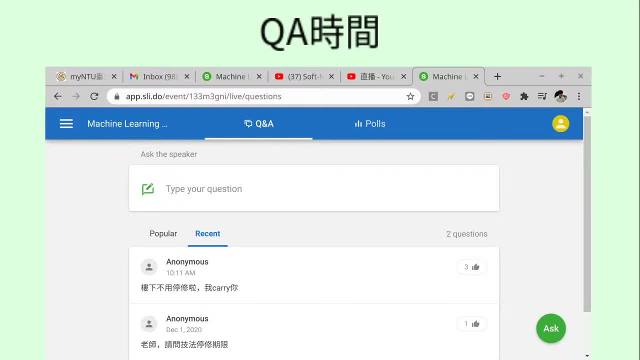 然後所以在 Facebook 吸收了很多經驗實際上在 Facebook 也見證了 Facebook 開始導入 Machine Learning 然後到大型產品的這些過程。. 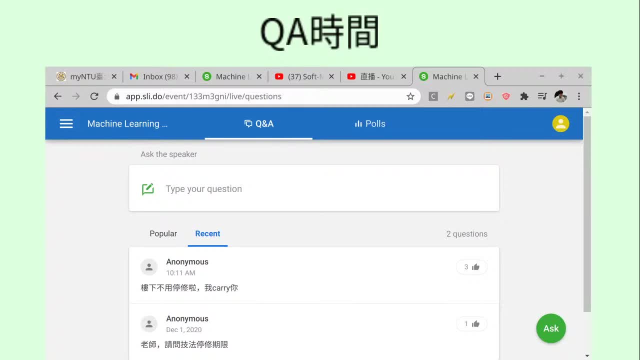 然後在 Facebook 進行的過程中呢他就開始做 Machine Learning 了。 在 Facebook. 若干年之後呢他離開 Facebook, 後來被挖角到 Grindr。. 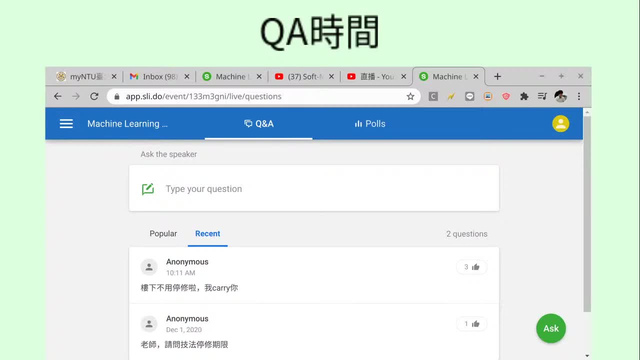 有的同學可能知道, Grindr 是同志的交友軟體。 然後他被挖角到 Grindr 當 Grindr 的 CTO然後後來是 VP。. 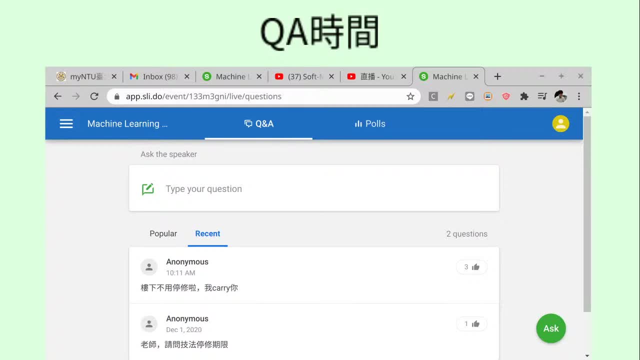 那他也成立了前幾年在 Grindr 的時候成立了 Grindr 的台灣研發辦公室。. OK, 那這個今年初吧。. 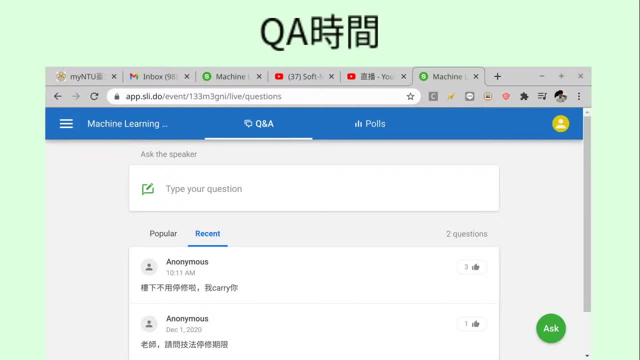 今年中的時候吧。 今年中的時候。. OK, 他結束了 Grindr 的這段旅程。 然後現在這個在台灣躲避疫情。. 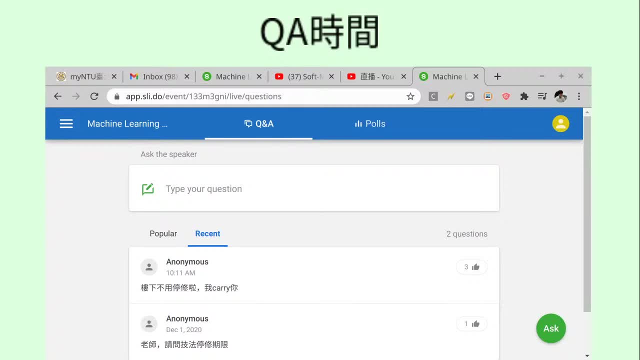 我們姑且這樣說好了。. OK, 然後那所以剛好他知道我們有這個課。 那他說他想要來分享一下不管在 Facebook 或在 Grindr 使用 Machine Learning 在 Real-World Application 裡面的經驗。 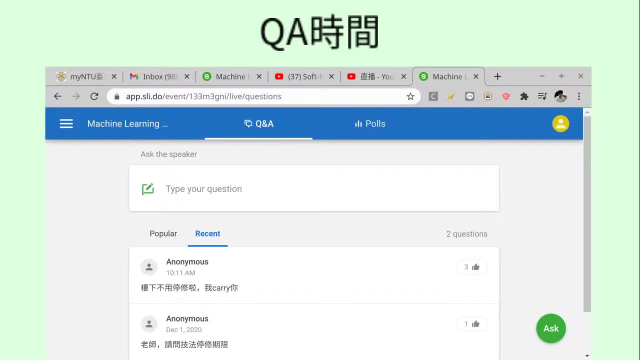 那我們這課裡面當然我們提到比較多的也許 Theory, 也許是 Algorithm。 或者是 Application 的時候是部分是稍微少一點。. 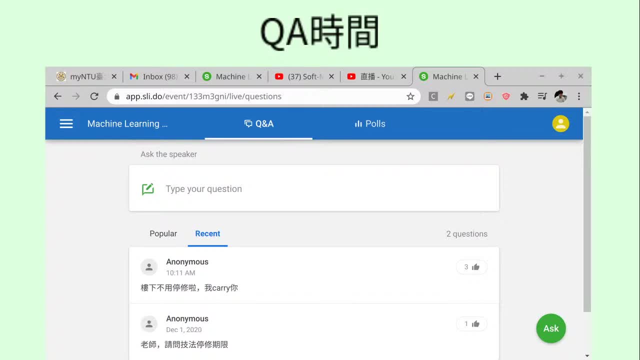 然後所以我也覺得這是個很好的機會。 我們很多同學如果對 Machine Learning 在業界是怎麼用有興趣的話。. 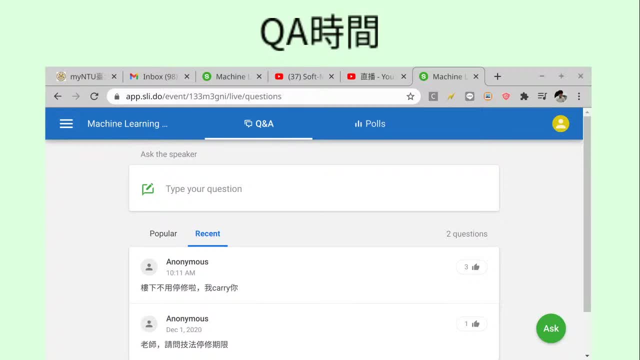 當然你可以問我我可以告訴你 APR 是怎麼用。 或至少在保密條款以內我可以告訴你在 APR 是怎麼用的。. 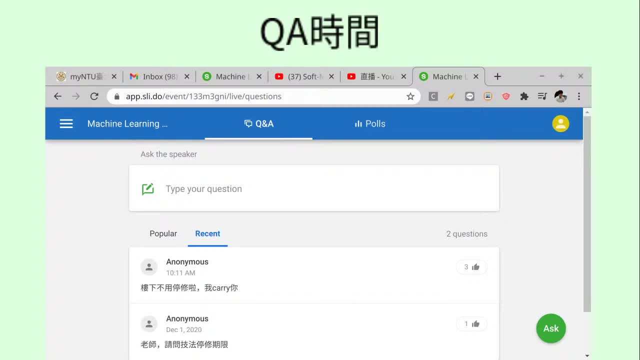 OK, 那但是有一些不同的這個業界角度來分享。 尤其是我們的 Speaker。 我們 Speaker 叫陳俊揚。. OK, Scott Chen。. 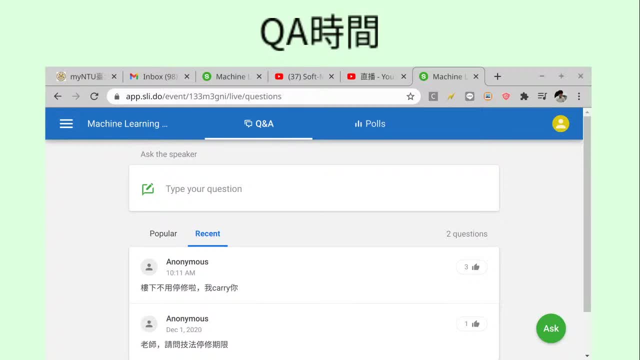 然後 Scott 他這個待過更大型的這些公司。 那我們希望他的經驗對同學們會有幫助。. 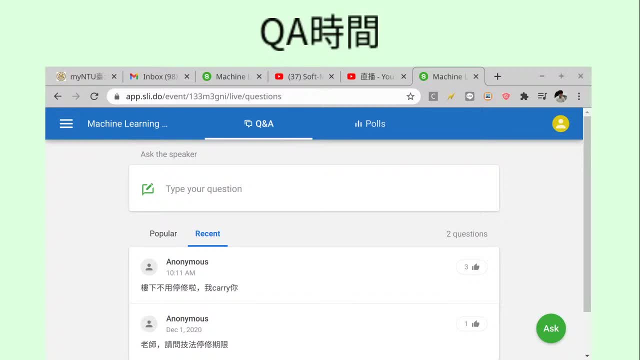 OK, 所以這是有關下個星期二的這個課程的部分。. OK, 好那請說。. 回應嗎? OK 好我要怎麼解決呢. 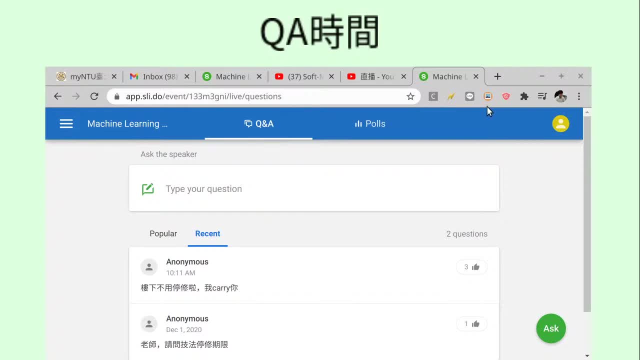 看一下。 我忘記我上一次是關了哪一個就不會有回應了。 All These Monitor 都是這個。 Recording 好。. 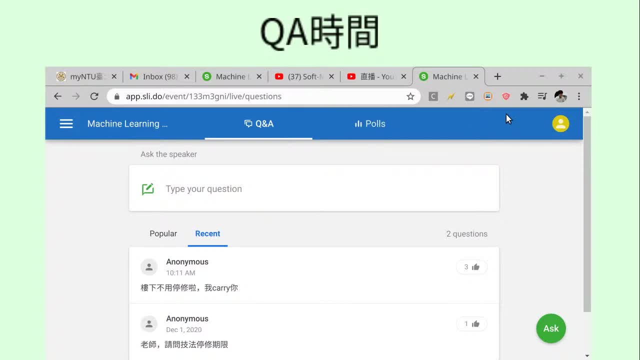 I don't know, 是不是先關這個就。 好像不是。 讓我來想想。 我們先把這個關起來。. 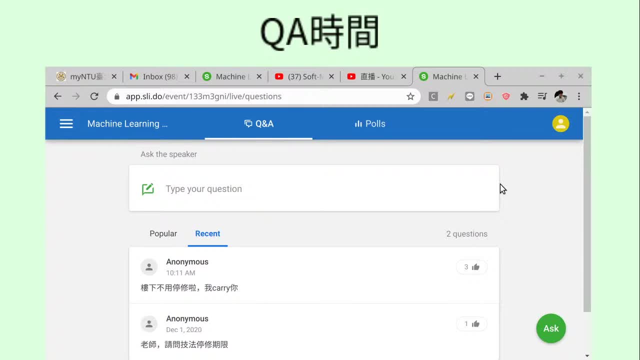 OK, 把這個關起來。. 等一下開影片的時候再打開就好。. OK, 好來還有什麼問題嗎? 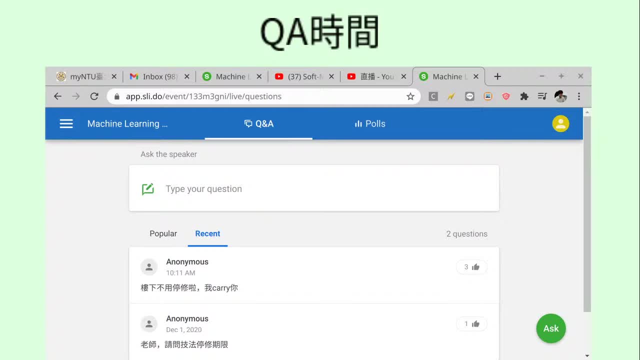 OK, 好沒有的話那我們就開始今天的課程的部分。 我們上一次的課程呢到我們跟大家講了。. 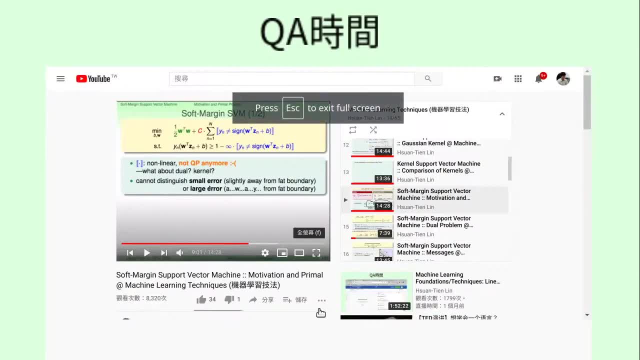 OK, 所謂的 Soft Margin, SBM。 我們到底是怎麼開始的? 我們說我們一開始想要做的事情呢是。. 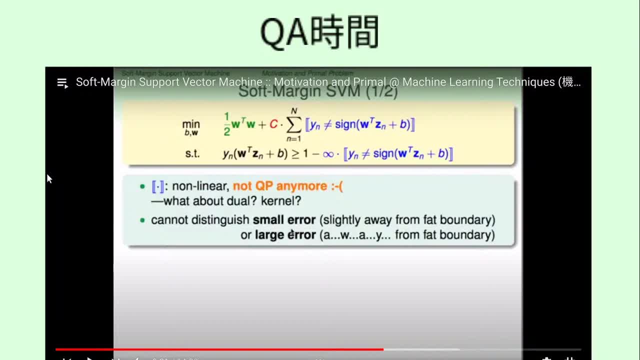 我現在才發現我沒有接螢幕。 現場同學想像力真好。 我們沒有感覺到任何不對勁之處。. 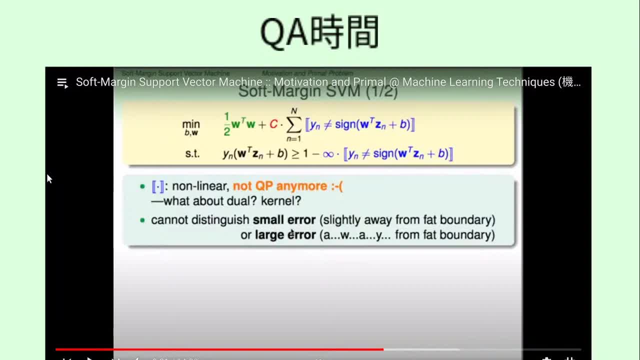 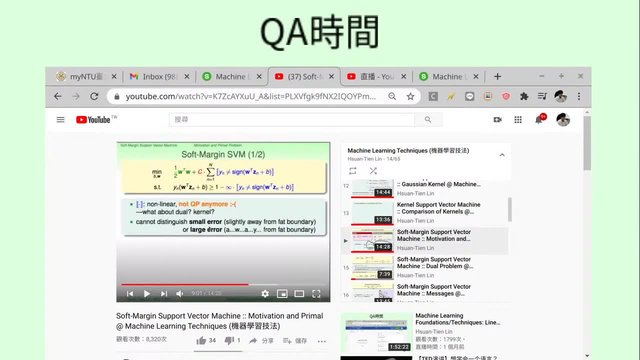 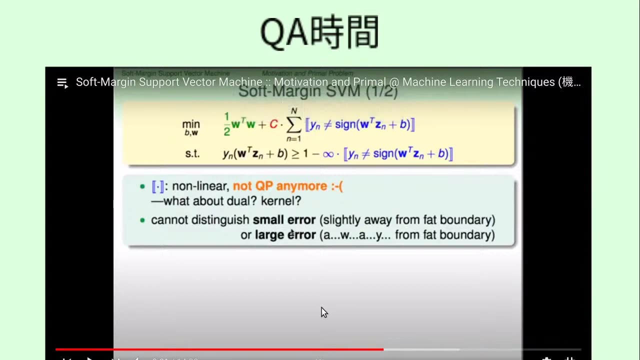 OK, OK, 好那我們上一次跟大家分享的事情呢是我們怎麼樣導出。 OK, 或怎麼樣設計出一個 Soft Margin的 SBM。. 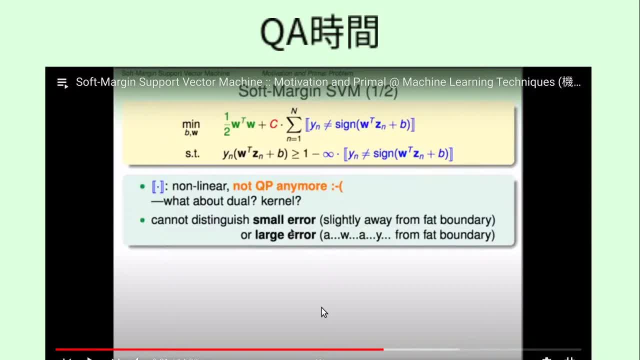 我們說我們一開始的出發點是從 SBM, 原來的 Large Margin問題。 然後說那我們能不能舉起手放棄一些點。. 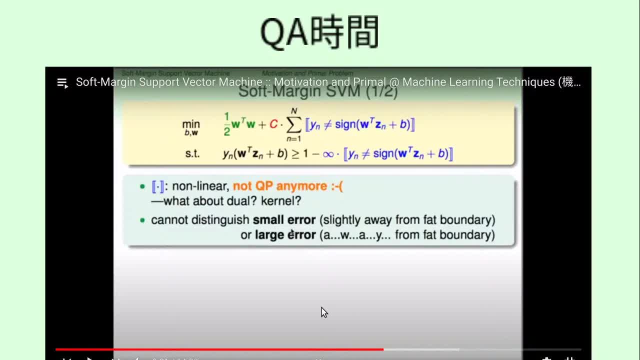 OK, 放棄一些點說你錯了錯了就算。 OK, 錯了我扣你一些分數。. OK, 但是我不是完全不允許犯錯。. 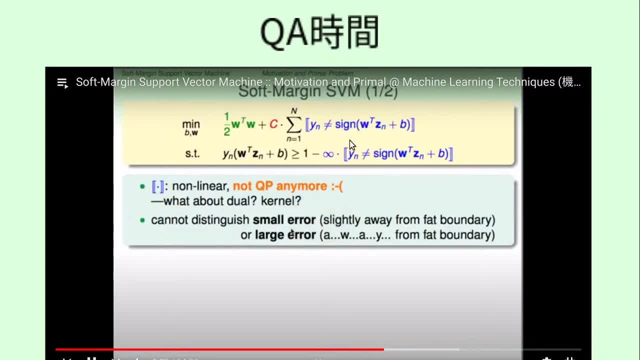 OK. 那從這樣的出發點呢我們寫出了這個上面的這個 Optimization 式子。 說我們把錯誤的個數 OK 拿去當作懲罰項。. 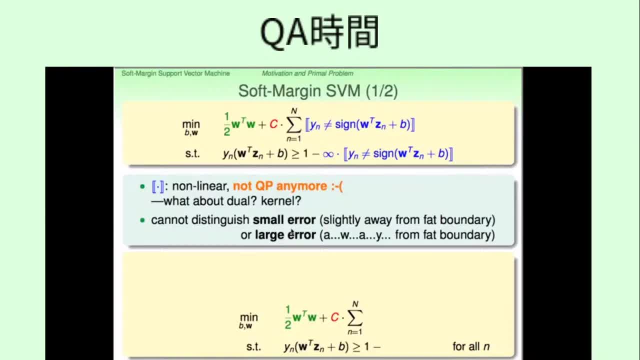 然後呢另外呢我們在條件裡面說好那錯了就算錯了。 就當這個你。 反正你就違反 Margin。. 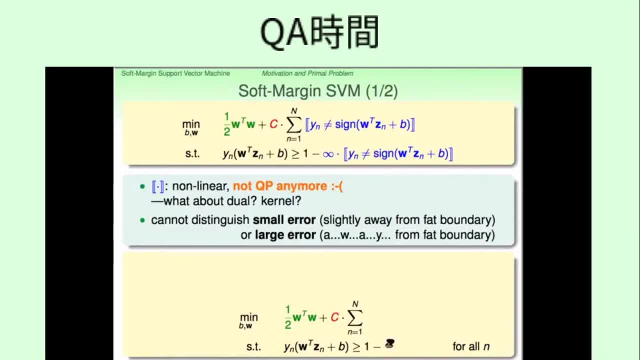 OK, 那但是我把它加到那個裡面。. OK, 那麼這個我們等一下會做的事情呢是我們上一次其實已經放了。. 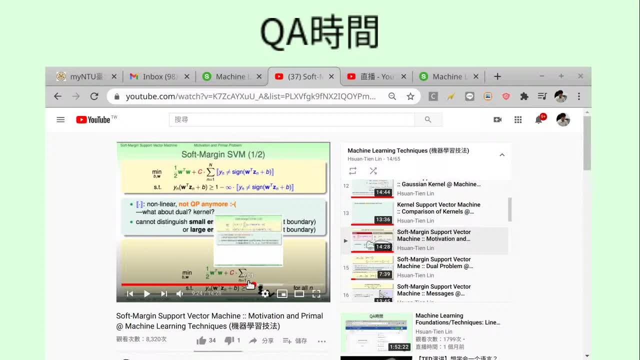 但是我想說讓大家稍微這個回憶一下。 所以我們會把這個事情說這事情有一些缺點。. 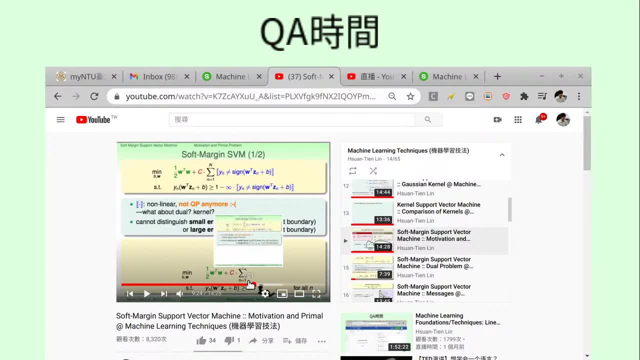 OK. 例如說它是 Discrete 的。 它不好 Optimize 等等的。 或它沒有考慮到: OK, 到底你今天是大錯還是小錯。? 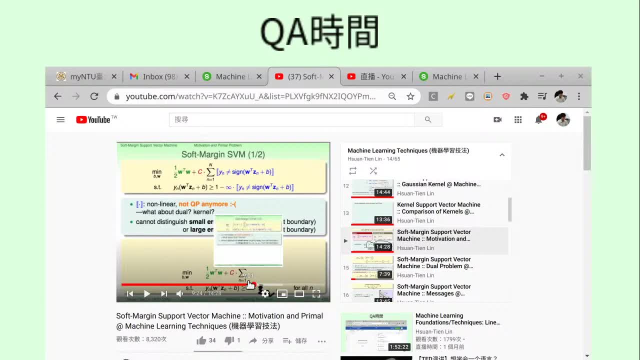 你離 Margin 是很遠還是很近。 然後所以我們做了一些選擇。 然後所以我們做了一些修正。. 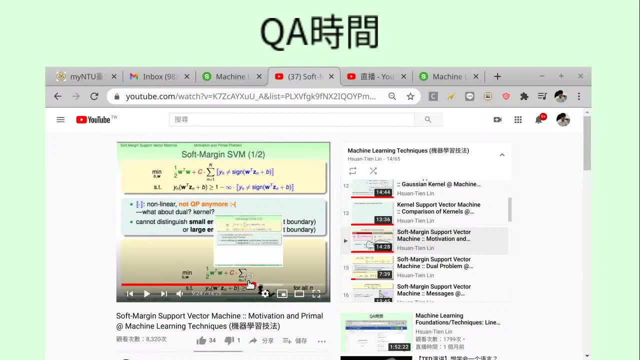 基本上來說我們把錯誤的那個項 OK 定義為離我們想要的那個 Margin。 我們想要的 1 的那個數字到底多遠還是多近。? 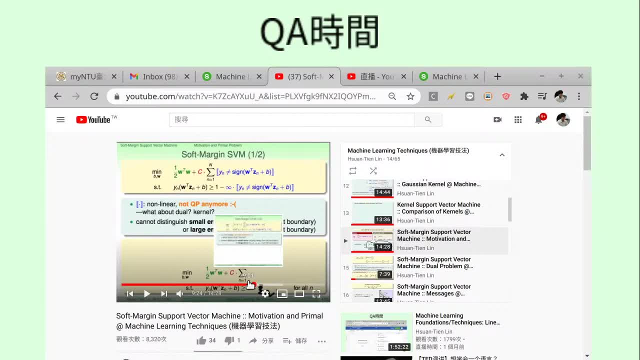 OK, 然後把它放進去懲罰。. 那這部分的推導我們就從等一下就從這邊開始放下去。. 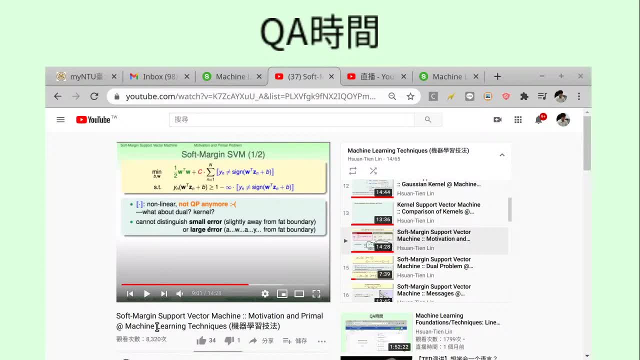 說好那我們怎麼得出一個 Quadratic Programming 的問題。 OK, 基本上我們加上錯誤項是一次項的時候。. 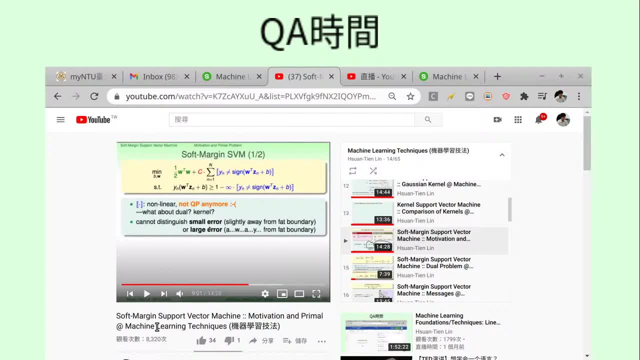 就會有個 Quadratic Programming 的問題。 然後那有 Quadratic Programming 的問題。 我們下一步就可以來說我們怎麼透過我們已經學過的 QP 的那些技巧。. 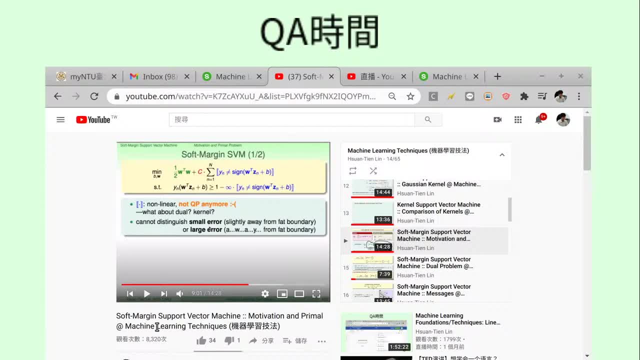 把它變成 Dual。 只要能夠把它變成 Dual。 我們學過所有這個 Kernel 的那些東西就統統可以用了。. 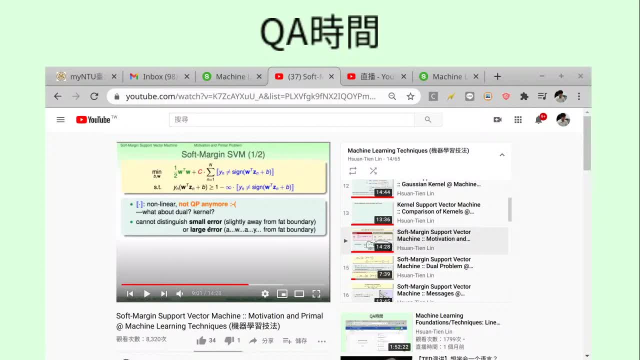 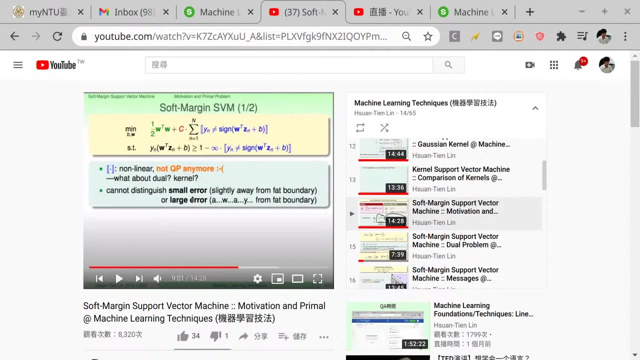 OK, 所以這是有關 Soft Margin SVM 的部分。 好所以我能夠做的是先把這個打開。 會想辦法區分出小錯跟大錯。. 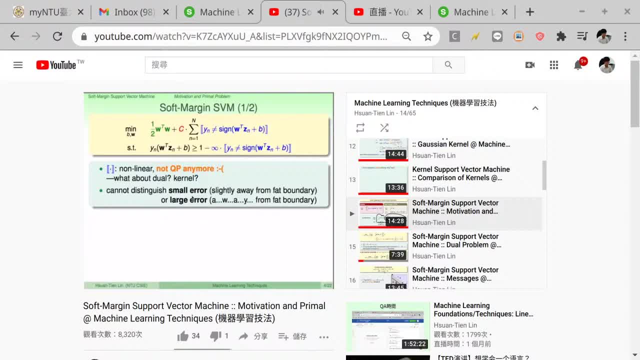 而且它可以維持 Quadratic Programming 的特性。 這個新的事實長這個樣子。 好所以我們現在要最佳化的事情跟剛才一樣。. 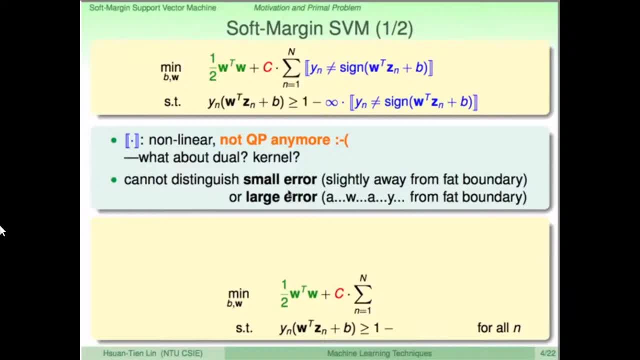 我們會有這個錯誤的部分。 我們要區分小錯或大錯。 我們把錯誤記錄在一個叫做 Casin 的變數裡面。. 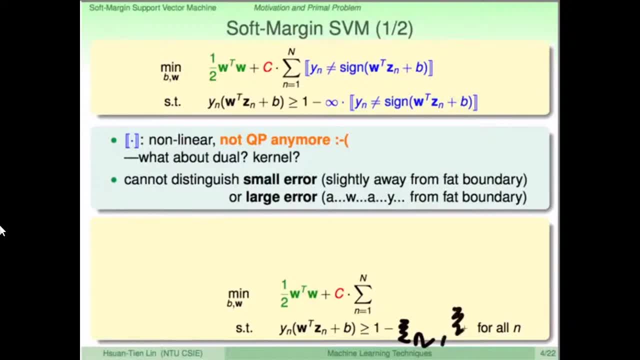 這個 Casin 的變數是大於等於 0.. 這個變數說什麼 你離我想要的那個值。. 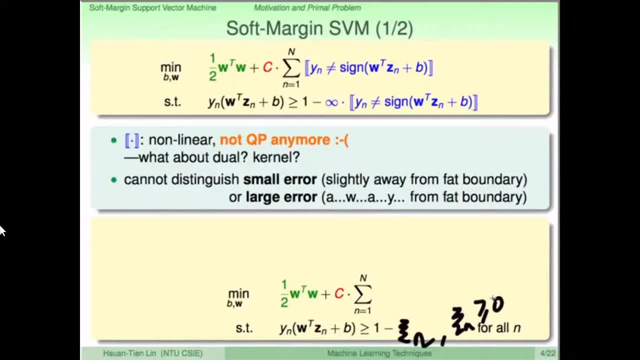 我想要那個值是 y, 乘上分數是 1。. 你離我想要那個值到底有多遠? 好所以你如果離我想要那個值你如果那個 1 很近的話。. 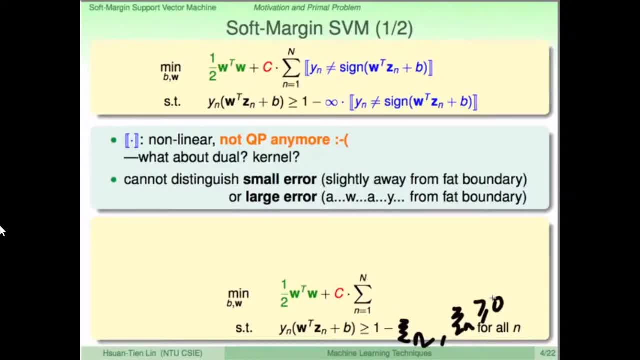 我說你是小錯。 你離那個 1 很遠的話。 我覺得是大錯。 然後就怎麼樣. 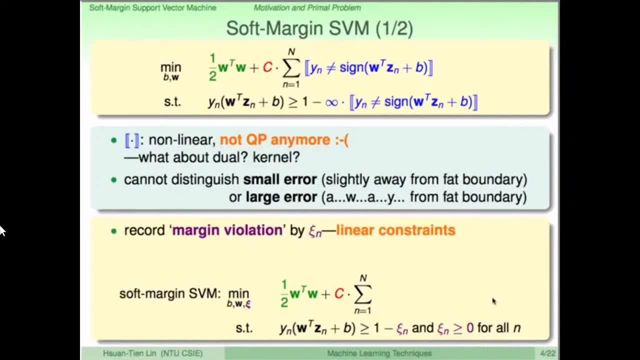 然後把這個記下來之後。 我們就可以做一件事情。 說我們把這樣的錯誤放到我們. 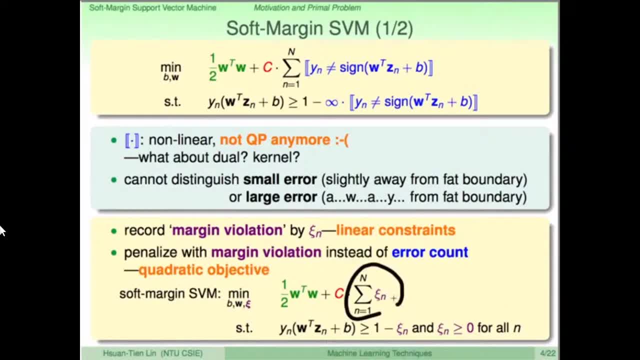 了明一脈的事情裡面。 也就是我在這裡加上了這個 Casin。 好所以我們記錄。 我們懲罰的事情是你犯了多大的錯誤。. 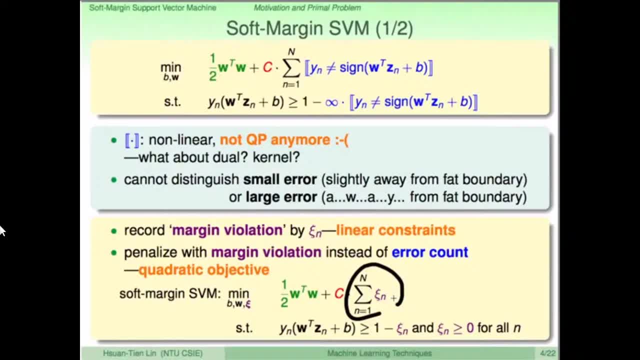 而不是你犯了幾個錯誤。 大錯跟小錯衡量起來不一樣。 這樣更改對我們有什麼好處? 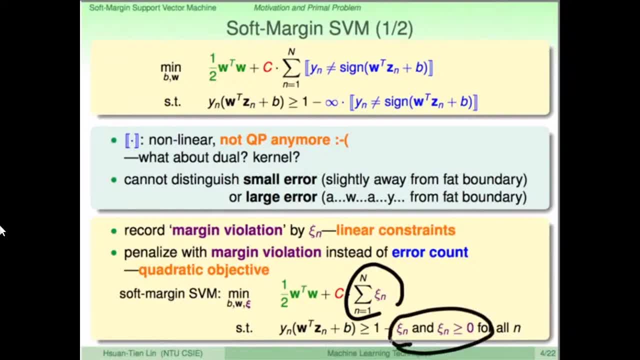 我們看看條件的部分。 條件的部分我們加上了 Casin, 這樣的變數。 但是呢我們加上了變數。. 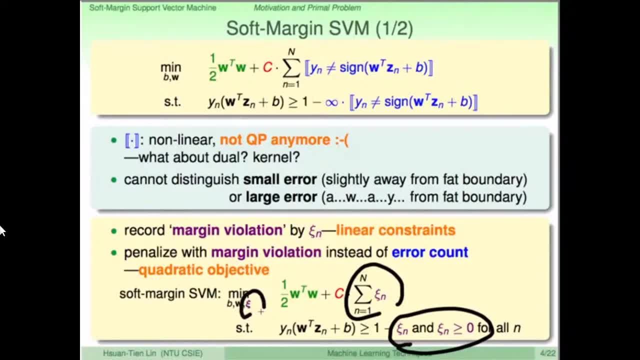 最後計算的這些條件是指是 Casin 的一次式。 一次式好。 QP 裡面需要所有的條件都是一次式。 我們在 QP 要最佳化的東西裡面。. 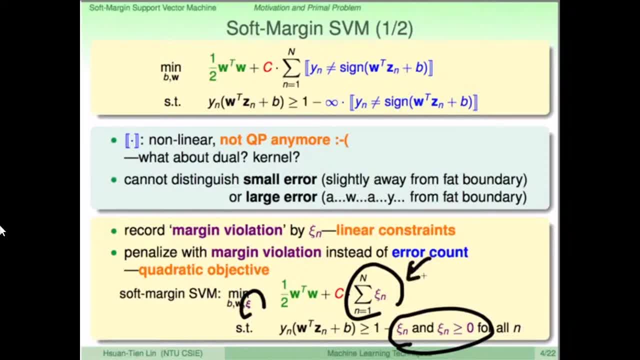 加上了 Casin, 加起來這個東西。 這個是 Casin 的什麼 一次式。 原來是 W 二次式。 然後加上 Casin 一次式。. 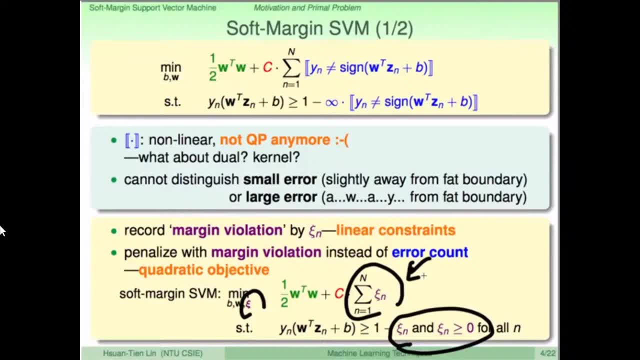 整個來說是 W 跟 Casin 的二次式。 所以這個問題還是一個 QP。 我們維持了 Quadratic Objective Linear 的 Constraints。. 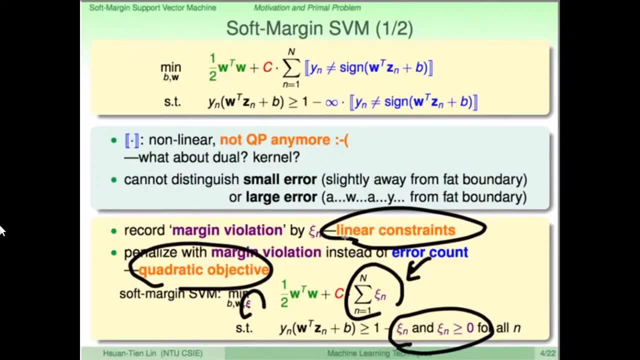 所以這個要解 Pocket 跟 Hard Margin 真正的合體不好解。 就像說我們之前, Pocket 說 Card is NP-hard 才能夠解決的問題。. 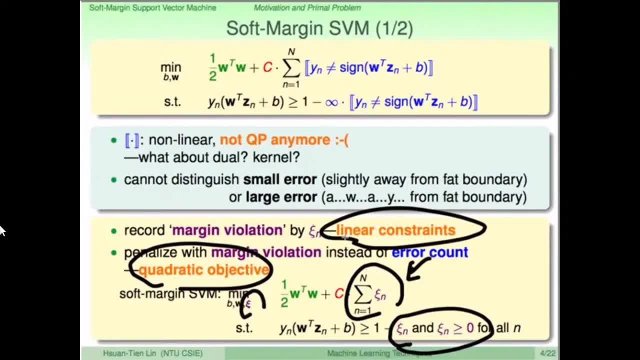 好所以這個回頭來說。 我們定一個新的問題。 它跟我們剛才那個合體有類似的地方。. 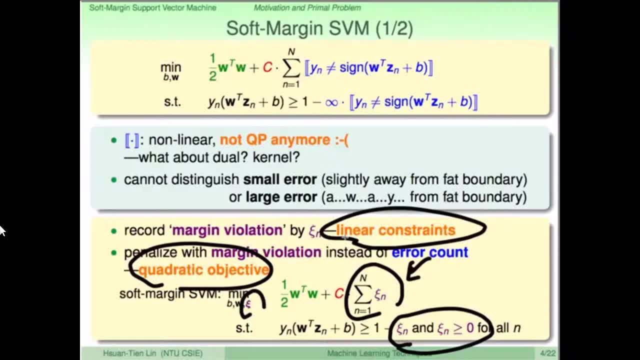 我們要記錄錯誤。 然後我們在要最佳化的東西裡面要有跟 Margin 有關的像還有跟錯誤有關的像。. 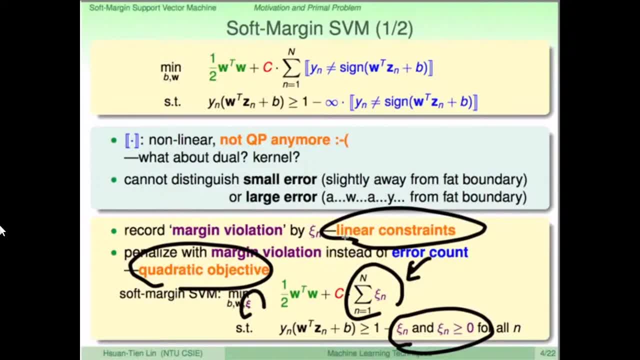 不過我們現在把錯誤改一改。 我們說那個錯誤不要再是非黑即白。 我們容許一些灰色的地帶。. 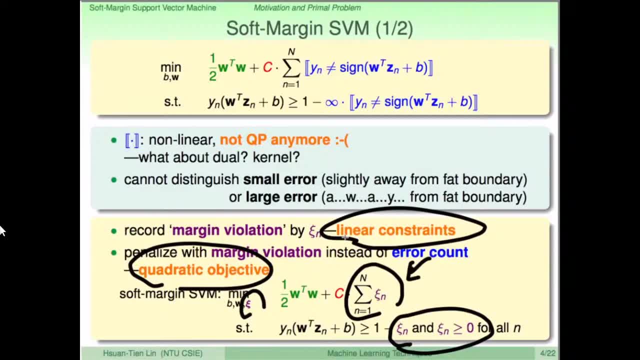 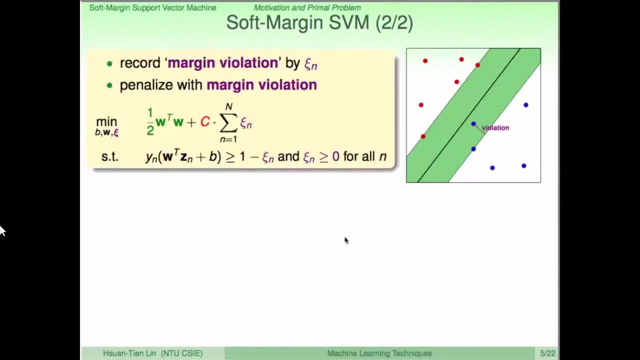 大錯小錯把它好好地算好。. 之後把它加起來當做我們要懲罰的錯誤像。 好所以這是我們新的式子。. 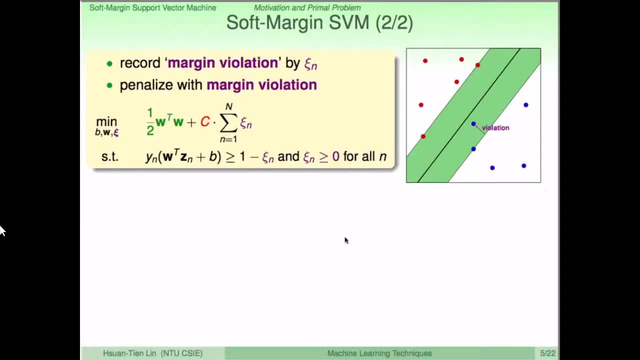 我們把用 Casin 這樣的變數把 Margin 的錯誤記錄下來。 我們叫做 Margin Violation。 意思是說我們想要 1, 但是你違反了多少。. 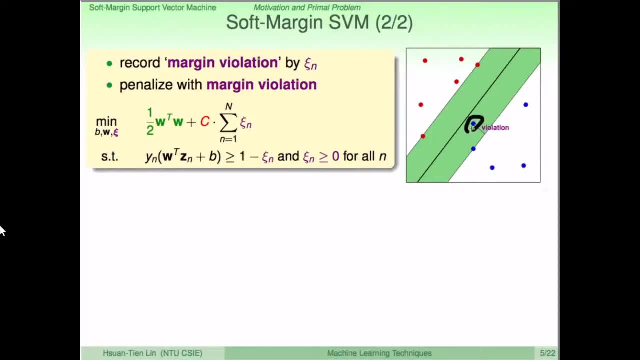 舉例來說像這個點。 這個點現在落在我們的 Margin 裡面。 落在我們那個中間想要那個胖胖的邊界裡面。. 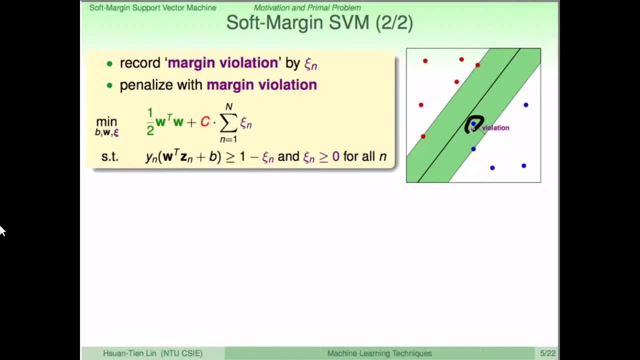 所以它違規了。 它違規了多少? 我們想要 1, 所以我們想要它在這個 Margin 的外面。. 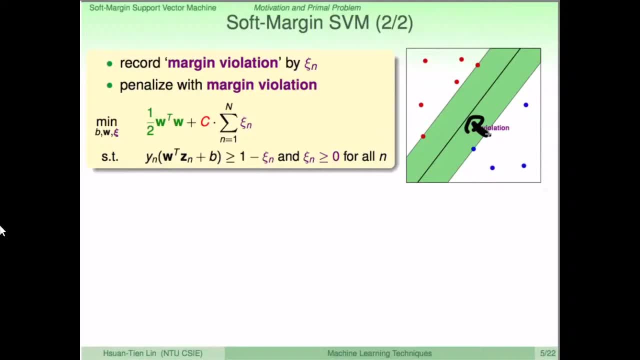 那麼它跟這個邊界跟胖胖的邊界的距離就是它違規的數量。 所以我們把這個數量記錄下來。. 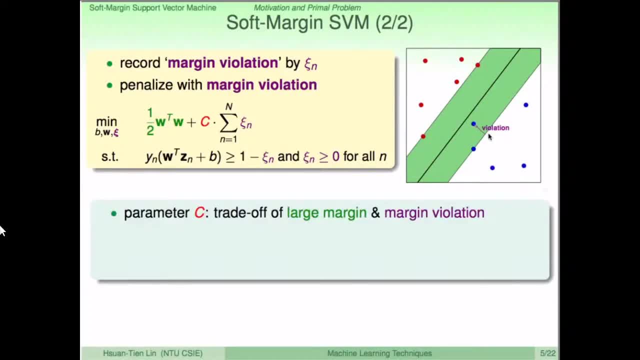 然後納入我們要最佳化的標準裡面。. 好那 C 控制什麼 C 現在就控制我們到底要多胖的邊界。. 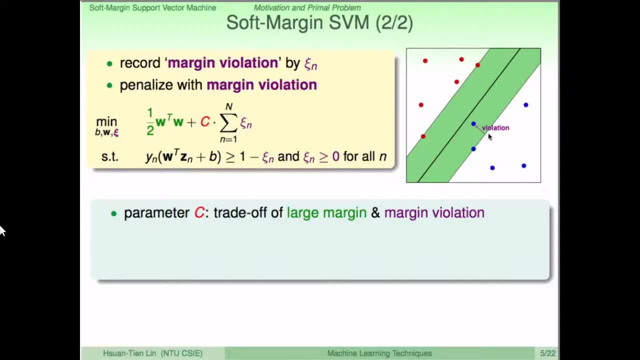 還是我們是非常的在乎我們希望 Margin 的 Violation。 違反 Margin 的這個情形。 越少越好。 那如果越大的 C 就代表我不要任何違反 Margin 的情形。. 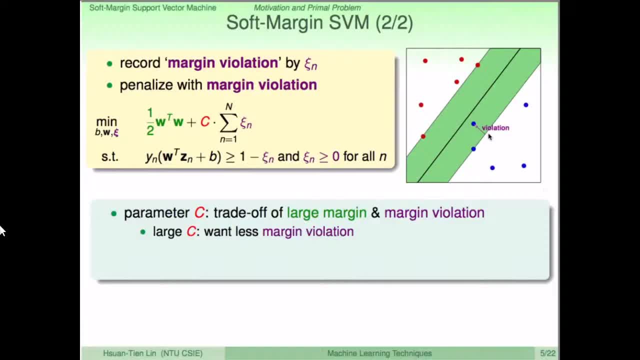 我寧可這個邊界瘦一點沒關係。 但是不要任何違反的地方。. 那如果今天是小的 C 呢, 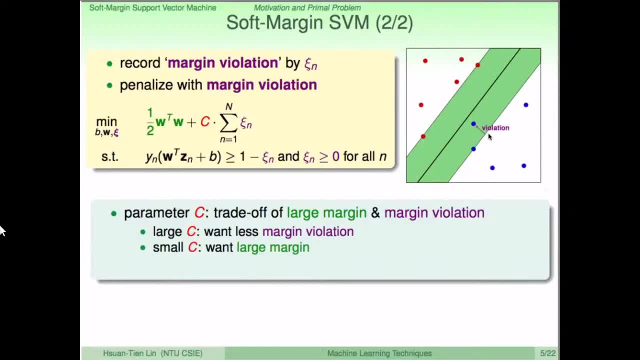 邊界胖一點。 不過可能很多人違反。 那就算了。 但是邊界胖一點這是我想要的。 所以 C 控制的是這樣的概念。. 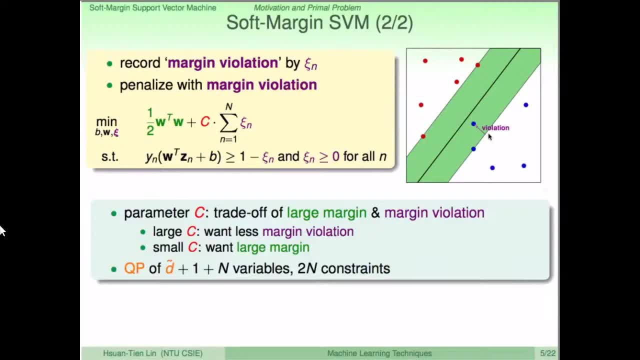 好那這個新的問題是什麼 這新的問題我們看有多少變數。. 我們一樣有 W. 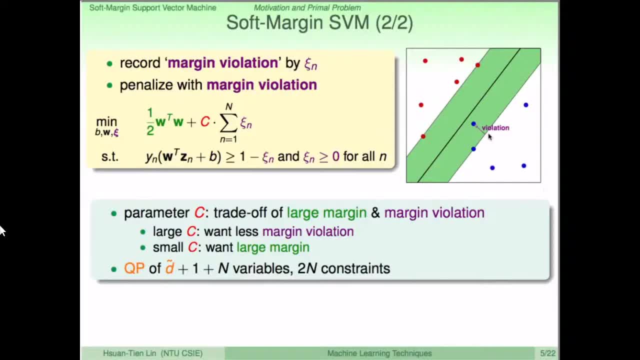 一樣有 B, 所以這是 D 跳塔加 1。. 那我們多了 N 個變數。 這 N 個變數用來記錄什麼? 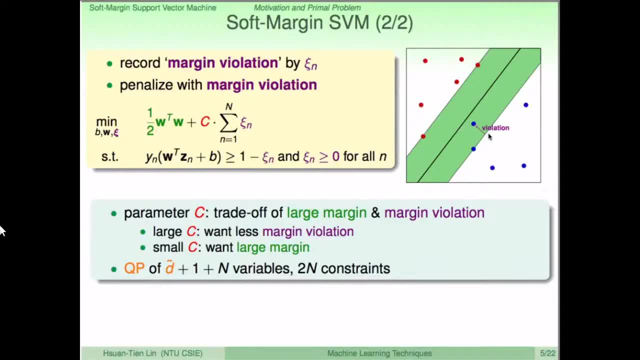 記錄違反了每個點到底違反了多少的 Margin。 所以是 D 跳塔加 1 加上 N。 但是它還是個它有密碼還是個二次式。. 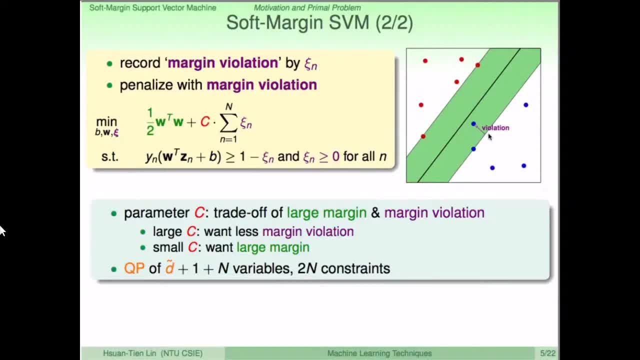 它的條件還是通通是一次式。 所以它是一個二次規劃的問題。 條件的數量多了一點。. 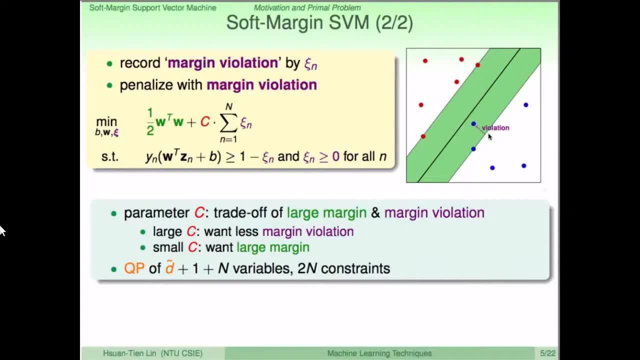 就是因為我們在記錄這個違反的數量的時候。 我們說只要有違反我們才記。 可是大於 0, 我們才記。. 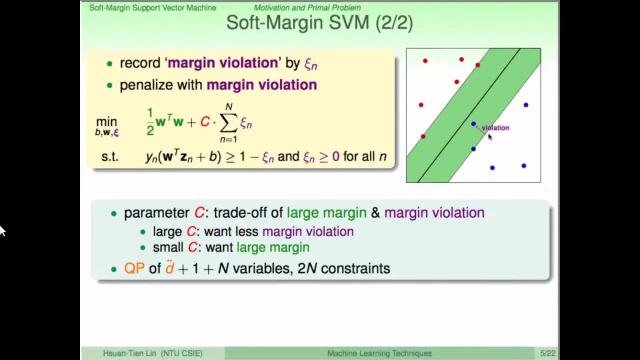 可是小於 0, 我們就不記了。 所以可是一定要維持那個大於 0 的地方。 所以我們多了 N 個條件。. 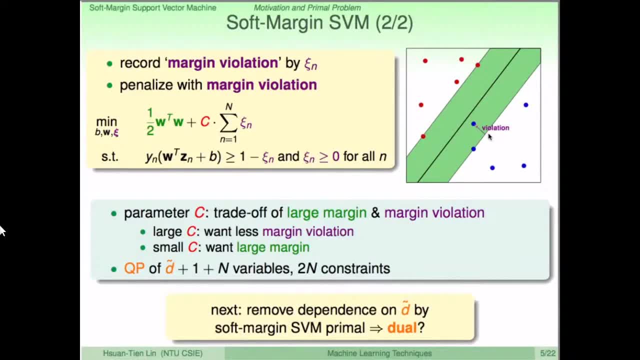 好那我們再來可以做什麼: 寫出一個 QP。. 你現在就會寫出一個 QP。 你就可以寫出另外一個 QP。. 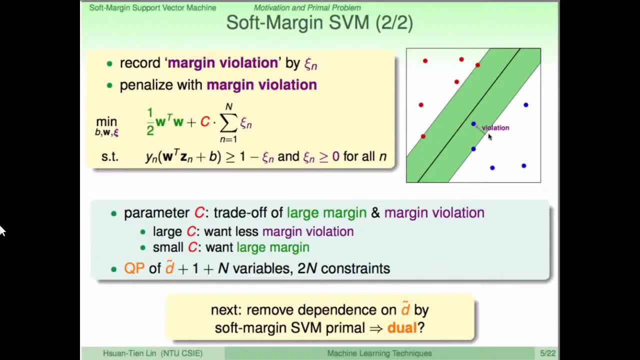 哪一個 QP 對偶的那個。 對偶的那個 QP。 做一做在 SBM, 這樣的問題裡面做一做。. 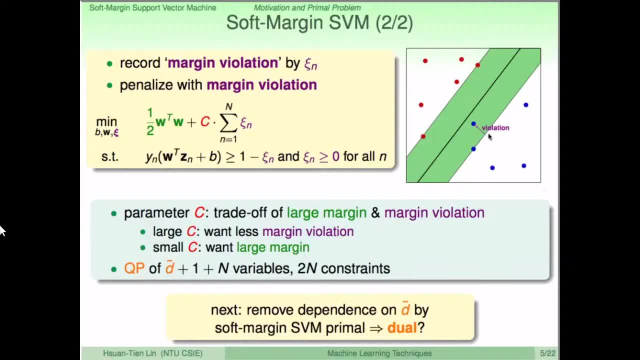 你就可以把對 D 跳塔的依賴拿掉了。 也就是我們上一次講的 Kernel Trick。. 好所以我們來看看這個問題。. 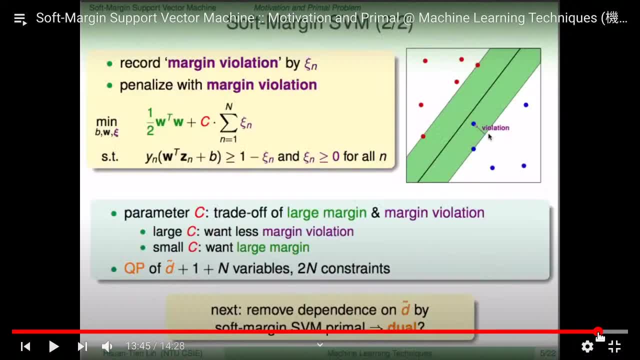 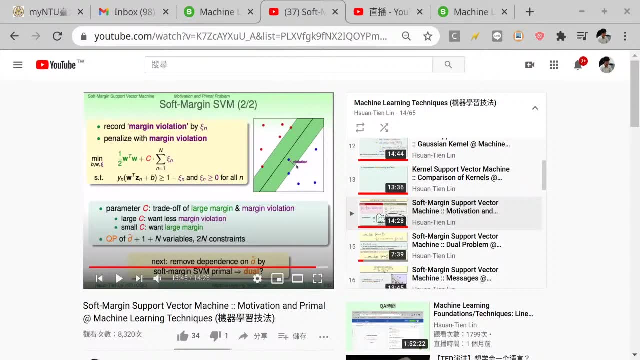 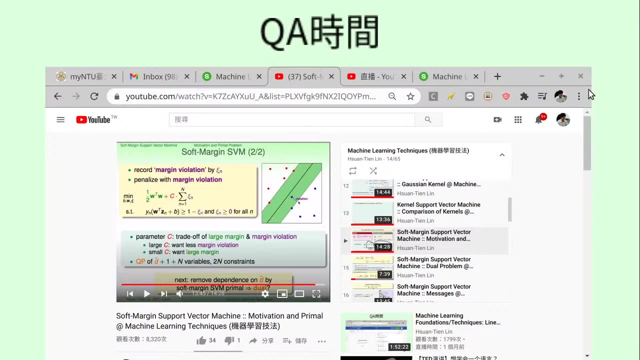 好所以就到這邊。. OK, 好先呢我們這個 Refresh 一下大家的 Memory 說。 這個我們已經導出了這個 SBM 的 Soft Margin, SBM 的 Primal。. 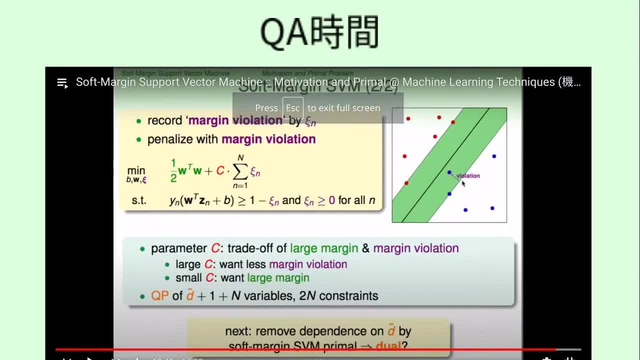 它裡面的東西意義其實對我們來說。 唯一新的只有 QC. OK, 這些變數。 OK, 那個字念 QC。. 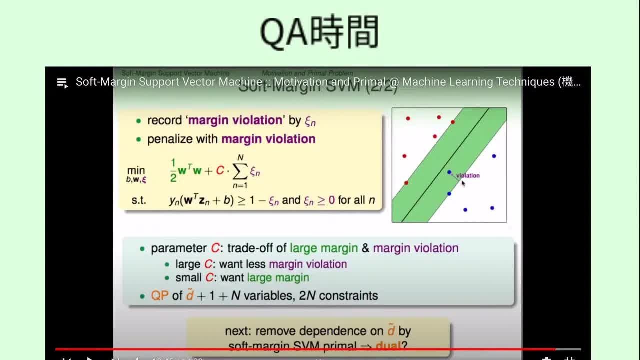 那 QC, 這些變數呢。 代表的意思就是你今天任何一條線。. OK, 那麼你都可以這個算出來。. 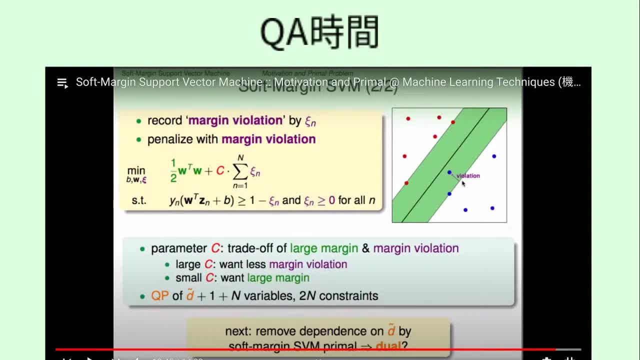 到底它有哪些點是 Violation 的。 OK, 那那個 Violation 的幅度。 那個 Violation 的大小。 OK, 就被存在 QC 這個變數裡面。. 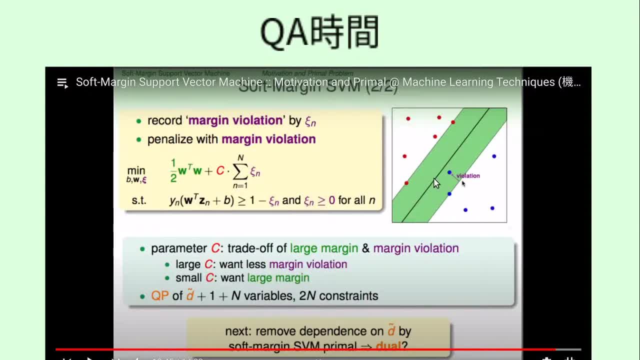 OK, 那如果好像這個是個胖胖可能胖胖的邊界。 那如果呢是說那個藍色點都在胖胖的邊界的這個正確的外面。. 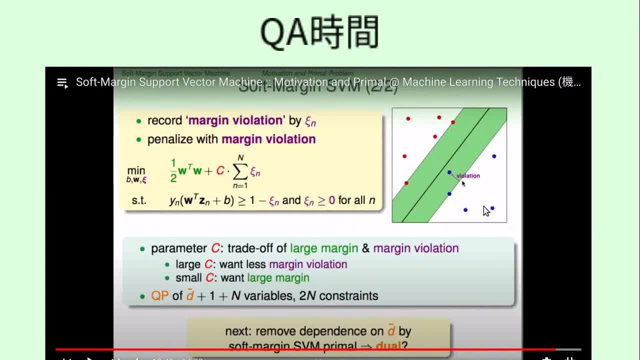 那它就沒有任何的 Violation。 那如果它落在錯誤的這一邊。 那就有一些 Violation。 當然如果你今天有一個藍色的點落到對面去。. 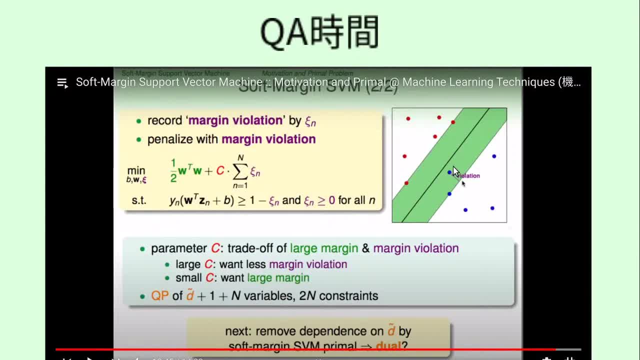 那它就有很大的 Violation。. 那所以我們的 Soft Margin SBM 其實就是這個在我們原來想像 Hard Margin SBM 之上。. 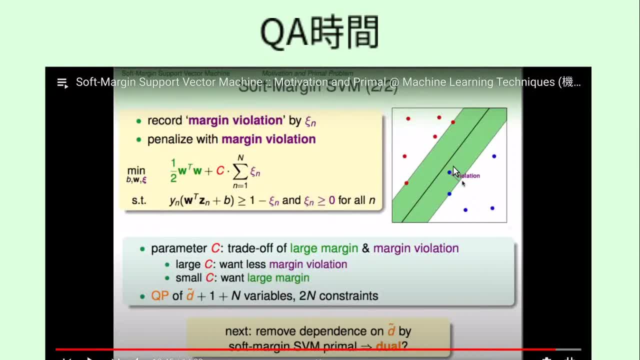 然後加上把這些 Violation 記錄下允許這些 Violation。 而且把這些 Violation 記錄下來的另外一個 QP。. 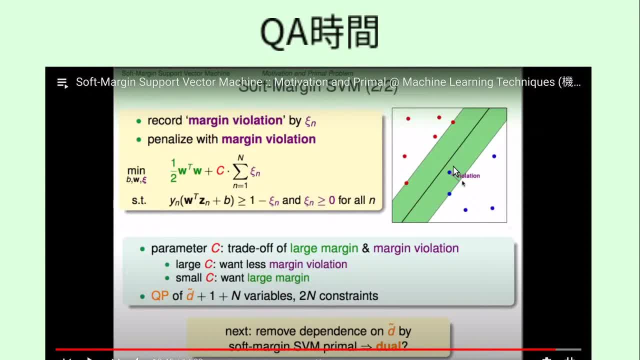 然後那我們用 C OK 的這個參數來有點像控制說。 那到底我們在不在意這個 Violation。. 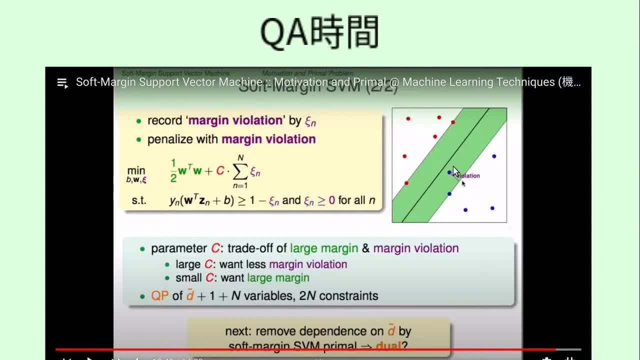 如果你想像說這個言行峻法。 OK, 就是一點點 Violation 就會被收很貴很貴的 C 的錢。 OK, 那麼可能我們的結果就比較接近 Hard Margin。. 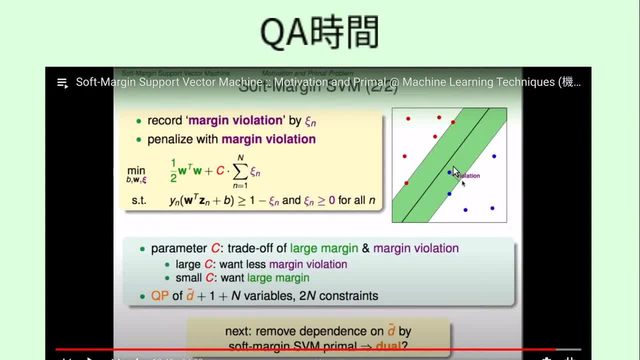 OK, 意思是說我們盡量盡量要避免這個 Violation。 那如果你今天 C 很小。 OK, 代表說你願意讓你的邊界 OK 長得寬一點。. 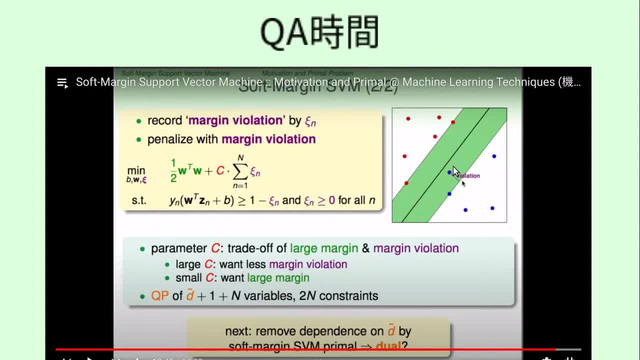 OK, 讓你的 Margin 長得寬一點。 長得胖一點。 然後但是那個很胖的邊界。 那個很胖的邊界裡面可能有很多的 Violation。. 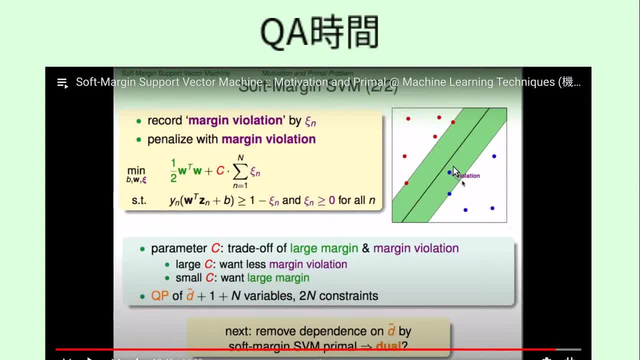 也許都是小錯不一定。 OK, 但是這個你會付出一些些 Violation 的代價。 好所以這是我們這裡的新的 Trader。. 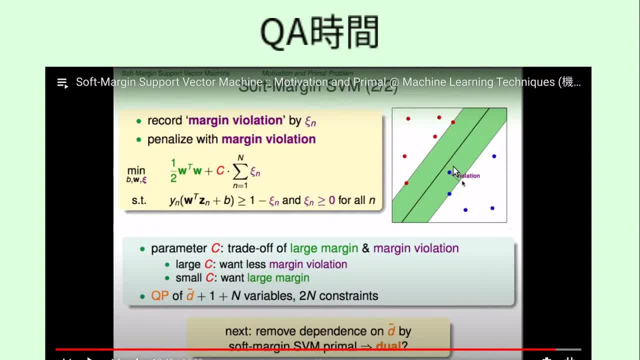 好那同學有沒有什麼問題請說。. OK, 好同學問題是說。 那我們剛才的講法 OK, 看起來好像是根據不同的 W。. 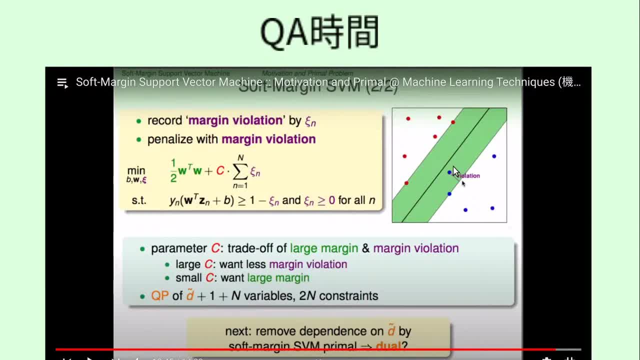 然後會有不同的這個 C。 OK, 那但是真正這件事情在 QP Solver 裡面是怎麼發生的。 大家注意到說其實 C 跟我們的 B, 跟 W 一樣。. 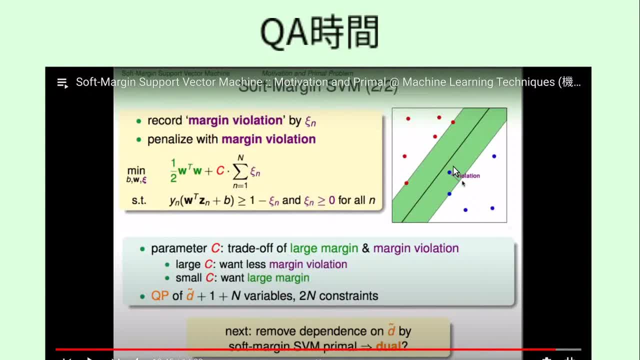 OK, 也是我們在 Optimization 的變數。. 好意思是說所以 QP Solver 做的事情是這樣。 反正不管你是 B 還是 W 還是 C。 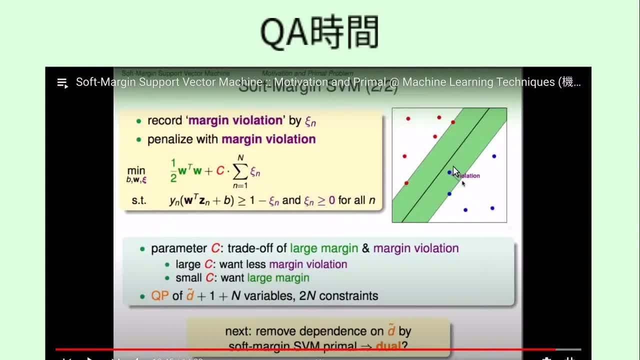 通通混在一起。 然後通通一起 Optimize。 OK, 可是那我為什麼說看起來好像這個你決定了你要的 B 跟 W。. 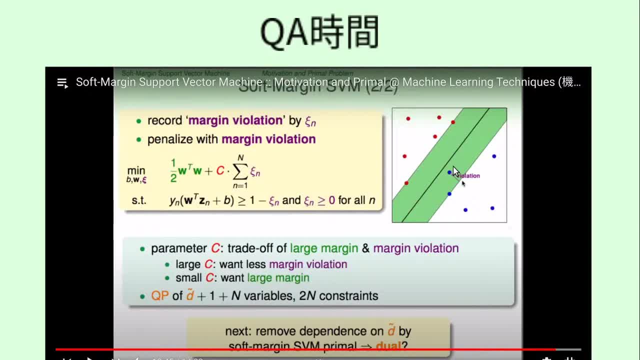 然後可是就決定了呢。 因為注意到我們在 Minimize。. OK, 所以呢例如說你今天想像說好我今天這個有個點。. 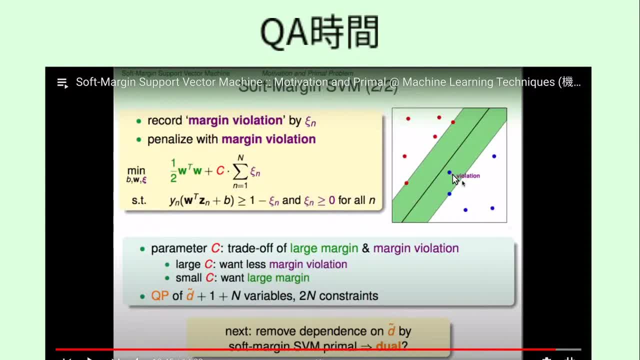 OK, 假設這個點位在這個 Y 層上分數等於 0.5 的地方好了。. OK, 那就表示我們要收它 0.5. 可能不是好例子。. 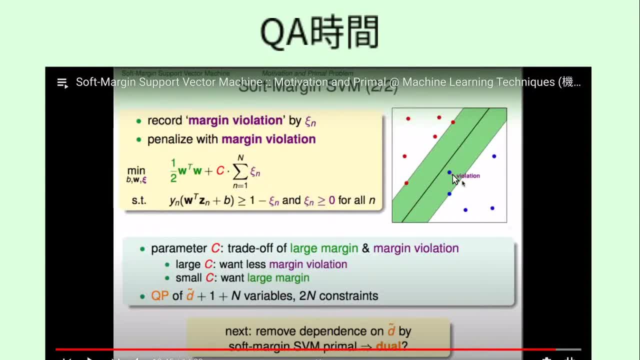 位在這個 Y 層上分數等於 0.5。. 等於 0.6 的地方好了。 OK, 意思是說我們要收它: 0.4。. 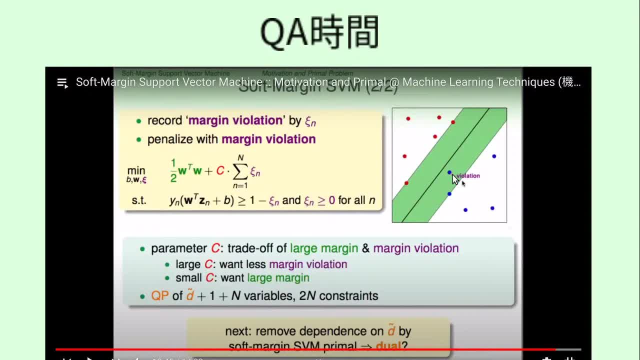 OK, 叫 Penalty。. 好那 0.4 的 Penalty 對 QP Solver 來說它是怎麼算出這件事的呢。 你可能可以想成固定 B 跟 W 的時候。. 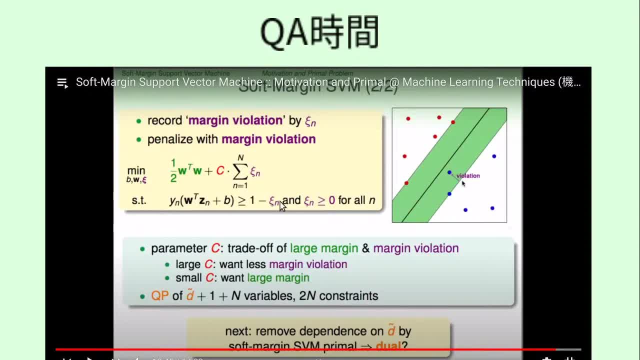 最好最好的可視。. 最好最好可視就是付出 0.4 塊。 意思是說你看這是個 Contrary 嘛。 這是個 Linear Contrary。. 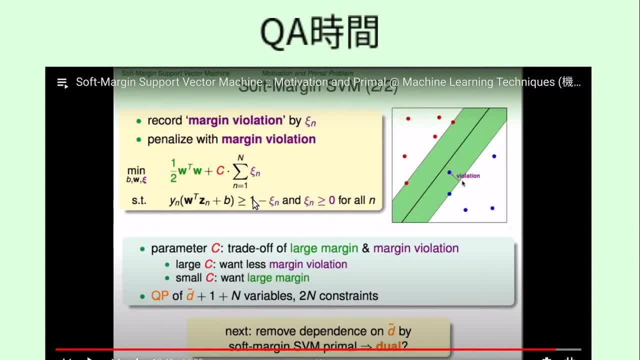 所以這個你要收它. 0.4 塊的時候。 在你的可視可以是大於等於。 你的可視可以是 0.4。. 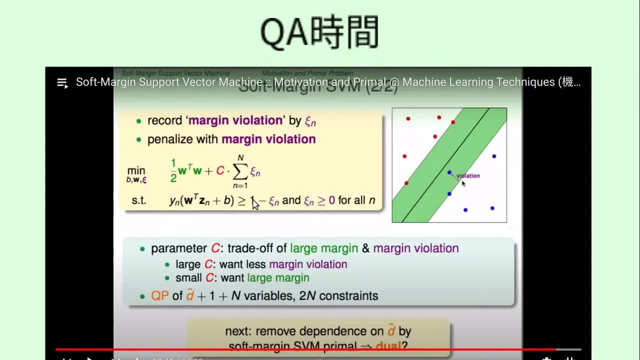 意思是說你這邊是大於等於 0.6。. 但是你也可以說大於等於 0.6。 那我大於等於 0.3, 可不可以。. 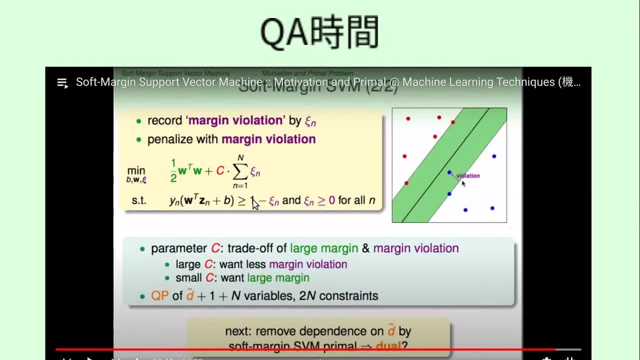 可以。 那時候你的可視就會是 0.7。. 好意思是說你這邊其實是有很多不同的可視。. 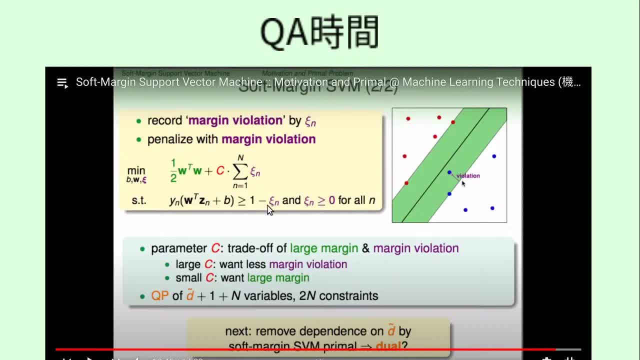 可以讓你的固定的 W 跟 B 滿足這個 Contrary。 但是你要你有很多不同可視同時都滿足, OK。. 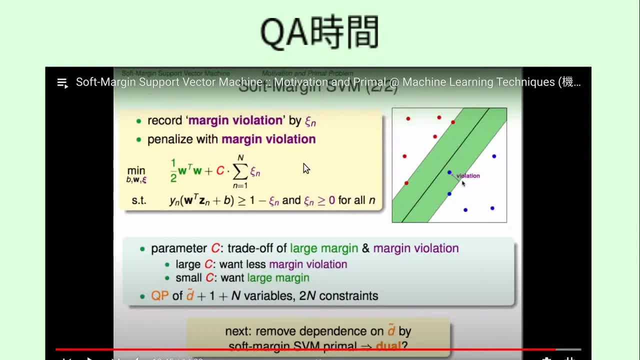 但是你最後想要是哪一個可視。 想要是讓這個 Objective Function 最小。 這個可視。 所以, OK。. 這時候你的 QPSolver 就會自動幫你說 OK。. 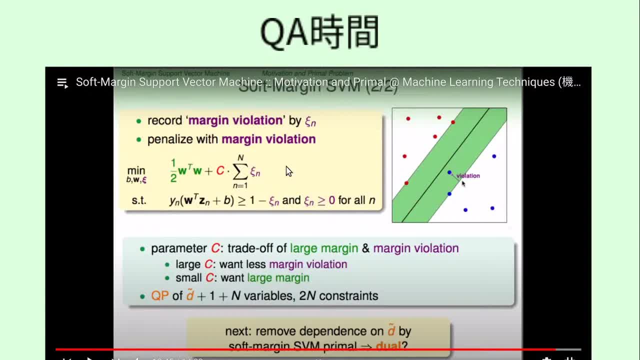 可視這個: 0.4 也行。, 0.5 也行。, 0.6 也行。, 0.7 也行。, 0.8 也行。 哪一個最小。. 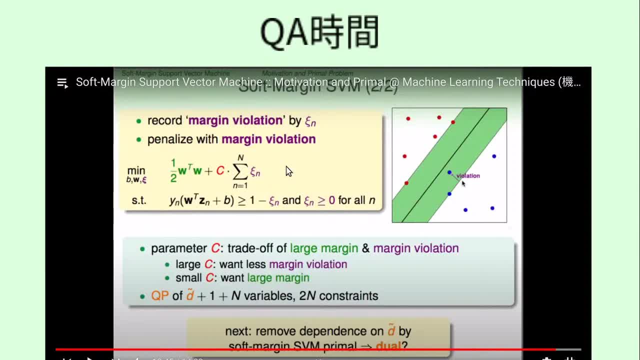 0.4 最小。 OK。 所以在它 Optimize B 跟 W 的同時。 對每一個 B 跟 W 來說它都有個最佳的可視。. 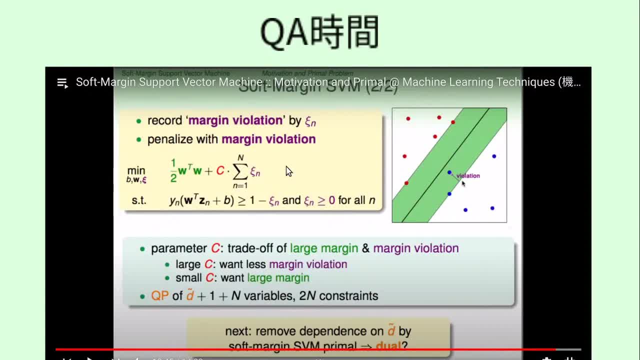 而那個最佳的可視記錄了. OK。 我們剛才講的 Violation 這件事情。 所以正確的來說這個原來我們送去 QPSolver 的時候。. 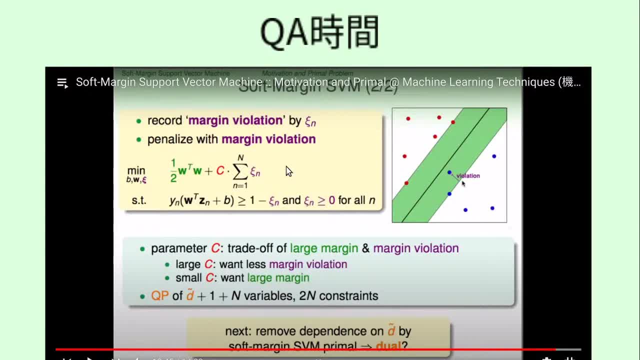 反正它們通常都是變數。 你只要把你的 47 號丟進去就好了。 OK。 但是從它的 Optimal Condition 來看的話。. 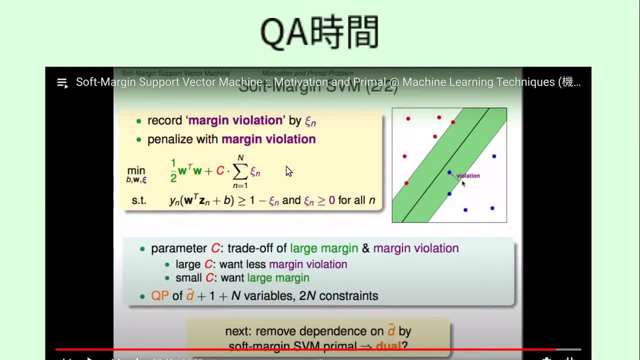 你任何一個給定的 B 跟 W。 OK。. 它都必須把可視 Optimize 到。. 記錄我們剛才講的那個 Violation。. 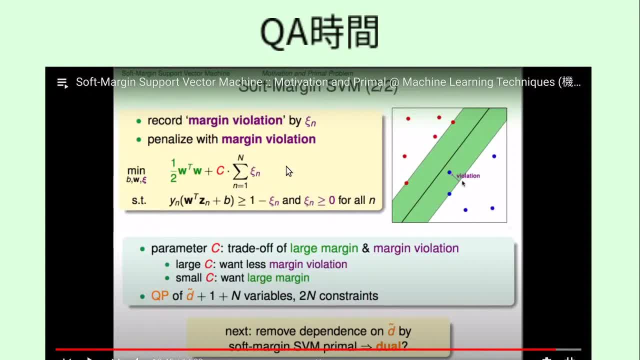 才會是對那個 B 跟 W 來說的最佳解。 OK。, 所以你最後解出來 QPSolver 的最佳解。 也會有這個性質說。. 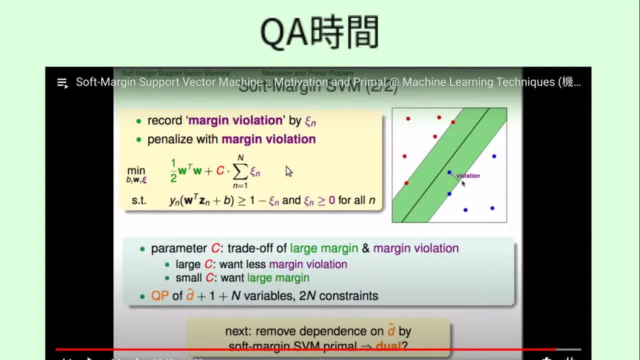 同時. OK。 它有 B 跟 W。 它也算出來了相對應的可視是多少。. 好。, 有沒有問題。 請說。. 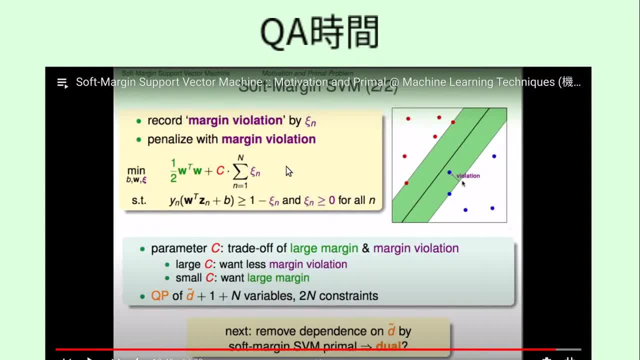 OK。. 好。 同學問題是所以我們位進去 QPSolver 的這個變數到底是什麼。? 大家記得在 Hard Margin 的時候我們就是位 B 跟 W 進去。. 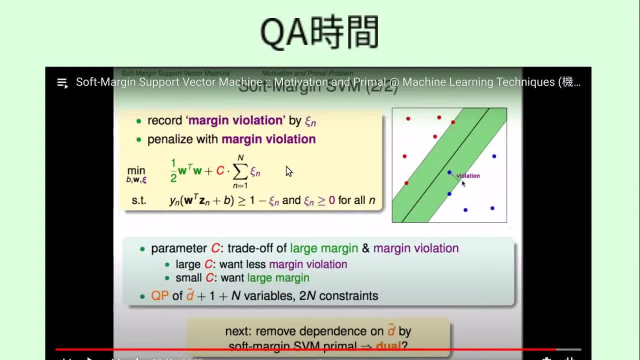 直到 Primal 的時候我們就是位 B 跟 W 進去。 現在我們就是位 B 跟 W 跟 Z 進去。 這些通通都是我們的變數。. 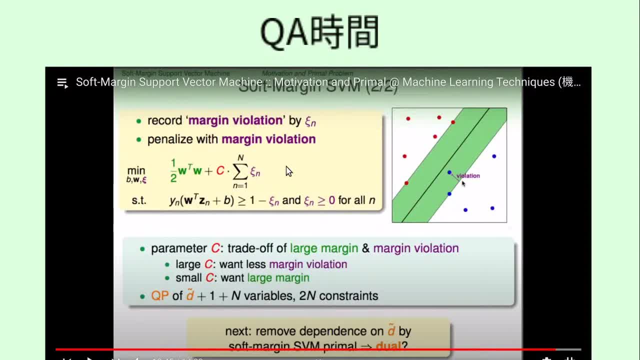 所以你如果乍看之下的話。 這是我們為什麼寫下面是 QP of D, delta 加 1。 那是 W, B 跟 W 的部分。. 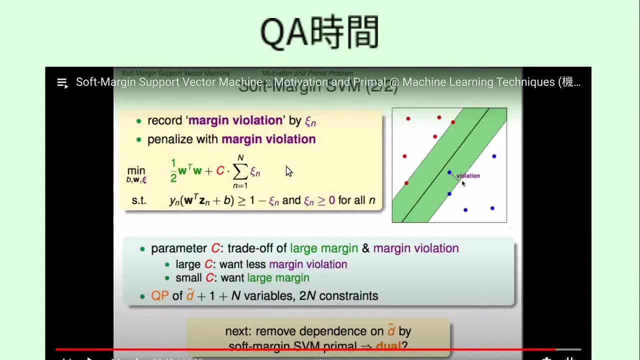 然後加上 N, 你有 N 個可視。 所以這是為什麼現在有那麼多個變數。 那可視跟 B 跟 W 的地位某種角度來說都是一樣的。. 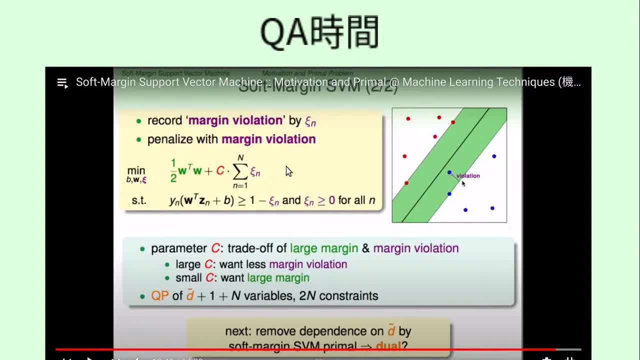 它們都是我們在這邊考慮的變數。 好。 還有問題嗎。 OK。 好。 沒有的話那我們來看看下一段的部分。. 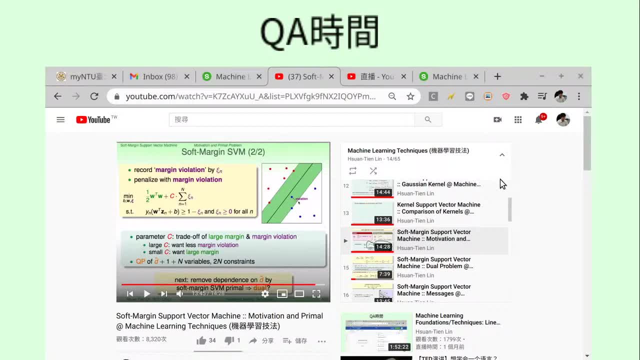 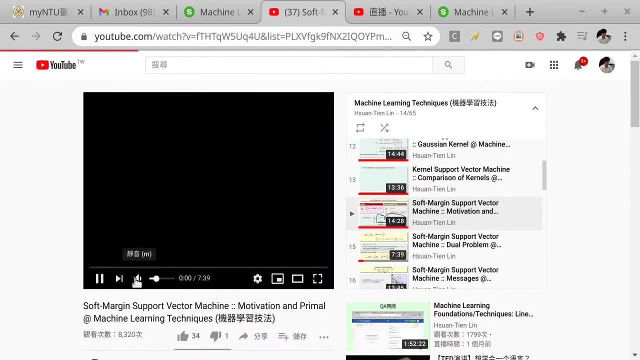 OK。 好。. 沒有的話那我們來看看下一段的部分。. OK。 好。 好。 這是我們剛才講到的這個 soft margin 的 SVM。. 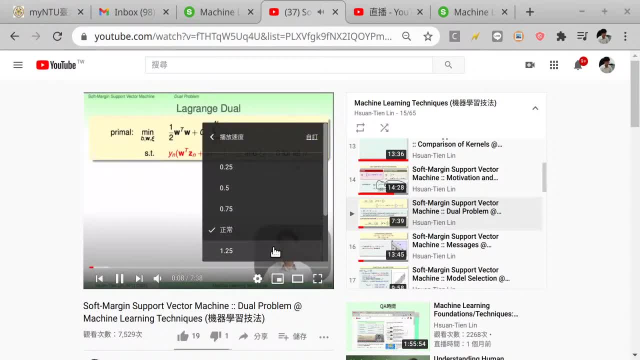 也就是今天我允許一些些對 margin 的違反。 所以我對 margin 的要求不再是 hard, 不再是那個強硬不可更改的條件。. 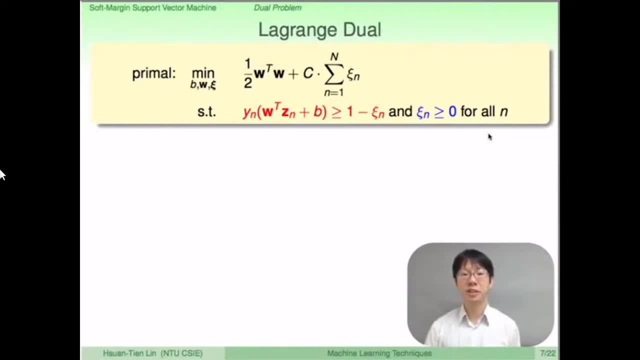 現在是 soft。 意思是說比較軟一點我允許一些違反。 接下來要做的事情就是對這個問題我們推導它的對偶問題。. 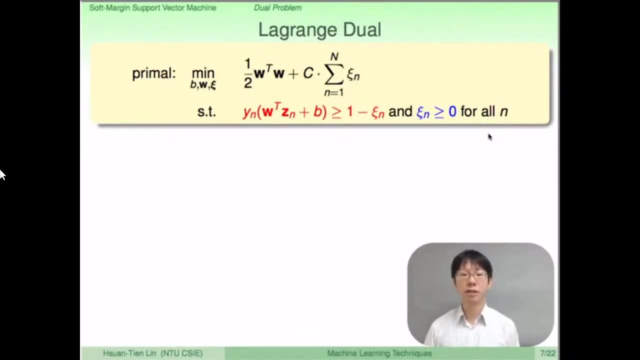 推導它的對偶問題。 就可以像我們之前的 hard margin SVM 一樣。 就可以像我們之前的 hard margin SVM 一樣。. 享用這些很輕易做 feature transform 的事情。. 享用這些很輕易做 feature transform 的事情。 享用這些很輕易做 feature transform 的事情。. 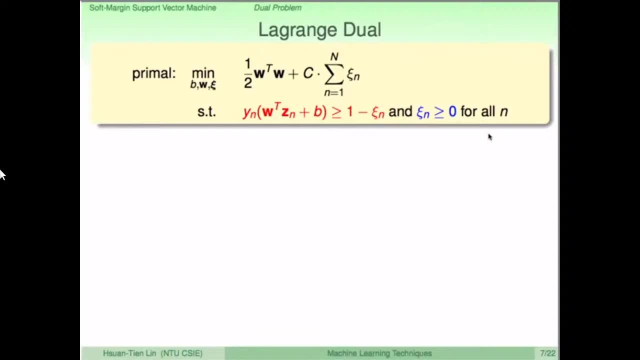 好。 所以我們要怎麼來做。. 好。 所以我們要怎麼來做。 我們就要推導所謂的 Lagrange Duo。. 我們現在已經非常熟悉了。 我們現在已經非常熟悉了。 我們原來的 primal 問題長這個樣子。. 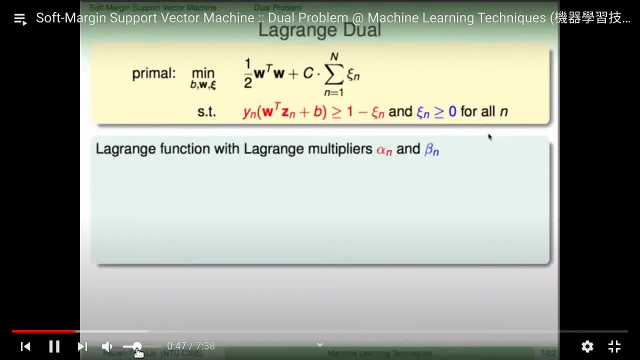 我們要怎麼推導 duo。 我們要先寫出 Lagrange Multiplied. 我們現在條件變多了。 第一組的條件我們用原來的 Lagrange Multiplied 那些 αn 來跟它對應。. 第一組的條件我們用原來的 Lagrange Multiplied 那些 αn 來跟它對應。 我們現在條件變多了。. 第一組的條件我們用原來的 Lagrange Multiplied 那些 αn 來跟它對應。. 那麼第二組條件那些可識點大於零的我們用一個 beta n 來對應它們的一 個條件。. 那麼第二組的條件那些可識點大於零的我們用一個 beta n 來對應它們的一 個條件。. 那麼第二組的條件那些可識點大於零的我們用一個 beta n 來對應它們的一 個條件。. 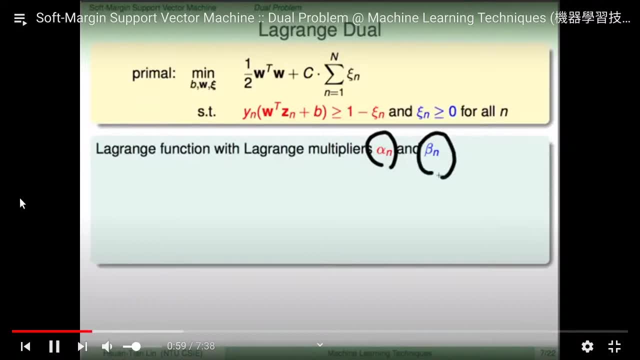 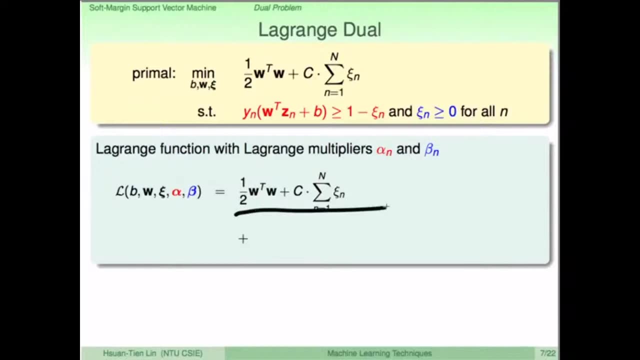 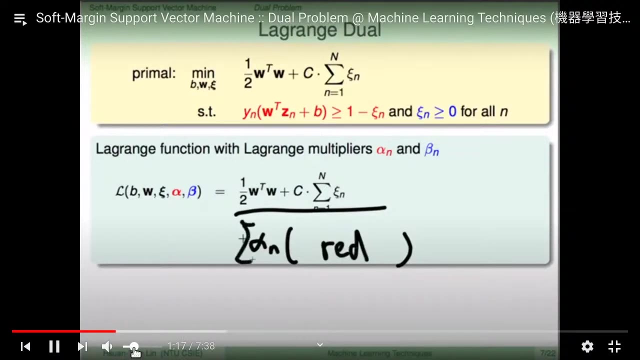 Legitimally. the next steps are: Look at our Lagrange functions. what eigene answer will look like this. The question is, if we worked this over again: 加上αn乘上红色的条件submission αn乘上红色的条件加上submission βn乘上蓝色的条件。. 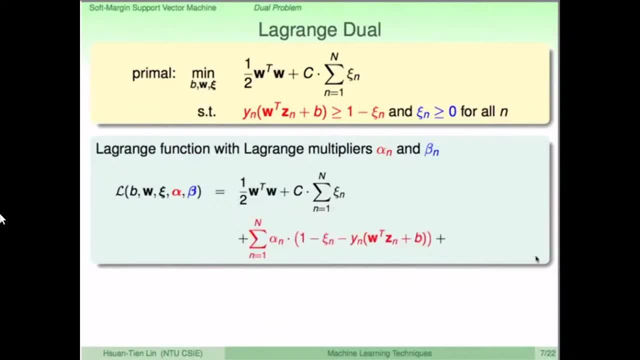 对不对跟我们之前在这个tower margin这边做的事情是一模一样的我相信大家应该还记得αn乘上红色的条件βn乘上蓝色的条件。. 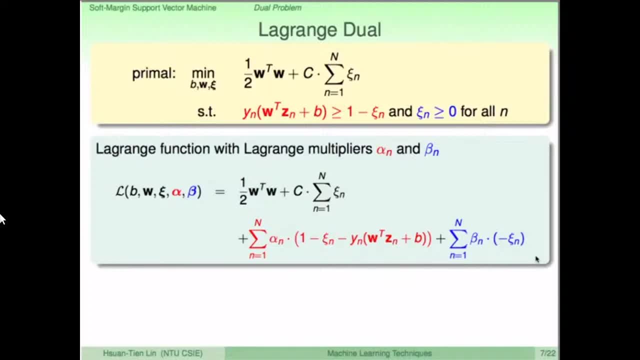 当然这边要注意一下一些符号等等等等例如说我们需要移向整个移到小于等于0的这边整个移到小于等于0的这边。. 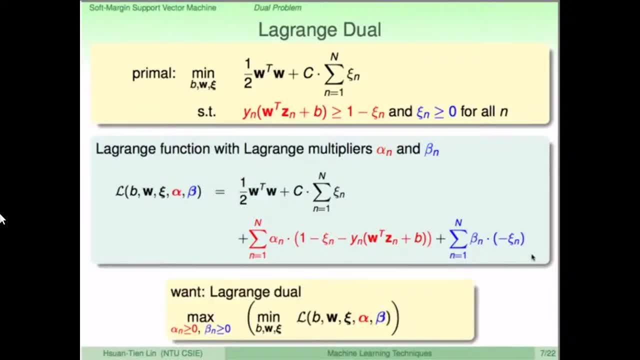 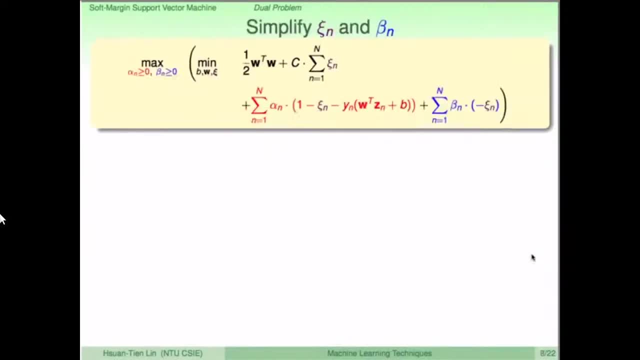 Lagrange函数写出来以后接下来要干嘛接下来我们就可以用Lagrange dual的问题把它写下来这个max mean把它写下来然后用KKT condition来简化这个问题。. 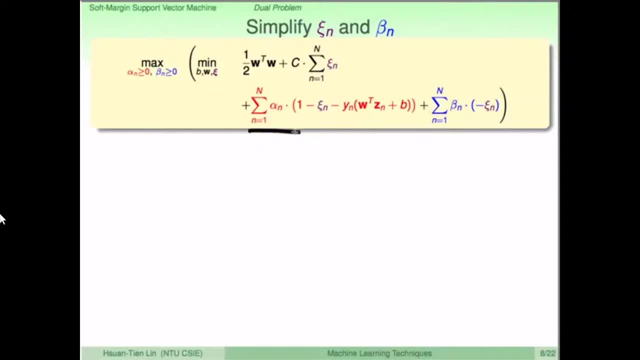 怎么做呢好这个问题写下来这个只是照抄的就是我的Lagrange function现在有红色的部分然后有蓝色的部分。. 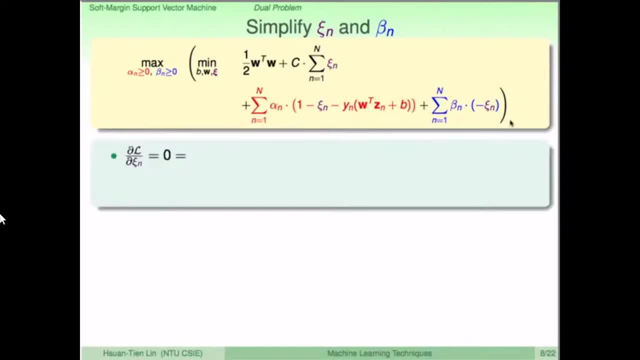 好我们先怎么做简化呢其中一个简化的方式是这样记得KKT condition吗它说我需要对primal里面原来每个变数的微分要是0,这是我在对加写的时候要满足的事情。 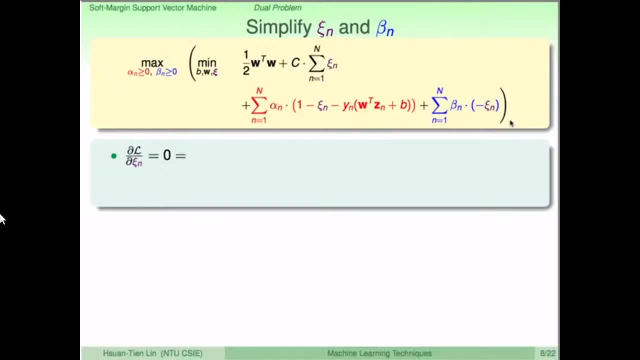 我们就先对可选函数写下来。 我们先对Cn做一做我们新的这个变数可选函数做一做看会发生什么事。. 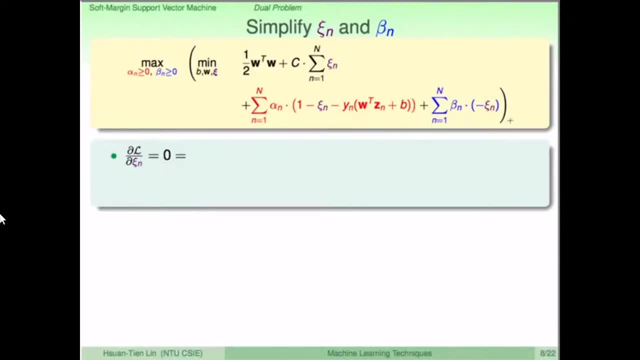 对可选函数做的时候我们来找找哪里有可选函呢. 原来的objective function里面有可选函你对它做偏微分对某一个特定的可选函做偏微分你得到C。. 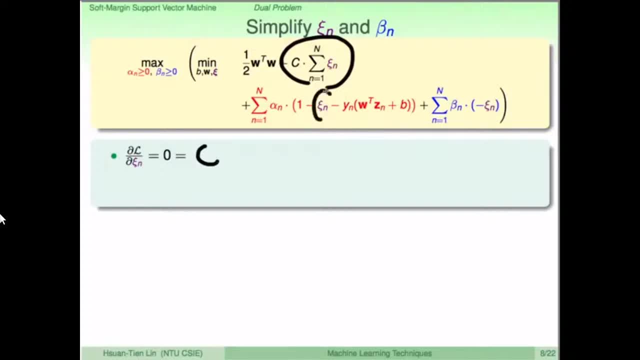 还有哪里有可选函你现在αn乘上去的这个部分有可选函所以这边有一个减掉αn。. βn呢乘上去的部分也有可选函这边有一个减掉βn。. 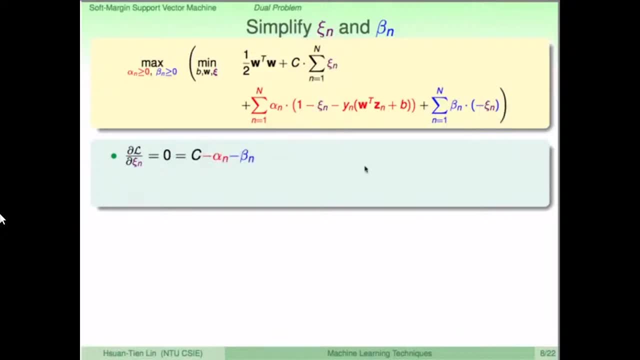 所以这个式子写下来会告诉我们什么αn跟βn加起来要刚刚好等于C。 在最佳节上αn跟βn加起来要刚刚好等于C。. 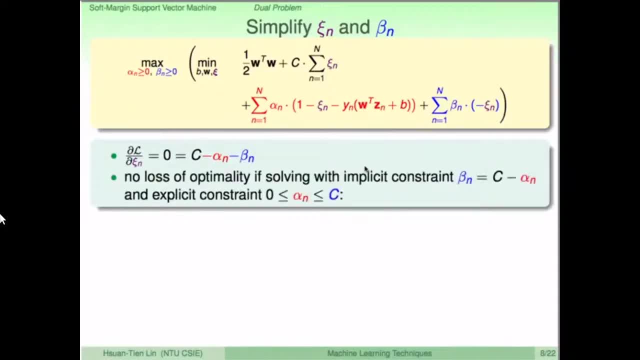 刚刚好等于C就代表我们其实可以把βn换掉。 换成什么换成C减αn。 反正在最佳节上它要满足嘛。. 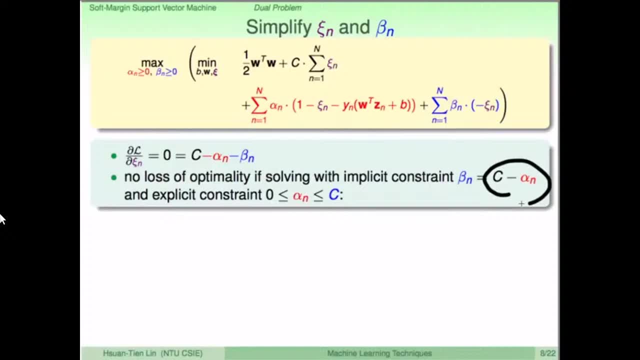 那这样的话我们就可以把βn换掉以后把它带进去。 于是我就事实就只剩下αn长得应该会跟我原来的这个hard margin的第二个问题会比较像。. 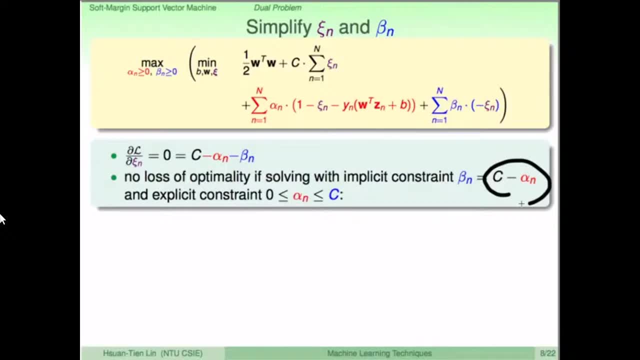 不过你说把它换掉但是我怎么确保原来αn跟βn的条件都还要满足呢? 原来的条件是什么? 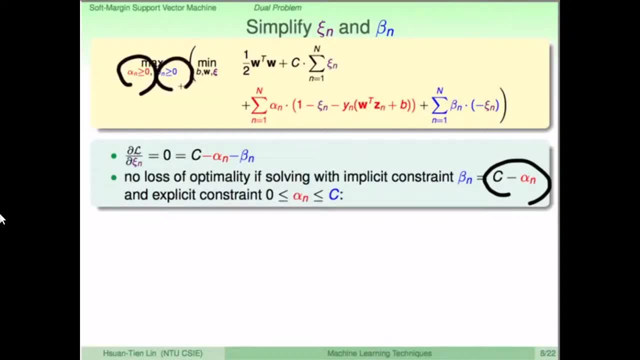 αn要大于等于0,βn也要大于等于0。. βn换掉以后是什么C减αn。 所以我今天有一个C减αn要大于等于0,. 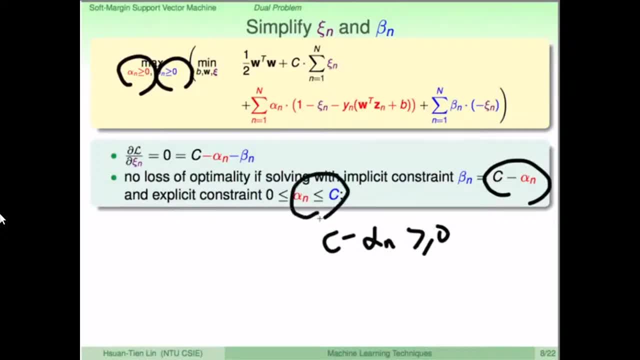 这就代表我应该要加上一个条件是αn要小于等于C。 好这样一来我就只要考虑αα要在0跟C之间β是C减α它会自然的大于等于0。 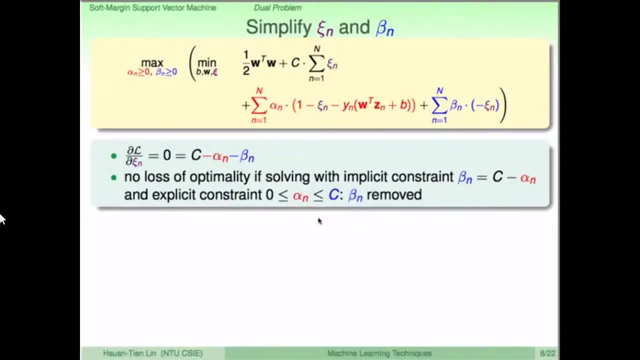 我完全不用考虑ββ就把它带进去。 带进去什么意思带进去所以这个βn会变成C减掉αn。. 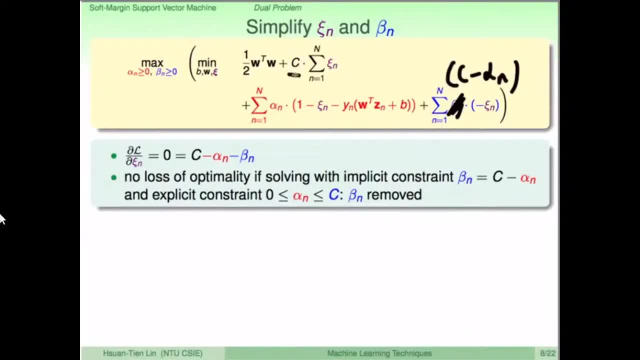 很有意思的事情是这样这边有一个C减掉αn这边有一个C减掉αn。. 两个箱减就怎么样就消掉了。. 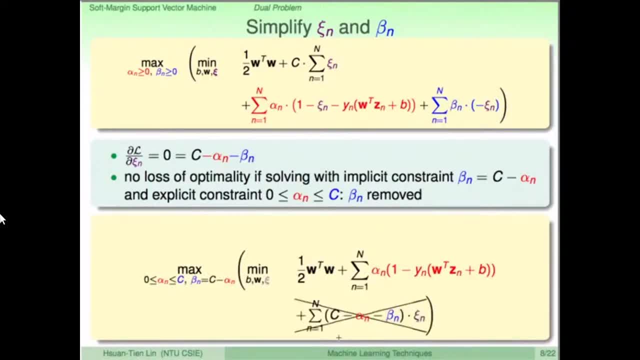 消掉什么意思消掉就是我会得到你看这边有一个C减αn减βn整个就是0。 所以这个消掉有两个意义我把βn拿掉。. 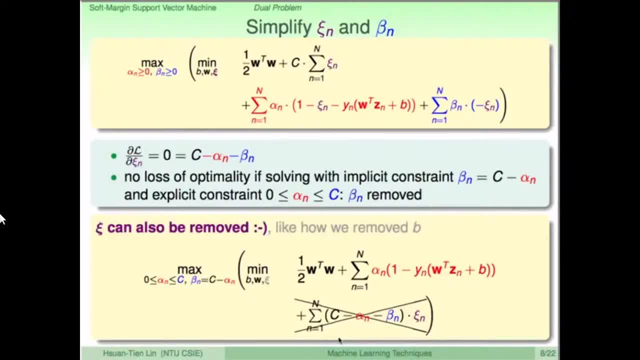 最重要的是我把可C拿掉所有的可Cn通通都拿掉了。 拿掉以后就像我们之前在哈尔玛瑞的视频里面把b拿掉的事情一样. 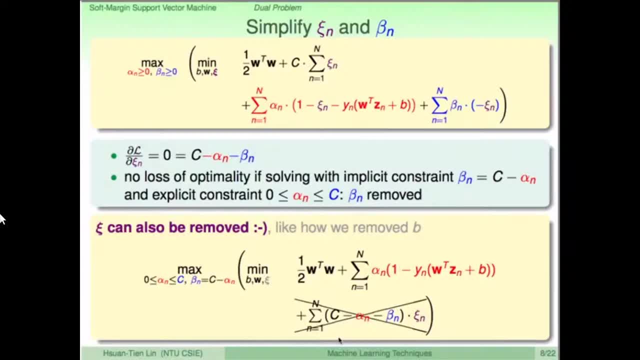 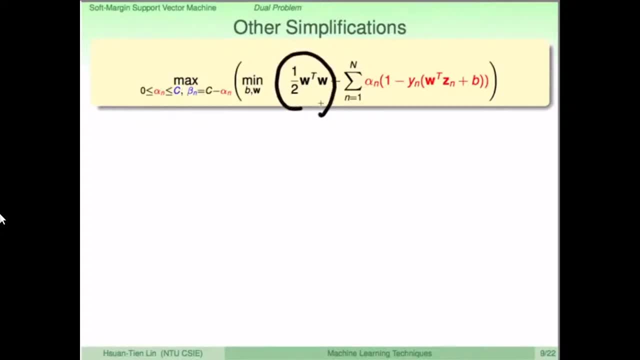 谁想不见了。 我们的式子变简单了。 变简单了变成什么样子变成这个样子。 我要minimizew的长度乘以2分之1,然后加上某一项αn然后里面是1减掉y乘上分数。 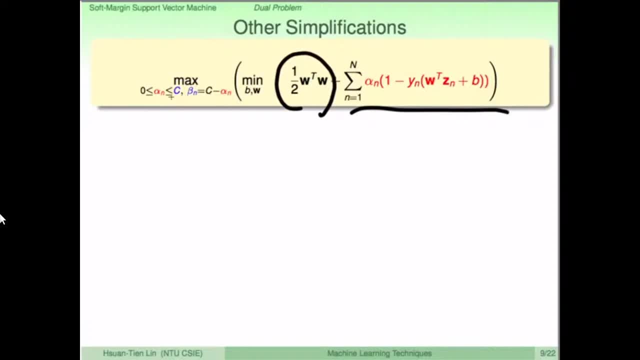 然后我的条件是什么我的条件有这个αn要在0到C之间还有一个藏起来的条件是我的βn要是C减αn。. 我们先请大家看看这个式子请问你在哪里看过它在哪里想一想。 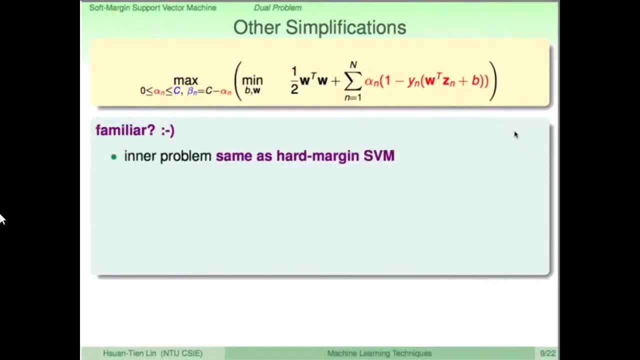 Hard margin SVN的la grunge dual。. 里面那个问题跟hard margin的dual里面的那个问题基本上是一样的。 你只有在外面多加上了一点点小小条件而已。. 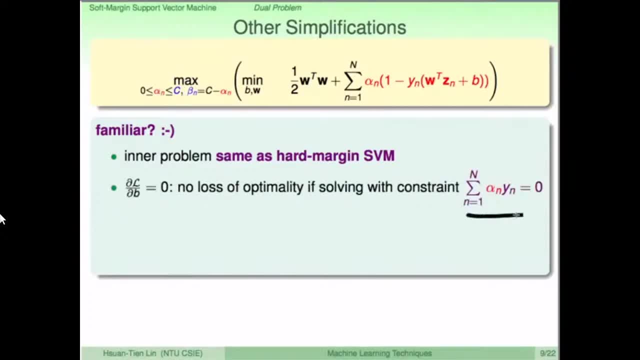 所以你可以对b为分然后就得到我们之前对b为分得到那个式子。 你可以对w为分就得到之前我们对w为分得到那个式子。. 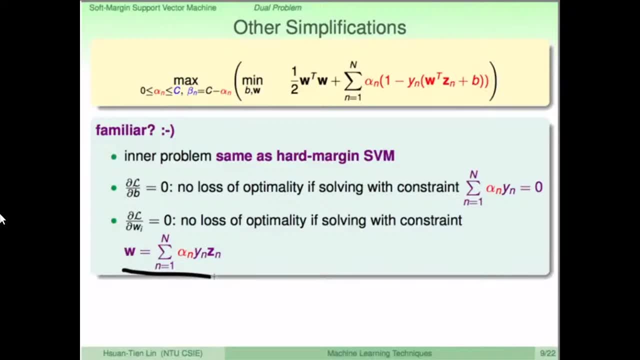 一点也不困难你在两讲之前早就已经做过。 所以怎么样如果你还不太确定的话回到我们的第二讲的课程再去稍微看一下。. 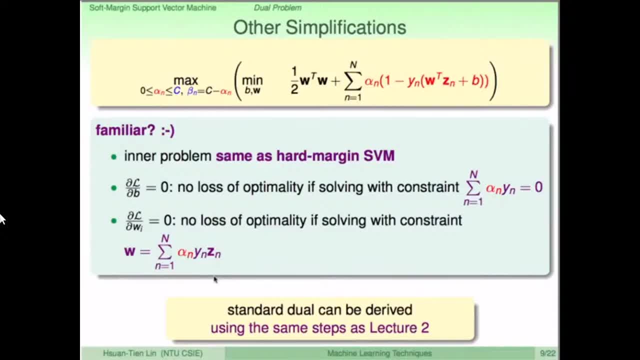 这些推导怎么样子做这些细节我们就不继续做下去。 做完以后你就会得到什么就得到一个跟原来的dual SVN几乎一模一样的问题。. 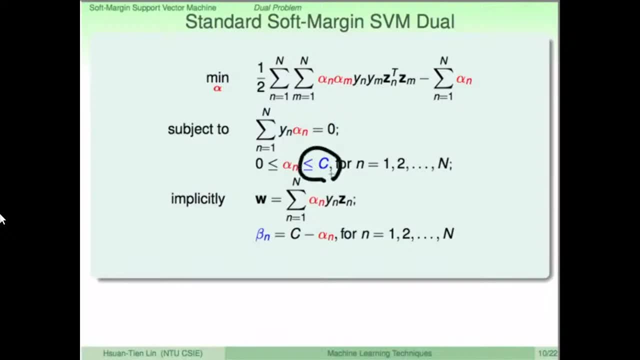 唯一的差别是什么唯一的差别是现在αn要小于等于C。 这从哪里来的从刚才我们要求我们新的la grunge multiplierβn跟αn在最佳解上要有一定的关系推导而来。 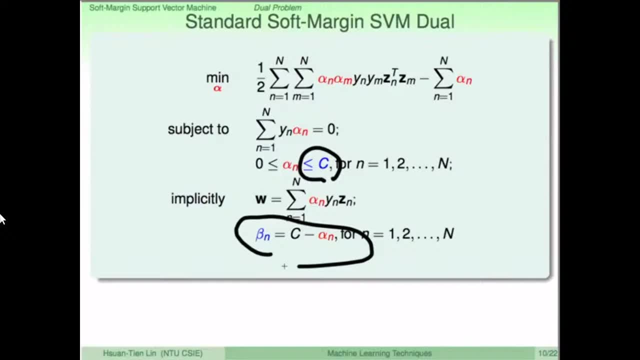 这个问题跟原来hard margin的dual问题几乎一模一样。 原来会讲hard margin你现在也会解现在只是你的α不再是毫无上限的。. 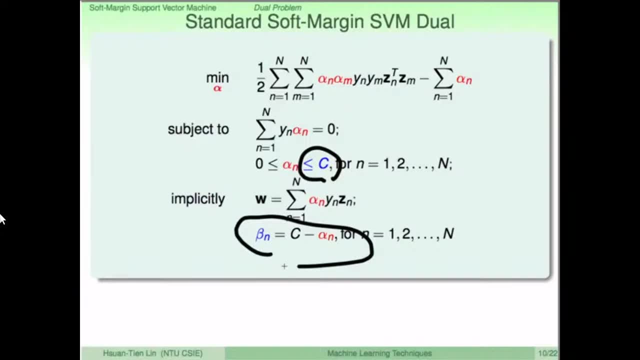 像α有一个上限上限是多少是C。 比如说你的C给1,2,6,α上限就是1,2,6。. 好所以这个上限是唯一的差别。. 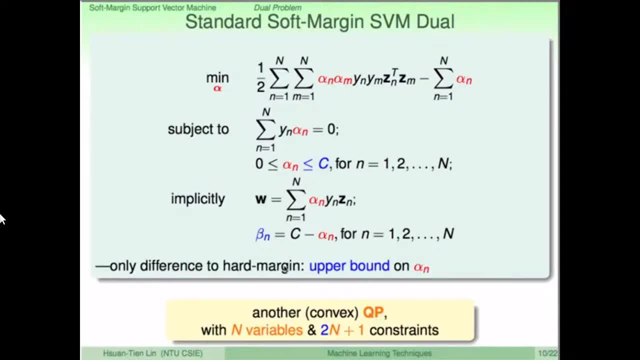 那么你现在这个问题有多少个变数n个变数。α跟以前一样。 有多少个条件你跟我看有效的条件跟α有关的条件的话基本上就是一个这是线性的条件。. 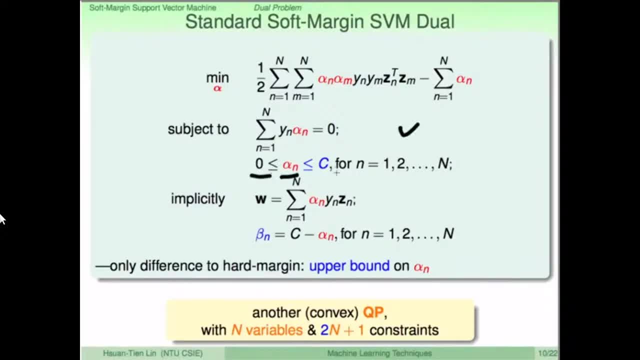 然后你的α每个α有两个条件它有一个下限是0,还有一个上限是C。 所以你可以说它是2n加1那么多个条件。. 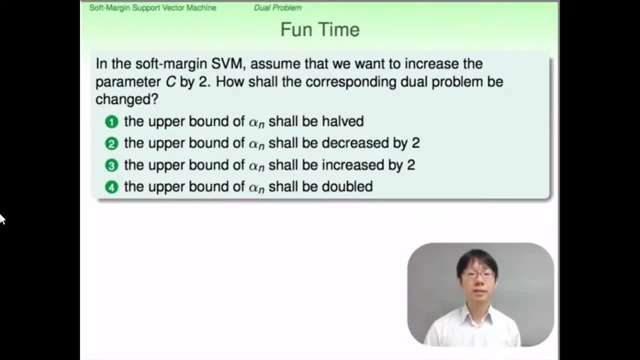 好讲到这边就给大家想一想如果今天是soft margin。 我把我的C变成原来的C加上2的话到底对α的限制会有什么样的改变? 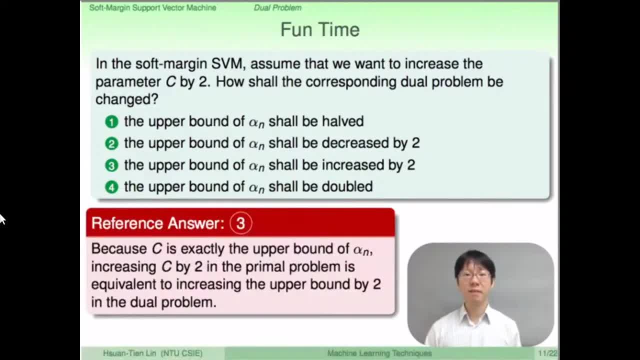 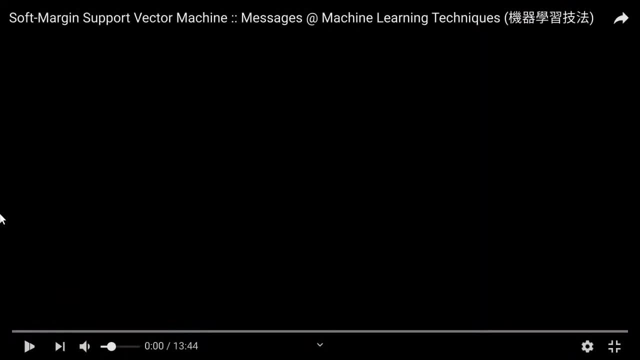 大家看一看之后我相信大家会选到正确答案是3,这个限制也会加上2。. 比如说你原来C是10,现在变成12,那么这个α上限也会从10变成12。 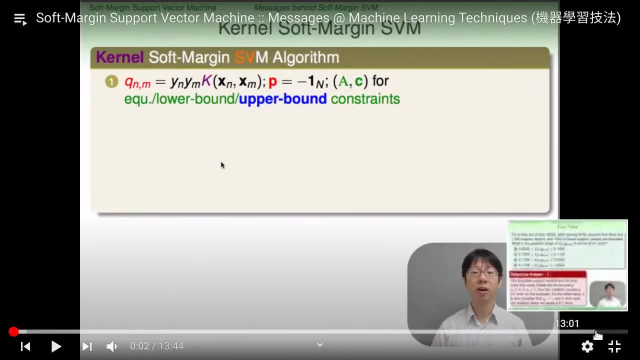 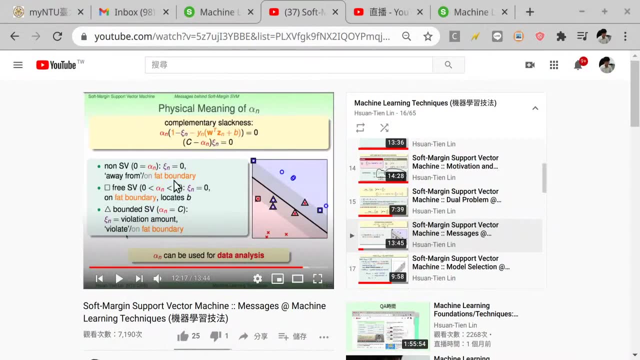 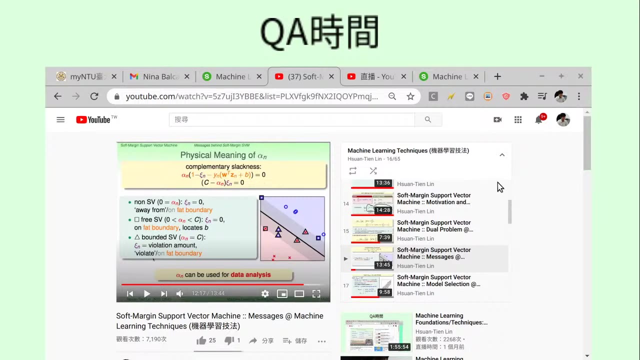 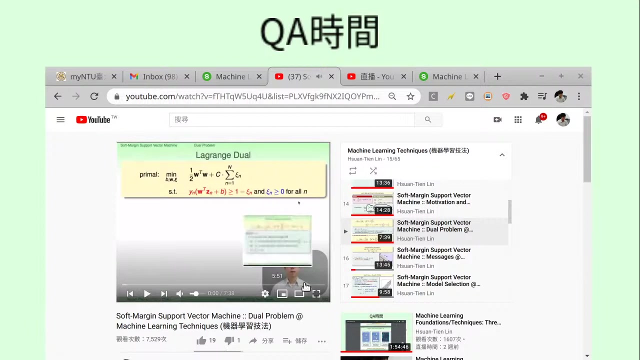 好推导完队友问题以后。. 好抱歉刚才跟主教discuss说我们万恶的作业2什么时候要公布。. 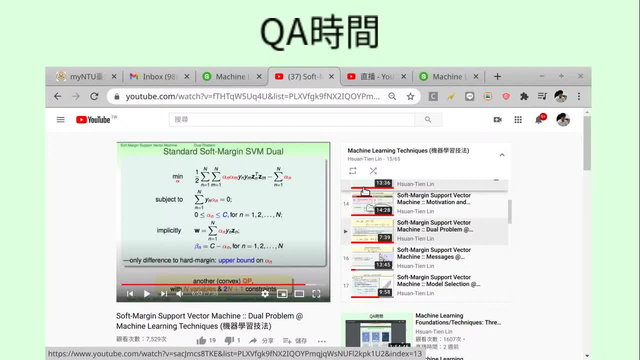 所以这个 有一些没注意到我们课程的进行。 好那所以我们很快的就把队友问题导完了。 OK实际上我们能够这么快的把队友问题导完是因为它长得跟我们原来就会的东西实在是太像了。. 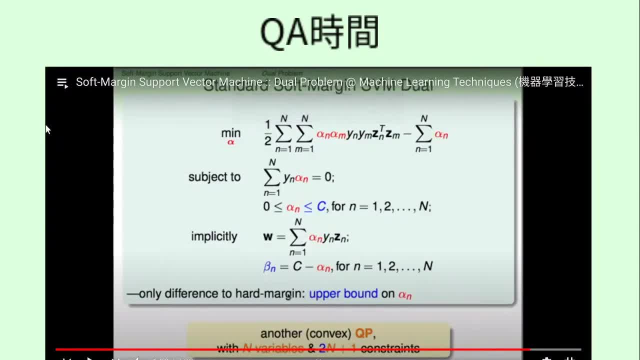 OK所以我们其实是偷师部的跳过了几件事情。 那这也, 其实这也是这个课我们进行的节奏也许跟你若去看其他一些FDM的课比较不完全一样的地方。. 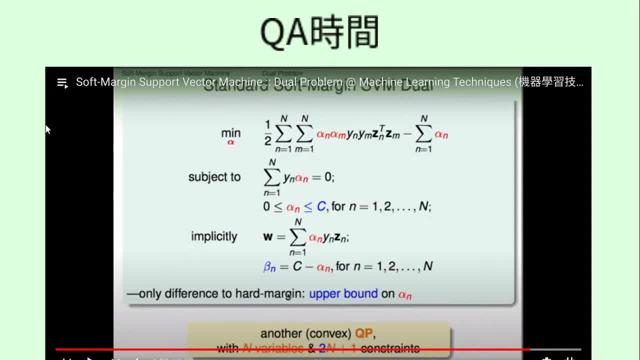 OK就是, 我们其实前面有点硬。. OK就是我们在做deal等等那些。 但是我们刻意的在那时候只做hard margin的SBM而不是做soft margin的。. 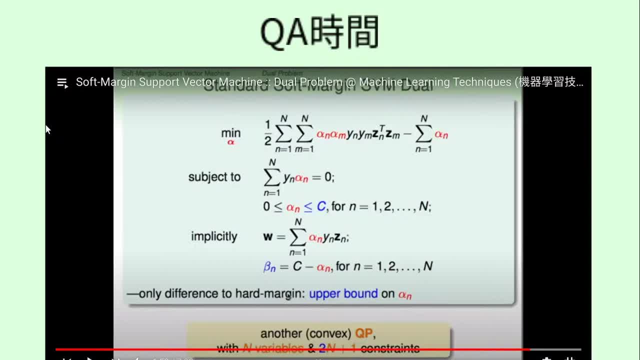 是因为如果我们那时候就要做soft margin你就有三组变数在那边然后会弄得昏头钻香。 所以不如我们那时候做hard margin的好好讲一讲然后把两组变数结束掉。 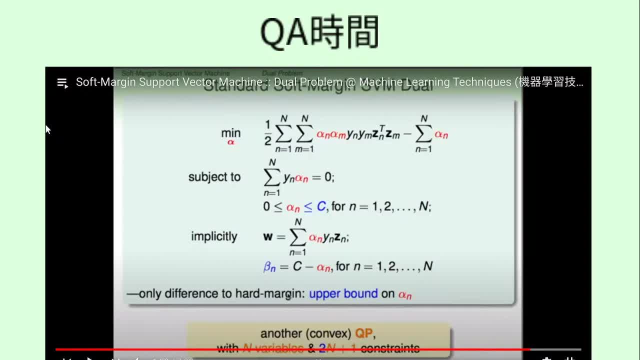 那现在soft margin的时候你其实几乎只多了一组变数而这个一组变数一样用最佳化的条件。 你很快就可以把它取代掉。. 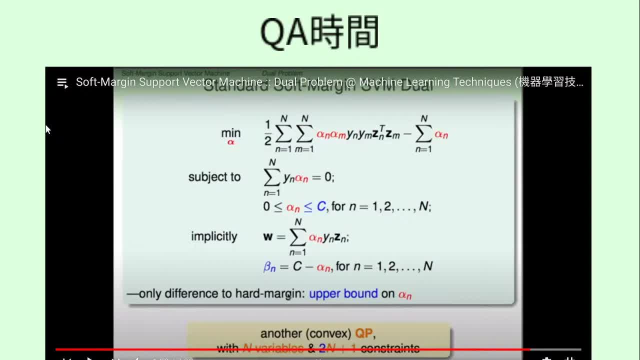 而取代掉以后就发现说长相上来说它跟原来的hard margin的deal问题其实是一模一样。 唯一的差别只有α加上了一个上限。. 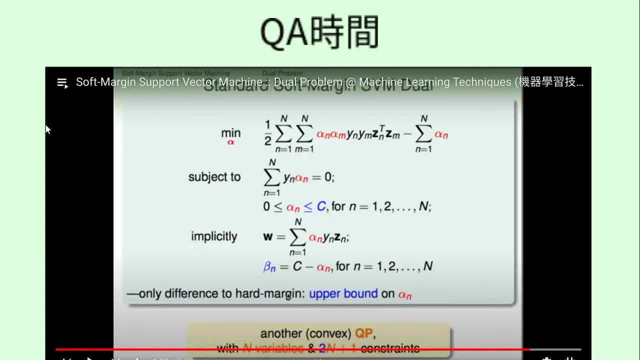 如果你记得的话hard margin原来我们是α大于等于0。 那现在我们有一个α小于等于c。 那c就是我们刚才的那个tradeoff对不对? 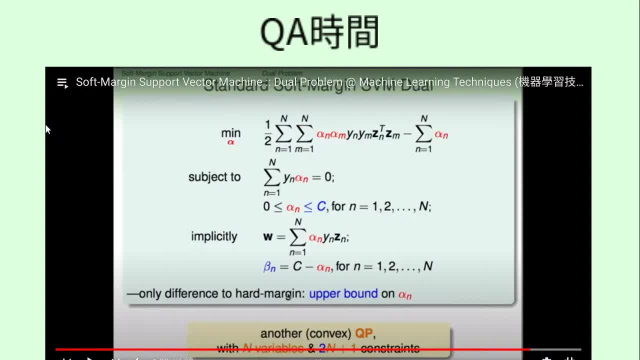 就是我们多在乎想要惩罚我们的margin。 至少想象上我们就没有证明。 但是想象上你把那个tradeoff就是我们多在乎想要惩罚我们的margin。. 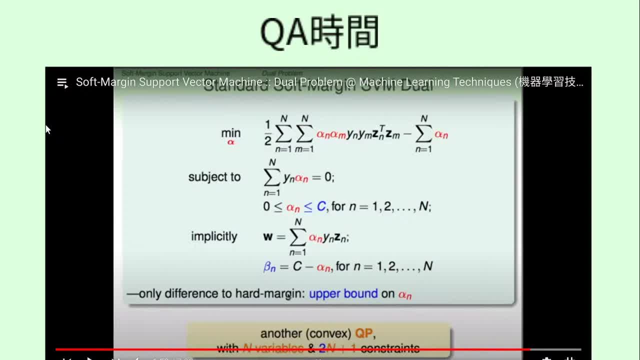 至少想象上我们就没有证明。. 如果你今天的问题是linearly separable你把c推到很大很大很大的时候代表。 你非常强烈的认为不要有任何的violation。. 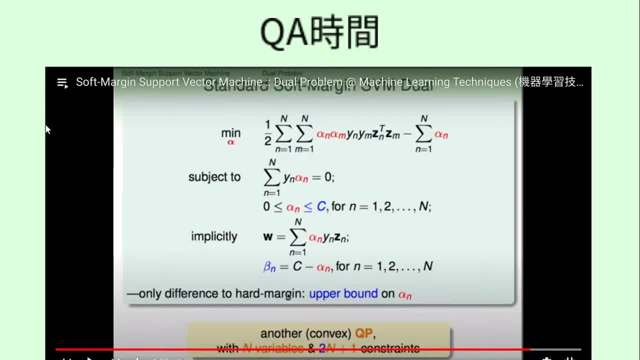 那这个时候你把c推到很大你就会像什么? 就会像hard margin SVN。. hard margin SVN你也可以想成就是那个c很大或者无限大的那个粒子。. 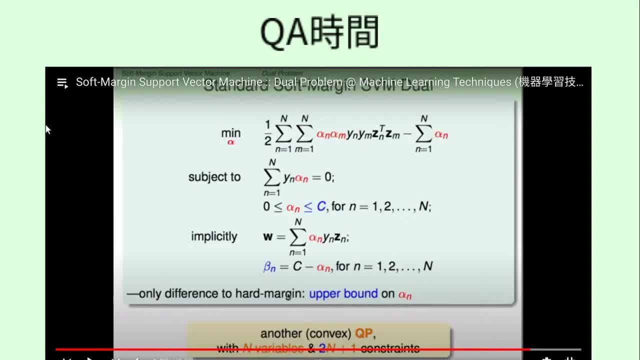 因为你的α就没有上限这件事情。 所以从这些事实之间的关联性大家可以想象说其实soft margin SVN。 也可以看成是hard margin SVN的一个更这个一般的版本。. 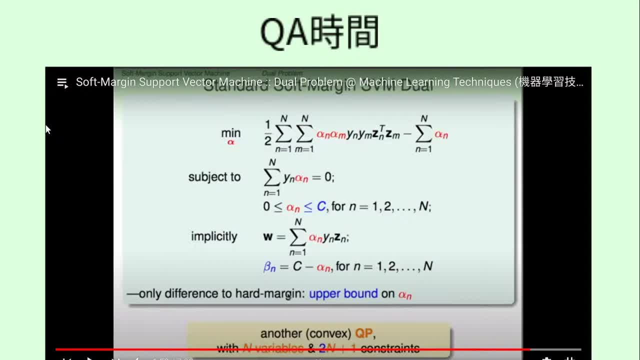 你现在有一个多一个参数然后这个参数可以来控制你的α要多大。 可以来控制你的这个margin violation的tradeoff是什么。 那透过调整这个参数等于是你可以更细致的控制SVN这样的机制。. 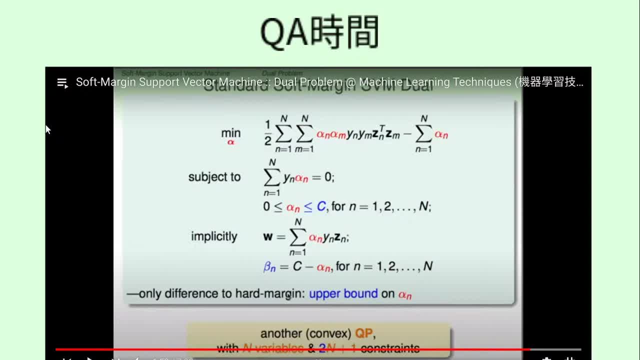 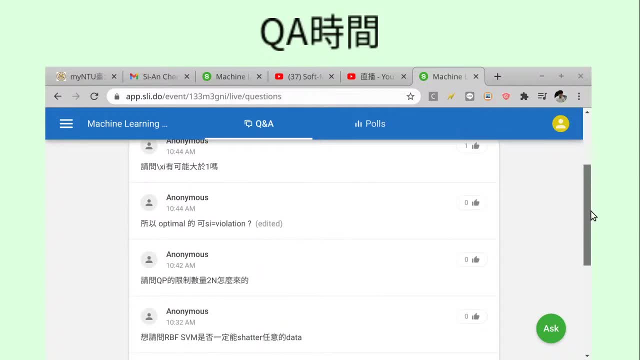 好同学有没有什么问题的. 没有OK我们来看一下线上的同学有没有什么问题。 OK好这边有个问题是可C有可能大于1吗? 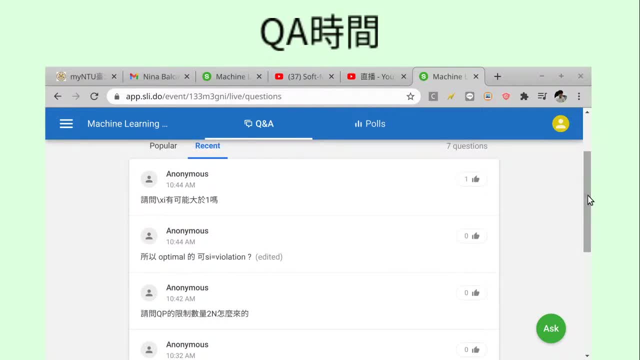 OK有可能。. 实际上我们等一下可能会有一些这个图片可能大家就会看到。. 意思是说可C其实有几种可能性。 一种就是0,0就是它在正确的那一边正确的地方。. 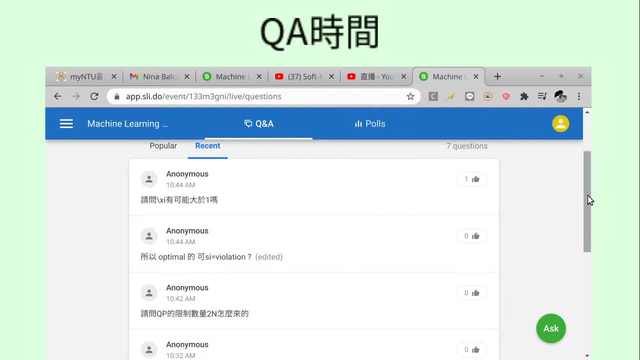 一种就是小小的尾板小小的尾板意思是说OK它可能是个比较小的值。. 如果比较小的值它可能是个比较小的值。. 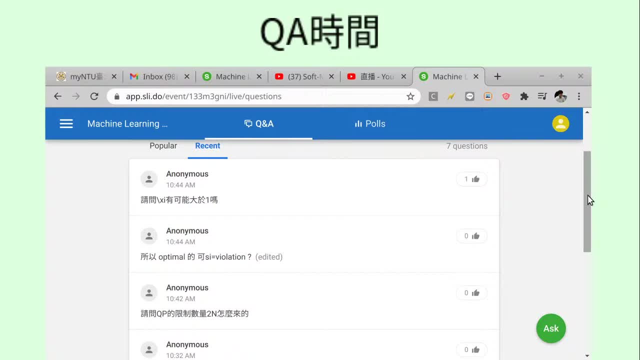 如果可C的值在0到1之间的话其实它都没有真正的跨过那个胖胖边界的中线的地方。 但是可C有可能会大于1,大于1就代表它跨过去甚至可C有可能大于2。 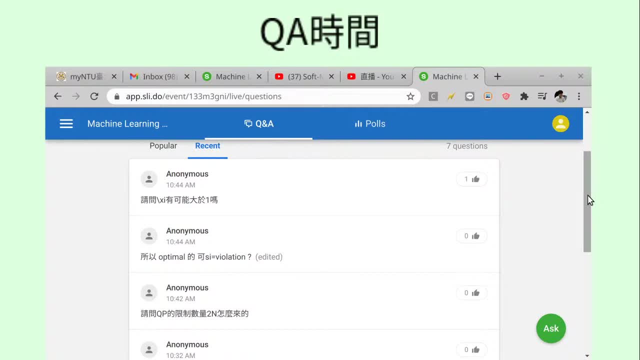 OK意思是说它还跨过胖胖边界的更大的那一边。 OK所以可C会是什么不太一定。. OK因为这个就要看你的最佳化的routine到底最后解出些什么东西。. 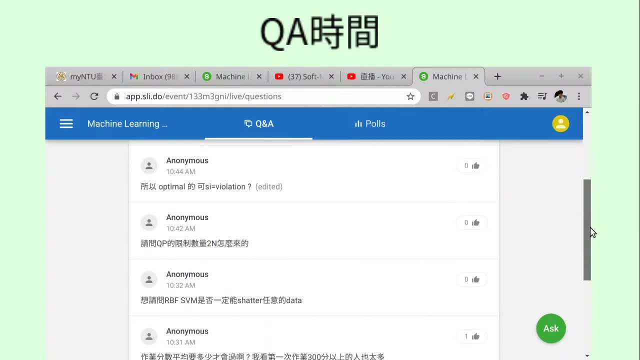 好。 那对所以我们刚才解释过optimal的可C等于violation。 那QP的限制数量2n是怎么来的我们在primal的QP里面的那个2n是什么? 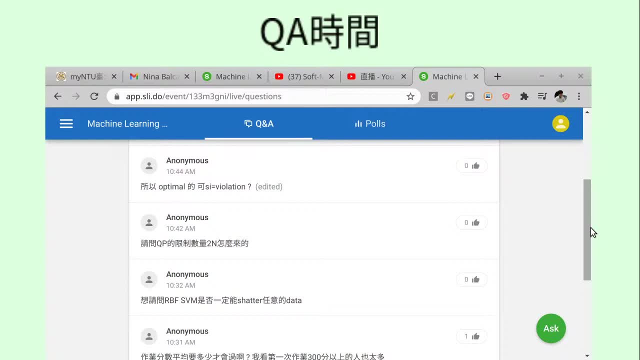 我们原来有n条我们原来的那个w乘上就是x加上bOK就是分数然后乘上y要大于1。 那我们现在有大于1减可CnOK所以这是这边有n条。 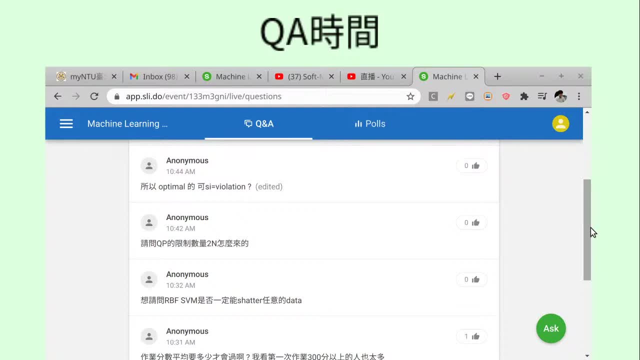 但是还有另外n条是什么我们要record的时有大于等于0的可C所以我们有个限制可C要大于等于0。. OK可是小于0,OK意思是说这些乖乖排然后离margin很远的OK那我们帮他拍拍手说你很好但是我们也没有要因为这个OK在objective function里面在奖励他。 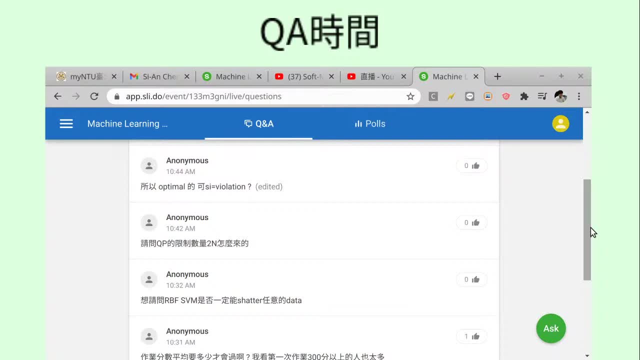 OK所以我们其实有两条变数对于每一个点有两条变数第一条变数说我的y乘上分数然后要尽量大于1,如果没有的话我记录下那个可C第二条说只有可C大于等于0的我就要记录下来。 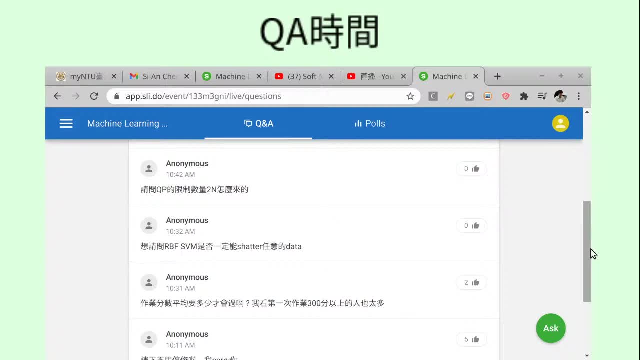 OK, OK想请问RBFSSVN是否一定能shatter任意的data不要破格嘛这是作业室的题目。. OK好然后嗯那我可不可以讲啊好可以啦OK那那那那就可以嘛。 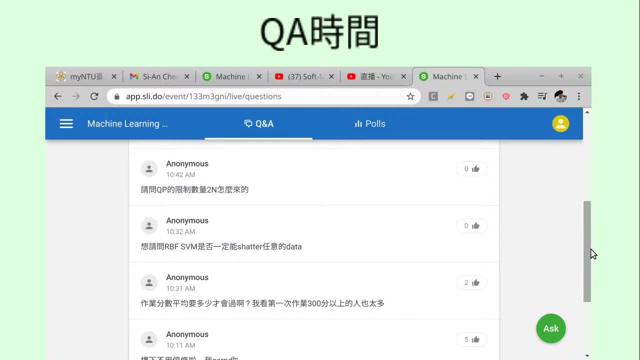 好这边有一点点的tricky的地方OK不过可以证明OKGaussian的SVN你的确是可以shatter任意资料如果你的这个资料长得都不一样的话。. 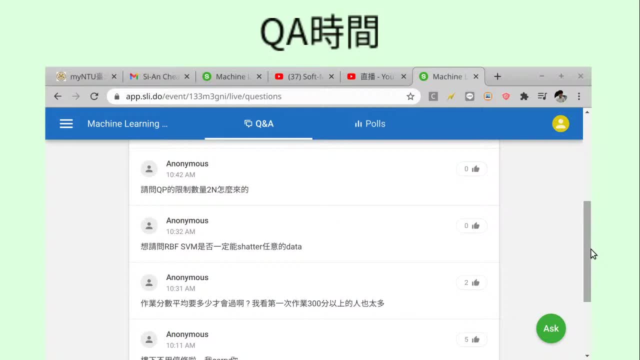 OK, 意思是说你如果点叠在一起你要它shatter是没有办法的对不对那叫强人所难。 OK但是如果这个这个呃点没有叠在一起的话那么Gaussian的SVN呃有有几个部分有有几种证明OK一种是你的gamma够大的时候一种是你的Gaussian够尖的时候你一定可以做到这件事情。 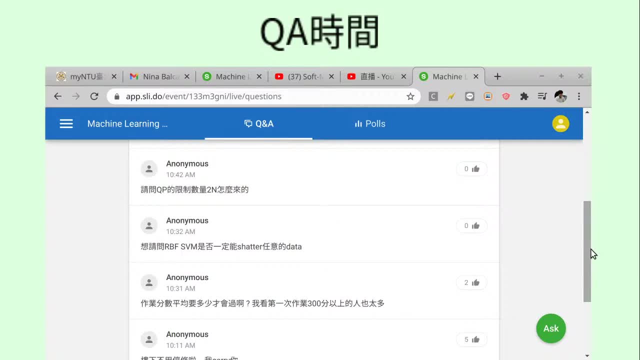 那呃这个各复杂的证明呢会说不管你的Gaussian尖还是不尖只要你那些点都长得这个不一样然后你就可以这个做到shatter这样子。. 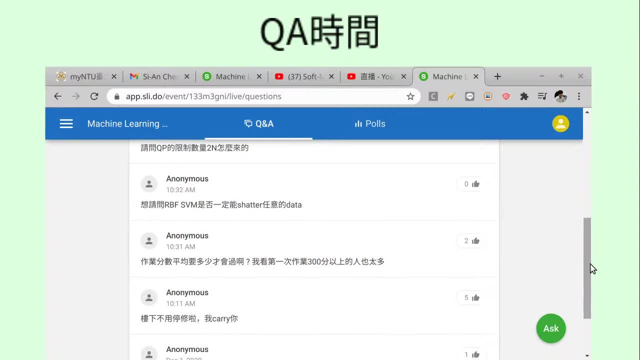 嗯好讲完这个之后我们要用力的想想作业室要怎么出比较好OK才能够呃帮助大家更熟悉这件事情。. 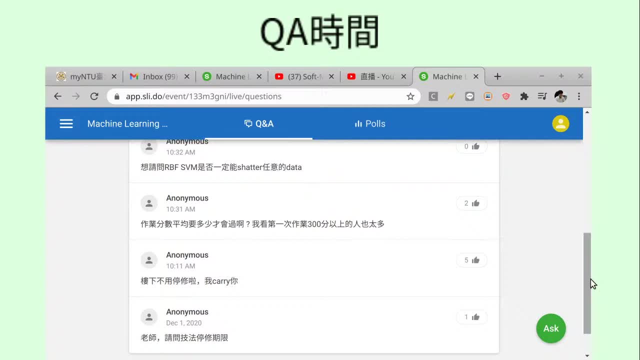 作业平均要多少才会过第一次作业300分以上的人也太多嗯对我也不知道呃这个这个这个我也不知道意思是说你要你知道这种东西是learning如果如果在以前啦以前我们这个这个以前做教批改作业的方式以前的班级的大小的话我搞不好还可以给你演示一下。. 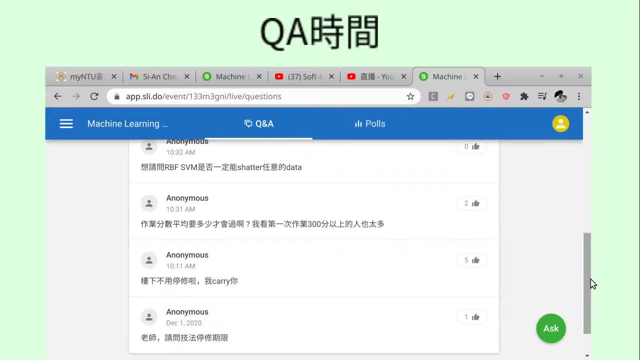 因为至少我这个教了很多年然后有一些data我可以从里面认出一个hypothesis然后跟你到跟你说OK那会过不会过是怎么样。. 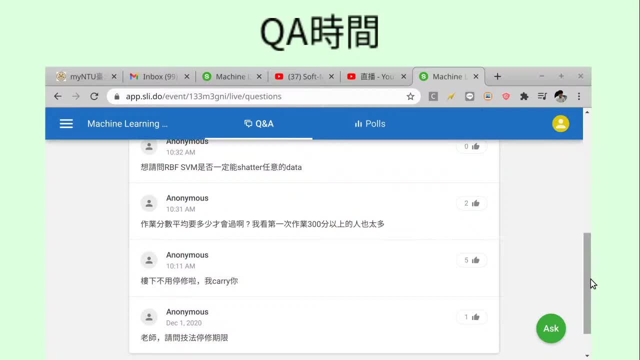 但是今年就是一个很特殊的状况因为我们今年的评分方式跟往年都不一样OK所以即使我脑袋里有data有往年data我能不能用这个data来告诉你一个好的hypothesis。. 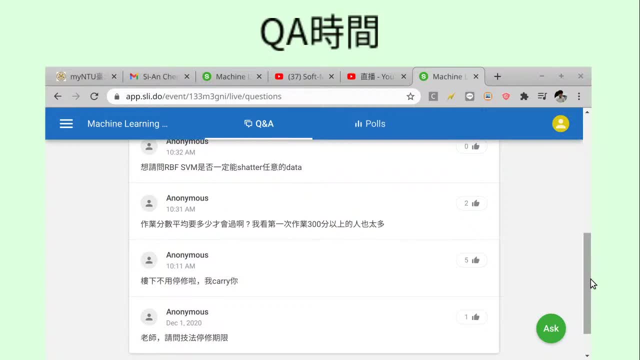 我不知道OK这个machine learning foundation是告诉大家说你training跟testing差太多的时候就可能有很麻烦的事情。 所以 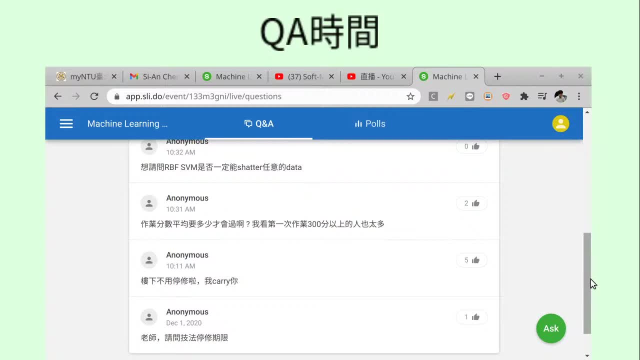 我不知道但是根据我刚刚跟助教讨论我们应该只几天作业二应该就有机会公布那到时候会比较明朗一点。. 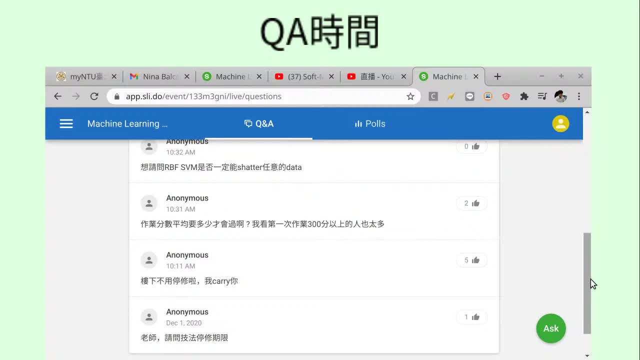 有些基石的同学跟大家讲一下就是我们的评分方式OK在基石这边的话会是我们最好的作业会乘上150%OK最差的作业会乘上50%OK然后那加上另外两次作业然后再去做平均这样子OK所以意思是说: 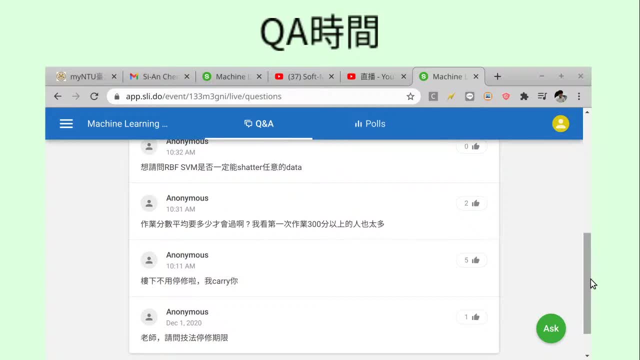 有可能OK你的成绩还会比你所想象的一般的平均再高一些些OK所以说我们会favor你最好的那个作业这样子。. 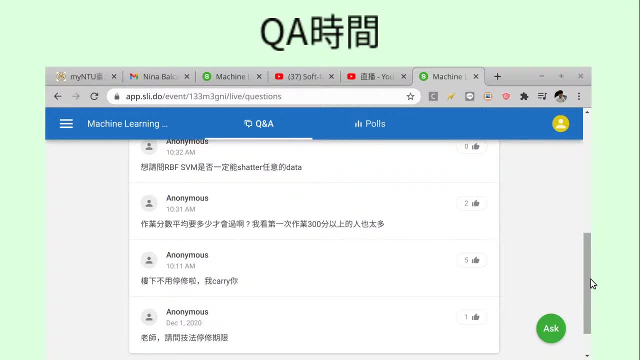 那这大概是我们课之前基石大概进行方式这样。 那基法我们只有两次作业OK所以150跟50好像没有什么太大的意义那但是我们还会有那个final project部分。. 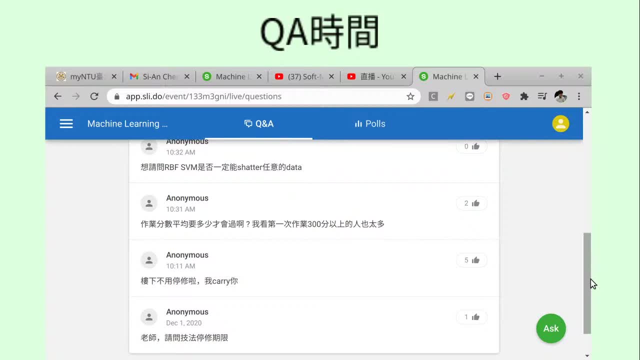 来各位我今天上课除了说忘记讲final project的话我们已经公布了题目我们已经公布了资料OK那我们建议大家尽早看一看因为这跟作业不一样这不是你最后两天再写就可以写出来的OK那里面这个资料的细节我们还是欢迎大家在forum上面这个讨论。. 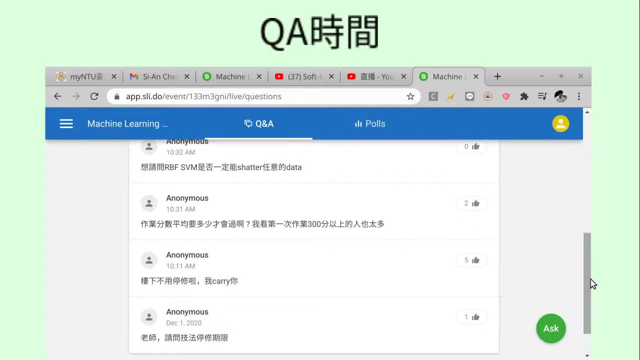 那你如果还没有那个组你的队伍的你可以在我们的discussion forum上组队伍然后赶快报名因为助教差不多我应该会要求助教下礼拜开始。. 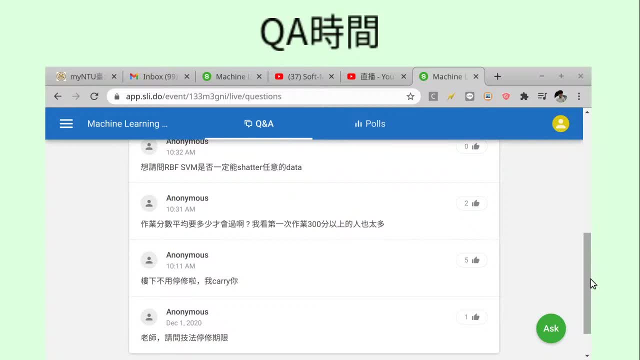 我们就要把那个competition网站建立起来然后让大家在上面做submission这样子OK所以这是project部分。. 然后同学问到停修的期限我不知道我儿子认识的时候我不知道因为基石的时候我们有特别去问是因为它是特别的课程期程设计。 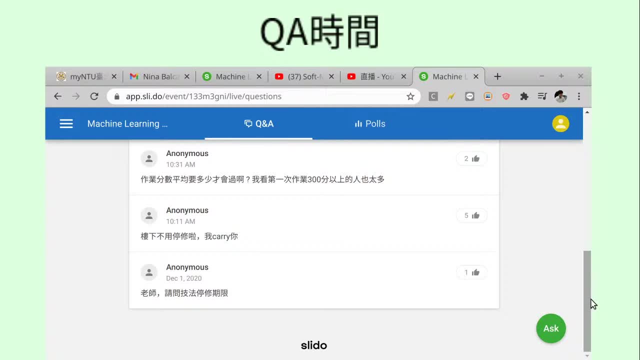 那基法的话我本来的assumption就是跟学校一般的停修期限是一样的OK那总之任何时间内你来过我签我所谓的签只是学校认不认账我不知道OK所以就是。 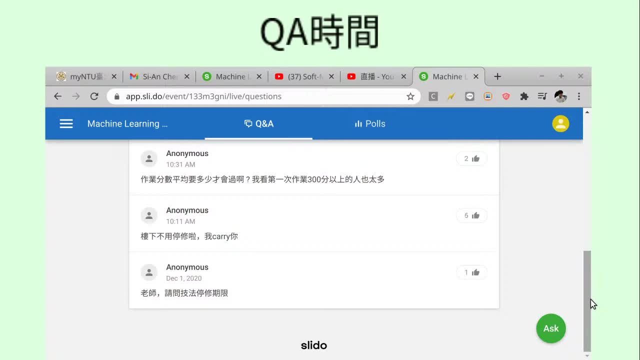 嗯。 大概是基法部分那尤其我们有不同学校的同学请你如果有想要停修或者想要任何情况的话麻烦一定要跟每个学校自己的注册组或相对的注册单位来做确认。. 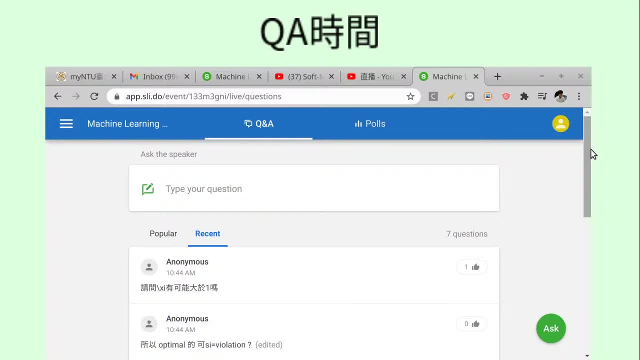 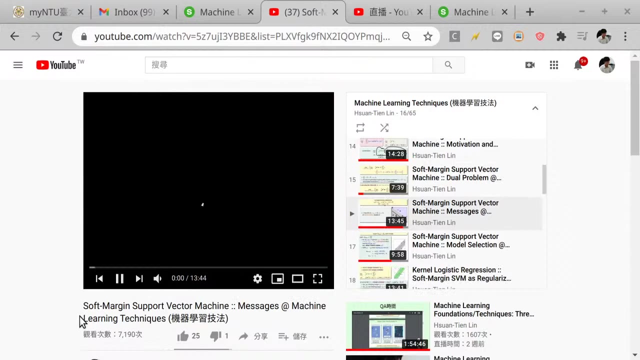 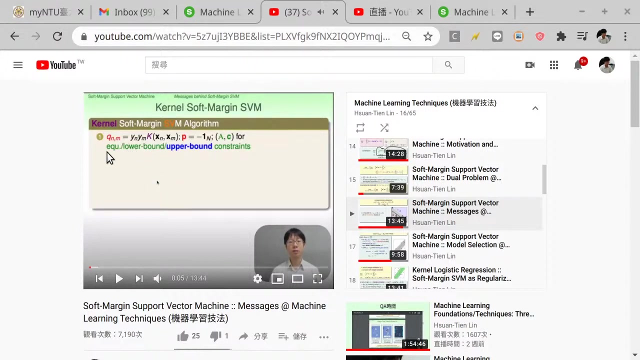 OK好有没有问题OK没有的话那我们来看看下面的一段。. 好推导完队友问题以后我们就可以得到所谓Kernel的Soft Margin, SVM所以现在不是HardOK是Soft说我们可以允许一些些违反胖胖边界的情形。 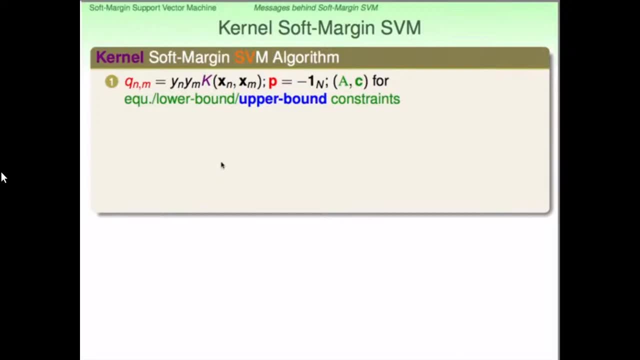 好那这个演算法看起来很简单。 跟原来我们知道的Kernel Hard Margin, SVM有什么不一样呢? 好其中一个不一样就是我们在解这个问题的时候我们需要加上额外的条件这些所谓Upper Bound这些上限的条件这从哪里来的? 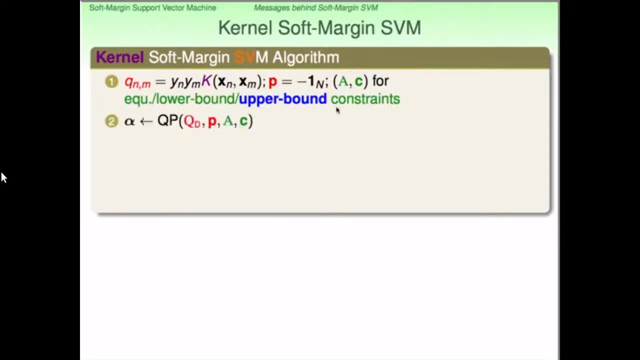 从我们那个C那个参数来的。. 好加上这个条件以后好一样我们就解出了这个QP的问题然后解到最好的Upper在哪里然后解完以后我们就做什么. 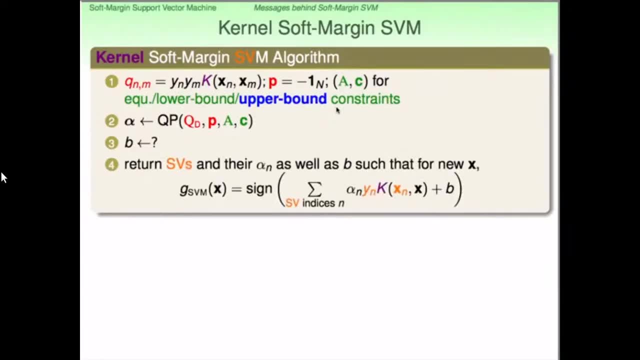 算B。 算B之后应该要得到最后的SVM的还怕是长什么样子。 Kernel的部分我们很熟悉了。 唯一剩下的事情是在这个问题里面我们算B的方式一样吗? 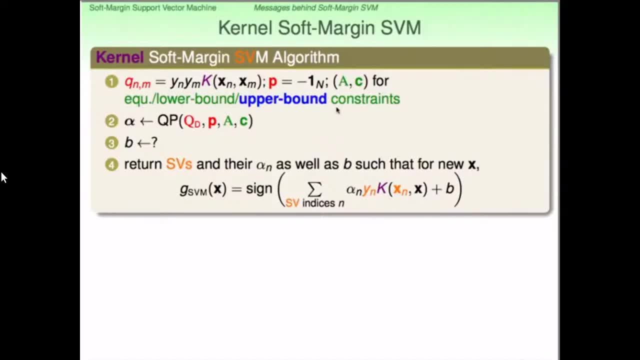 大家记得我们在Hard Margin怎么算B. 我们把KKT Condition列出来发现其中的某一条告诉我们说我只要用一个SVM的话我就可以得到B是多少。? 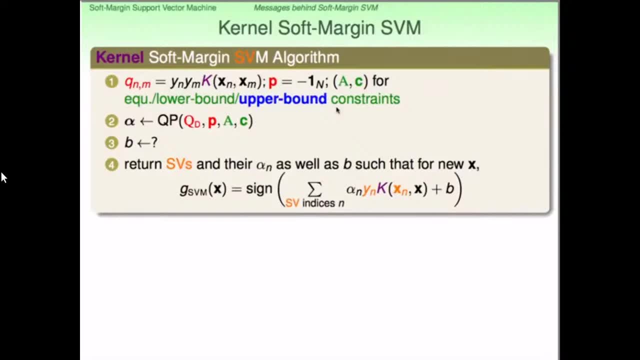 现在因为是一个新的QP问题所以它的KKT Condition已经变了。 变了之后我们是不是还能像以前的方法来算B呢? 这是我们要探讨的下一个问题。. 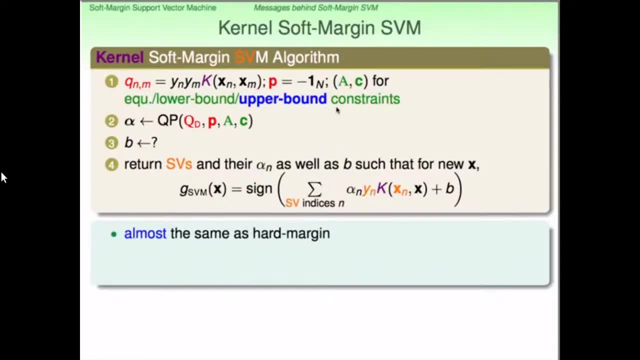 如果以这样的程序来算的话SVM其实几乎除了那个Upper Bound的部分跟Hard Margin是一样的。 但是这个问题会比Hard Margin来得Flexible。. 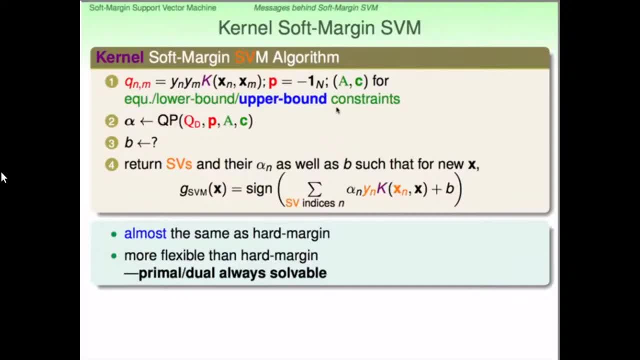 因为你可以控制你的这个C的值然后得到不同的你到底比较在乎胖一点的边界还是你比较在乎犯的错误很少。? 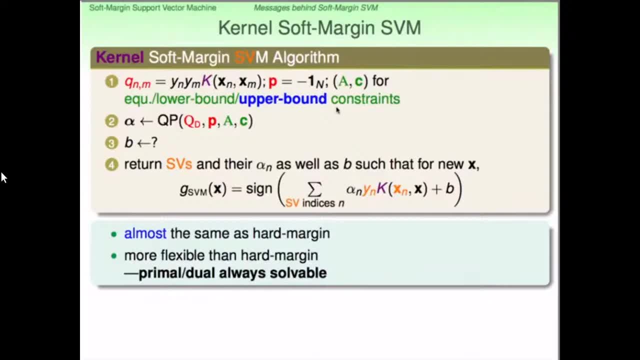 而且呢这个问题跟Hard Margin不一样Hard Margin说你一定要Separable才有界。 现在呢你不一定要Separable反正你总会得到一个界。. 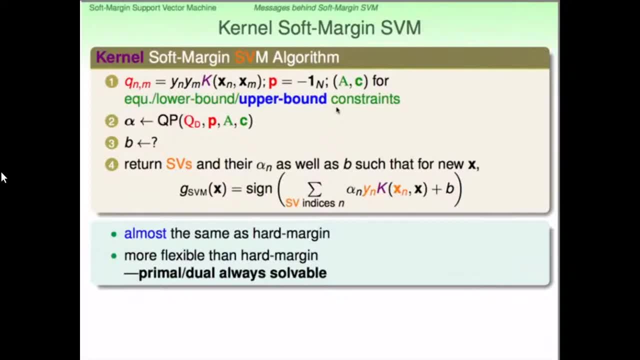 So Soft Margin实际上是实务上比较常用的SVM的形式。. 唯一剩下的事情是什么第三步要怎么算B到底要怎么算? 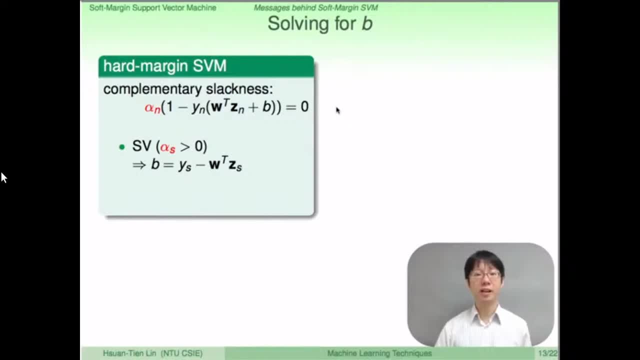 我们来看看我们在Hard Margin我们说找一个Support Vector. 它说Affa还有那个E减掉Y乘上分数这两个人Hard Margin跟Folium永远不能够说两个人同时活下来。 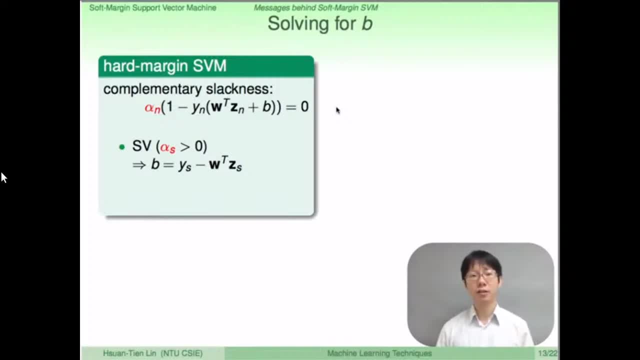 所以如果今天Affa活下来了Affa是大于0的那后面那项就要等于0。. 等于0的话我们就可以算出B的值是多少。. 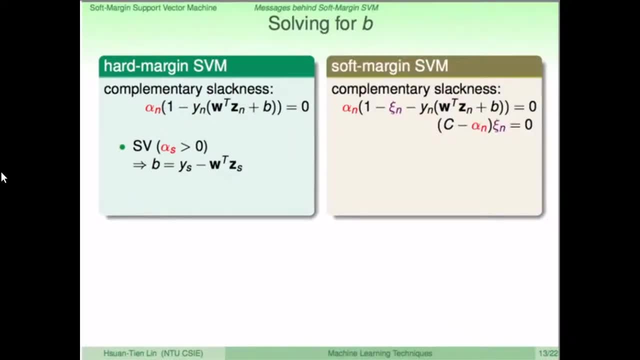 好那我们再来看看Soft Margin要怎么做呢? 我们也可以一样画葫芦列出这些Complementary Lackness也就是不能同存于世的这些条件。. 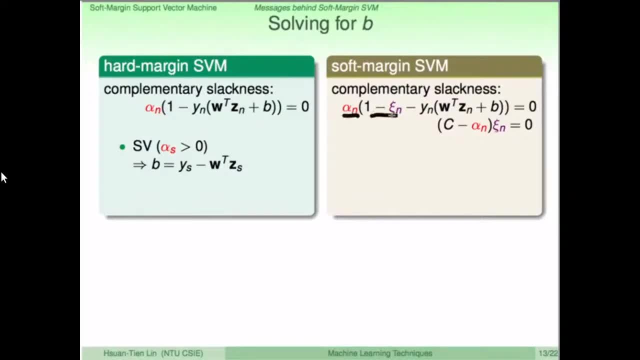 这些条件有什么呢其中一组是Affa乘上一个跟Hard Margin很像的A一个项然后要等于0。. 这个项里面不一样的. 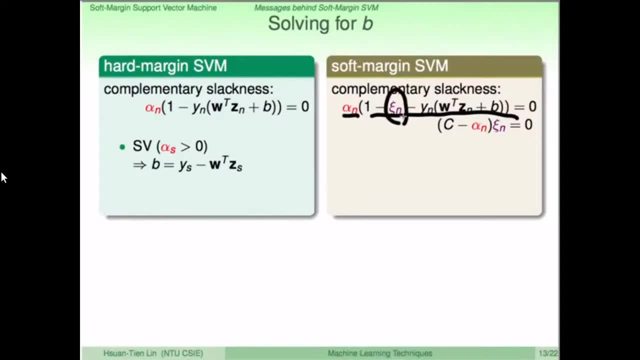 只有我们多了一个Cn这个变数这是我们用来记录到底违反多少变数。 然后还有另外一组条件是什么 另外一组条件大家记得的话我们应该有个Cn大于等于0,这组条件会对应到这个-Cn. 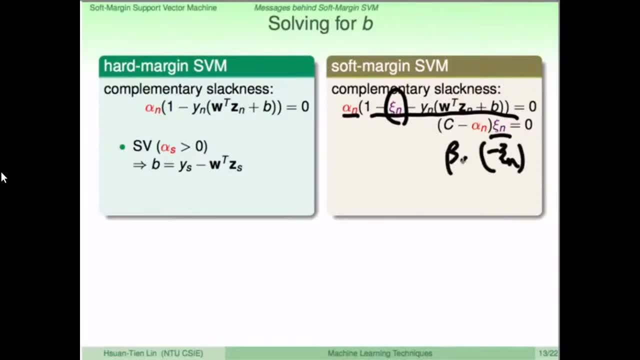 乘上它的Lagrange Multiply也就是我们叫做βn要等于0。. 不过从我们之前的推导大家已经知道βn最后就会是C-Affa n。. 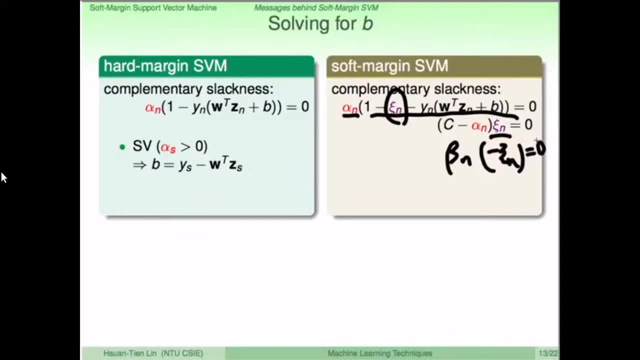 然后因为这个符号影响不大所以我们就简单的把它写成C-Affa: n乘上Cn要等于0。. 有这两个条件我们要怎么求出B呢? 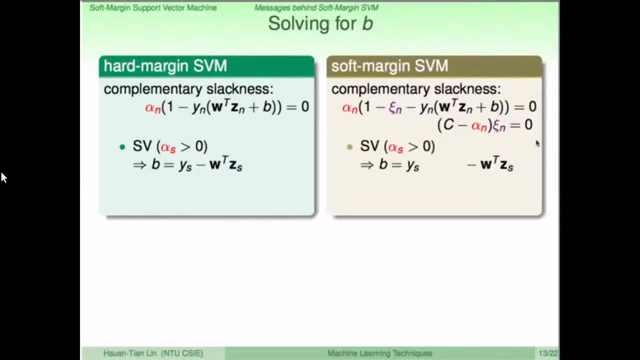 好我们照子来看。 以这Hard Margin的方式我们想说先找一个Support Vector。 Support Vector是什么Support Vector是Affa大于0的。 AFFA大于0的话我们就可以用第一组条件它会告诉我们说里面的这一串等于0。. 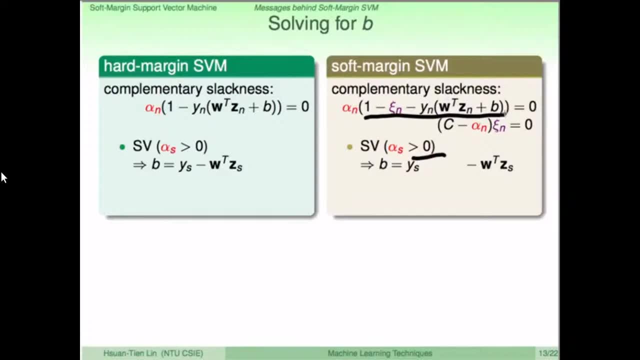 里面这一串等于0以后我们有没有办法求出B. 我们算一算B应该要等于Y减掉这个W乘Z这个分数可是还多了一项是Y乘上C. 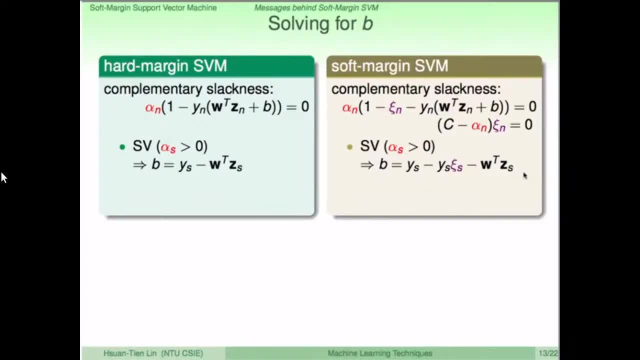 说要算出B我要先算出C可是C其实是违反的量所以要算出C我要先算出B。 哇这样来来来。 这位机身烂单身机好像就算不完了。. 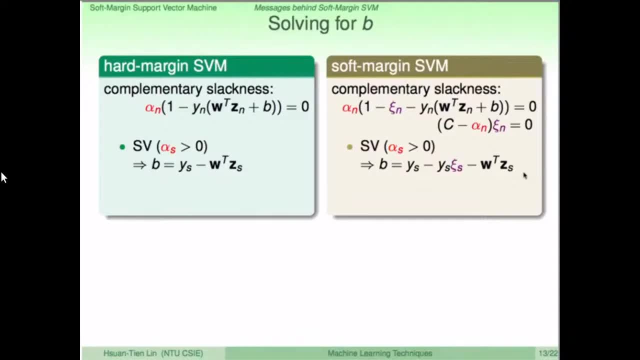 这样好像没有办法帮助我们很容易的得到B。. 我们要怎么很容易的得到B呢我们最想做的是什么? 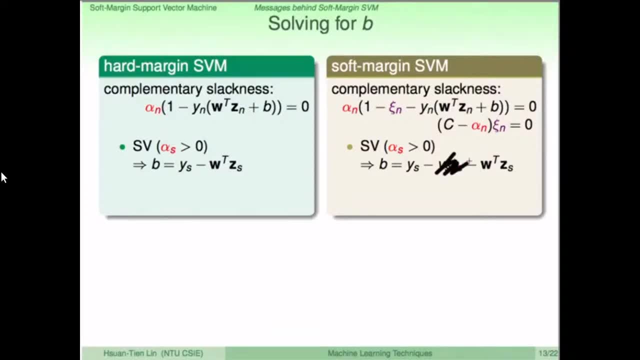 如果我可以把这一项干掉如果我让这一项挂掉的话那么我的B就可以像Hard Margin一样轻易的求出来。 我要把这一项干掉我要让这一项等于0的话也就是我就看上了这里我要可C等于0。 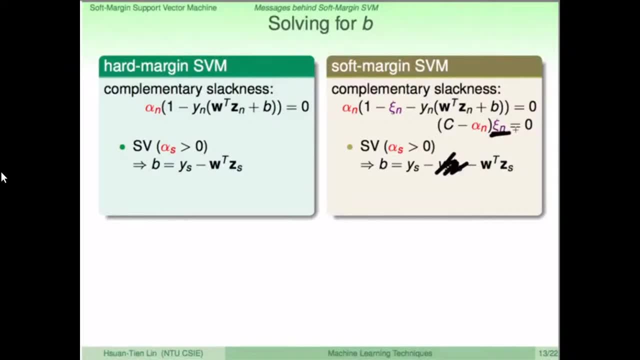 我要可C等于0,我就要确保另外一个人可以活下来另外一个人可以活下来的话也就是Affa N不能够等于C它要比C来得小。. 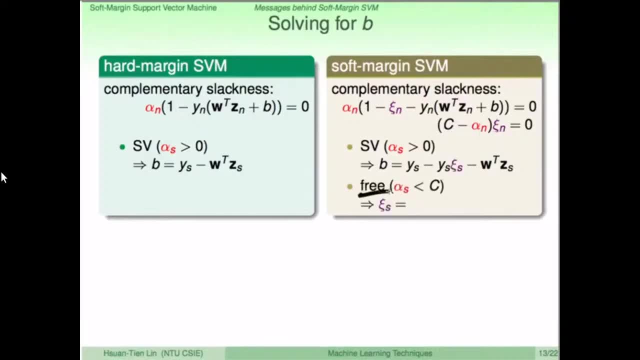 这种比C来得小的我们一般把它叫做Free的自由自在没有被那个C绑住的那它的可C就会等于0。. 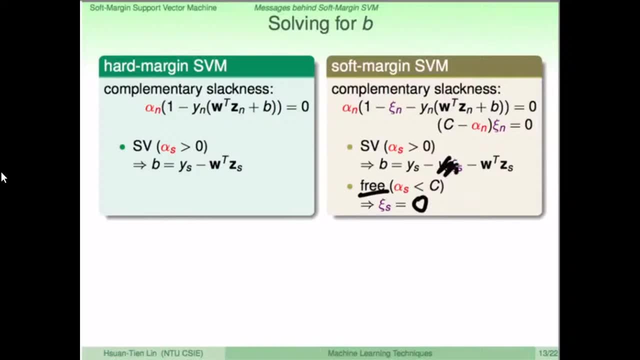 可C等于0之后我就可以把这里涂掉我就可以得到跟Hard Margin一样减低的式子了。 所以我们这里是这个样子做的我们想象说找一个Support Vector现在不是任何的Support Vector是一个Free的Support Vector。. 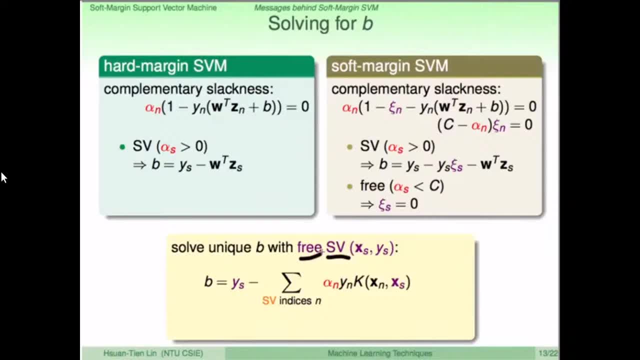 如果找了任何一个这样的Support Vector之后我们的B就可以很容易求出来它就是它的Y的值减掉算出来分数的值。. 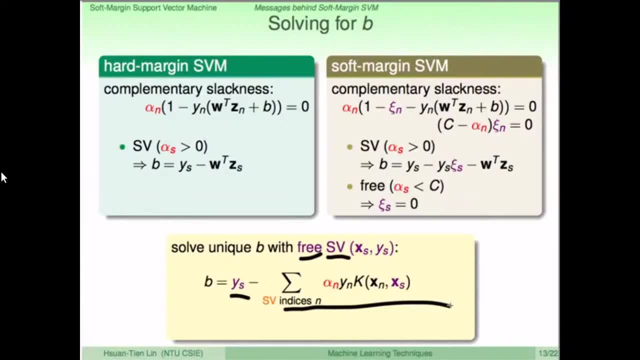 这个值是可以由Kernel转出来的。 这个B是个唯一解任何一个Free Support Vector都应该要告诉你这样的解。 你说那要是没有Free Support Vector怎么办会不会有这种情形? 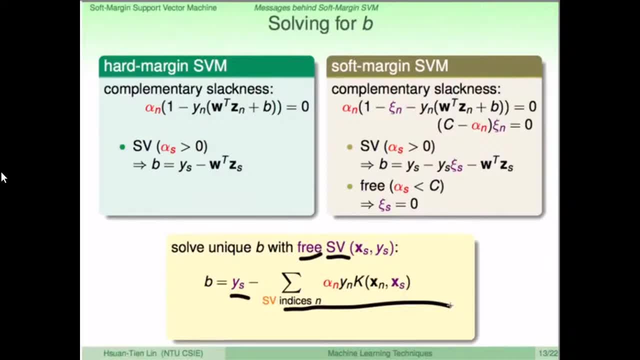 极少数的例子会会有没有Free Support Vector的情形。 那么你的B就只能有一堆的不等式来限制这个不等式可能会给你不止一个B的答案然后这些B的答案只要它满足所有的KKT Condition的话这些B的答案都是可以的。. 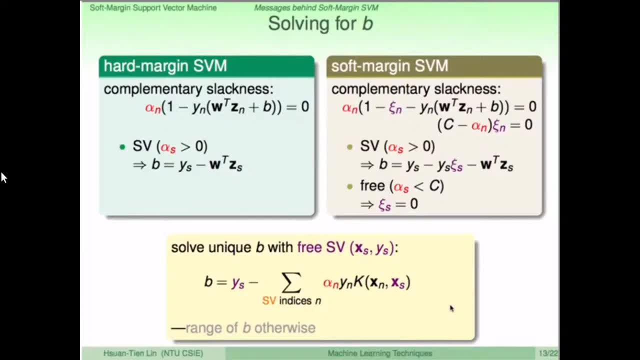 这个细节比较复杂我们这边不讲。 绝大多数的情形你都有Free Support Vector。 你有Free Support Vector之后你就只要用上面那个式子就可以得到B的唯一解了。. 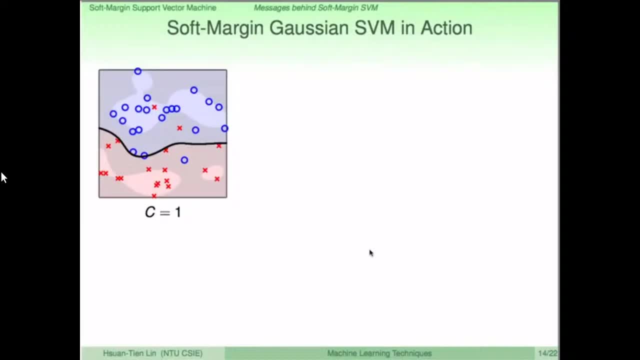 好那我们现在知道Soft Margin知道它的Kernel的方式之后我们就可以做什么, 我们来看看它的表现怎样。. 好我们一样使用我们的所谓的高悬Kernel然后来看看我们现在把C的值做一些不一样的变化的时候发生什么事。 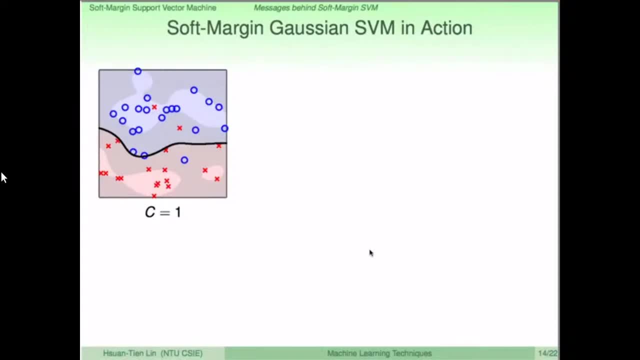 这个是某个高悬Kernel我们用C等于1的时候。 好大家看到得到这个边界这个边界说这个边界的上面是蓝色的然后下面是红色的。. 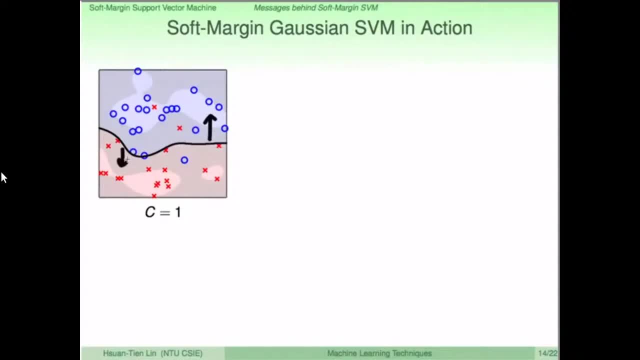 我用灰色的地方标出它的Margin的部分。 就是那个胖胖的边界。 在Z空间里面。 胖胖的边界对回X空间到底长什么样子。? 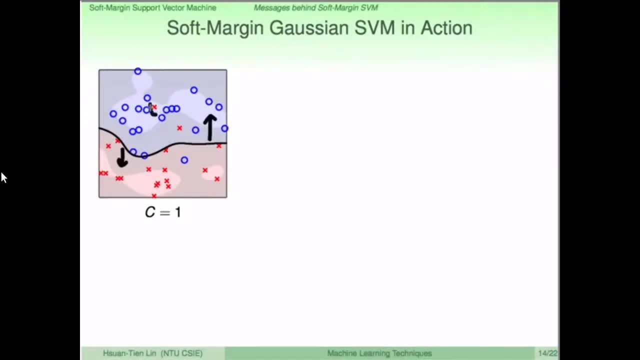 然后大家看到说这个C等于1的时候我们的SVM犯了一些错误像这个红色的落到蓝色里面这显然是个错误。. 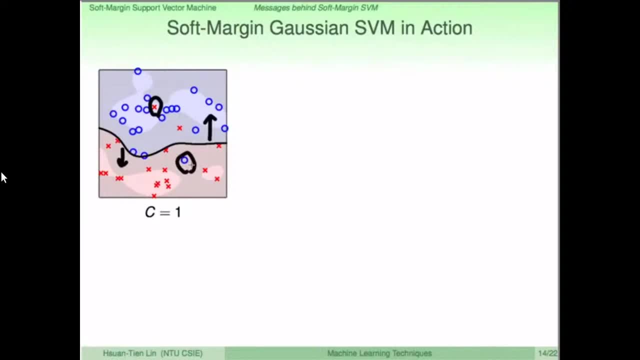 然后这个蓝色的落到红色区域里面原来说落到边界的红色区域里面这显然是个错误。 也会有什么也会有蓝色的落到它是正确那边但是还是落在边界里面。. 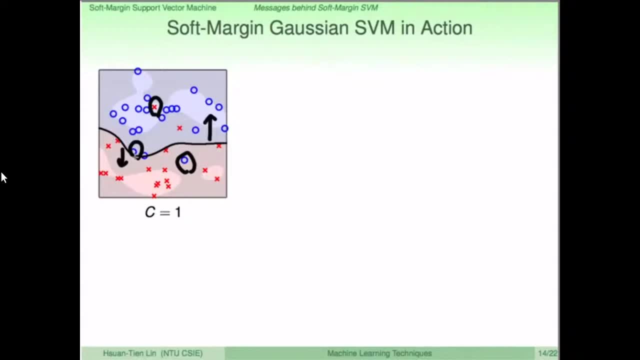 所以有很多个错误错误意思是说我违反了Margin的错误。 好那如果今天C等于10呢我很在乎尽量不要犯错。. 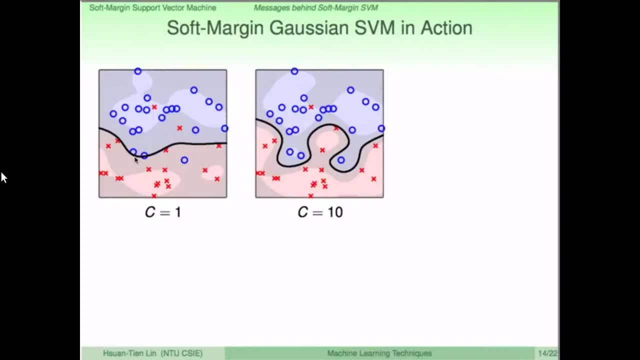 边界少一点这个瘦一点没有关系。 大家可以看到说犯的错误相对来说变少了。 也许这个点还是错的但是刚才犯错这个蓝色的点已经到了对的那边。. 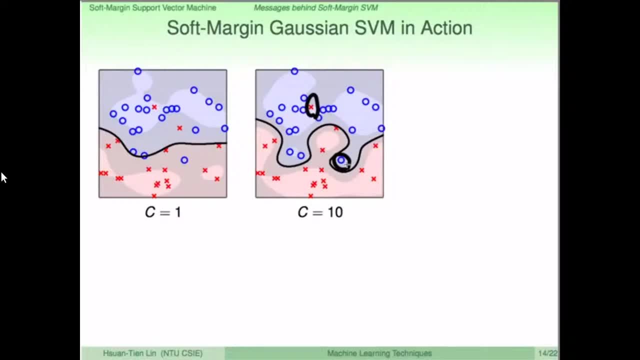 它可能还是有一点点小错因为它还是在胖胖的灰色的边界里面。 但是已经不是像刚才那样算是个大错跨座边界的大错。. 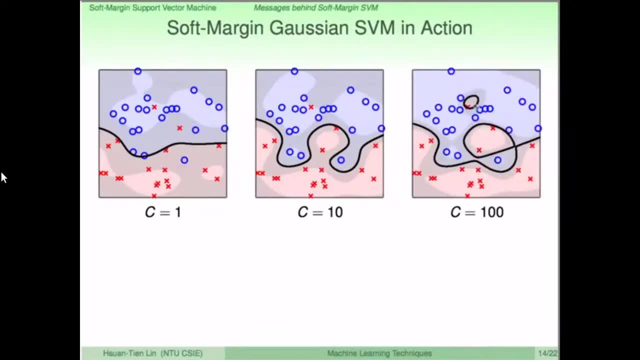 我今天C等于100呢看起来刚才这个做不好的XX也几乎刚才这个上面这个做不好的XX也几乎做对了。. 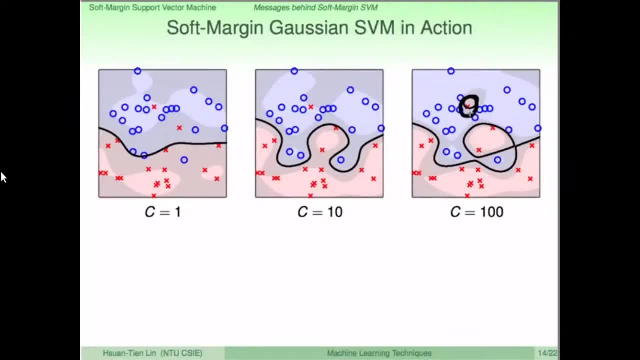 所以C越来越大的时候 看起来能够做对的就会越来越多。 因为我们希望说Margin Violation越小越好不要做错。. 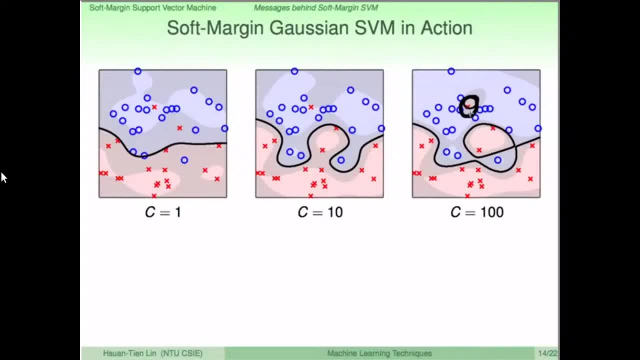 但是当然大家看这个图的话可能也会觉得有必要用像C等于100这么复杂的吗. 会不会上面那个XX根本就只是个杂讯而已。? 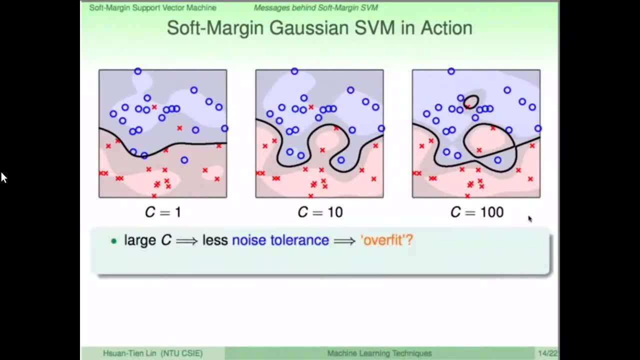 所以一样你的C的值如果调不好可能你的Soft Margin SVN对于杂讯的容忍度就没有那么高。 那会怎么样那会Overfit。. 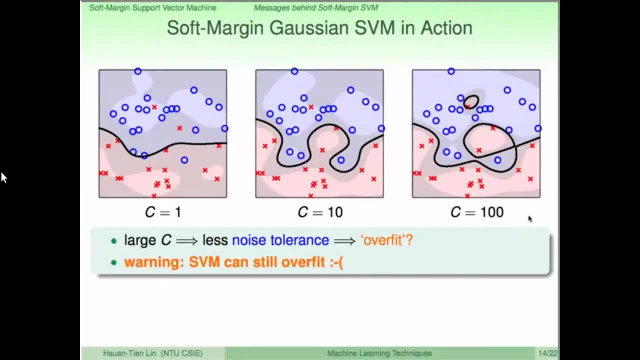 所以再给大家一个讯息SVN就算是Soft Margin SVN也是有可能会Overfit。. 如果你没有把SVN就算是Soft Margin SVN也是有可能会Overfit。. 参数弄好的话。. 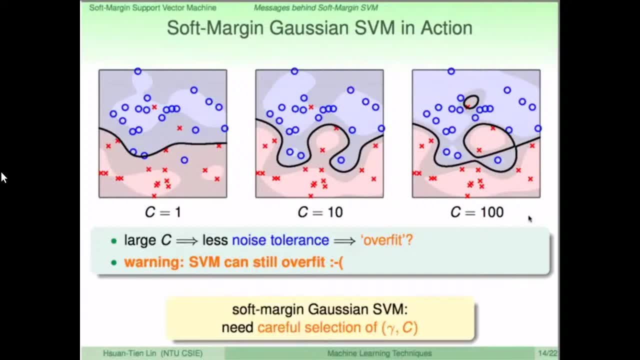 所以我们需要做什么需要好好的选参数。 选Gamma选C。. 想高选SVN可能要选Gamma选C。 若是Polynomial SVN可能有更多的参数要做选择。. 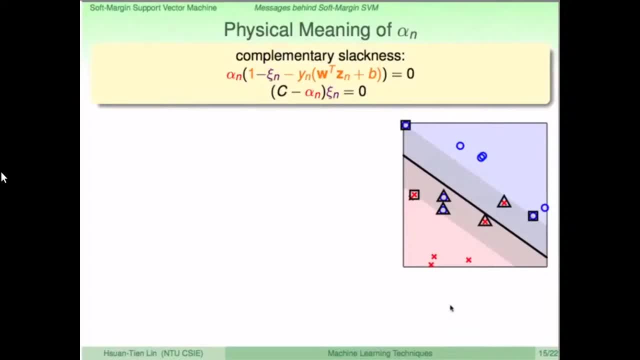 好那我们刚才已经用到Complementary Slackness这样的条件来为1,解到B。 我们再从这条件来看看Support Vector MachineSoft. Margin的Support Vector Machine到底告诉我们接什么讯息。 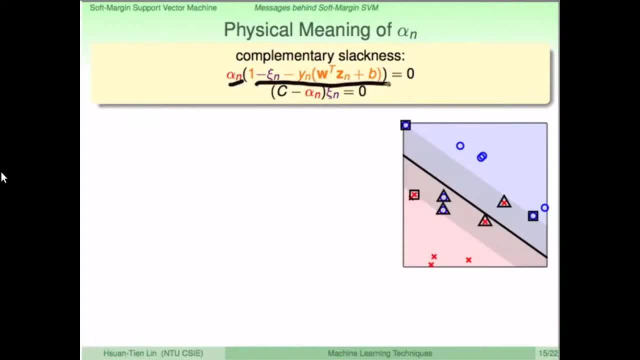 我们说我们有两组条件α乘上某一长串的东西要等于0,C-α乘上Cn要等于0。 从这两组条件我们可以把我们手上的点每个点是配一个α分成三种。 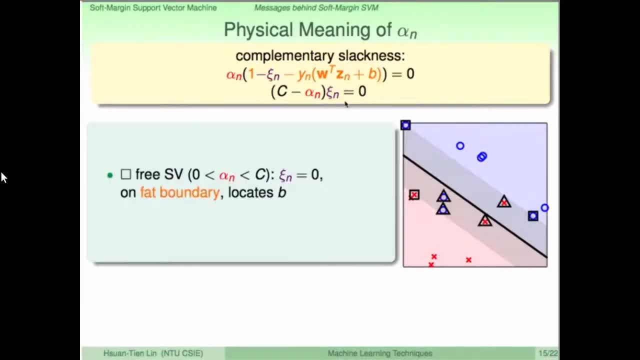 第一种是我们刚才已经用过了Free Support Vector。. Free Support Vector有什么特性它的可C会等于0,因为α接在0跟C之间所以前面这项不是0,后面那项就是0了。 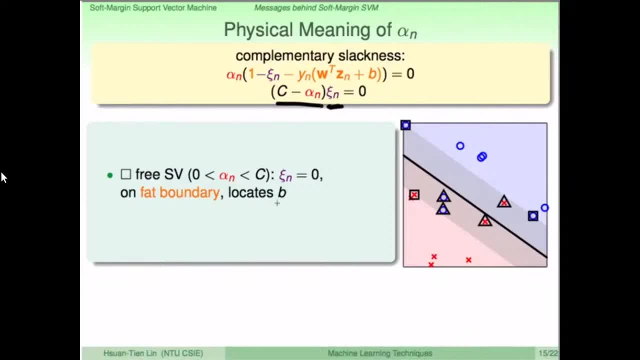 我们刚才用这个条件来什么来为1的算出B到底是多少。 为什么可以算出B是多少我们来看看这个条件α大于0,所以里面这一串样是0,然后我们刚才又说可C是0。. 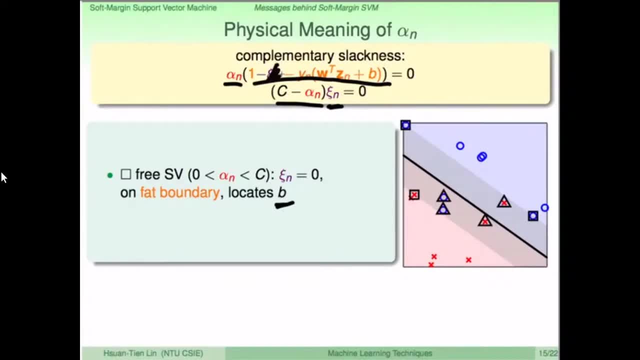 所以它实际上是0。. 实际上得到的事情是1减掉y乘上分数要等于0。. 这些是什么点好从我们hard margin一路介绍下来大家已经知道y乘上分数要等于1的那些点就是刚刚好在胖胖的边界的点。. 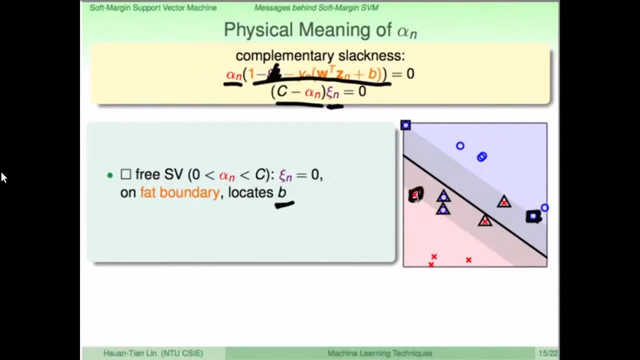 我这边用框框框来代表。所以Free Support Vector就是这些框框框刚好在胖胖边界上的点。. 然后还有哪些我们说还有Num Support VectorNum Support Vector就是α等于0的。 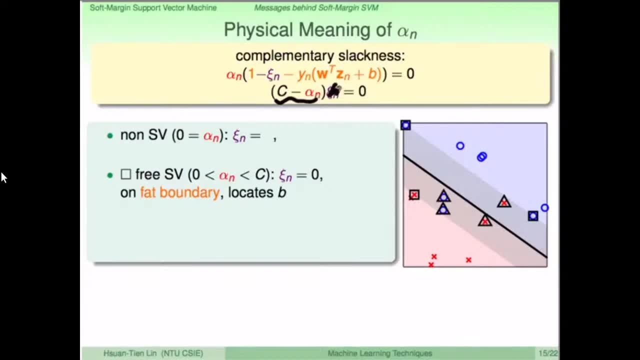 α等于0的话我们看到这边这一项就不是0了所以可C就是0。. 可C0的是什么? 可C0是没有违反任何胖胖边界的点。. 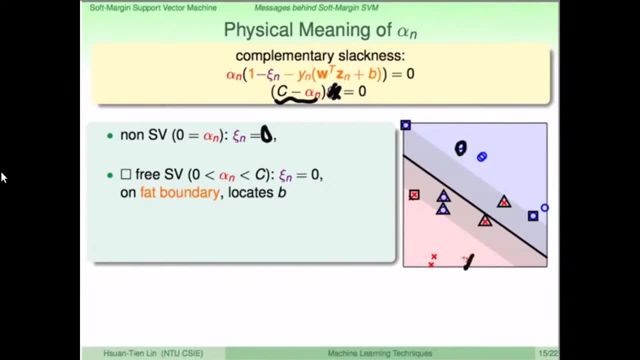 这些可C是0的所以例如说这个圈圈没有违反胖胖的边界这个xx没有违反胖胖的边界这些点都是可C是0的。. 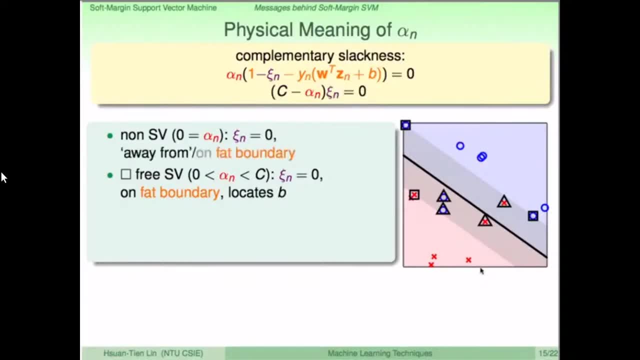 这些点大部分会落在哪里大部分就会在胖胖的边界的外面因为这样才没有任何违反。 当然有极少数的情形它会刚好在胖胖的边界上不过那是少数的情形。. 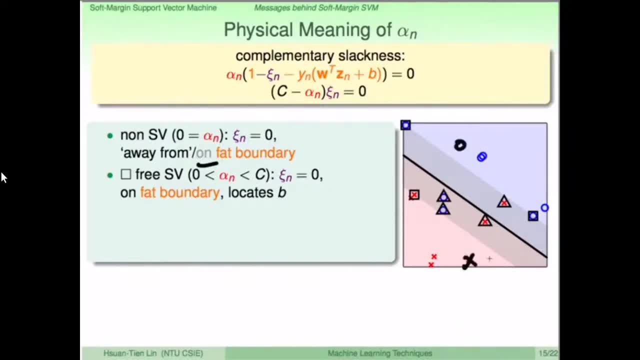 绝大多数的情形都会向往这边飙转这个圈圈或这个xx离胖胖的边界还有一段距离。. 好所以我们有αn等于0的αn在0到C之间的下一种情形就是什么就是αn刚刚好是C的。 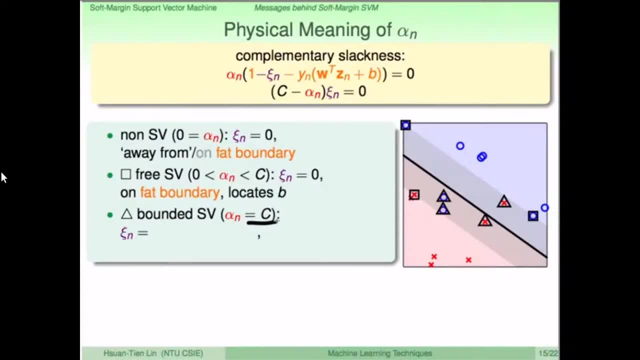 αn刚刚好是C的从我们上面的那些条件告诉我们什么事情αn刚刚好是C所以里面的这一项要是0哦。. 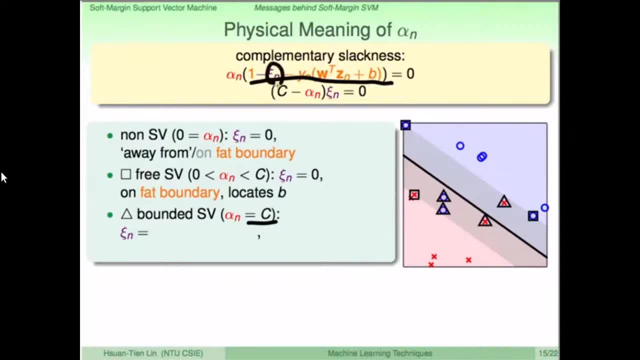 里面这一项要是0就代表什么代表我们的可Cn刚刚好就要等于1减掉y乘上分数也就是什么. 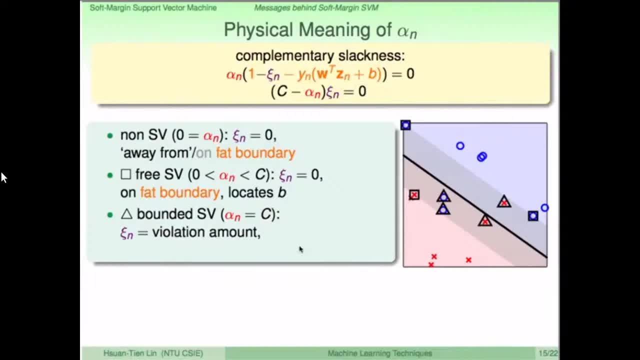 可Cn就刚刚好记录了到底违反了多少。 所以这个情形一定是有违反有违反然后我们用可Cn记录下来它到底违反多少。. 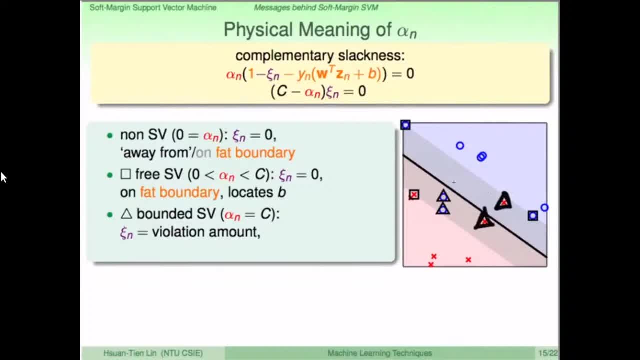 哪些点我标三角形的这些比如说这个xx或者是这个xx或者是这一个圈圈这些是有违反的。 大家注意到违反还有两种违反一种是小小的违反像这个xx是小小的违反小小的违反有没有跨过中间那条中线没有。. 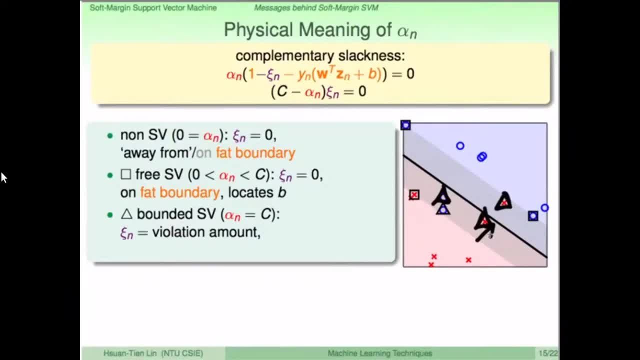 所以它虽然有一点点违反但是没有造成我们的分类错误。 但是有另外一种是什么大大的违反它已经跨过中线甚至跨到更远的地方去了。. 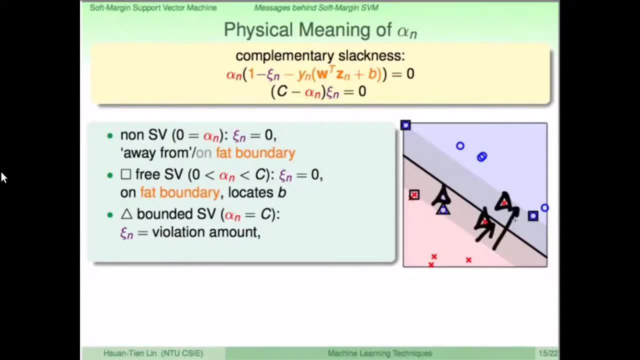 那这种就是很严重的错误。 好所以这些违反的情形都会有αn等于C。 极少数的情形刚刚好在边界上也会有αn等于C不过那个极少数的情形大部分你只要看到αn等于C就知道它有违反了我们要的方向的边界。. 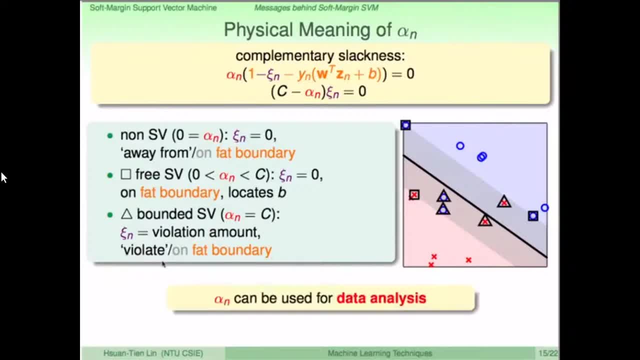 所以从这样从α值我们就可以把我们手上的点做完SVN之后分成三种。 那这三种对于你做资料的分析哪一些是可能有noise的哪一些是可能有帮助的哪一些是可能可有可无的容颜。. 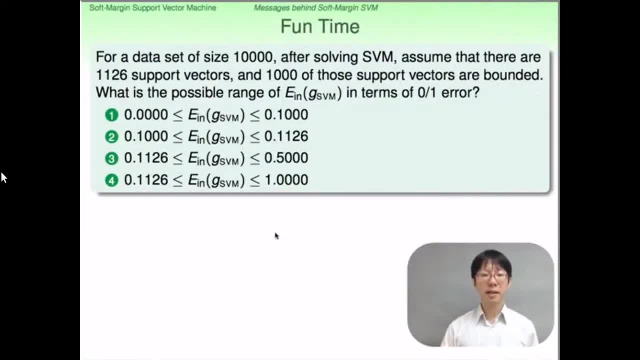 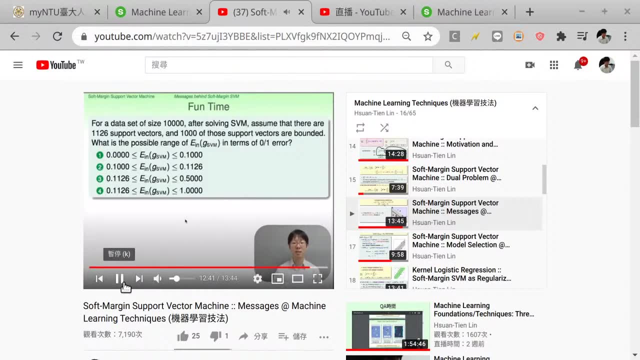 这些你都可以去看。 你都可以分得出来。 好讲到这边呢我们就给大家一个练习说如果今天有个资料它有一万笔的资料那解完soft margin SVN我们现在就直接叫它SVN了因为它其实是最常见的。 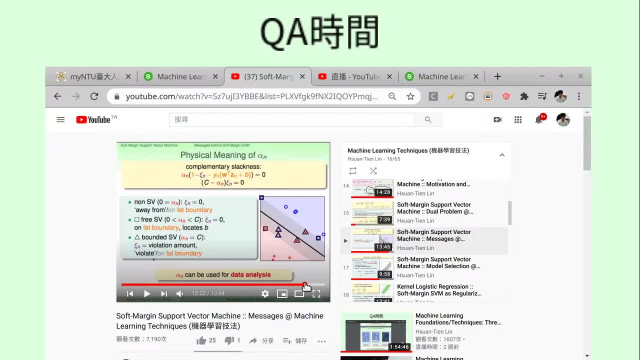 好所以我们上完了这个soft margin, SVN背后的这些东西。 一样你丢到一个QP。 你丢到一个QP丢到一个QP然后有kernel等等的。. 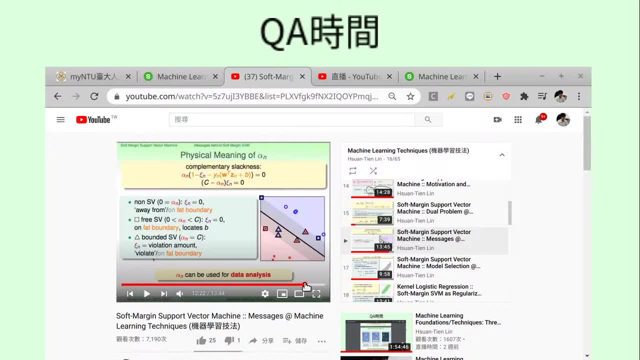 那丢进去以后然后把它解完。. 那解完以后我们教了大家怎么算B。 如果你有一个free support vector就是在0到C中间的那个α的话那就可以拿来算B。. 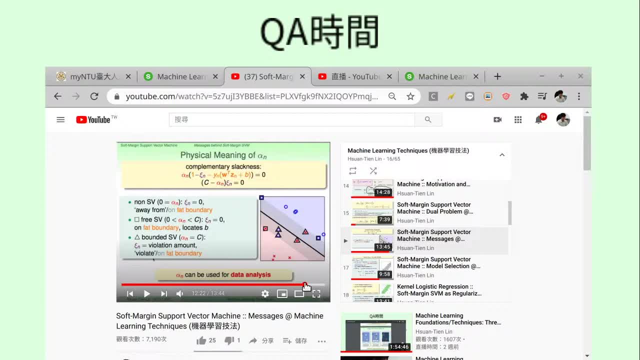 如果你有很多个free support vector每个给你的结果应该都要是一样。 Hard margin是类似的就是那些真正在胖胖的边界上面的点。. 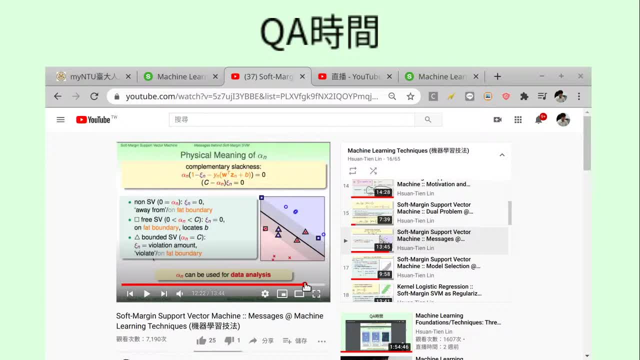 如果你没有free support vector意思是说你说的点你不知道它是不是在胖胖的边界上。 有可能它刚好是但是有可能它落在外面或者就落在另外一边就是你的B。. 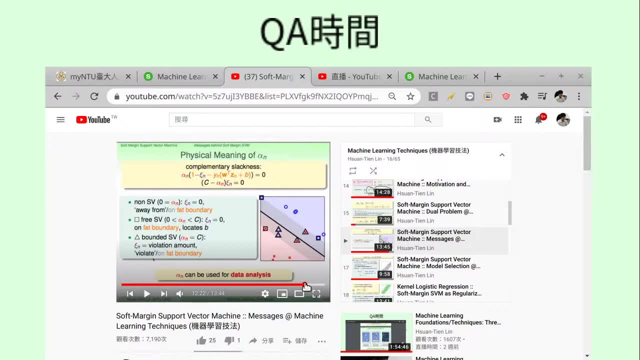 那就会有一些范围来做决定。 意思是说因为你的每个把法都是0或C的时候代表说你可能只有一堆的不等式。. 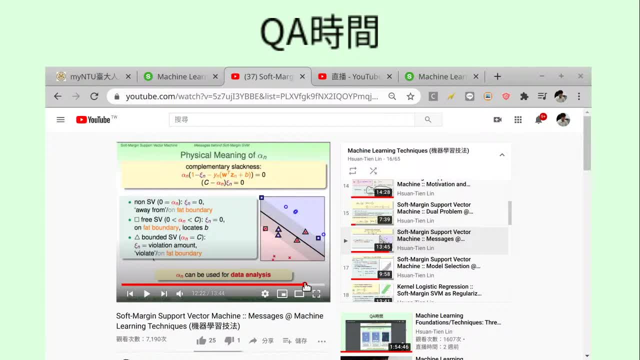 这些一堆的不等式会告诉你的B要满足哪些条件可是有很多个B通常都会对。 所以有这个解B的方法。. 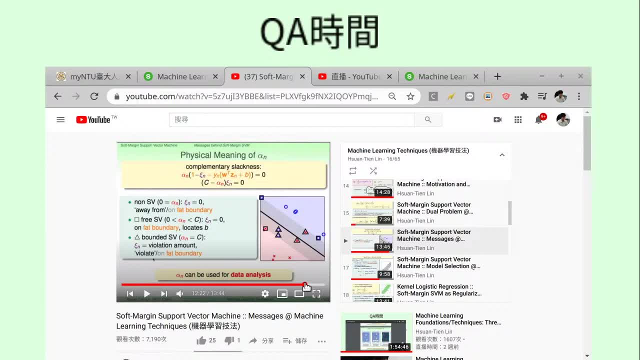 你如果看一般的software package例如说libspn的话它当然就是把比较完整的case都inform出来说. 今天不管你有free support vector还是没有free support vector它都会帮你算出一个它觉得合理的B的值然后对它的输出。 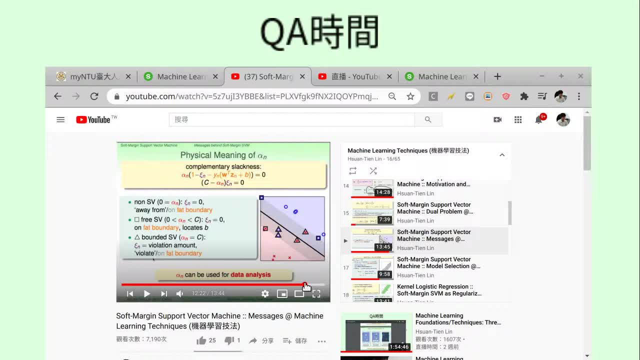 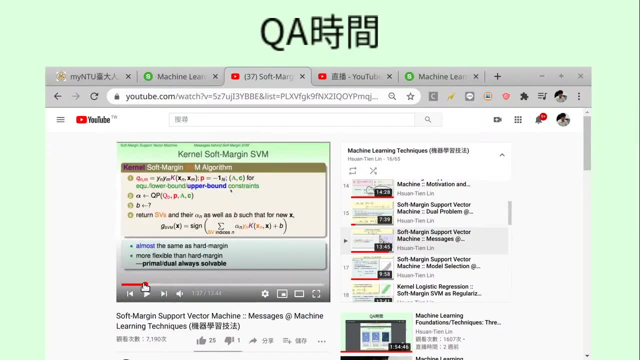 所以跟hard margin一样你得到了α你得到了一堆α你得到了B你就有你最后的kernelspn的输出。 那我们附带告诉大家的是说α的值其实是有一些意义的。. 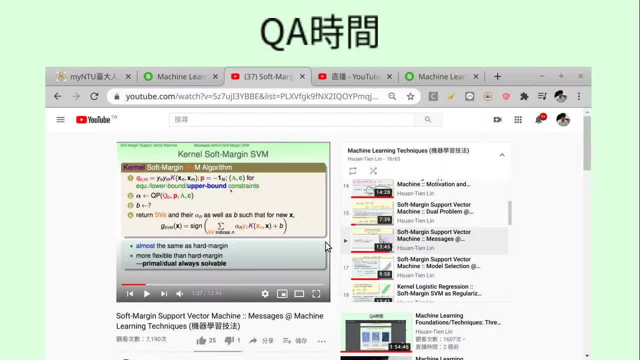 就像我们在hard margin的时候我们说那时候α有两种。 一种是是0的α一种是不是0的α不是0的是那些support vector它告诉我们胖胖的边界在哪里。. 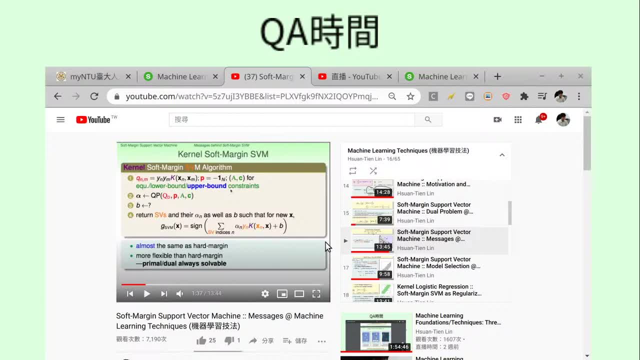 现在在soft margin里面α有三种。 一种是是0的一种是在0跟C中间的然后一种是是C的。 那是C的代表有violation。. 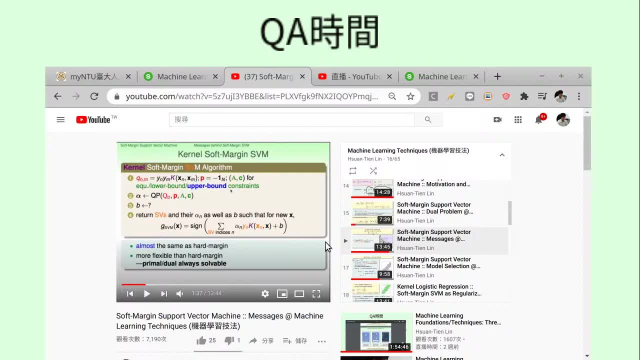 那是0的代表generate代表没有violation。 那如果这个是在中间的代表在胖胖的边界上面。 那所以这其实是蛮好的一个方式说如果你今天把一个spn用在你的资料上面。 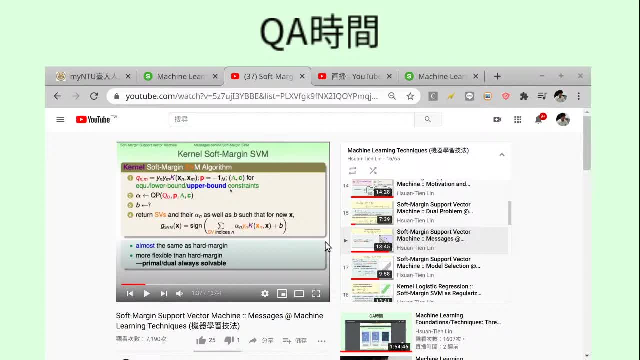 用完之后你想要看看spn到底怎么看待你的资料里面的每一个点的话。 那它可以告诉你一些额外的讯息比如说那些outlier你搞不好可以human看一看到底有没有什么问题。. 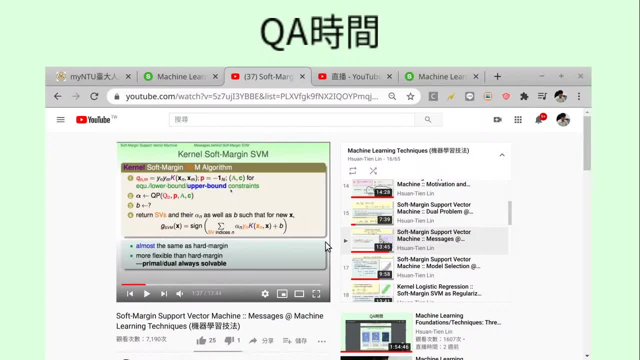 或者是进一步的解决。 进一步的去想一想说落在边界上的那些有没有什么重要的information。 好所以这是soft margin spn的部分。. 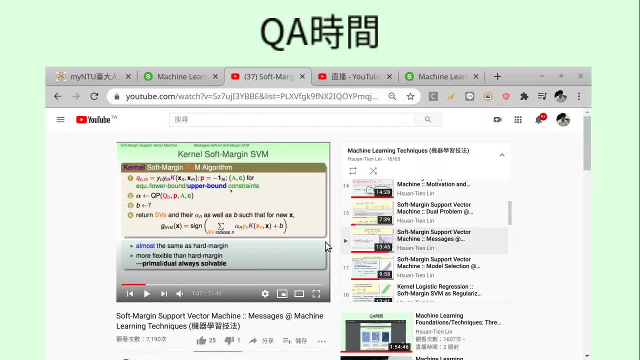 大家有没有什么问题. 请说。 如果是落在边界OK所以同学的问题是说落在边界上的可能有这个什么information。 那举例来说OK在spn里面OK因为我们知道包括你从hard margin的时候来看可能比较清楚hard margin的时候我们说落在边界那边就是你可以把其他东西通通丢掉留下边界那边你就可以重组出你最胖的边界是什么。 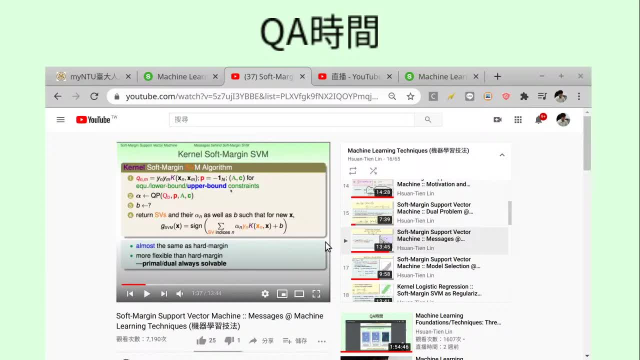 在soft margin这边也是类似的OK说那落在边界上的那些其实你只需要那些你就能够重组出你的classwork。. 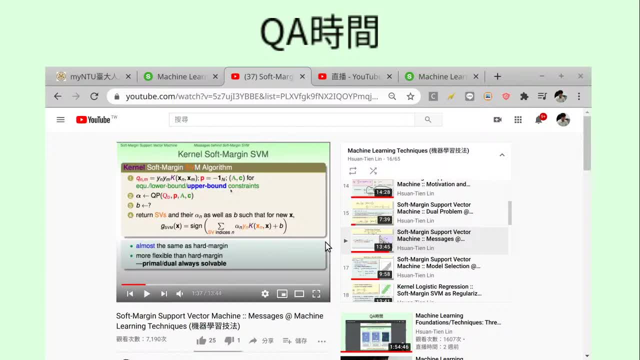 所以这些最靠近边界的OK你可能可以拿去解释OK说有点像你的classifierOK就是由这些产生的。 如果在高选spn里面的话你另外一个可能可以想象的事情是除去那些不在边界上那些等于c的等等的靠近边界上的其实是你的高选前面呈上的那个系数。. 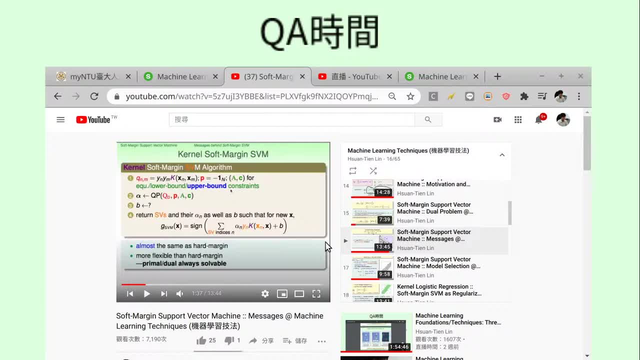 意思是说它是你的整个资料里面最代表性的部分OK。 如果你可以把spn想成一个去无存在。 你本来丢给他的3000笔资料他现在只留下50笔。. 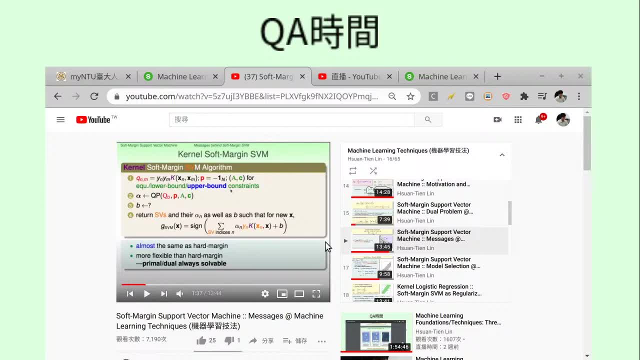 所以这50笔资料OK你是可以去看说那对你来说有没有道理。. 据来说如果今天是一堆这个病人的资料然后你要做一些事情的话会不会这些病人就是所谓的关键病人。. 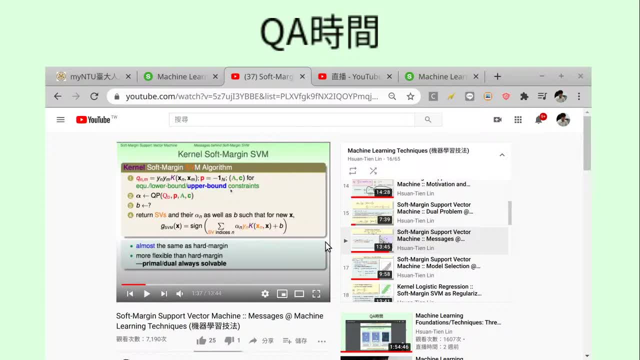 那这些关键病人它里面透露出一些什么讯息人类可以进一步的去解释然后去想说怎么样也许是refine模型也许在特定的应用里面。. 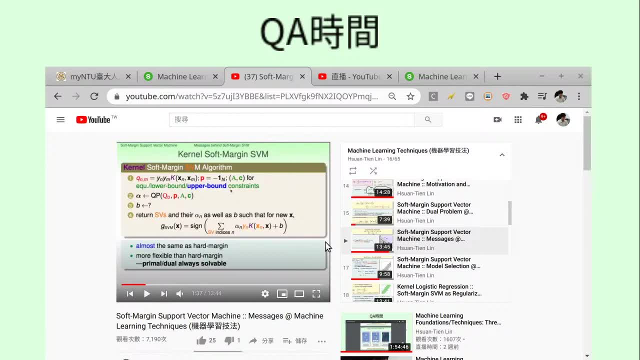 他可以对这个。 这个spn的决策得到一些解释。 我们说高线spn其实不是一个特别好解释的模型对不对。? 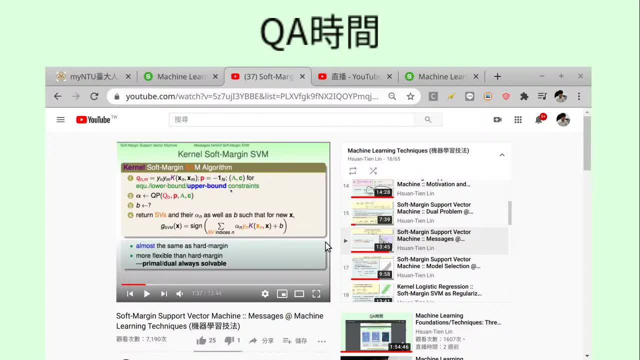 这个我们每次说你很难跟你老板说高线spn这个东西就是把我们的资料映射到无限多维度上然后在上面找一个胖胖的边界然后我们再对回然后找高线spn。. 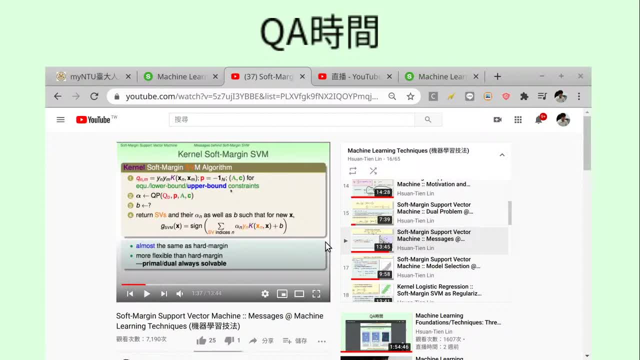 这件事情很困难。. 可是另外一个角度来说如果你跑完高线spn然后说好所以这些是高线spn看到的关键点那我们有可能可以说那我们是不是来做个case study说。. 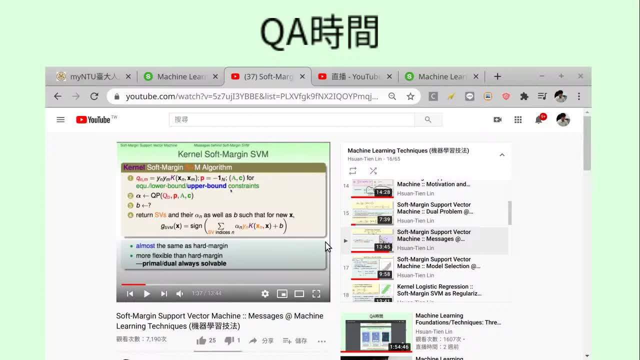 这些人例如说如果你今天是拿spn去分析你的客户资料那这些客户到底有什么特别的地方为什么这个客户是关键的购买的客户那个客户是最关键的没有购买的客户。. 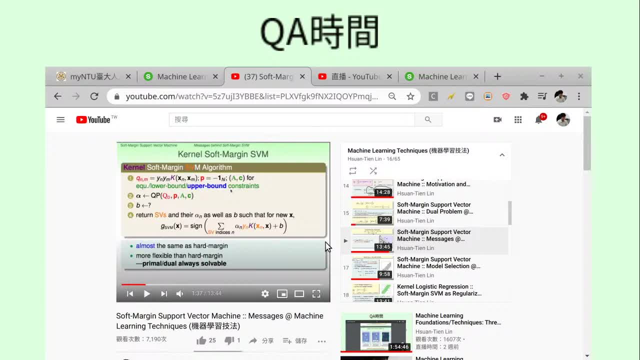 那可以后续的做一些case study。 所以我们highlight说他作为analysis tool的意思是这个就是说其实除了你的monitor你得到一个局之外你还得到一些额外的资讯而这些额外资讯抱歉在特定的应用里面。 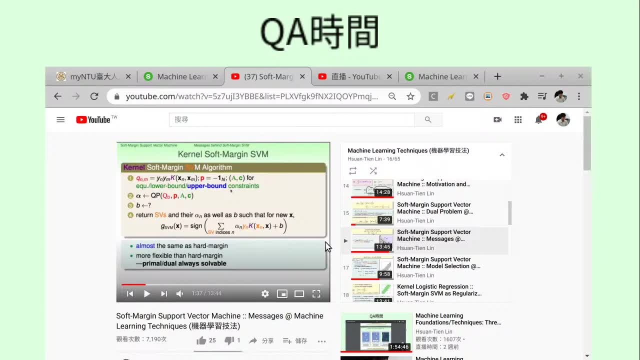 你可以选择要不要去使用它。 好还有问题吗? OK好没有的话我们这个上礼拜听说有个建议OK说这个我们要不要中间休息个五分钟这样子。. 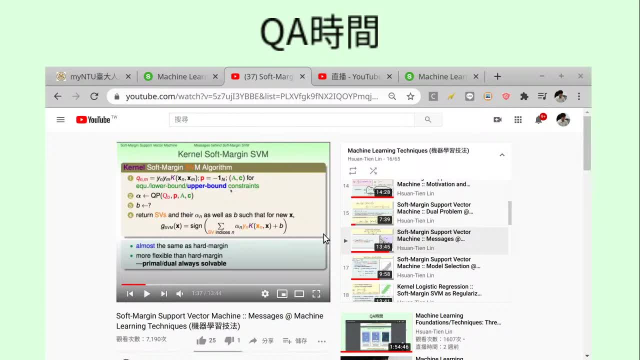 那我本来有点想说到下个礼拜等下下礼拜再来做这件事但后来觉得如果这是大家觉得适合的事情的话我们也可以先开始尝试一下至少知道有什么优点或缺点。. 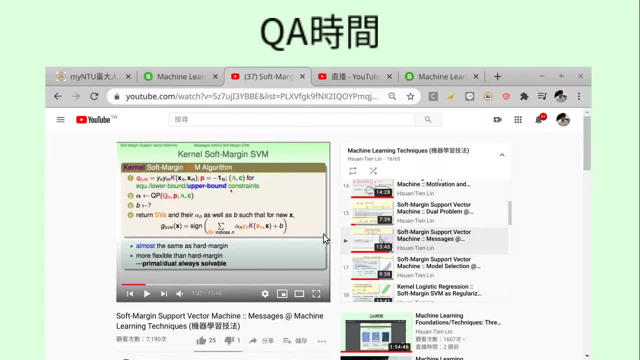 那所以我们先从五分钟开始。. 尝试起好了我们要休息过的十分钟所以我们现在大概十一点十五分左右我们就休息到二十分然后大家休息一下。. 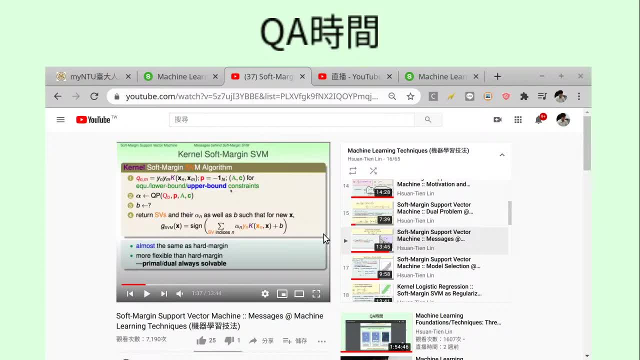 那如果有问题的同学可以来前面问我那我们看看状况怎么样我们再决定后续我们要怎么进行。 所以我们先做个五分钟的休息那唯一的一件事情是一轮上我要调一个五分钟的timer。. 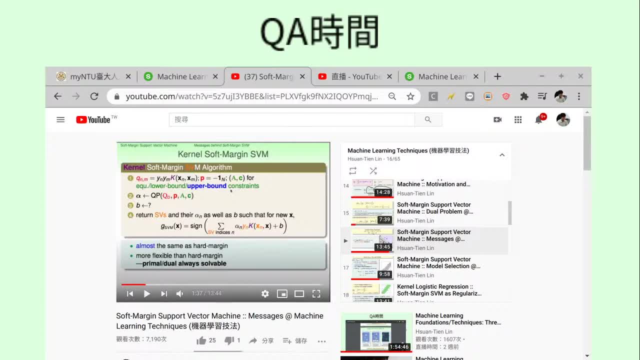 OK, Oh my god, 感谢感谢感谢你提醒我。 好。 五个小时也是挺不错的。 OK, 好谢谢。. 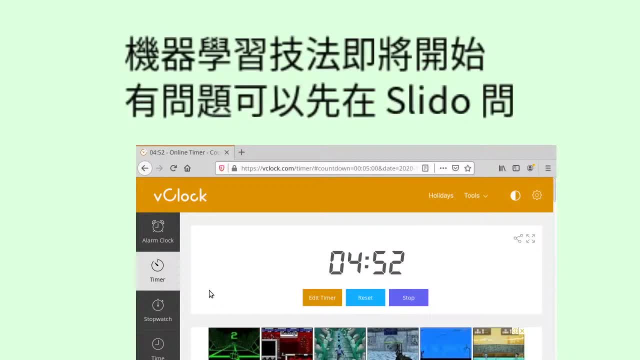 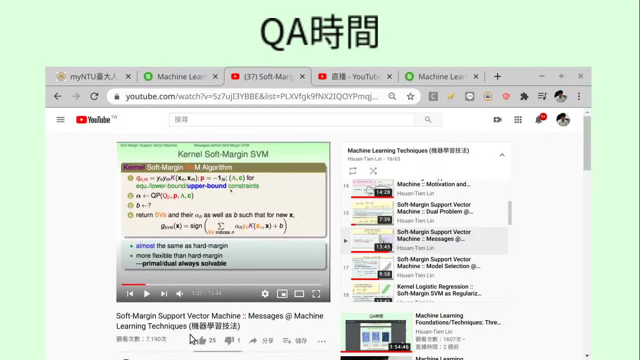 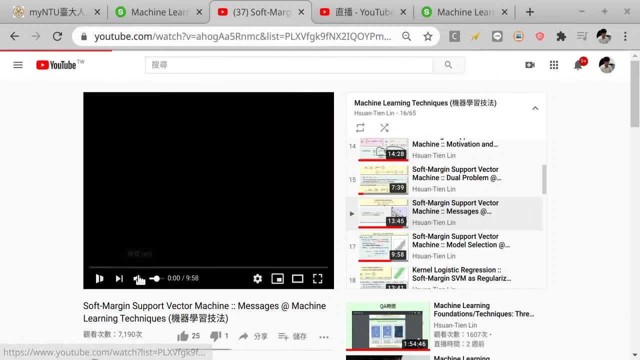 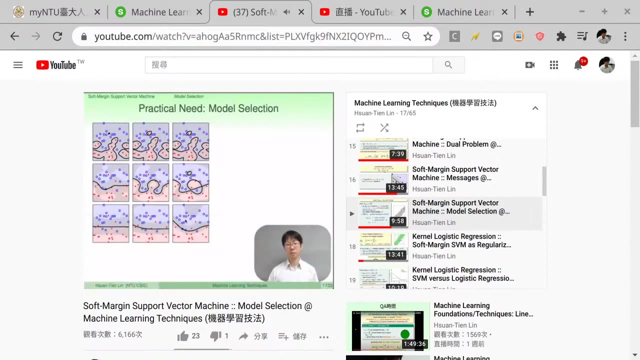 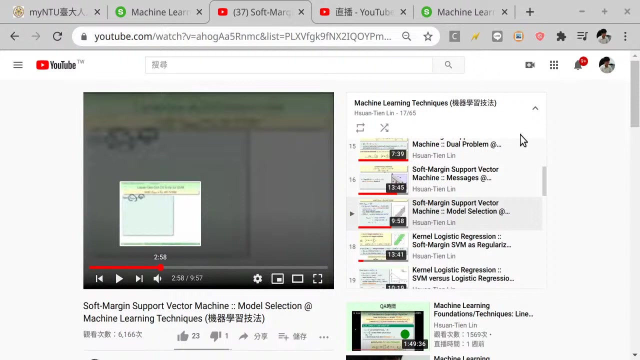 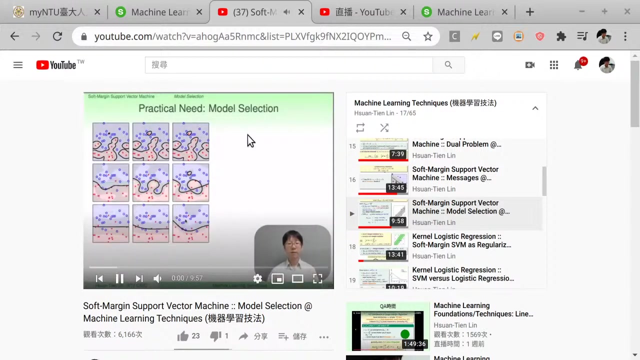 大家有没有什么问题? 没有的话, 那我们就来看下面一段的课程. 好那讲完了Soft Margin, SBN, 我们来看看. 我们说到选Kernel很重要. 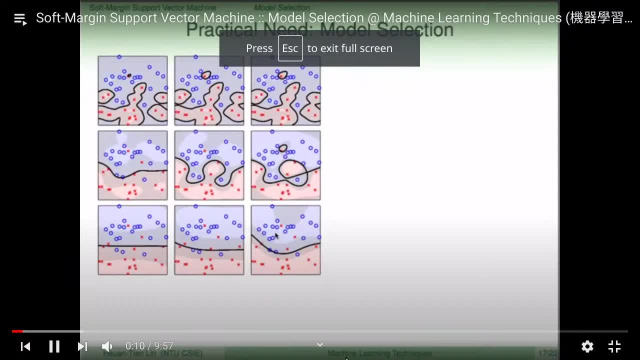 选参数很重要, 包括选C也都很重要. 那我们到底要怎么选呢? 大家看到说我列出来这个图是什么 是我通通都用高选Kernel. 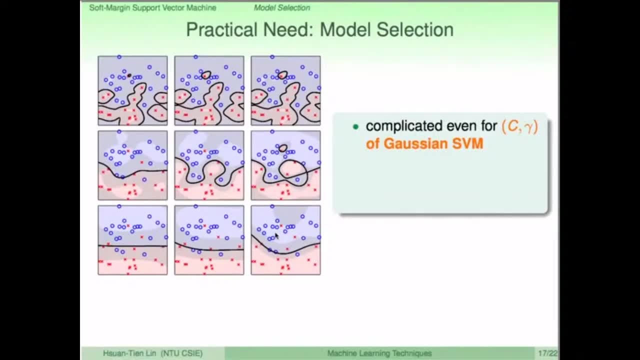 但是我用了不同的C跟γ的组合. 那这个横轴这边是各式各样不同的C 然后纵轴这边是各式各样不同的γ. 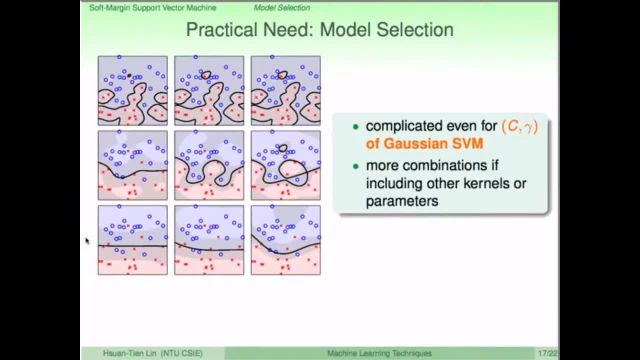 那如果你今天用的是Polymer 或其他的Kernel, 那可能你要做选择的事情就更多了一些. 好那怎么选? 我们唯一之前在机器学习提示里面教过. 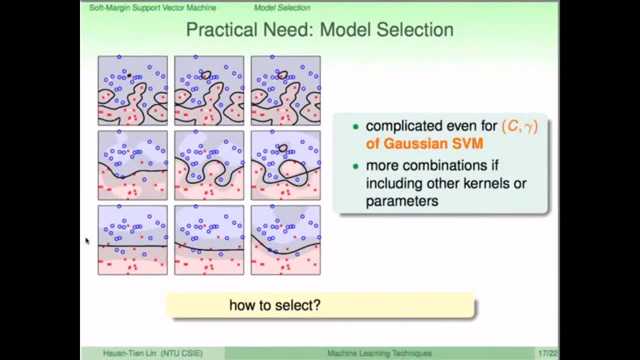 给大家一个非常肯定的答案: 你要选的时候最简单的工具, 最好用的工具实际上就是Validation. 你已经学过了Validation. Validation有什么? 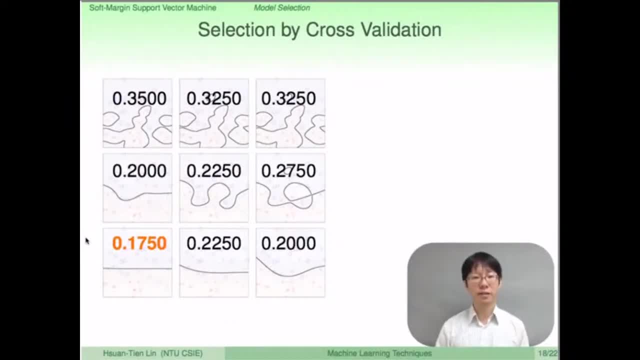 你说我就把Cross Validation值算出来, 然后看看Cross Validation值哪一个最小, Cross Validation Error 哪一个最小我就选哪一个. 像刚才那个情形. 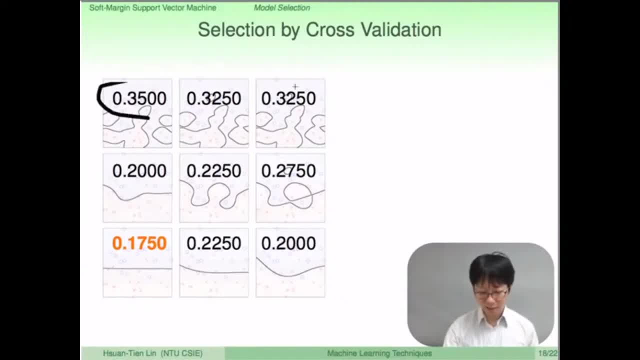 我列出来他们的Cross Validation Error. 大家看到上面这些 我们看起来好像很overfit的情形. 看Cross Validation Error其实还蛮大的. 那么下面的这些比较小一点. 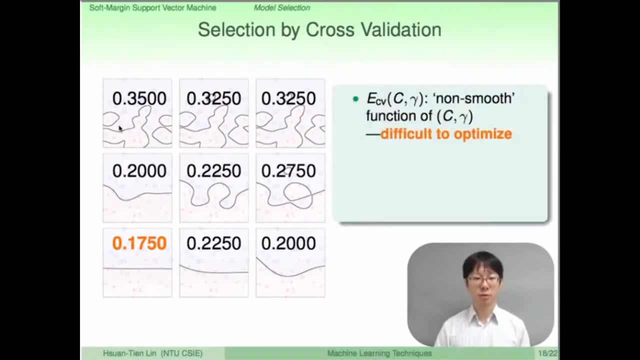 然后你就选一个最好的. 好这个大家应该已经会做. 你说为什么最佳化这个 故事是这样: Cross Validation Error是 你每个C每个γ送进会有一个值. 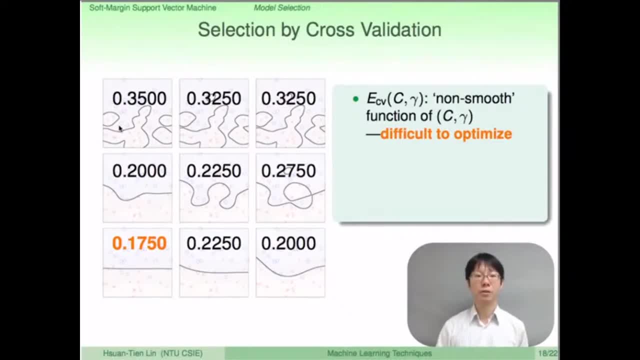 但它不是一个很容易的平滑函数 能够让你对C跟γ说最佳化, 所以通常你只能透过送进去 几个不同的C跟γ值. 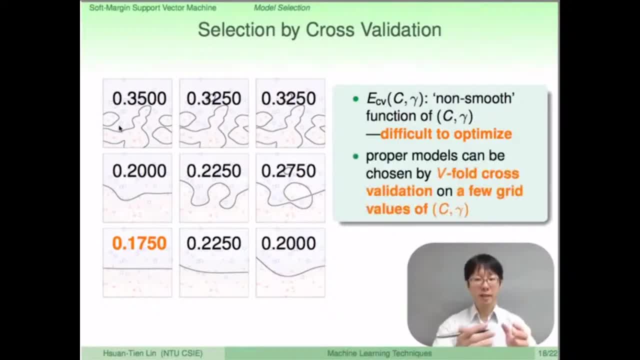 看看哪一个比较好. 其实我们这里做的事情就是: 比如说我把C跟γ九宫格上 好 每一个C跟γ的组合. 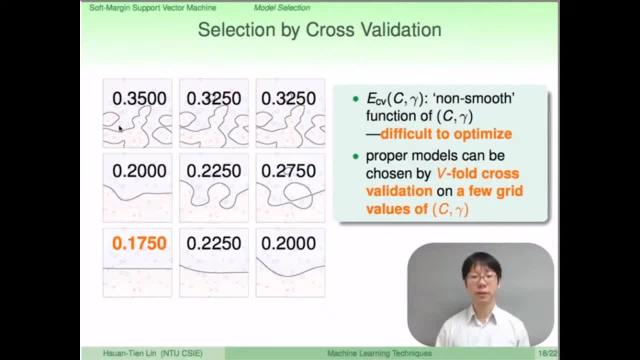 然后来算一算 然后看一看哪一个比较好. 我做了这个v4的Cross Validation. 我们之前在机器学习机时里面 已经讲过这样的工具了. 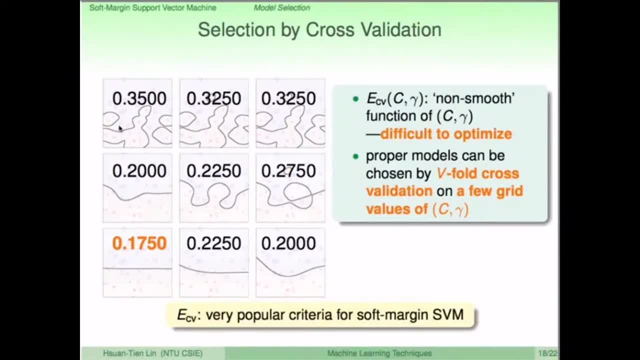 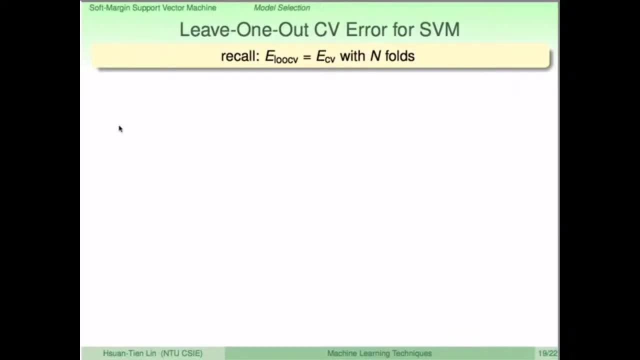 好所以这是Cross Validation. 对SPM来说这是一个非常常用的方式 用来选择适当的参数. 好如果Cross Validation推到极限的话. 大家记得我们那时候说: 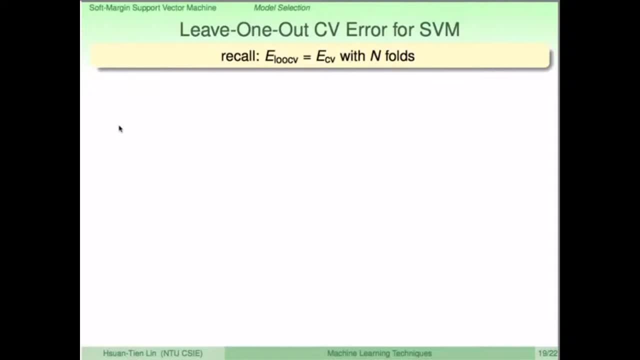 Cross Validation你说你把资料切成五块十块. 如果你说你今天有一百笔资料, 你把资料切成一百块来做Cross Validation. 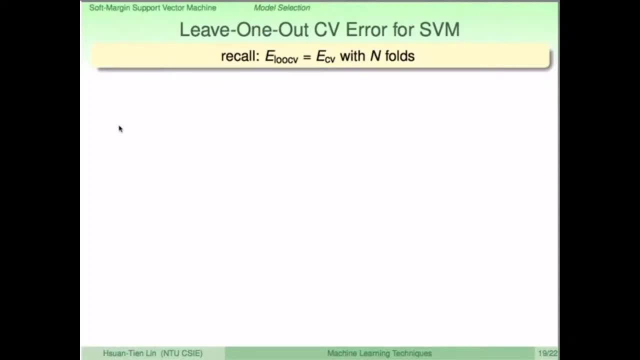 那我们那时候说: 它有一个推动的方式. 它有一个特殊的名字叫做Leave One Out. 每次留一笔做Validation, 其他来做Training的这种Cross Validation的方式. 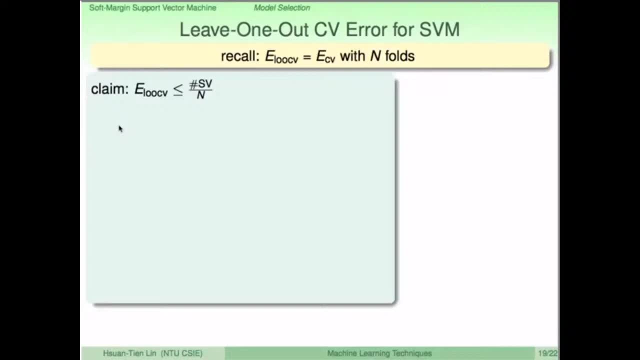 好那Leave One Out在SPM上 有一个很有趣的结果. 我们这边跟大家分享一下说, SPM的Leave One Out, Cross Validation Error 跟Support Vector的数量. 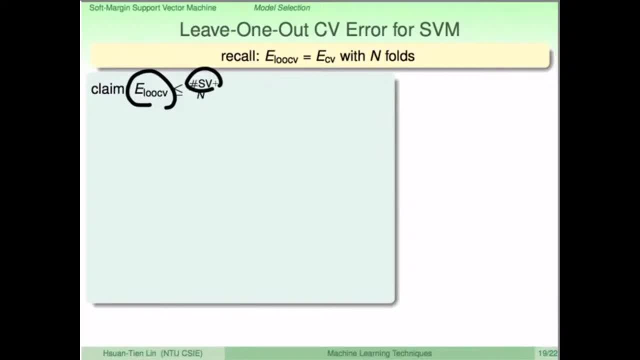 其实是有关系的. 我们可以证明 Leave One Out的Cross Validation Error 会小于等于Support Vector的比例. 好例如说你有一万笔资料, 里面有一百个是Support Vector. 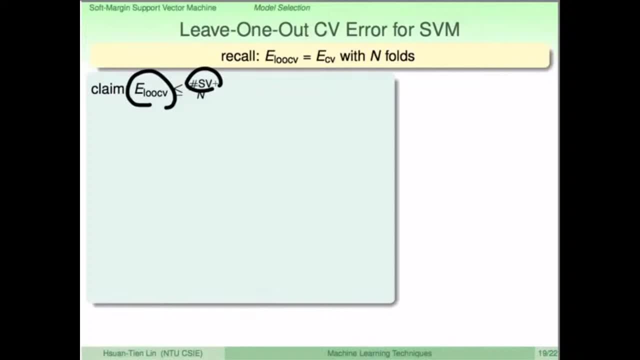 那我可以说你的Leave One Out Cross Validation Error 会小于Support Vector的比例 一百除以一万也就是百分之一. 好那这个要怎么样子证明呢? 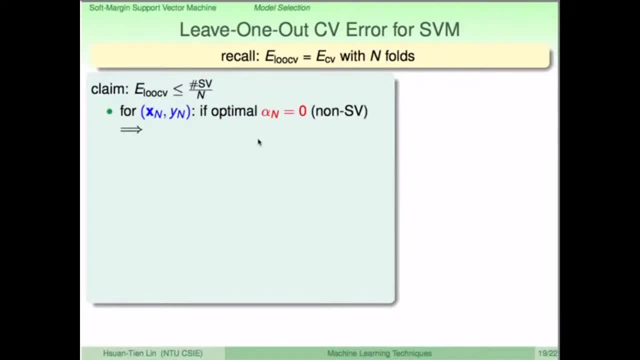 我们可以想: 如果你今天已经有一万个点, 好然后你解完这个SPM的问题以后, 对于第一万个点, 刚好它的最好的alpha是等于零的. 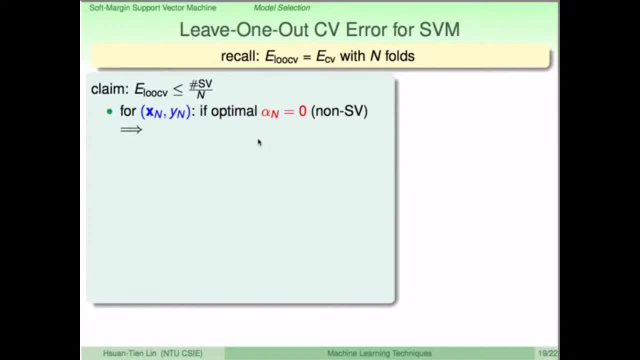 你解出一组最佳解: 那个在第一万个点上. 它的alpha是等于零. 我们的宣称是这样: 你把前面9999个alpha送进去. 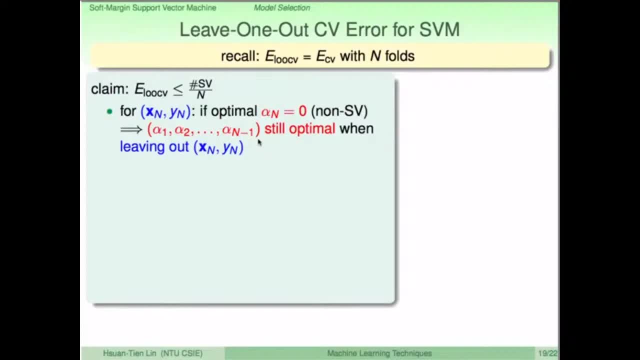 把最后第一万笔资料踢掉, 把前面9999个alpha送进去. SPM的问题 只用9999个点的时候 这一组alpha 还是会是最佳解. 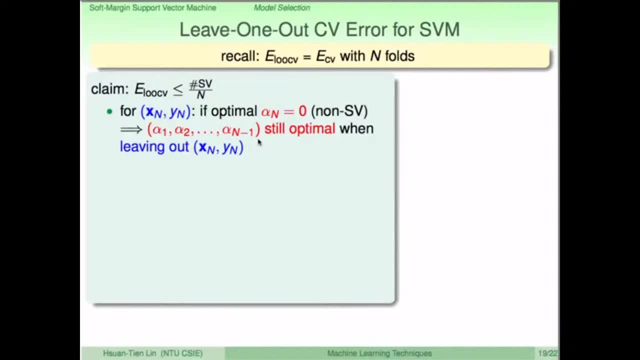 为什么? 因为如果这一组alpha不是最佳解, 那就表示有一组更好的, 9999个alpha有一组更好的, 一组更好. 那你说我把这个点加回去. 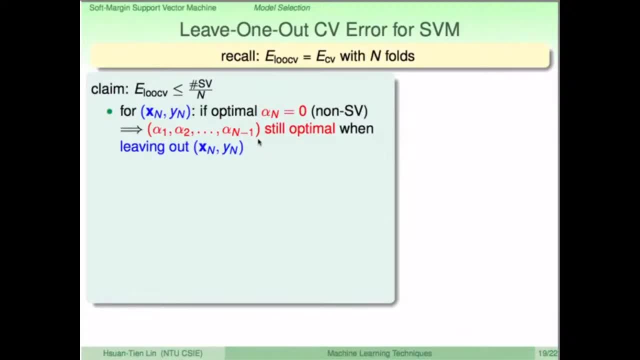 那就又有一组更好的. 这矛盾嘛. 所以呢, 既然你原来一万个的时候是最佳解, 那么说进去9999个的时候还是最佳解. 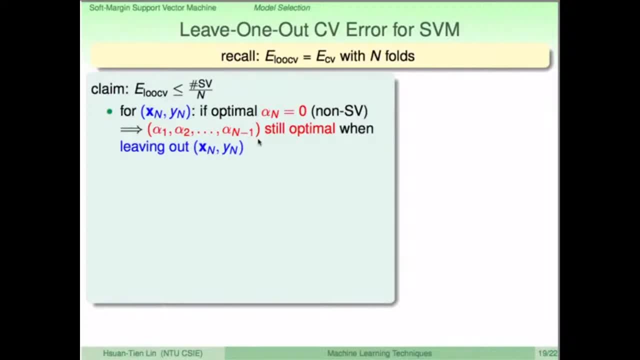 因为你剩下那个根本就没有用. 那个就是alpha零的. 记得这跟我们之前在Hard Margin的时候说: 我如果把那个Non-Support Vector拿掉, 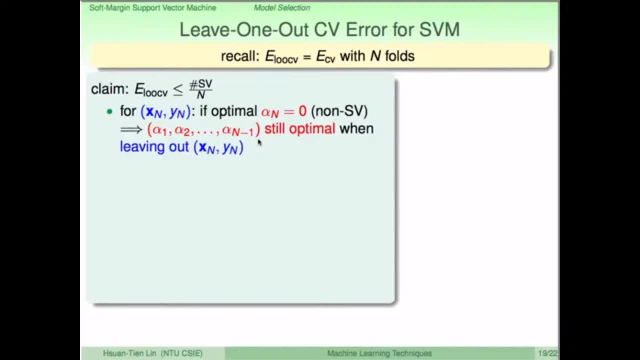 对于我找到胖胖的连接 一点影响都没有. 那这是它的 数学问题. 数学上的解释说: 从最佳化的角度来说, 你的G跟你的G-拿掉了一个点以后的结果. 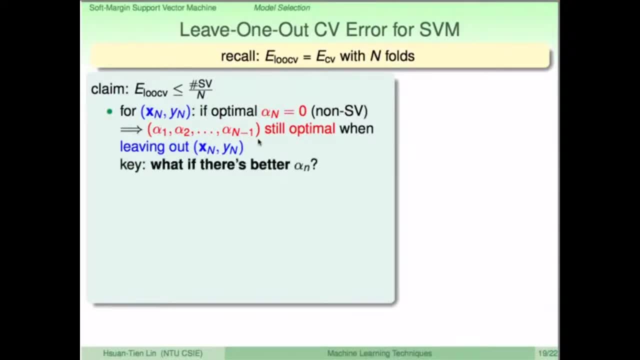 会是一样的 好. 所以我们刚才阐述了说: 不可能有更好的alpha, 这边9999个alpha一定是最好的 那所以我们就可以说什么. 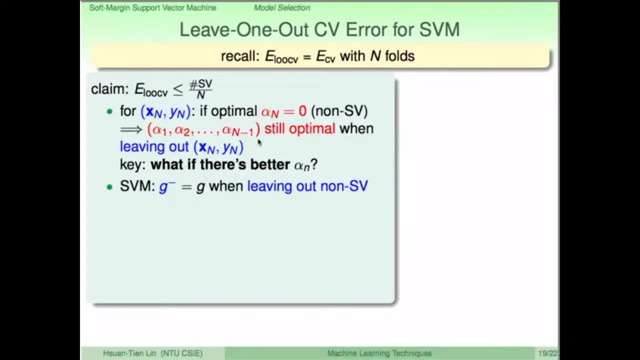 这个时候, 如果今天是一个Non-Support Vector, G-跟G是一样的 那么今天Non-Support Vector上面, 那个点上面的小小的error 就会是什么. 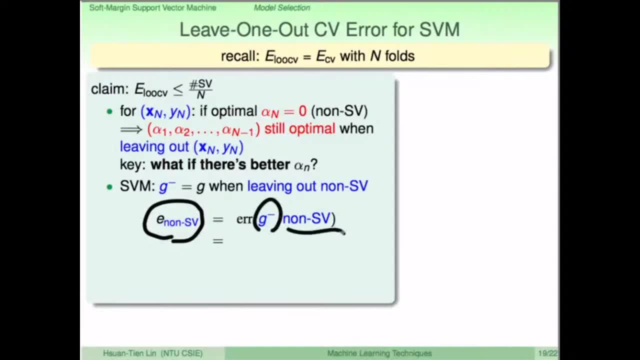 我们原来应该要算G-跟它这个点上面的error 那对这个点来说 G-跟G是一样的, 但是这个点来说, 所以就是G-跟它的error. 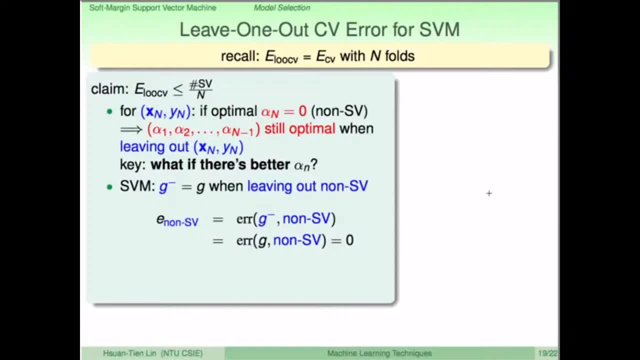 G-跟它的error是什么 G在G上面? 它不是一个Support Vector. 不是一个Support Vector就表示 它离边界还远的 领度就在抗抗边界上. 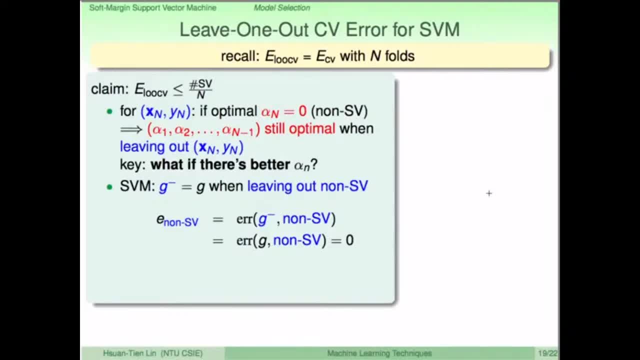 所以它的error一定是0 Non-Support Vector. 在Leave-1-Out上面的贡献一定是0 Support Vector呢, 在Leave-1-Out上面贡献 可能是0可能是1. 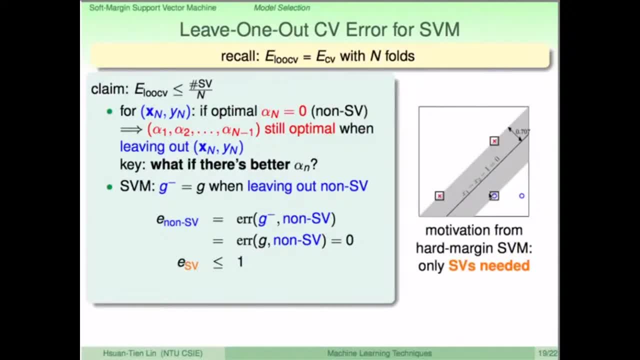 最多最多就是1嘛. 这样的结果平均起来 我们就得到一个非常有名的棒的. 这个有名的棒的就是 SVN的Leave-1-Out Cross-Validation Error. 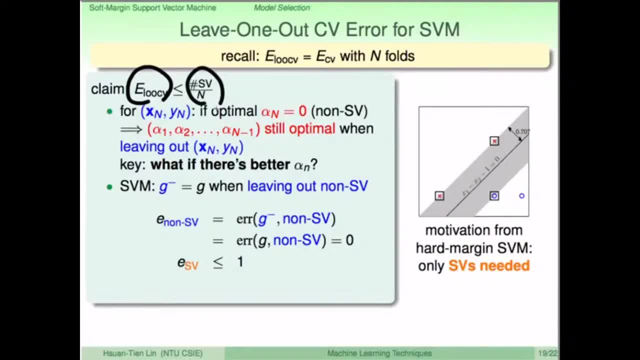 会小于等于Support Vector的比例. 这其实回应了 我们之前在Hard Margin看到的事情说 我们把Non-Support Vector移掉 对于我们抗抗边界一点影响都没有. 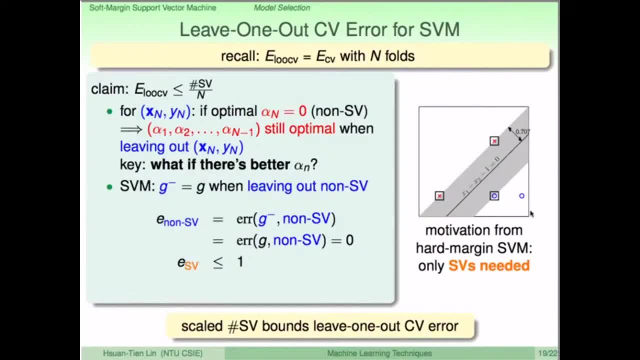 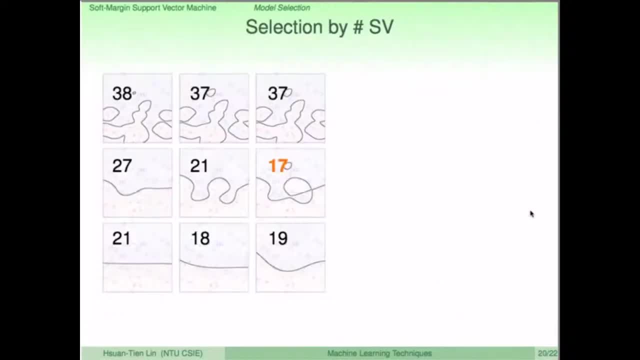 好所以Scale的 这个就是说放出过的Support Vector数量 跟Cross-Validation 跟Leave-1-Out Cross-Validation的error是有关系的. 所以我们也可以用这个来做模型的选择. 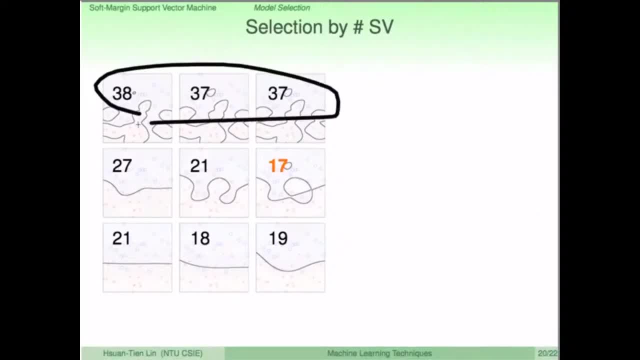 大家看到说 上面这三个比较糟糕的例子. Support Vector的数量 我这边列出来 其实是很多的. 那下面这些比较简单的例子: 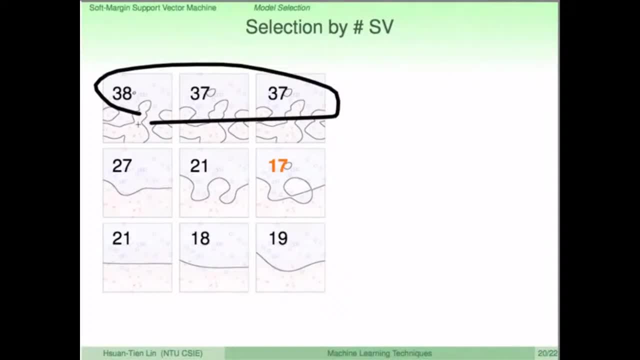 Support Vector的数量 可能是相对比较少的, 所以你可以拿它来做选择, 不过当然这边我们要给一个警告: Support Vector的数量 除了它不是一个平滑函数以外. 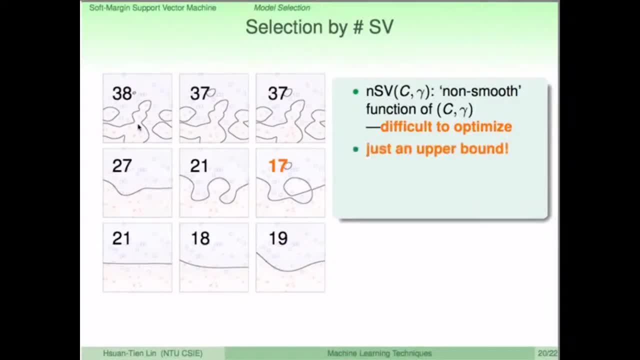 另外有一件事情是 它只是个上限. 我们不知道实际的Leave-1-Out Cross-Validation是多少. 我们只能从Support Vector的数量 估计一个上限而已. 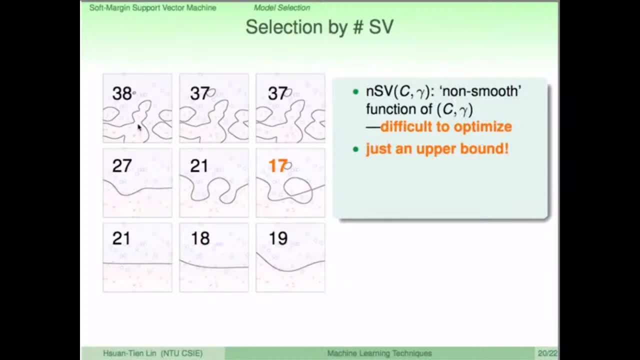 因为是上限, 所以你对它做最佳化. 可能你只是把上限做到最好 或代表你把真正的值做到最好. 好所以呢, 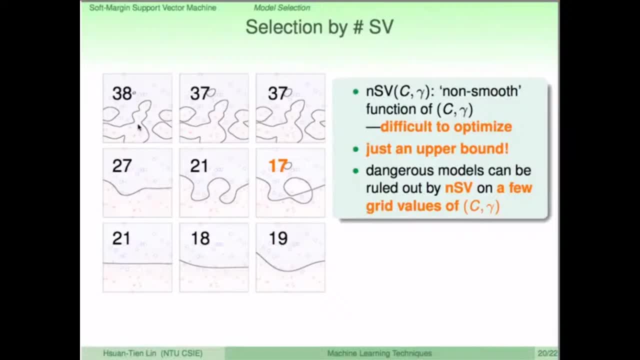 这个Support Vector的数量. 通常拿来做什么? 通常拿来排除一些比较危险的 像上面这些Support Vector的数量很大, 这些 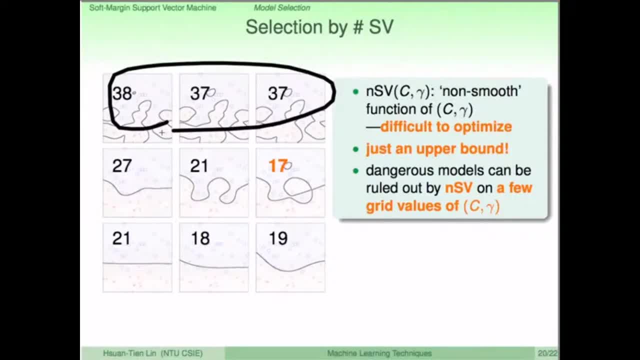 我们就觉得有危险. 所以你做一个SVN. 看Support Vector的数量. 如果很大, 可能表示你的这个模型不是太好. OK, 然后排除了这些以后. 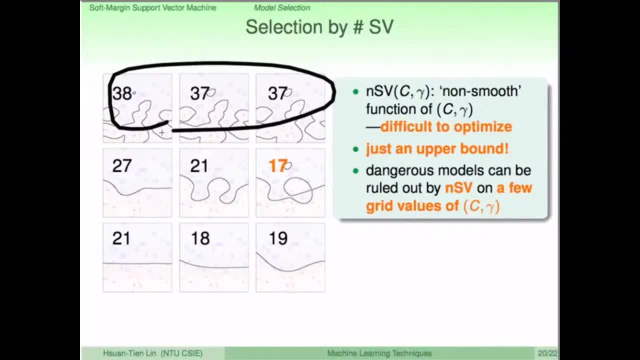 你可以在其他上面进一步做Cross-Validation 来选择一个你觉得更适合的参数. 所以这是Support Vector的数量. 通常可以用来做SVN的. 我们叫Safety Check. 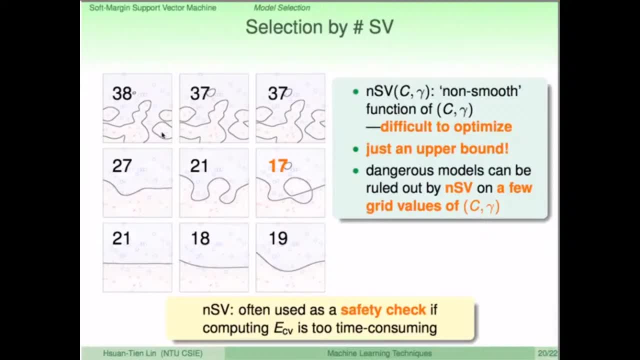 安全检查. 看看你做出来的这个GSVN 到底合理还是不合理, 特别是如果算Cross-Validation 真正算Cross-Validation, 有时候比较花时间的时候. 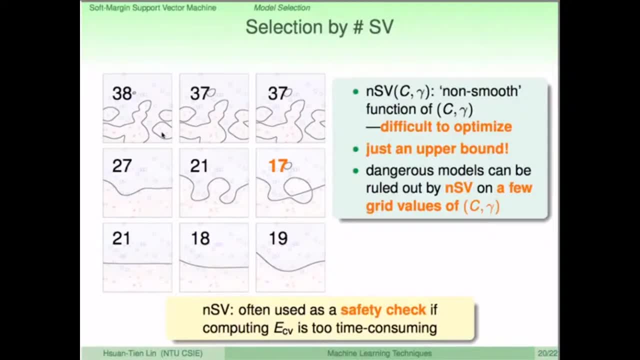 Leave-1-Out. 反正这个你Training做完, 你就得到这个SVN的Support Vector的上限了. 所以你会比较神秘气一点 好, 所以讲到这边. 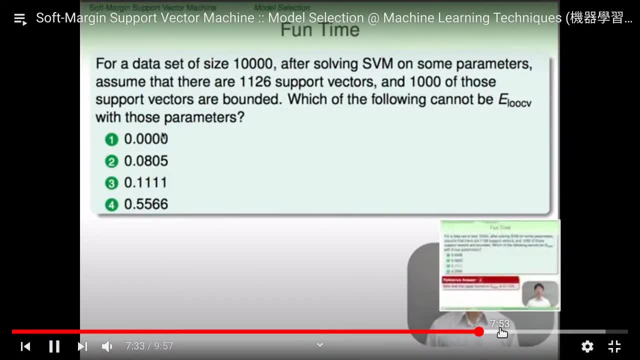 给大家最后一个练习说: 一样我们的资料是1万笔, 然后一样我们有1100个是0.126. 那么如果能够选到正确选项是4. 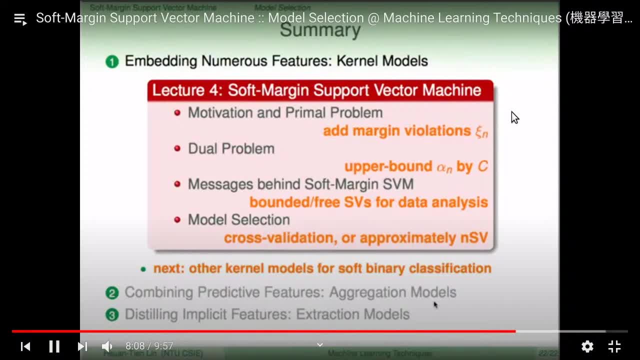 好, 那总结一下: 我们这边讲到了Soft Margin的SVN 一个SVN的新的形式. 实际上这是最常用的一个形式. 那我们的出发点是: 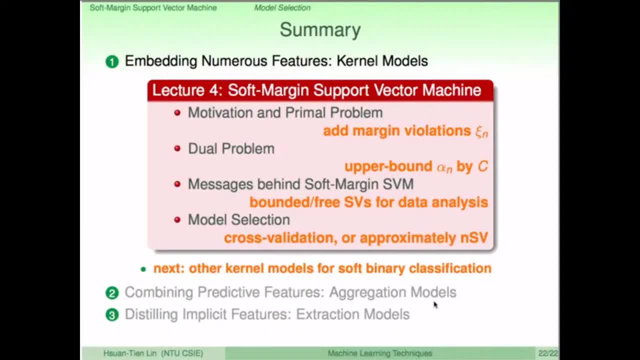 我们希望不要坚持, 一定要把所有的圈圈材料都分开. 所以我们加上 说我们违反Margin的这个大小是多少, 然后把它当做一个惩罚项. 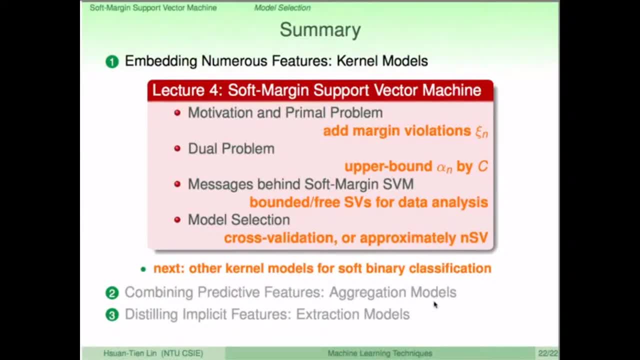 然后推导说它也是个QP, 所以我们可以推导它的QP的队友问题. 然后发现说它跟Hard Margin几乎一样, 只是你的R8n. 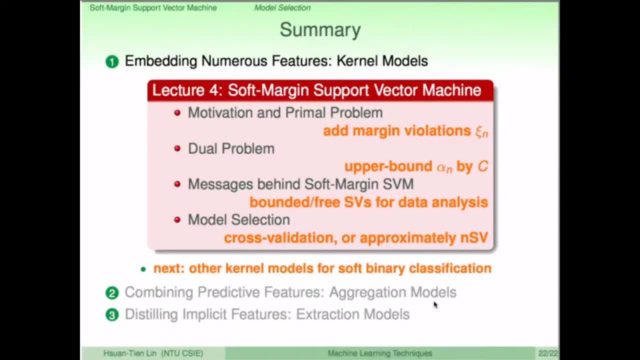 现在上面有个C压在上面而已. 它告诉我们的讯息就是: 透过SVN 我们可以把资料分成三种. 不是Support Vector不重要的. 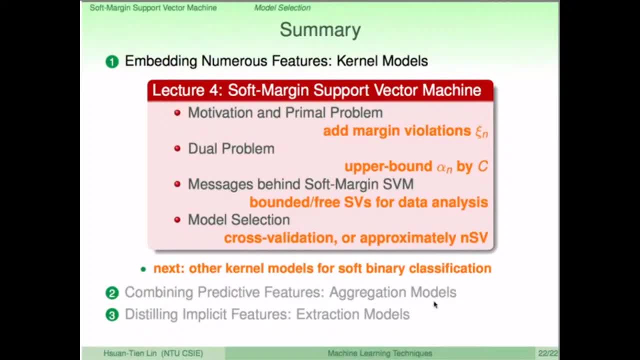 然后在边界上的Free Support Vector 然后再来如果是Bonded, 如果已经到那个C的 这是可能违反了胖胖边界的这些Support Vector. 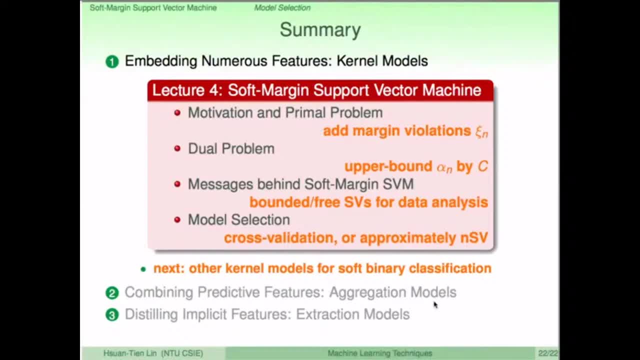 对于我们的SVN, 我们做资料的分析非常的有用. 然后另外我们提到 Model Selection是SVN里面重要的问题. 那可以使用Validation, Cross-Validation. 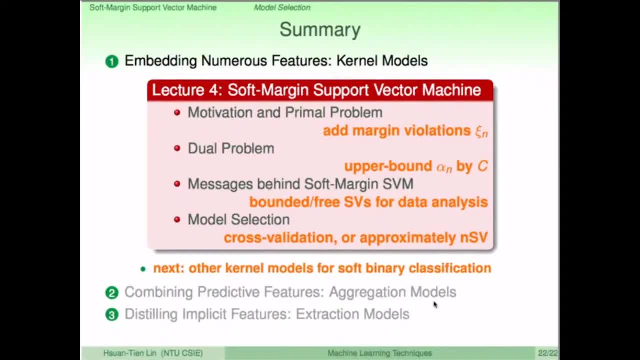 这样的工具, 那也可以用Number of Supports Vector 来当做一个安全的检查 好所以这是我们讲过. 前面是讲这是最流行的. 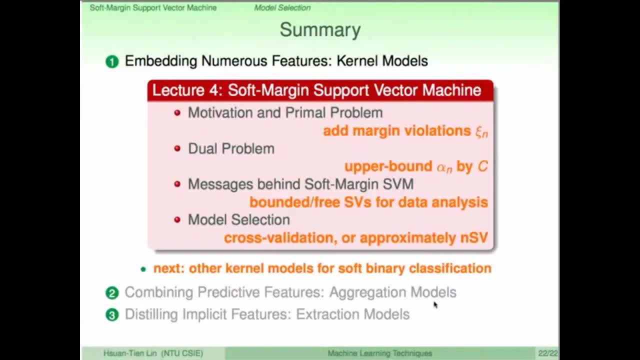 这个Soft Margin SVN的完整的介绍: 从Hard Margin然后到这个Duo到Kernel 一路推到Soft Margin 那所以这些都是在Binary Calculation上. 我们下一讲要讲的是. 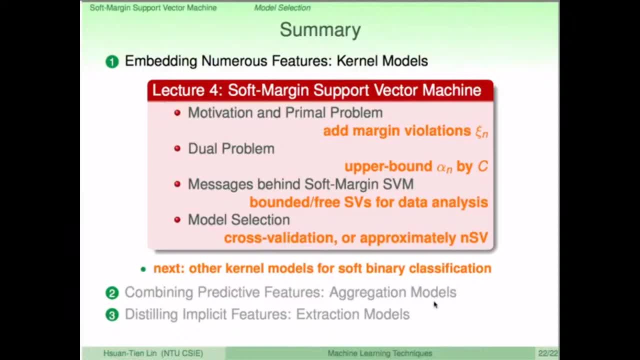 我们怎么把Base SVN这样的机制 延伸到做一些不同的问题. 那欢迎大家 下一次回来. 谢谢 感谢. 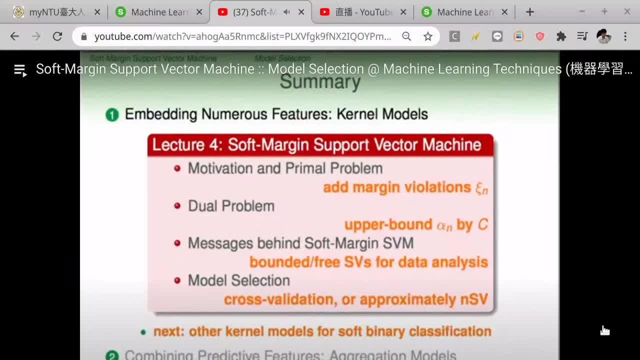 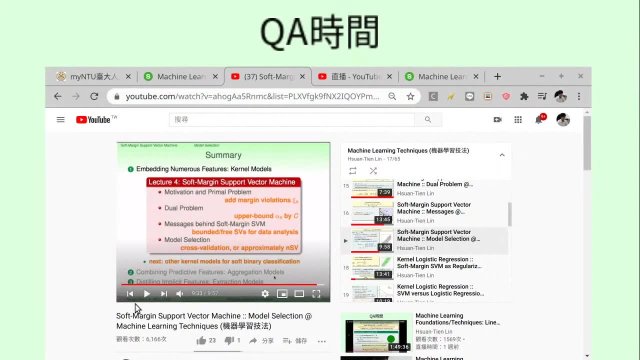 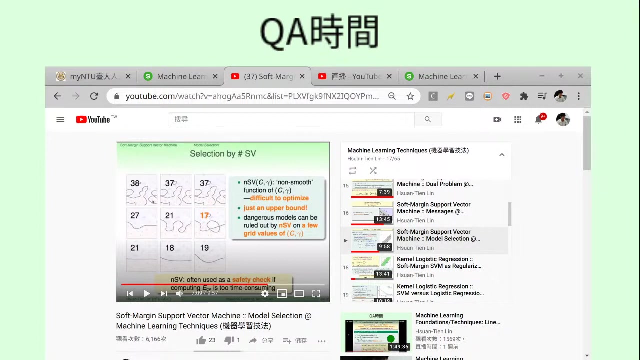 好那我们结束了这个Soft Margin的部分. 那最后给大家其实是 补充着一个所谓的 用Number of Supports Vector 来表示的Leave One Out的Bound. 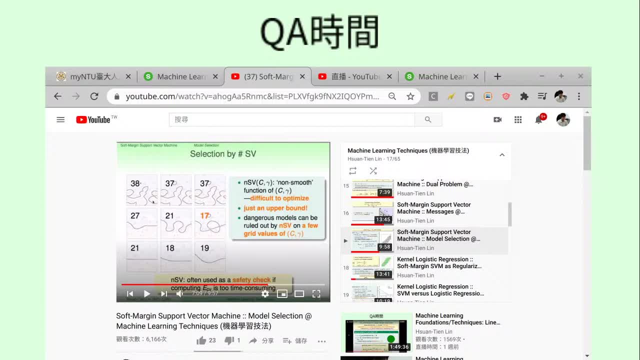 我知道大家在, 比如说在这个SVN里面, 如果你有修基石的同学, 你现在在写作业词的话 有一些Leave One Out的题目. 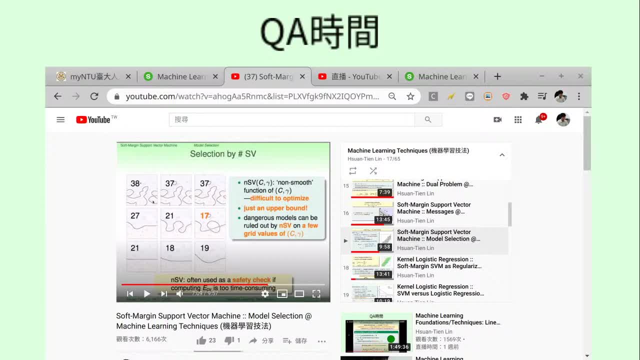 可能还没有搞得很清楚的. 那这边刚好有个机会 让大家再想象一下 所谓Leave One Out的Process. 怎么一回事? 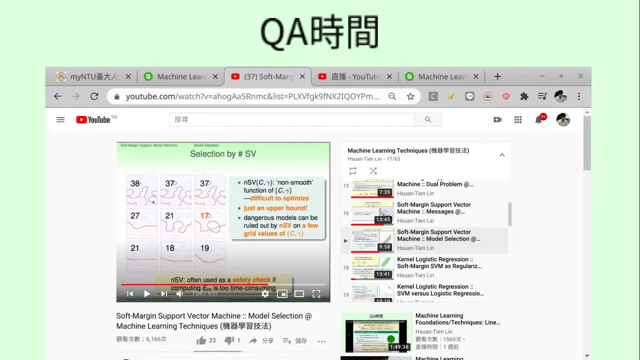 每次留下一个点, 然后用其他的点去做Training, 然后用那一个点做Validation. 重复这个步骤在每一个点上 然后再把结果平均起来. 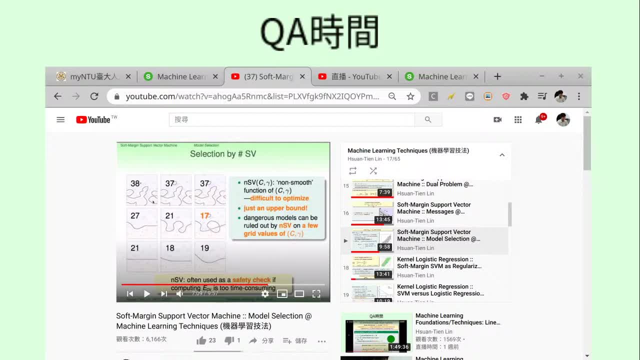 那当然一般来说 做Leave One Out是非常Time Consuming的事情, 但是Leave One Out在 我们在 基石那边我们推导的 这个理论上面是有一些些好处. 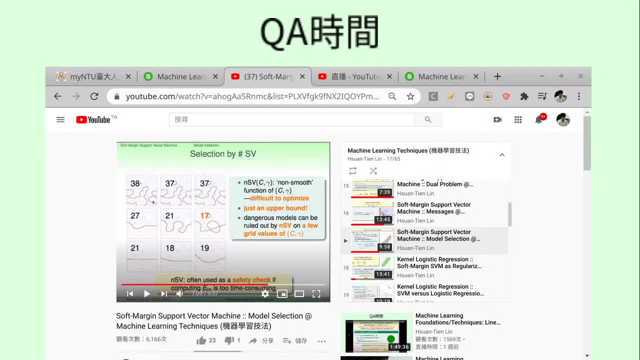 有一些些保证的 那所以这边呢 等于是从另外一个角度说: 那有没有那个你做完Training, 你就算出Leave One Out的这个Error. 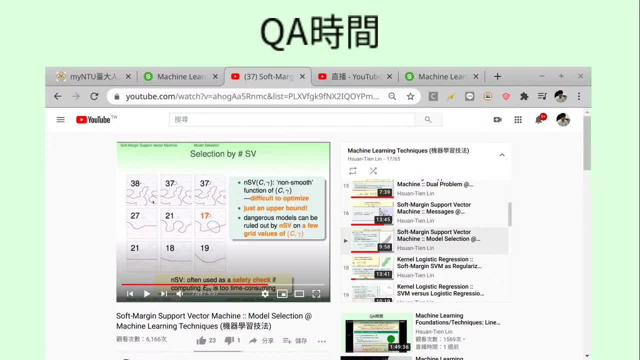 而不用真的做N次, 做那么多次. 那Supports Vector Machine 是其中一个这样的模型. 说好你其实不用做Leave One Out, 你只要把你的东西. 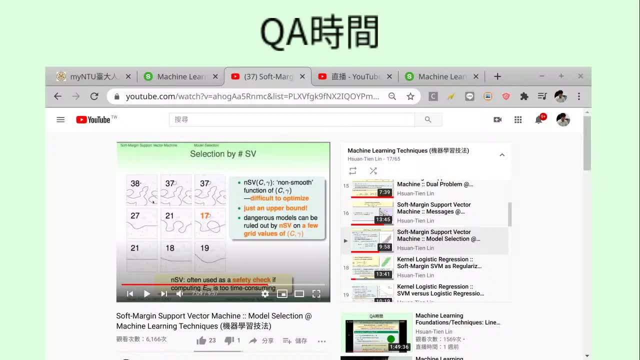 按照你的参数丢下去: 1000米之较1000米之较 丢下去. 做完以后你Read Out 那1000米之较上面Supports Vector的数量. 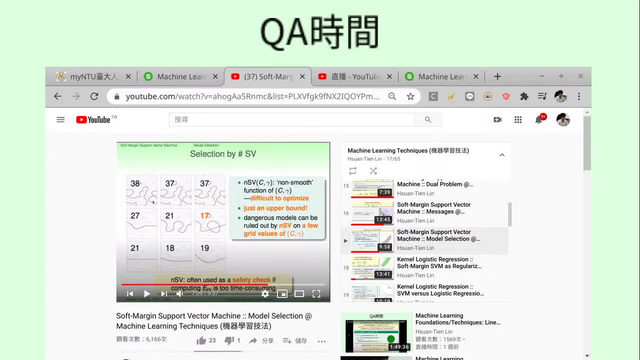 你就可以有个估计, 有个想像, 说到底我的Leave One Out Error是怎么样? 那应该是说 我们刚才说你用可以用来排除一些不好的情形. 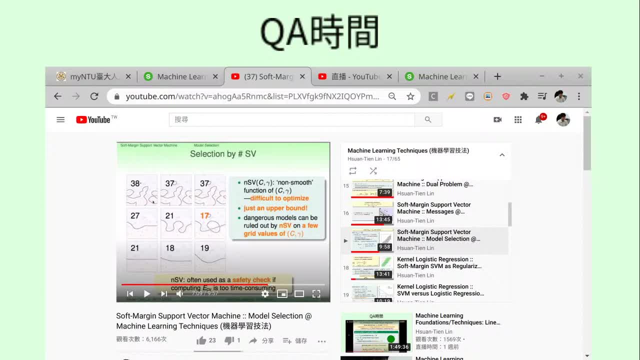 实际上我们比较常用这个Supports Vector数量 来做所谓的Sanity Check, 也就是说你Chain完之后 这个SVN到底Chain是好的还是不好的. 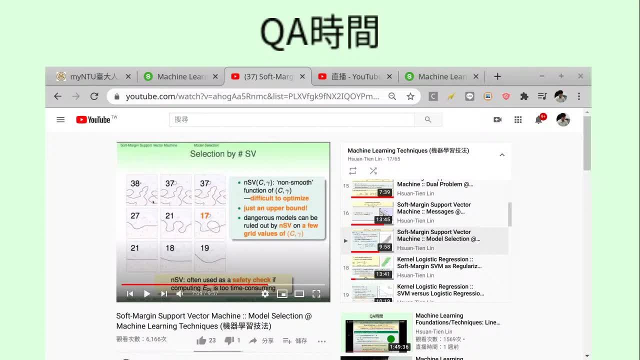 非常Typical的SVN你丢下去的话. 你可能会想像它留下来的资料量, 它的Supports, Vector数量: 可能是一层可能是两层. 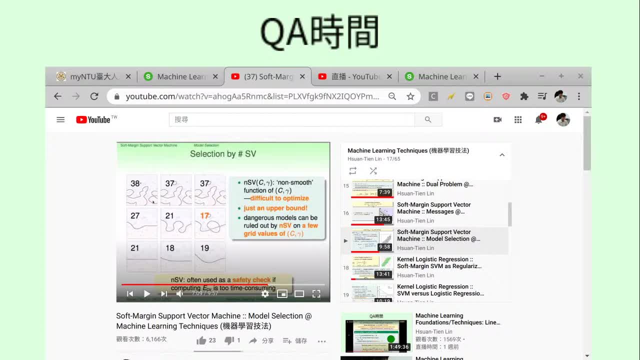 如果你超过五层的Supports Vector数量的话 可能就会怪怪的 因为感觉你的Supports Vector Machine 就把超过一半的资料通通都记起来了. 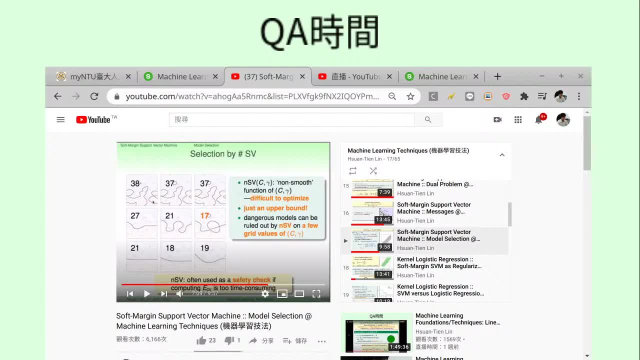 所以如果今天是20%的Supports Vector, 那还蛮正常的. 它留下一些边界的, 留下一些Margin Violation的. 但是如果今天是你有八成资料都是Supports Vector的话. 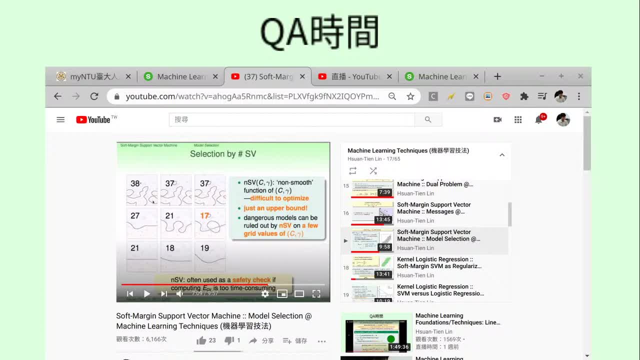 那可能不太好. 这就表示你的参数下的不是很好. 我们看过一些很Typical的情形说: 什么时候很多Supports Vector? 例如说我们之前看到高悬很尖的时候. 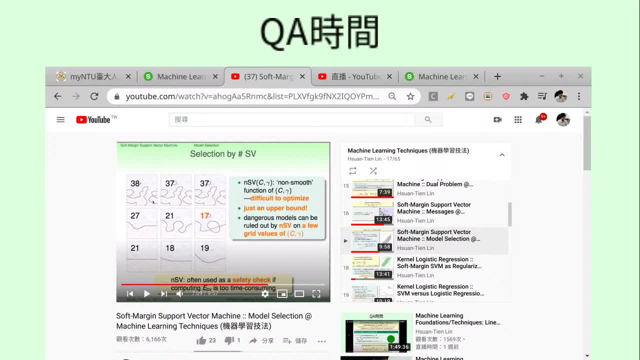 伽马很大高悬很尖 那些尖尖的高悬. 你看到每一个小岛通通都记起来Supports Vector. 所以你有一半左右的Supports Vector. 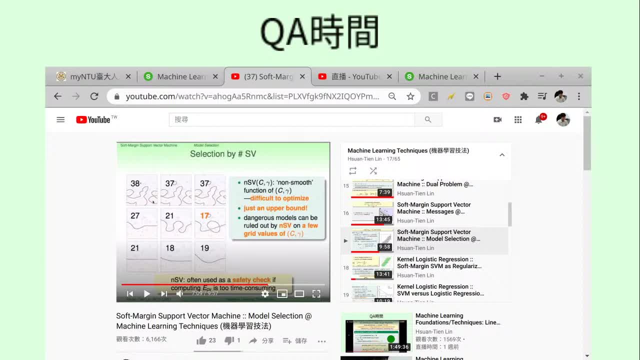 或者是你今天C设的很小, 也就是你看似边界很宽, 但是你需要把每一个违反边界的点 通通都记起来你的Supports Vector很多. 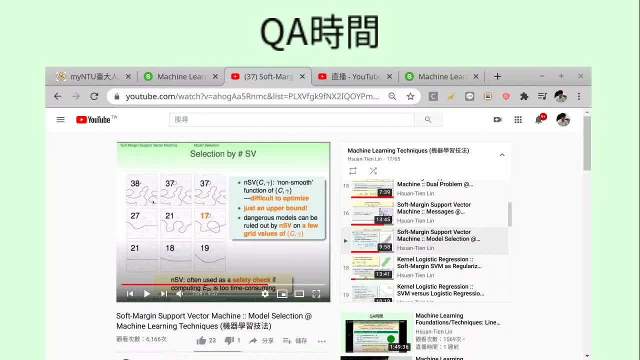 那这些都严重的Supports Vector 也许不是太好的情形. 所以SVN这个东西我们叫Supports Vector Bound, 并不是说我们真的可以由这个Bound去Optimize什么东西. 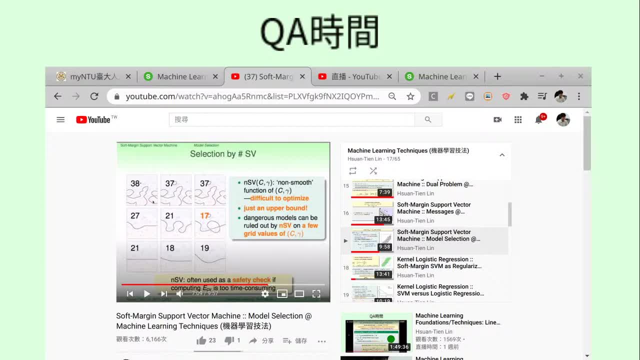 但是如果你做完一个SVN以后, 好习惯其实是自己做一点 这个Percent of Supports Vector的检查, 说到底是不是在我们觉得相对合理的Range. 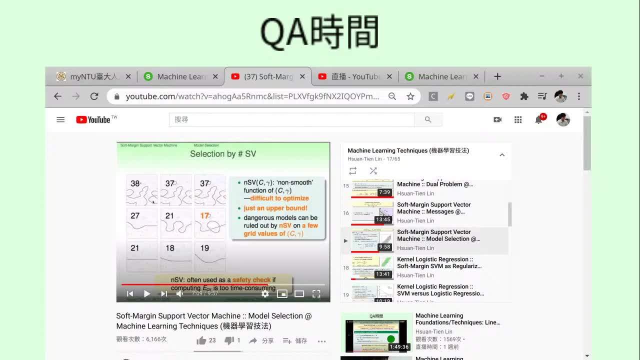 好所以这是SVN然后跟他的Model Selection的部分. 实务上来说其实你最常用也不是Supports Vector Bound, 也不是Leave-1-Out, 就是好好的做个Cross-validation. 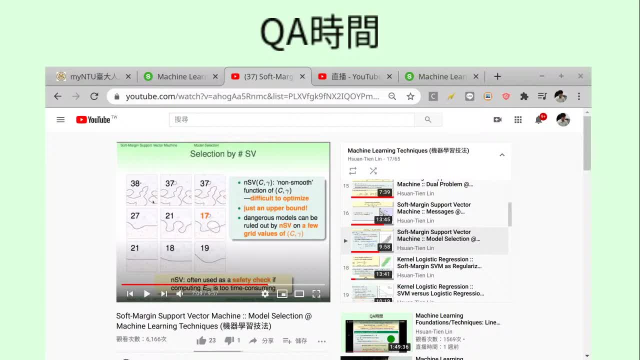 有点像大家在作业室里面做的那个样子. 作业室的时候大家是用Logistic Regression在做 SVN的世界一样. 如果你今天是高线SVN. 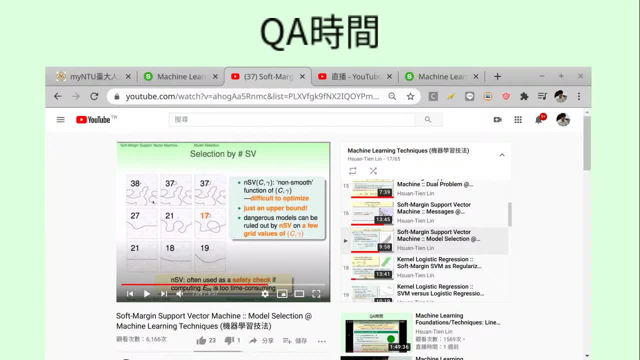 不同的C不同的Gamma, 然后做个Cross-validation 估计一下在C跟Gamma上面的Performance怎么样. 那就是好的选择参数的方式. 好有没有问题. 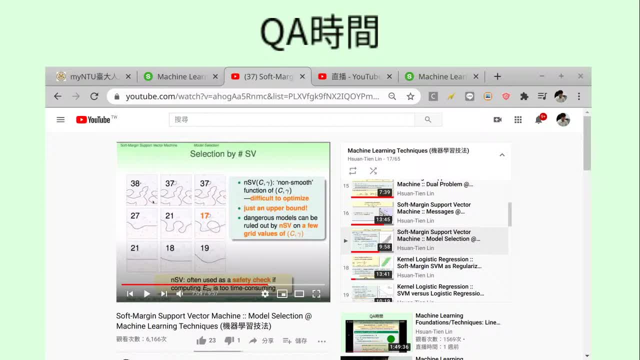 请说 OK好同学问题是说Leave-1-Out Error的这个估计方式 OK可不可以是我们就先Train一个Full Model OK然后那每一次 拔掉一笔资料的时候? 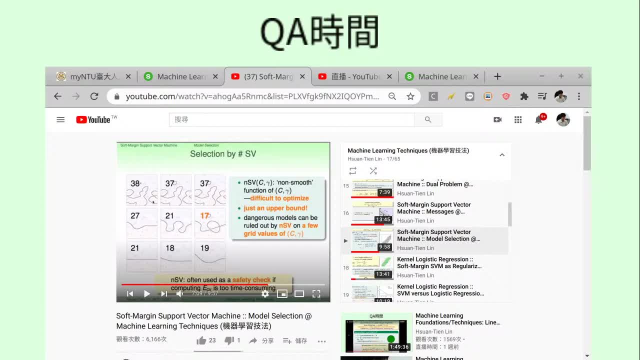 我们估计说拔掉这笔资料最多的影响有多少. OK然后那于是做完一个Full Model以后 我们就可以得到Leave-1-Out Error是多少? 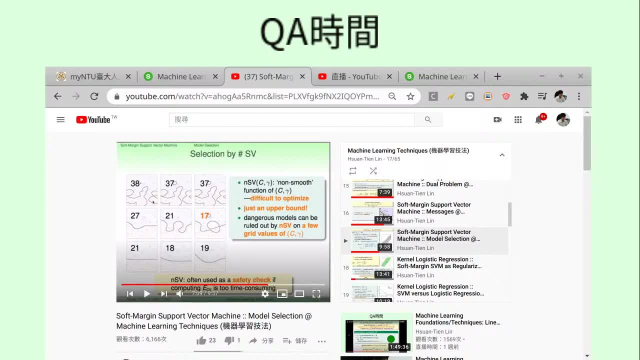 那实际上我们导致SVN的Bound就是这样做 对不对他说来我拔掉资料, 你拔掉资料如果在这个完整的Hypothesis里面 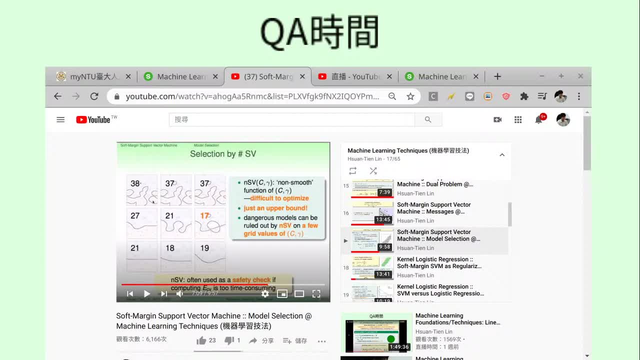 是个Supports Vector, 那他最多就犯1的错误. 如果拔掉资料是Non-Supports Vector, 那么拔掉它也没有关系. OK它本来就是垄圆. 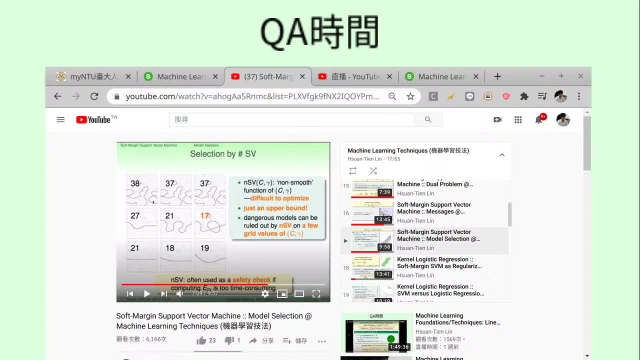 那所以呢这个有了这样的. 然后我们推导出这个用Supports Vector的比例 OK来做的一个Bound. 那所以SVN是一个这样的例子: 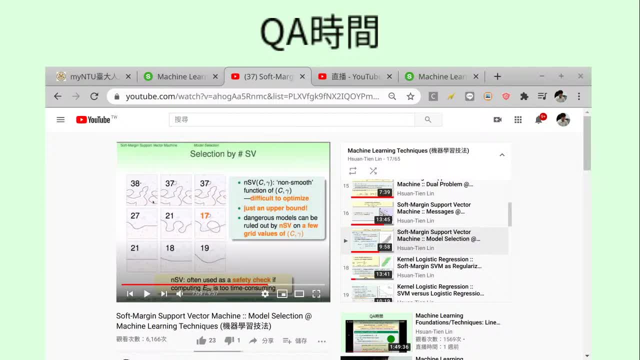 你如果去看的话Linear Regression, OK你可以做类似的事情. OK, Roughly来说, 你Train好一个Linear Regression的这个Hypothesis, 或者在Train的过程中 你从去分析Linear Regression的矩阵里面的那些值. 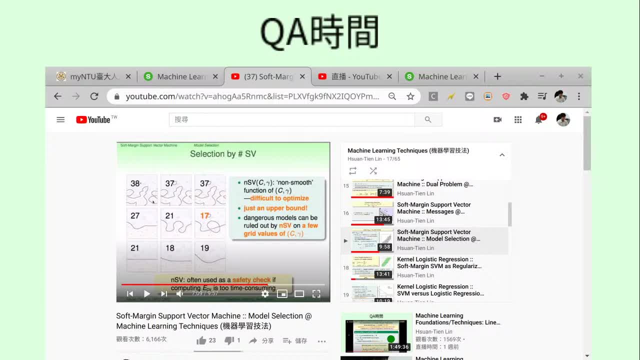 OK然后你可以算出来它的Leave-1-Out Error是多少, 但是这毕竟大概就是比较特别的 方法OK你可以做这件事情, 但是也有很多的方法. 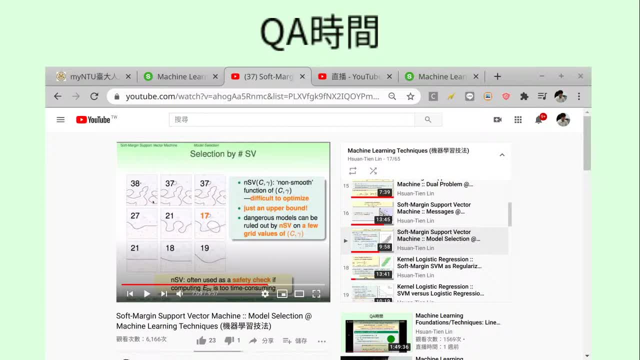 你的确很难从一个Full Model就去估算, 或你可能会估出一些很不准的东西 或很高估的东西. 其实SVN这个东西也没有真的很准啦. 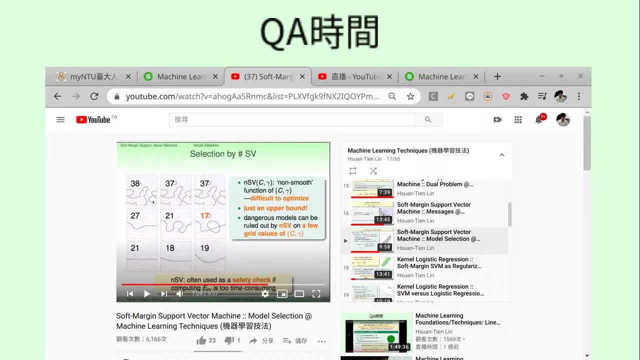 OK因为它是说: 你看我们刚才在Supports Vector的时候 它说Supports Vector反而Error就是0. Supports Vector的时候可能是1可能是0, 我们不知道. 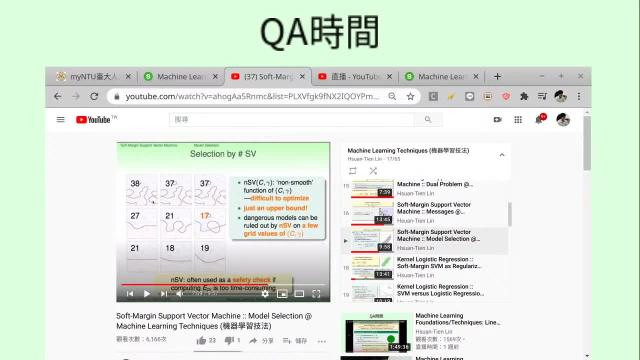 那就先高估一下先算1吧. OK所以实际上它的Leave-1-Out Error 应该要比OK我们刚才那样 估计的应该是要在小一些. 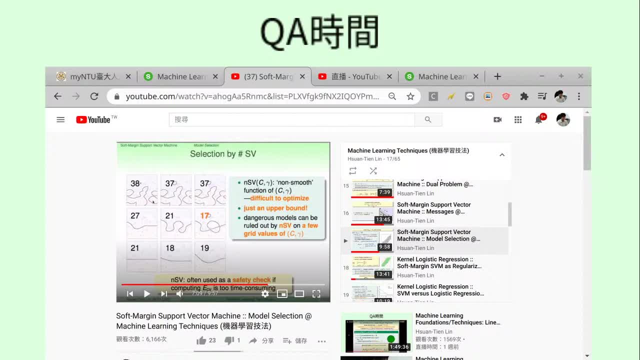 但是SVN这个宽松不算太宽松. 意思是说马马虎虎堪用, 但是有很多模型的话 你真的要去估计. 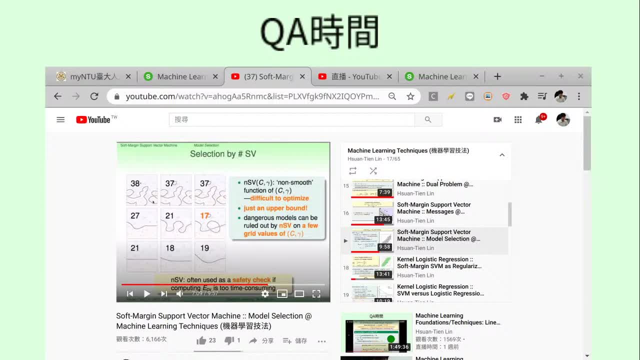 这个Worst Case好像很容易. 你在你Leave-1-Out的那个点上会犯Error, 然后你就会得到一个很宽松的估计. 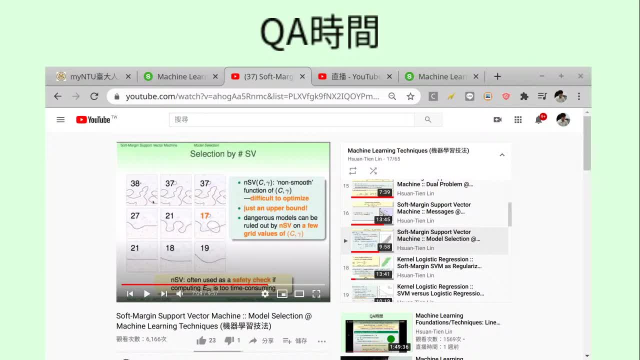 然后太宽松可能就不一定会有用 这样子所以这是有关Leave-1-Out的部分 就是其实实务上来说 大家都很想得到估计. 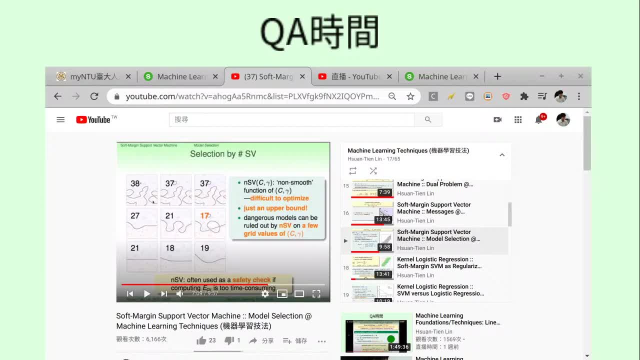 实际上SVN的这个Bound 还有很多版本的Refinement 说怎么样可以做得更好等等等等的, 但是其实不太容易. 意思是说不太容易的意思是: 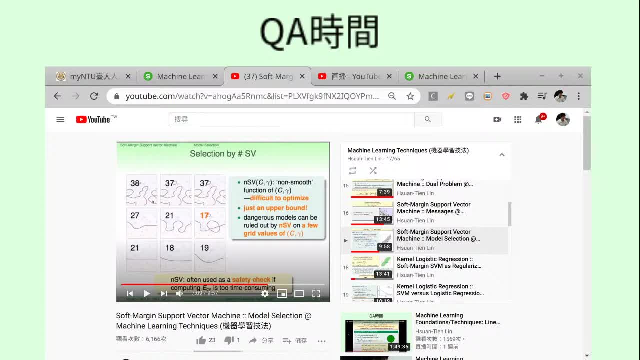 其实到最后大家就乖乖的去做, 例如说5-fold的Cross-validation 或What-Ever那一类的 在参数选择上搞不好比Leave-1-Out 还要有用一些. 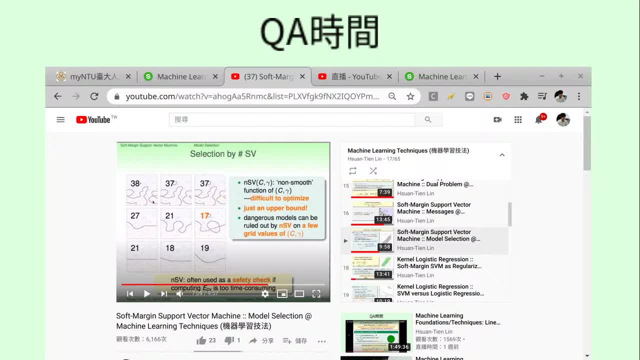 这是我们实务上看到的事情. 也补充一下: 其实另外一个Leave-1-Out没有用的地方是: 就算你花了很大的力气. 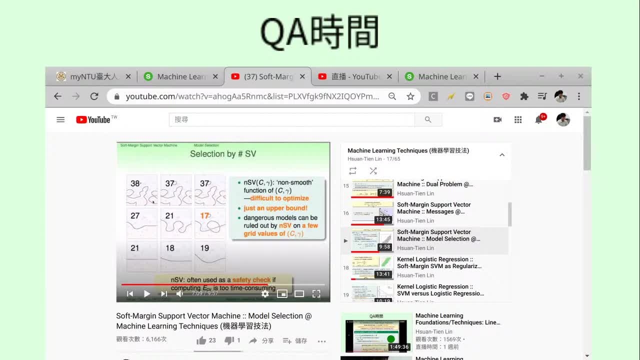 把那个真正的Leave-1-Out Error算出来了. 那个Leave-1-Out Error还蛮 某种程度上它的Variancy还蛮大的, 意思是说它毕竟还是一堆. 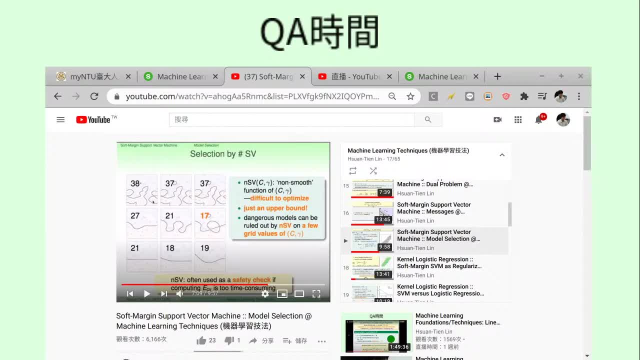 跳动很大的东西Average起来的结果 然后所以它的Variancy还蛮大的. 那有一些些研究在说 因为它的Variancy太大. 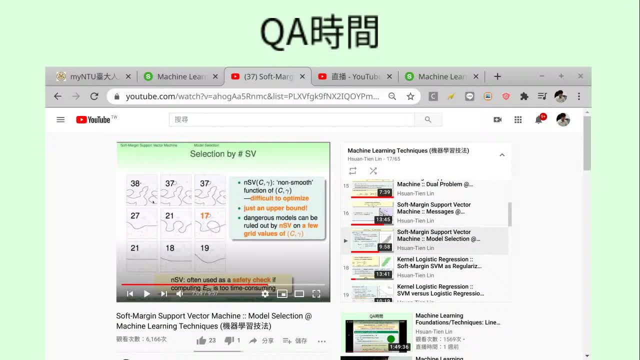 所以你真的要选择参数的时候. 比如说你现在有A参数跟B参数 然后你要选哪个好. 也许平均来看A比B好. 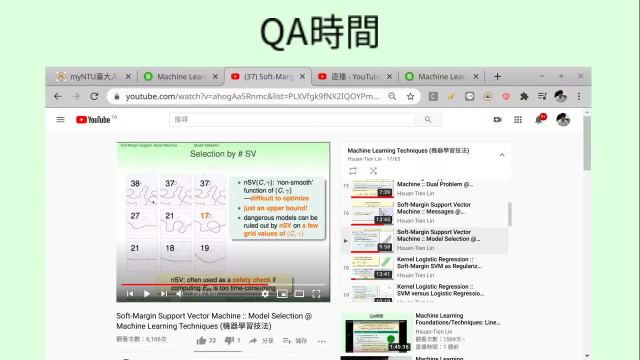 可是把Variancy加进去以后 到底会不会看到A比B好等等. 其实不太一定. 所以Variancy太大的时候 有时候在参数选择上有另外一层的困难. 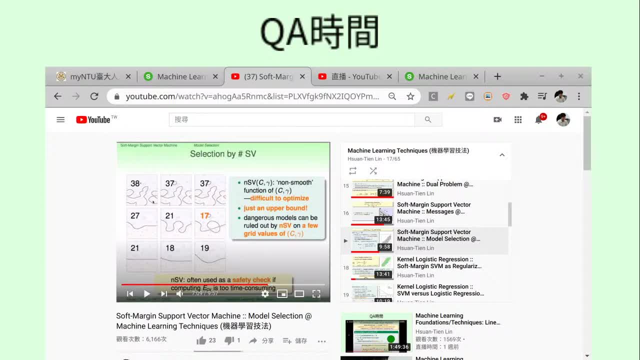 相对来说5-fold Cross-validation 可能Variancy没有那么大, 所以在参数选择上还比较好用 或还被一些人觉得比较好用一些. 那这是我们观察到的事情. 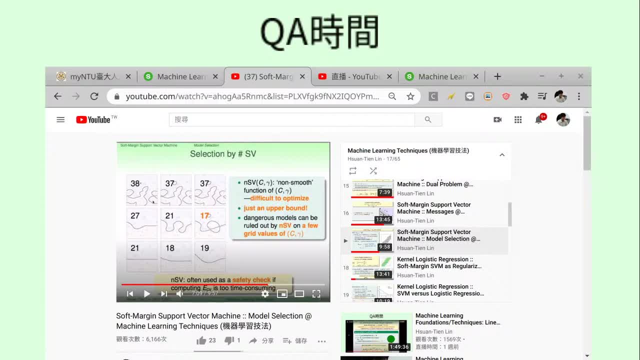 OK好还有什么问题吗? 请说 OK所以同学问题是说 我们本来在下一段会教, 其实我们Kernel method还有两家, 然后我们再来会有Aggregation. 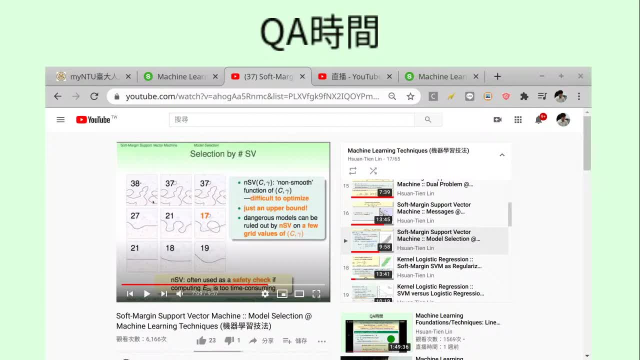 那Aggregation完才是Neural Network 或这个Feature Extraction Model. 那为什么要先教Neural Network? 那就像我课程开始的时候说的, 因为我们想要先教推荐系统. 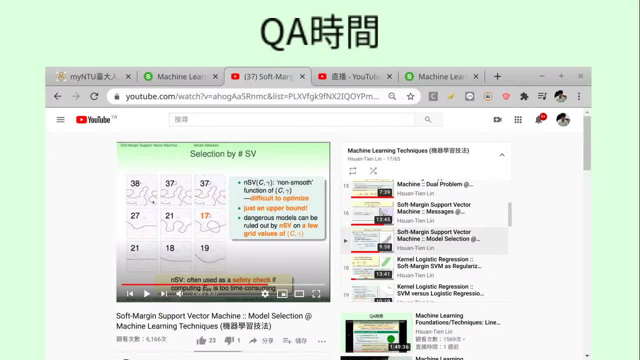 然后想要教推荐系统的话 在我们原来课程设计里面 推荐系统有个Pre-requisite: 是我们这种Neural Network Model发展出来的 然后所以我们就把它拉到前面来教. 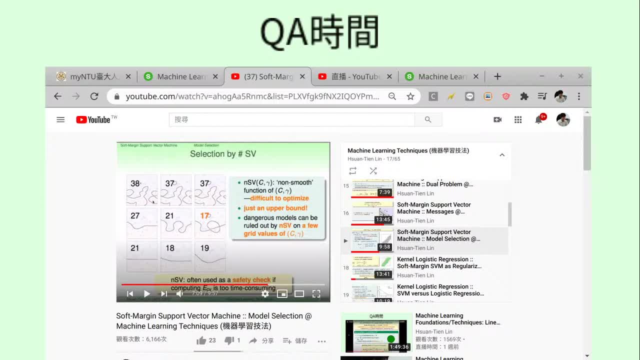 大概是这个样子, 应该说后面技法的部分. 大家可以想象说 技法跟基石有一些不一样的地方 是即使我们有一个蛮明确. 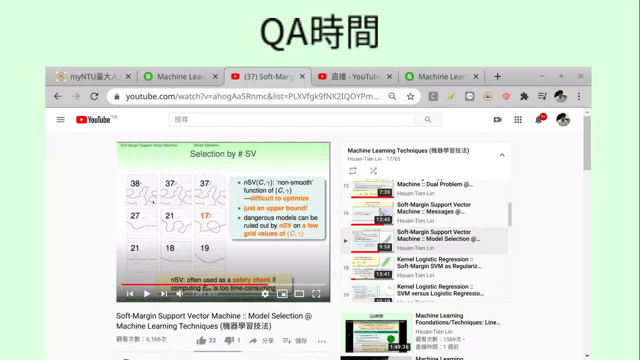 我们觉得这个教起来比较好的顺序, 但是技法的话比较像是分支长出去, 所以它当然在原来课程设计上. 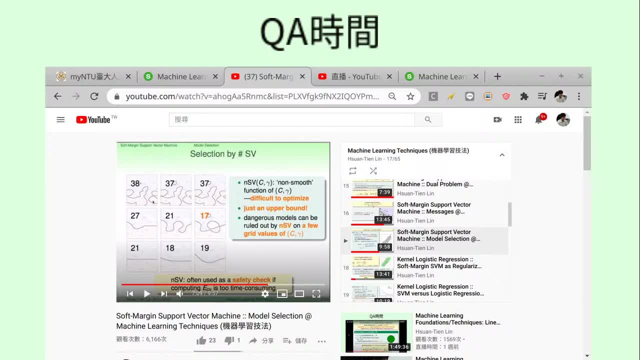 有一些Dependency, 不过那Dependency没有太strong 所以要先教什么后教什么. 是有一些些弹性的 那我自己的计划就是: 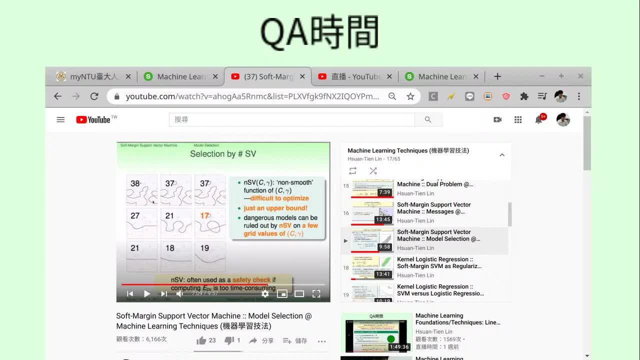 每年搞不好会做一些不同的调整. 今年先教这个看看 再来先教那个看看 那也尝试着未来发展不同的. 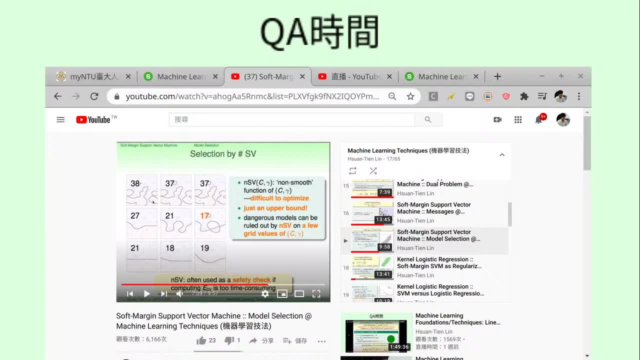 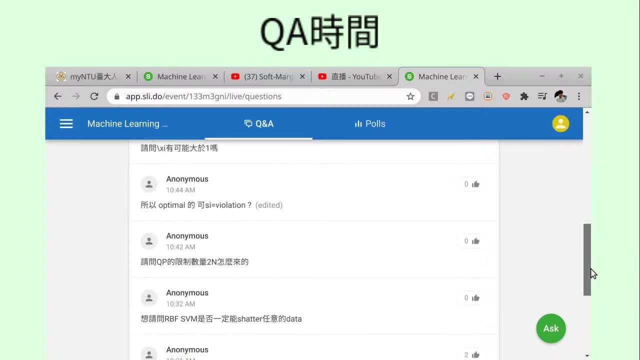 课程的可能性. 还有问题吗? 刚才线上的同学有一些问题, 那我们用这个机会稍微的看一下. 一个是这边有同学说: 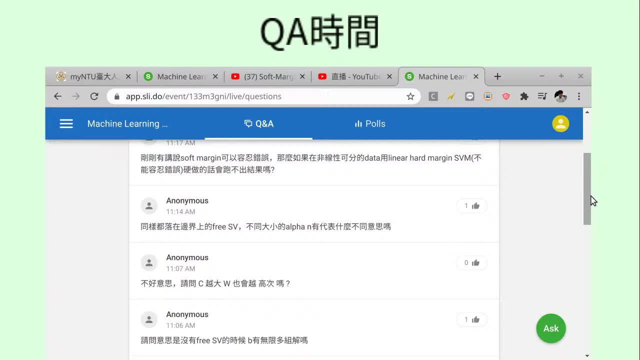 没有Free Support. Vector B有无限多组解吗? 是B有无限多组解, 但是这个无限多组解其实是有范围的. 例如说你可能会得到一个范围说: 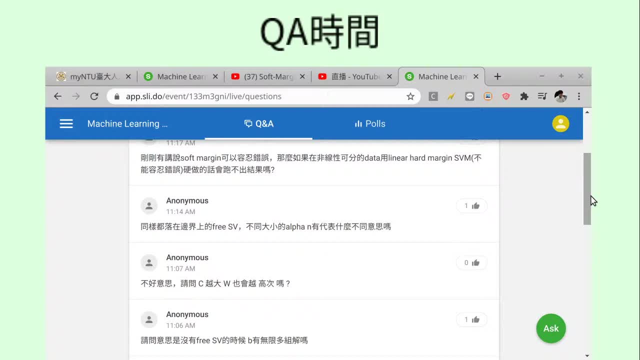 B是1.5到8.7之间, 意思是说1.5到8.7之间 任何一个值都可以是你的B. 那真正你如果去看一般软体里面. 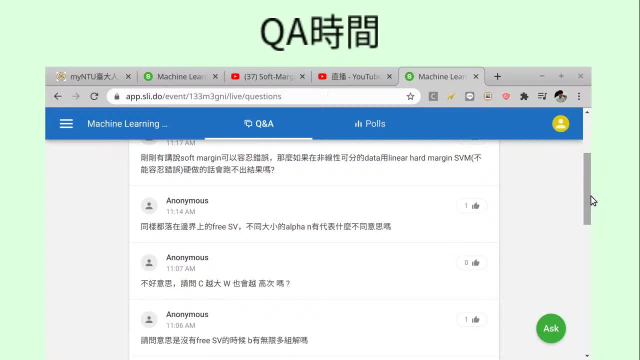 要选哪一个B的话 就会有一点点tricky. 不过像力北实验 他大体上就是选1.5到8.7, 那个最中间的那个值. 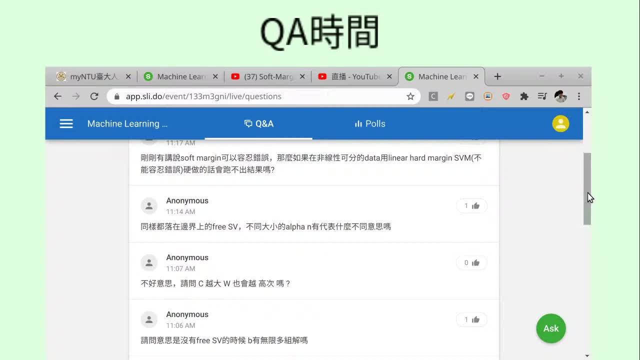 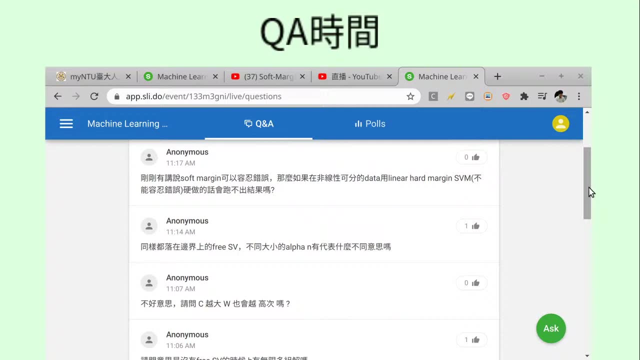 同样的落在边界上的Free Support Vector. 不同大小的αn有代表什么不同的意思吗? OK好这是个很好的问题. Technically没有或至少没有很容易解释的. 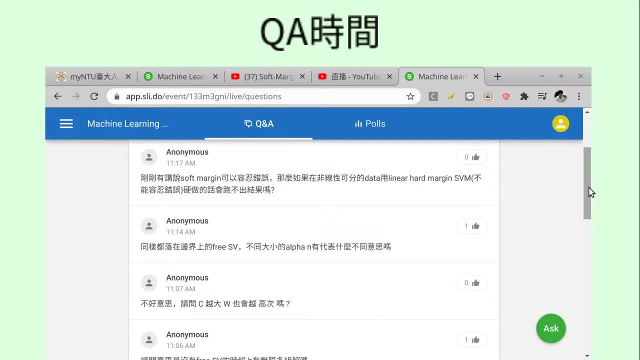 Physical meaning. OK那, 但是我们可以很容易解释为什么没有. 大家记得那时候在Hard Margin的时候, 我曾经说过说 为什么会有落在边界上? 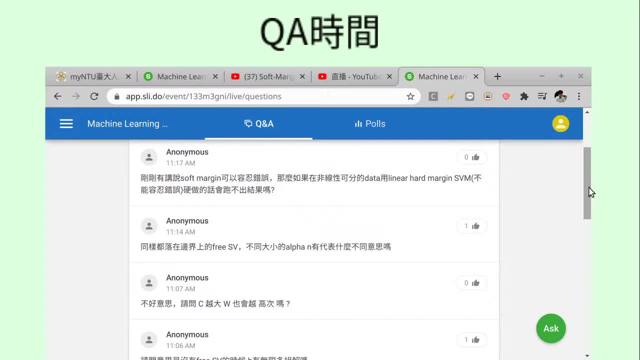 但是α等于0的那些 因为如果我们train好的一个SVN 然后我现在在胖胖的边界上狂撒一堆点的话, 这些点我们可以说他都不是需要的. 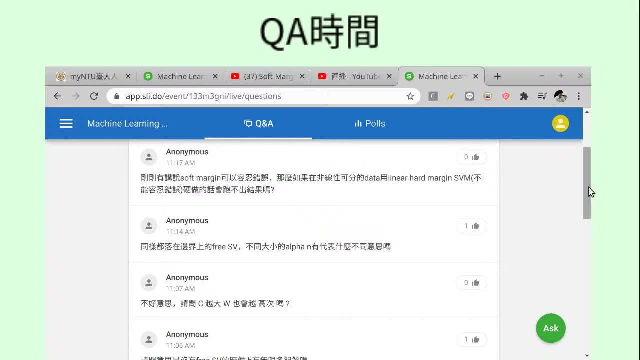 OK所以他都是新加入的龙元, 他的α可以是0, 但是另外一方面来说, 其实他α也可以不是0, 就是因为落在边界上的那就是一些Free Support Vector. 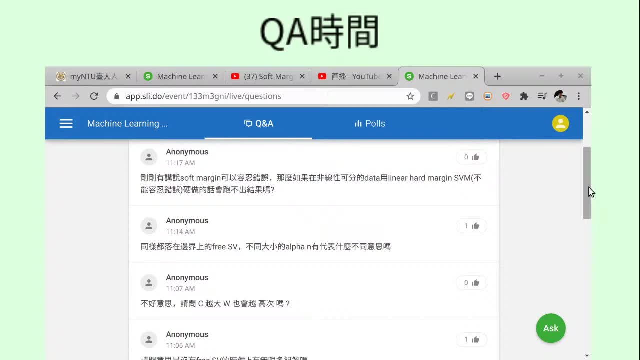 这α也可以不是0. 所以可以想象说你在那边撒了很多点的时候. 其实你在那个边界上. 你一般把它想成需要的α. 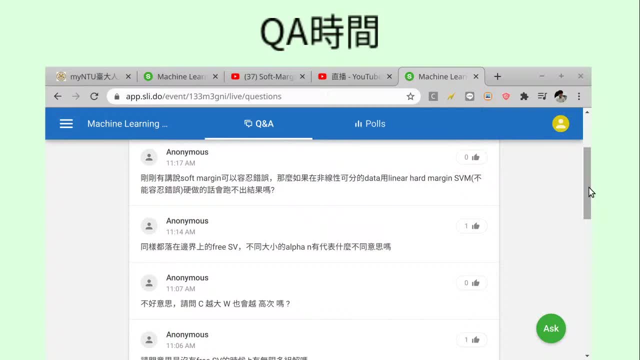 是可以等于是, 例如说我现在原来有一个点 然后它的α是3, 这个3是可以分散到其他的α上面的. 当然怎么分散 可能就要看你的Optimal Solution怎么做. 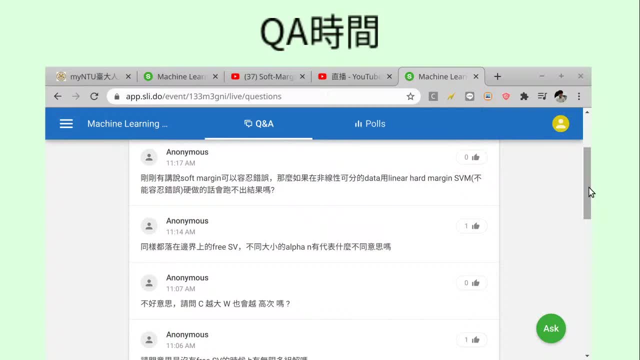 但是在那个情形里面 其实你可能可以想像你是会有很多个Optimal Solution, 很多个在α那边的Optimal Solution. 那既然可以分散的话, 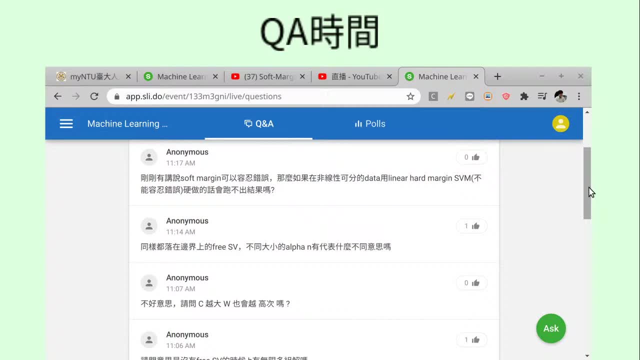 你说好那我现在假设我有两个点. 我们很rough的讲, 说两个点一个点的α原来是3, 一个点的α原来是0 那我们可以也有可能可以做1.5, 1.5. 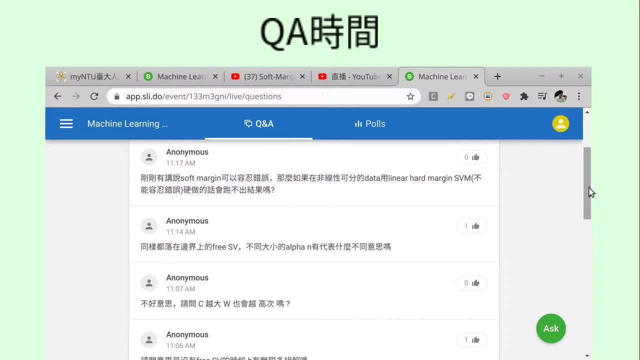 那可能也可以做1.126跟1.874 好然后所以我们可以, 如果可以把α这样自由的分散的话, 看起来α的大小 意义就没有那么大. 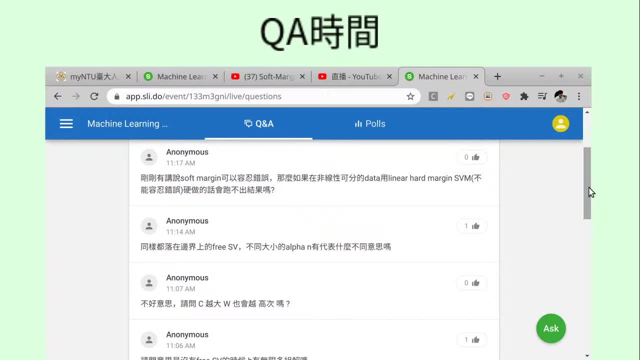 这是个比较rough的解释. 这种平均性没有那么容易解释, 但是我们希望给大家一个概念 说为什么α的value不见得有那么强的意义. 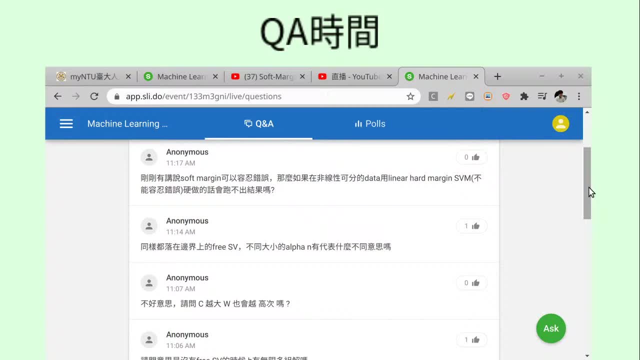 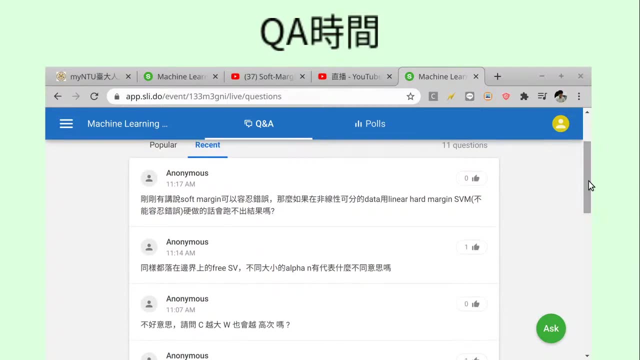 因为α上面是有一些些可能的自由度, 尤其是如果你落在边界上的电比较多的话. 刚才有说soft margin可以容忍错误 如果不是线性可分的data. 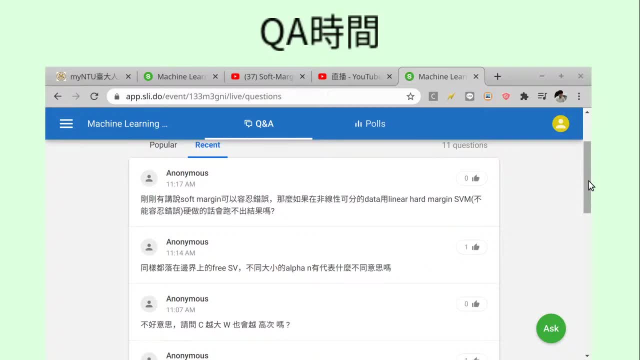 用linear hard SVN会跑不出结果吗? 会, 或至少你跑一般的QP. 它就跟你说它解不出来. 就是说这个在optimization问题里面叫做invisible. 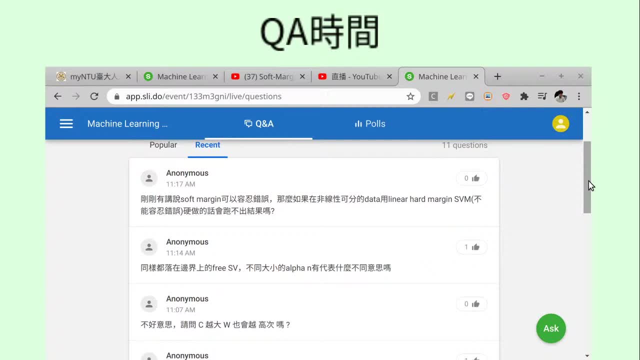 意思是说没有任何一组变数 可以满足所有的contraint, 所以基本上来说会处于一个解不出来的状态. 当然这跟你的solver有关. 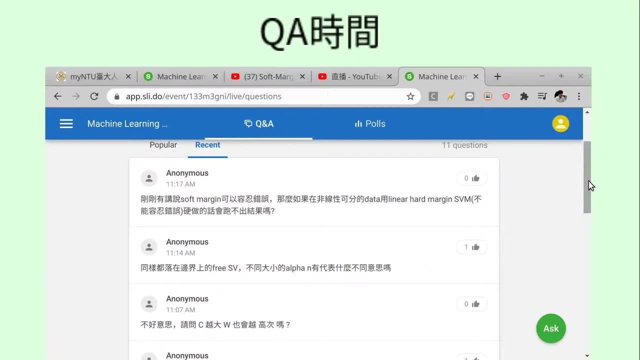 有的solver比如说你丢给它要写hard margin SVN的时候, 然后它里面偷偷的做一些 有点像contraint coloration那类的事情. 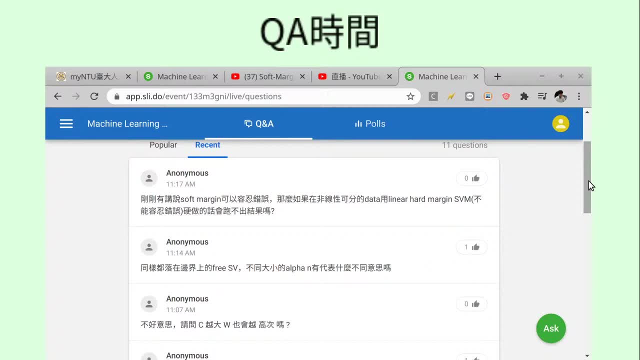 它先想办法容忍一些contraint violation等等. 那种solver就还是会给你一个解. 只是那个解就不是解嘛, 如果违反了所定的contraint的时候. 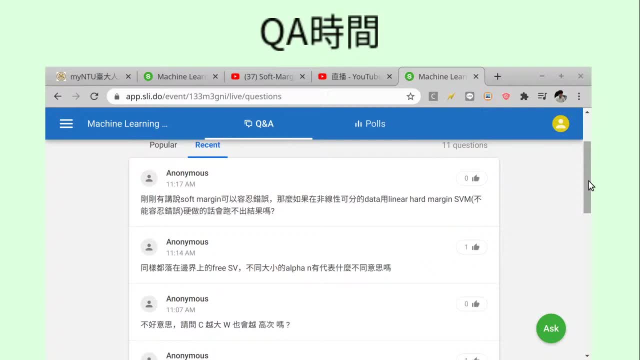 那个解显然就没有太大的意义了. 对 脑袋一直想要讲说: 这个社会住宅的钱定的太高的时候. 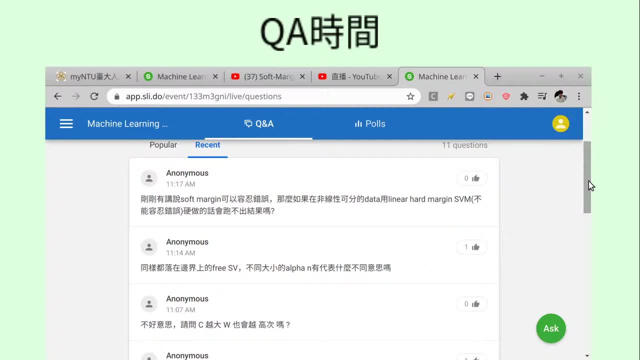 社会住宅就没有意义了, 但是 不小心又讲出来, 真是糟糕. 总之回到同学的问题的话 就是hard margin SVN的缺点. 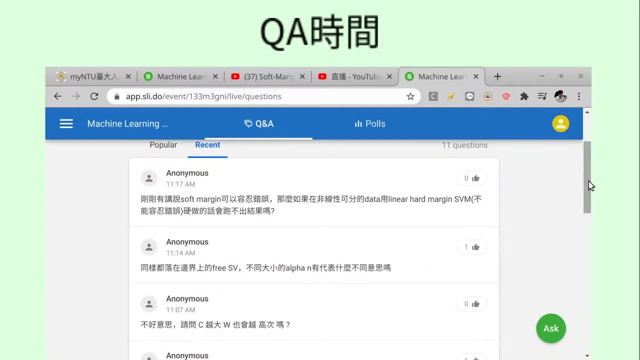 就是它可能会没有解, 会是infeasible的. 那soft margin SVN相对的优点就是什么, 不管是什么你总有解. 你只要给一个finite C, 你总有解. 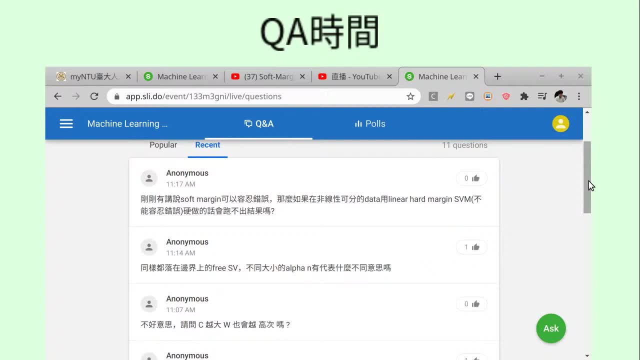 那个解可能很好可能很烂, 看你给的C是什么东西, 但是总有一个解. 所以我们的课 另外一个很重要的message就是: 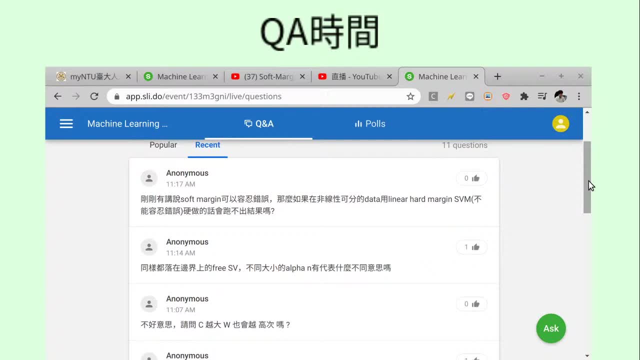 其实我们要的? 我们实务上在用是soft margin, SVN, 不是hard margin, SVN 就是hard margin只是教学上比较好用一点. 我说我们当做一个切入点. 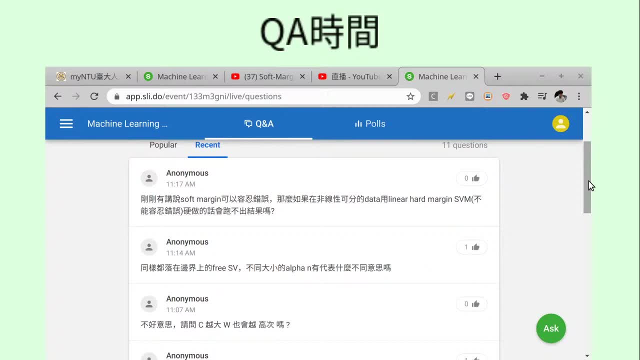 但是实务上来说没有人在用hard margin SVN. 你就是用soft margin. 你很想要hard margin的效果. 你用soft margin把C设得很大, 但是这个不会特别. 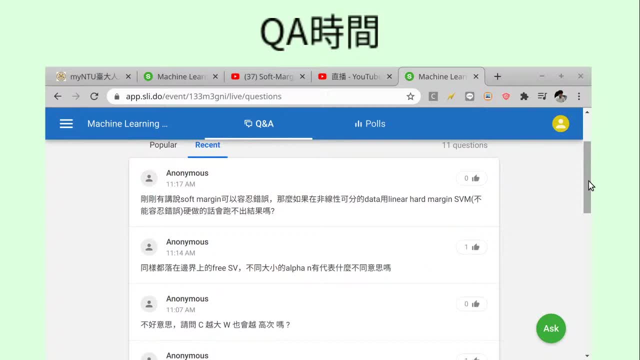 至少大部分的时候, 你在SVN的package里面不会特别找到 的hard margin SVN来应用的package. 人家一般提到SVN的时候 所指的是soft margin SVN. 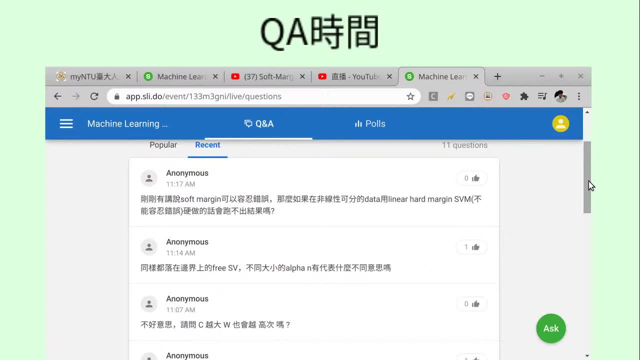 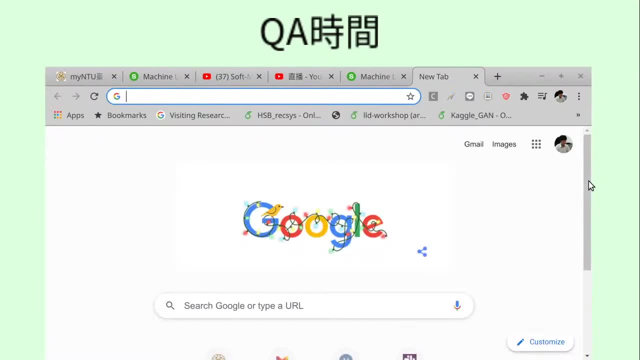 所指的是我们今天所教的这个版本. 好, 现场同学还有问题吗? OK, 我想要用这个机会 稍微带大家看一个东西. 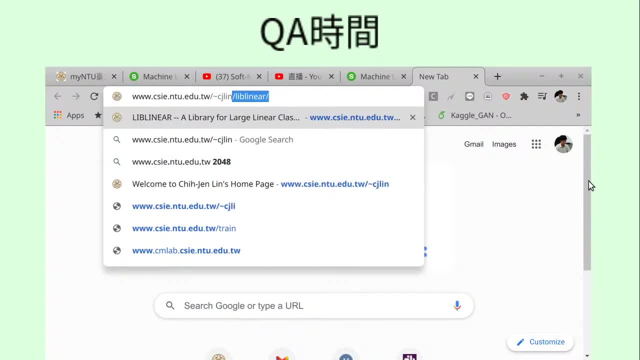 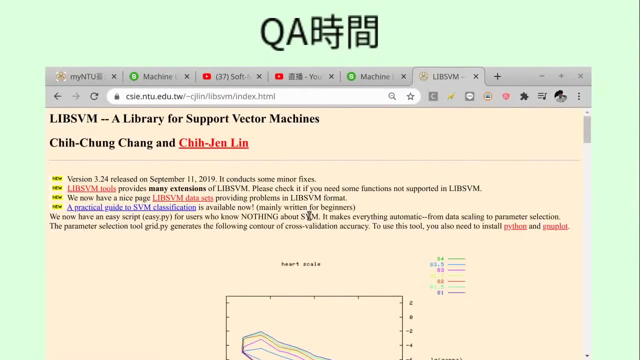 就是因为我们刚才提到了 有关SVN的参数选择的部分, 白位如果你对SVN充满了好奇, 我们今天玩的这些东西充满好奇的话. 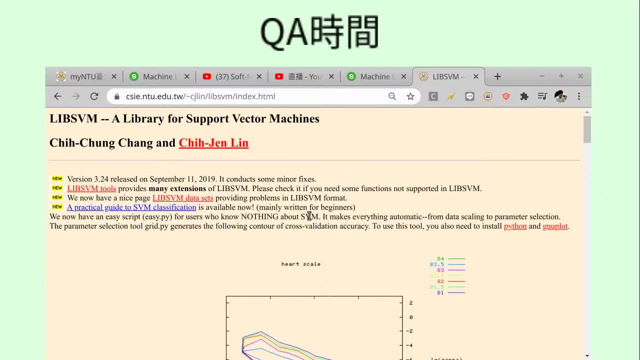 大家注意的是, 如果你休息时的话 注意的是你用过LibLinear这个package. 另外有个非常有名的package叫LibSVN. 这个package是林郑老师的实验室所开发的. 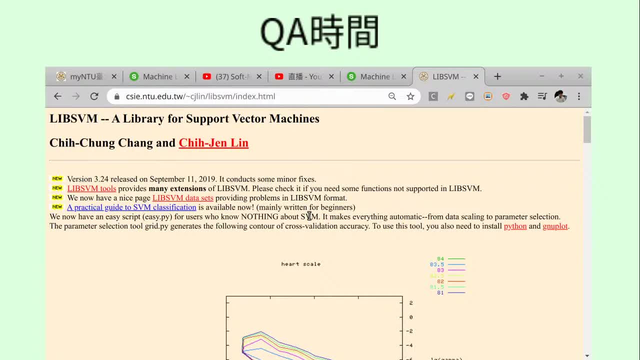 应该是全世界最多人使用的SVN的package: LibSVN这个package解的是dual problem 就是soft margin的dual problem, 就是我们今天后来讲的这一段. 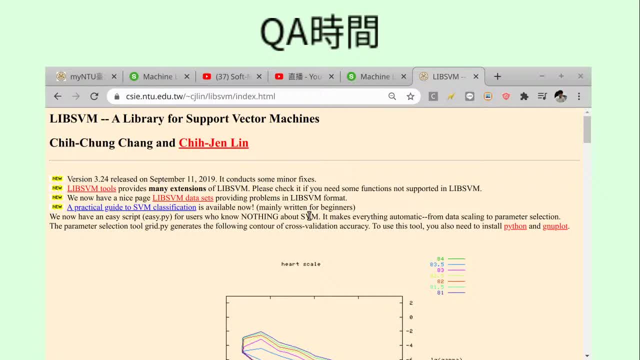 LibLinear. OK, 大家在作业室里面 那个package解的是大部分的时候 解的是primal problem, 包括SVN的primal problem, 包括logistic regression的primal problem. 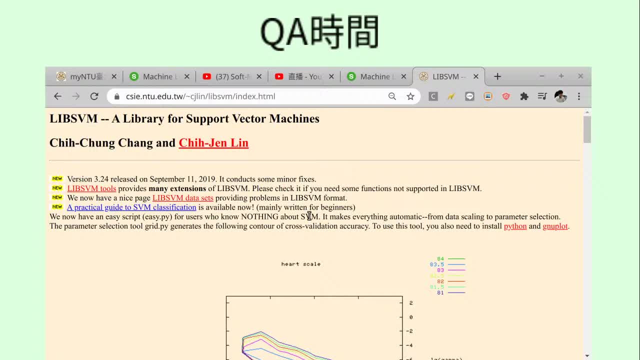 那你会看到说在一些参数下 它有解logistic regression的dual problem等等. 那是一些比较特殊的用途. 不过我们这边不特别探讨. 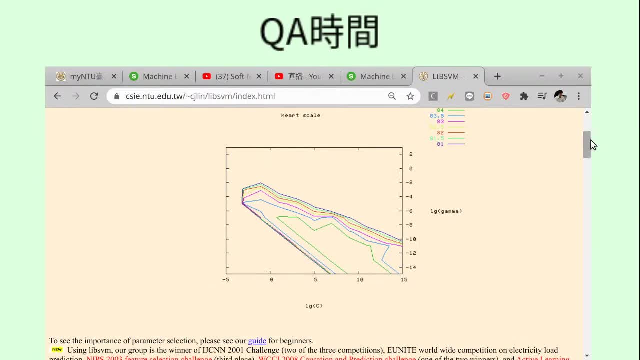 那我今天带大家看LibSVN这个网页. 主要是想要讲几件事情. OK, 这个事情其实是SVN的参数选择. 我们刚才说你就是不同的C跟γ. 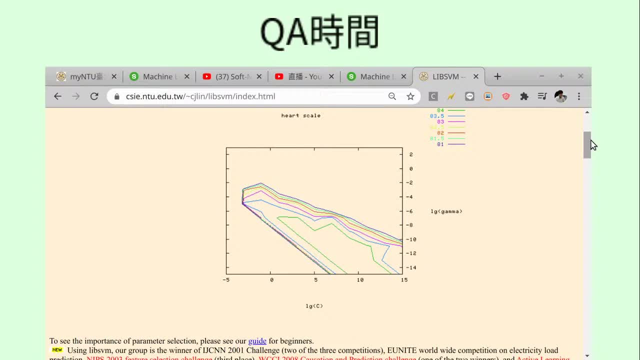 然后试一下去做cross validation 然后看看会发生什么事情. 这是高选SVN的东西. 这个结果常常可以被化成一个这样的contour plot. 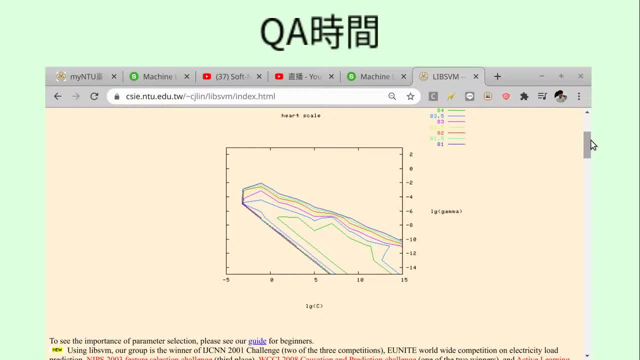 就是等高线图, 等高线里面的每一圈代表什么意思呢? 代表roughly它的cross validation的error 是多少 在这个图里面它化的是accuracy. 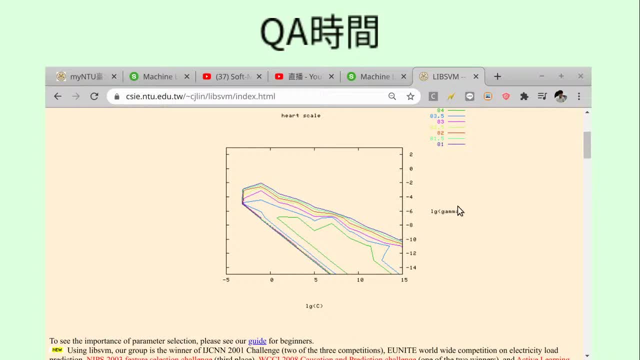 而不是error. 所以例如说我们看到说在这个图里面 它这里最内圈的这一块 可能是84%的cross validation accuracy 稍微外圈一点点显蓝色的. 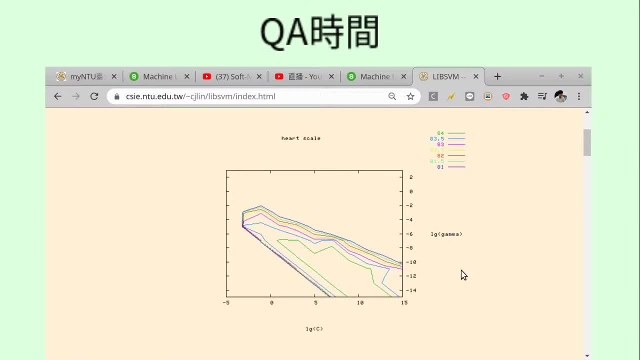 可能是83.5, 然后往外等等. 所以你从这个图 那这个图怎么做出来的呢? 这个图就是在γ跟C的世界里面. 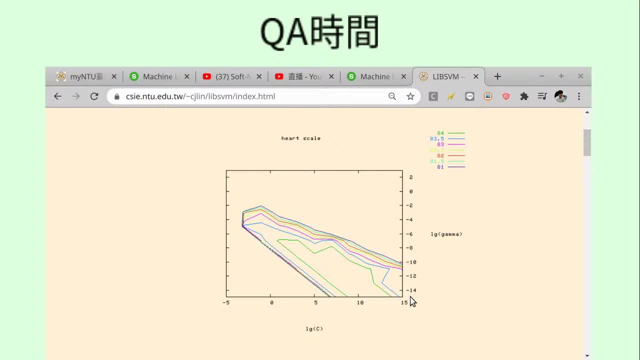 做一堆格子点, 去找它的cross validation error, cross validation, accuracy, 所以你就一堆格子点的值 然后再把那些格子点的值送去做一个. 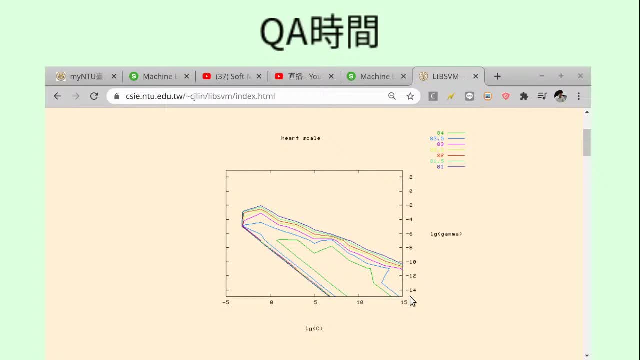 等高线估计的演算法 然后去估计来说: 好, 所以那几个点附近都是84, 所以画一个 这个说84的大概是这个区域. 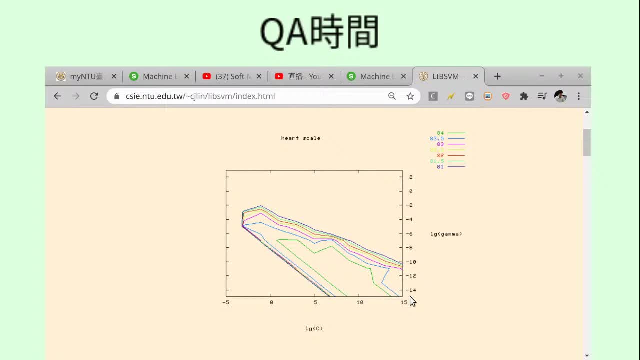 那几个点附近是83.5等等的, 其实就把那些值 在这空间里面的每一个地方做个内差, 或者用Machine Learning的Terminal宇宙的regression. 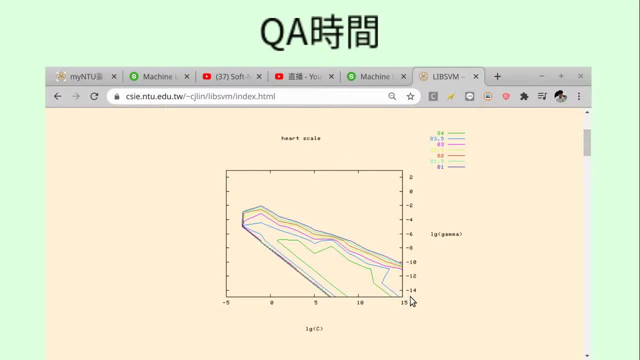 OK, 然后给你看regression: 那个regression curve 切出来等高线的结果是怎样? 为什么大家看这个图呢? 因为大家实际上会看到说: 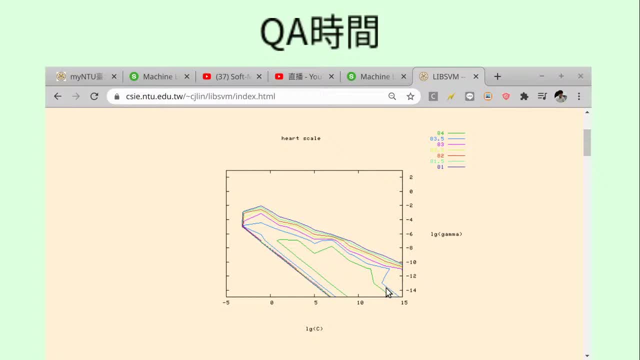 这好像有一个有一个山峰状这样子. OK, 说这个最好的accuracy, 可能你会想象说: 你要爬到这个山顶上的话 会落在大概是我的游标所指的. 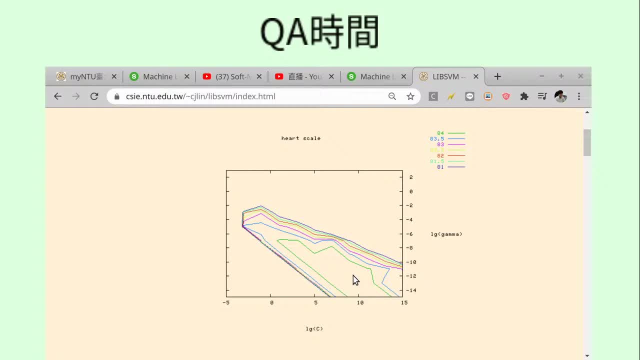 这个附近的地方. OK, 那这是一个蛮typical的SVM的behavior. OK, 证明说为什么这个图会长这样等等等等的, 但是这是个很好的工具. 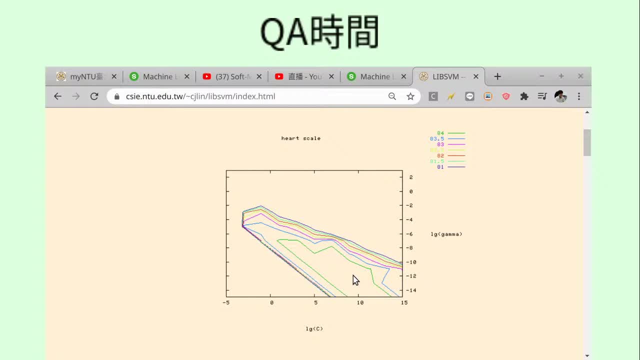 来帮助你看什么呢? 举例来说你如果这个跑一跑 跑了一些些比较粗略的参数之后 你可以zooming. 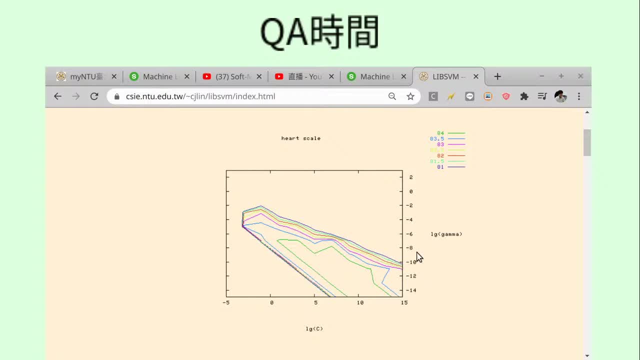 然后你发现说好的参数好像落在这个区域. 那你就在这个区域里面 你再撒一些比较精细的格子点下去. 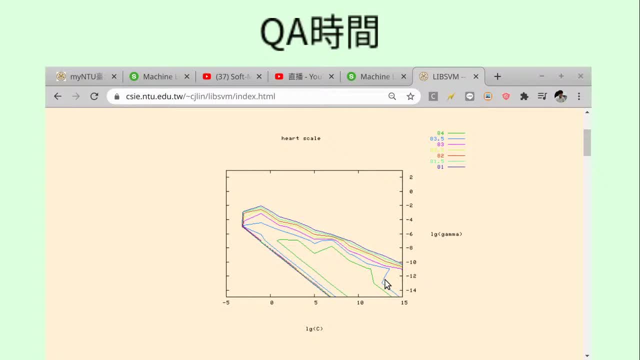 然后去做你的参数选择. 这样的参数选择的方法也是蛮常见的. 反正我刚刚说这个两个轴, 一个是C一个是Gamma, 实际上在原来画这个图的时候 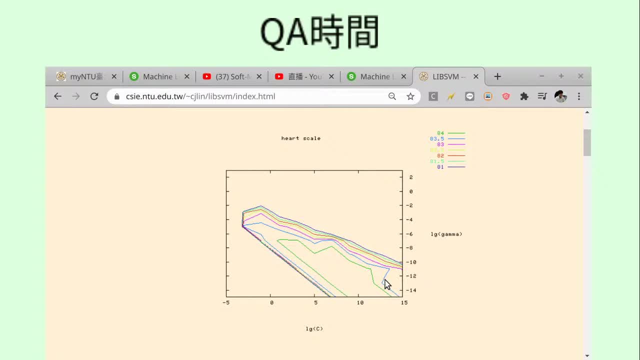 用的是Log Scale, 意思是说一边是Log C一边是Log Gamma, 但是整个的讯息 刚才跟大家陈述的是类似的, 所以我们会看到几件事情. 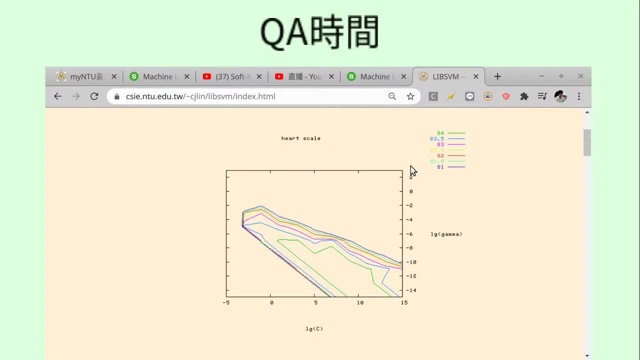 太大的Gamma不是太好. Gamma一路往上, 太大的Gamma其实不是太好. 我们之前有跟大家讲过: 好C要大一点, 可是不要太大. 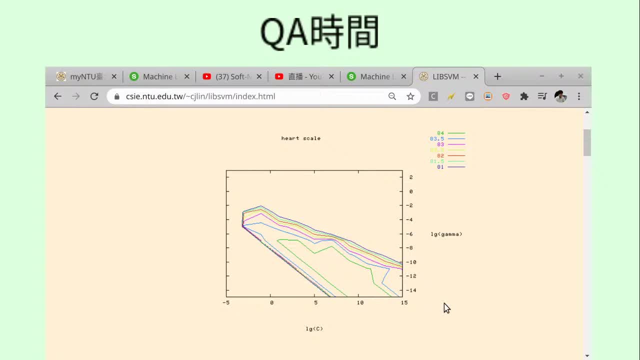 因为如果这个C真的跑到太大的话, 大家可以想象 你会有比较像Hard Margin Overfilling出现. 但是C太小, 往左边这边走也不是太好. 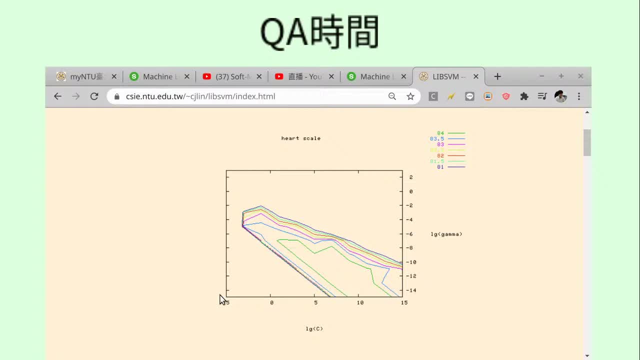 因为你说你号称有个胖胖的边界, 但是一堆Violation 这两个东西其实是没什么用的. 所以我们希望用这个图. 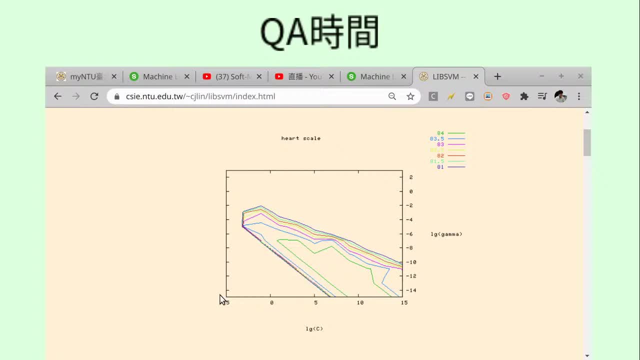 来跟大家稍微补充一下, 就是SVM在这个所谓的参数选择 这时候发生什么事情? 那你如果对玩SVM真的 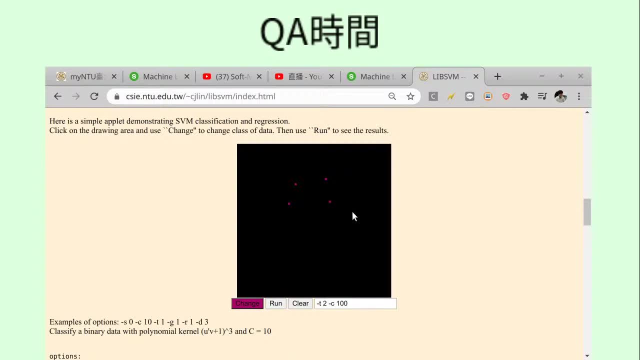 真的很有兴趣的话. 这边有个传说中的Java App 然后你就可以做一些事情, 比如说在上面随便点一些点. 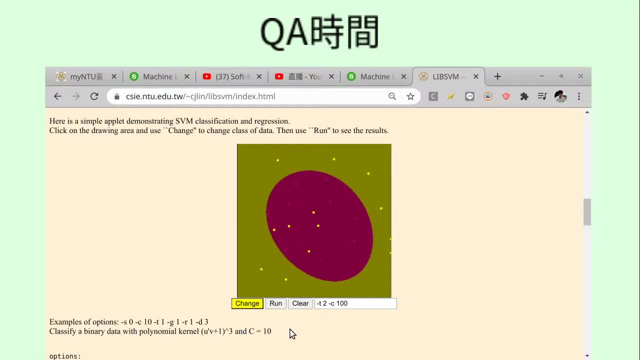 Run, 然后你的SVM就跑出一个 分类的结果这样子, 我当年就是被这个东西. 我讲片序. 这样对林志老师太不敬了. 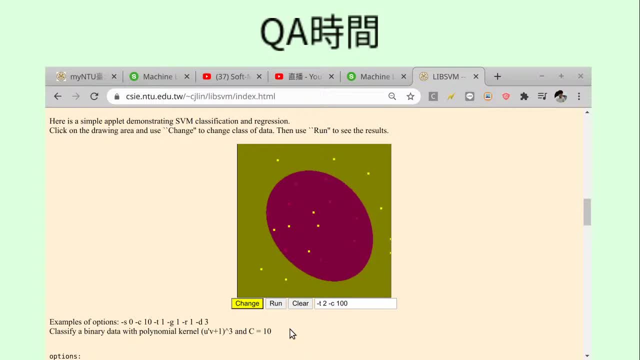 我当年就是被这个东西吸引了 开始做我的Machine Learning Research. 就是基本上非常视觉化的 在看SVM在做些什么事情. 当然你可以下一些有趣的参数. 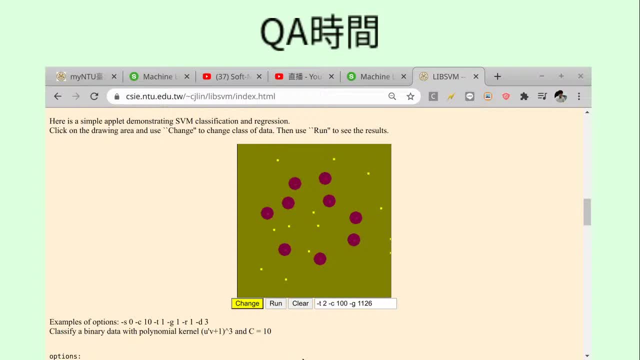 然后看看会跑出些什么. 比如说你要跑出我们 这个上一次说的: 你有很大的Gamma, 然后跑出那个尖尖的东西. 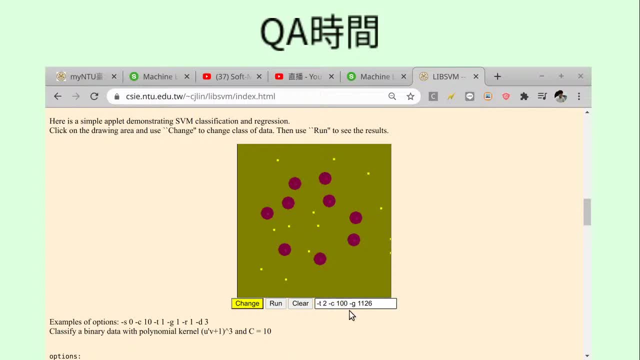 这个不是真的非常的困难. 然后小一点的Gamma好了. 然后大一点的C: 你会看到一些些不一样的Behaviour 如果你写Machine Learning作业. 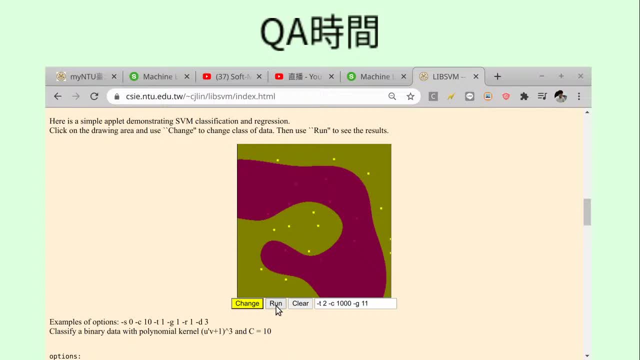 写到心情不好的时候. 玩这东西其实蛮疗愈的 好了我觉得很疗愈. 我不知道你们有没有觉得很疗愈. 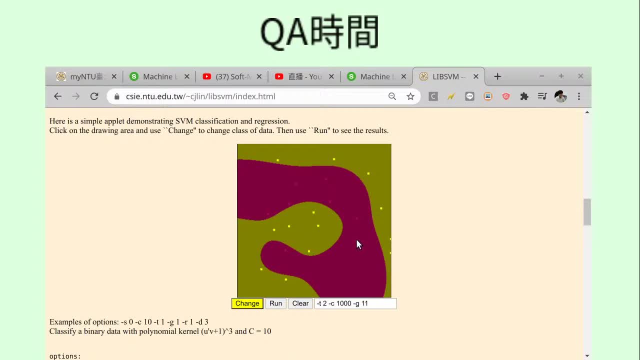 可怕你们觉得超烦的那也不一定, 但是这是另一个方式 可以帮助你说. 不只是我们课堂上画给你的那些图. 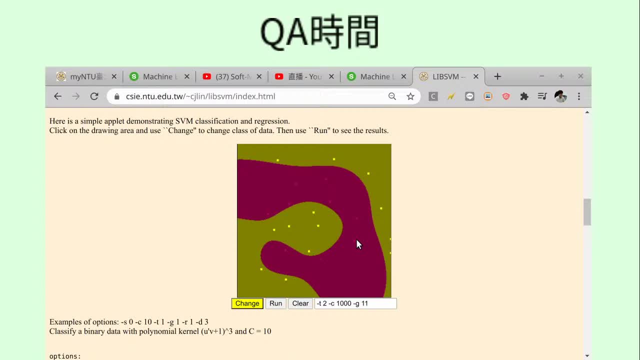 你自己想要画什么样的图, 就画什么样的图 然后来帮助你了解SVM这样 那摆着位 你如果真的使用这个的时候. 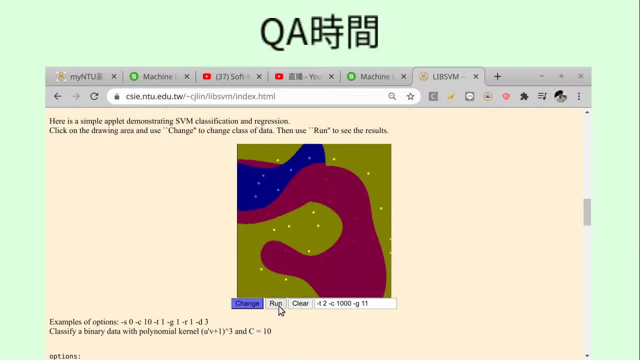 你会发现你不只可以画两个颜色的点, 你可以画三个颜色的点, 然后那也会出来三个颜色 不同颜色的Boundary. 在LibreSVM里面它是内建有Multiclass的. 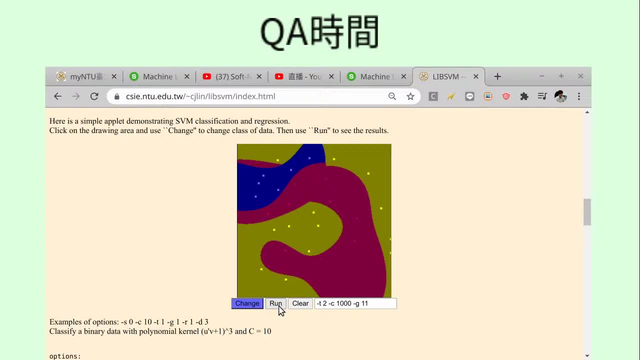 而它Multiclass是怎么做的? 它Multiclass是用1vs1做的. 就是在我们基础学习基石的时候就讲过的. 而你如果看LibreLinear的话: 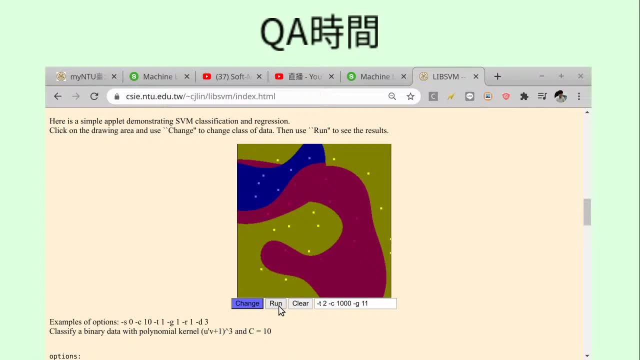 LibreLinear有Multiclass, LibreLinearMulticlass是怎么做的? 它是用1vs0的, 它是用Multiclass的 然后那当然有一些不一样的SoftwareChoice等等的. 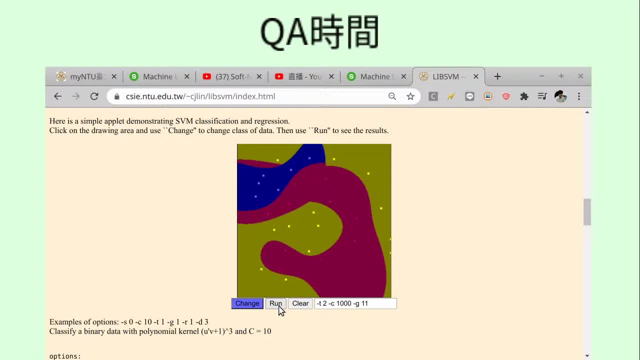 但是也给大家看看. 说其实你在, 如果你跟着我们在基石一路上来的话, 你在基石学到的一些东西 你在这边都可以看得到. 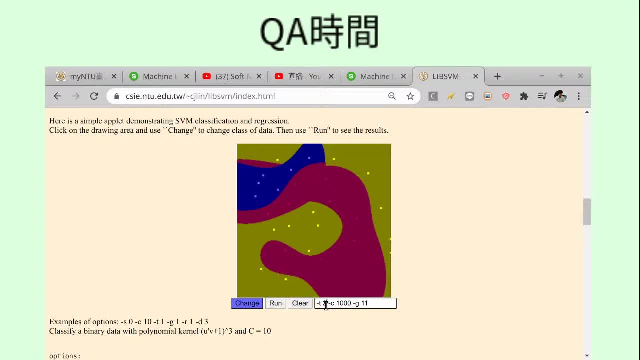 都可以用得到. 如果你们硬要用LibreSVM解这个 线性的分类的话 那也可以. 所以这是一个Linear结果. 当然就有很多的Violation 因为我刚刚故意弄的是一个. 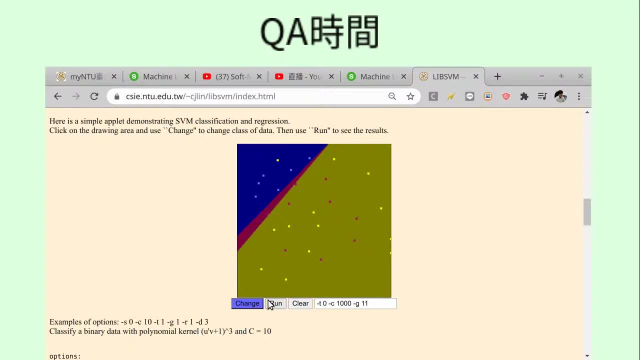 不是线性可分的DataFit, 但是大部分的时候 我们都不建议用LibreSVM解Linear的SVM 因为一些原因. Linear的SVM在Dual解 可能会很慢. 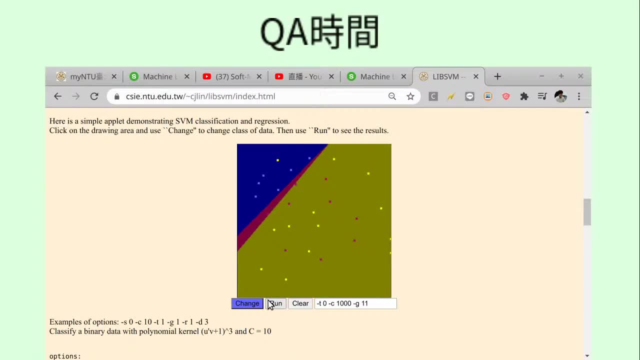 可能可能会很慢 然后那所以 很多时候不会太建议 用LibreSVM来做. 你如果真的要用Kernel, 你用LibreSVM做. 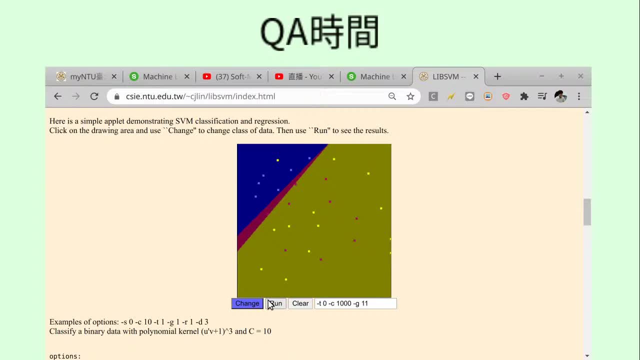 但是你没有用Kernel的话, 你只想要Linear 就乖乖回到像LibreLinear 这样的Tackage去做, OK好, 所以这是跟大家补充. 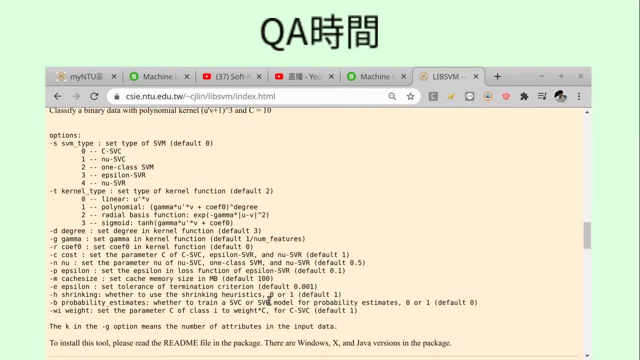 OK一些有关SVM的部分. 那大家有没有什么样的问题? OK好没有的话, 那我们来这个接下来 我们会进入. 我会先简单的进入Neuron Network的影片. 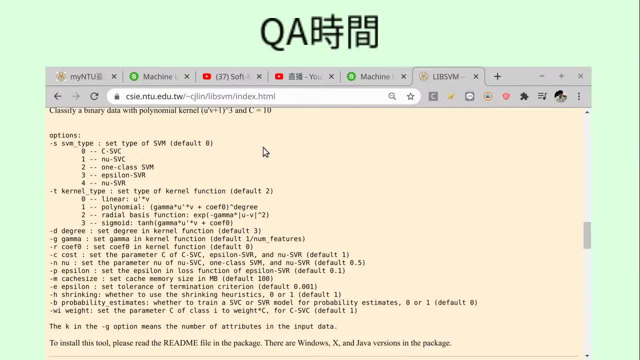 我们也许不会讲完. 也许不会讲完完整Neuron Network. 我们会先放适当Neuron Network的影片, 然后下一次上课. 我们会先进入把Metric Factorization. 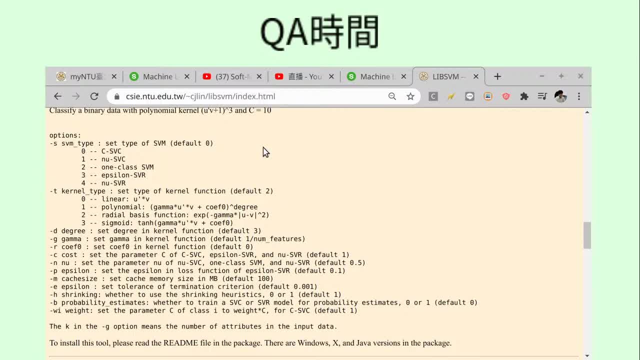 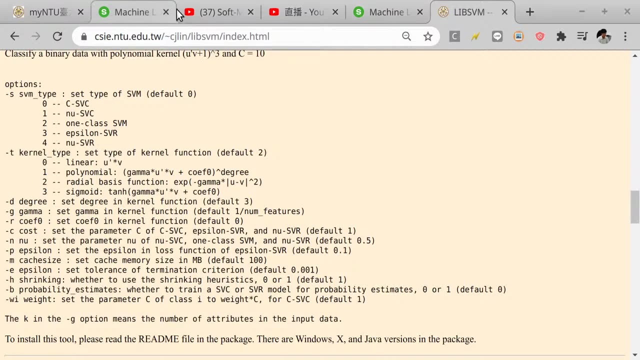 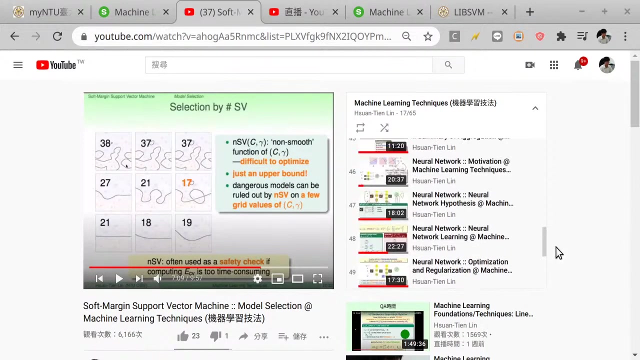 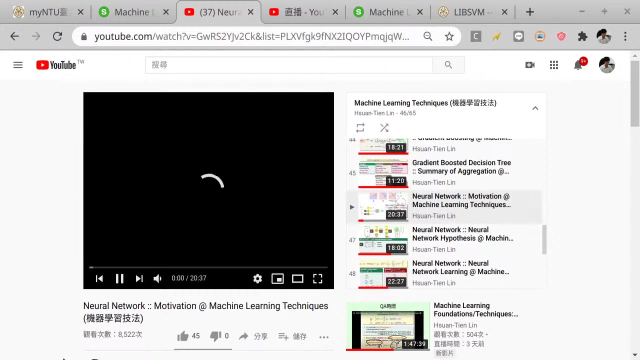 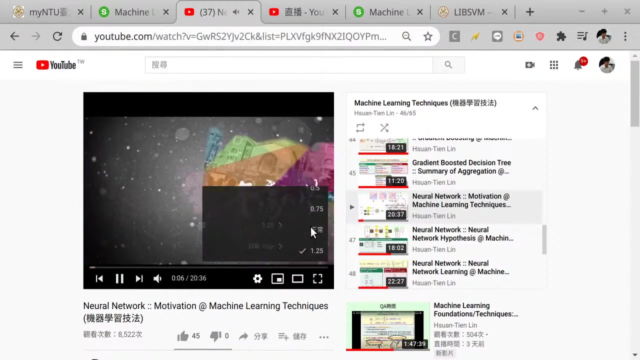 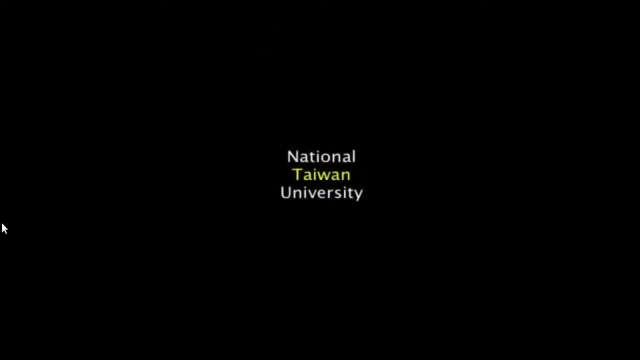 也就是在推荐系统里面 一个主要的方法把它讲完 OK然后回头后面的课程. 我们再做其他的设计. 大家好大家好. 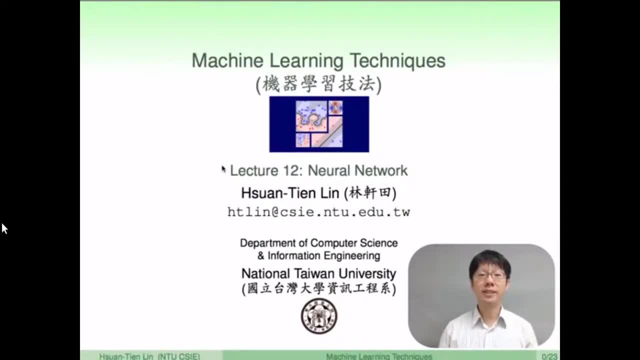 欢迎回到今天的机器学习技法课程. 我们今天要教给大家的是Neuron Network. 这是在机器学习里面 非常元老级的一个模型. 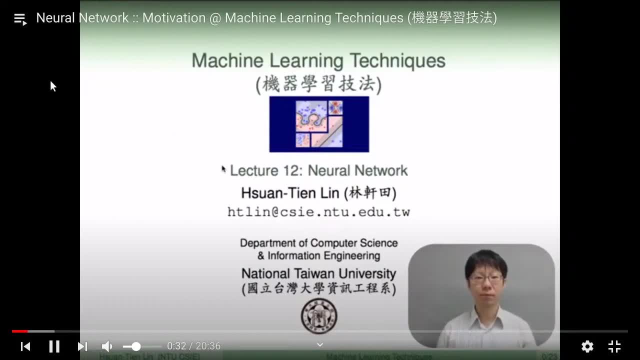 那我们待会会为大家做简单的介绍. 我们先来复习一下: 我们上一次上了些什么. 我们上一次讲到Gradient Boosted. 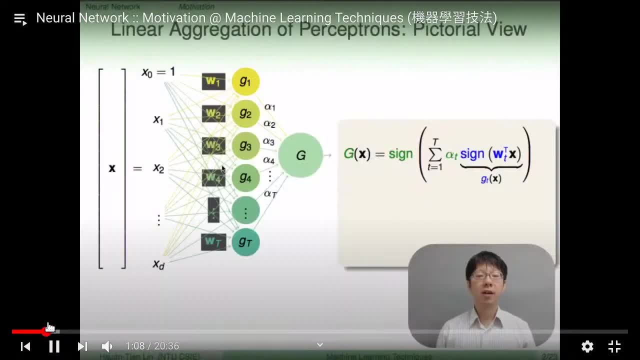 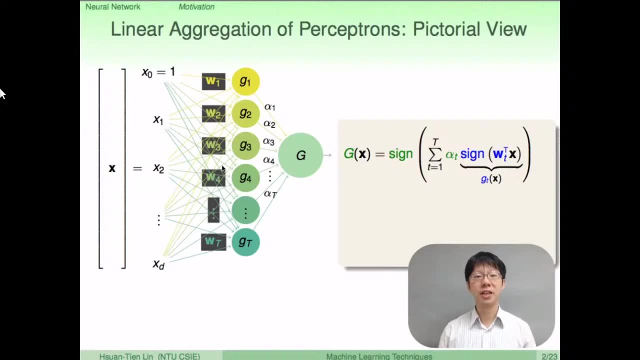 任何的. 那我们先从我们之前讲过的部分. 想像我们现在已经学过 Perceptron这样的模型. 我们说Perceptron这样的模型 就是你把你的输入. 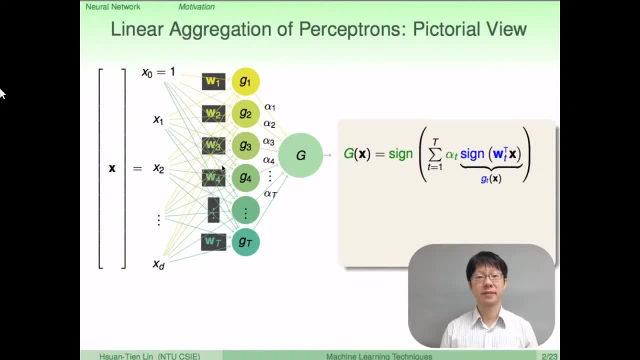 乘上一堆的选择, 算出一个分数以后 好像这个就这个分数. 切一刀 说大于0的是正1, 小于0的是负1. 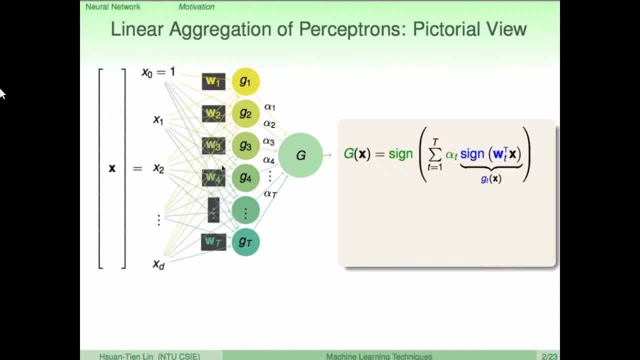 如果我们今天把一堆Perceptron 用Linear Aggregation的方式组合起来的话 图示上我们可以想象: 可能是这个样子的 从我们的输入出发. 我们例如说: 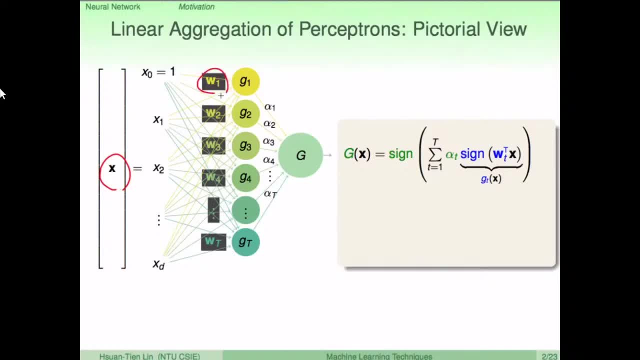 如果把它乘上第一组的选择 然后去取正负1的话 我们等于是做了一个G1 这样的Perceptron. 我们可能把它乘上第二组权重. 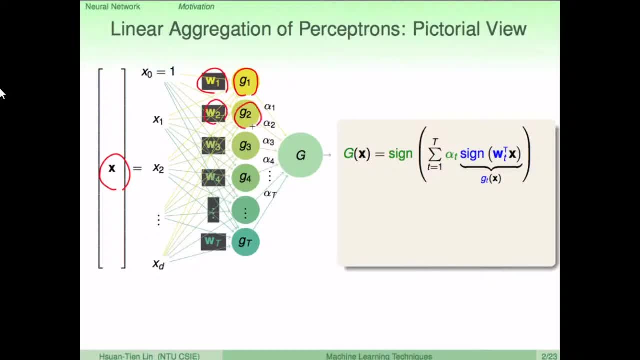 我们得到G2这样的Perceptron, 所以得到这样一堆的Perceptron之后. 这些Perceptron各自有各自的票数, 这些Alpha, 我们之前使用的这些票数. 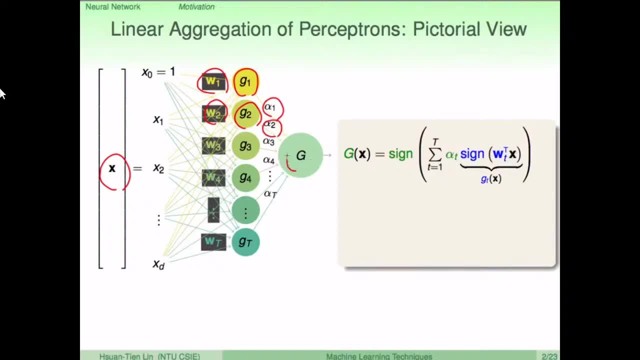 然后我们把它组合起来, 最后得到我们大大的G. 所以这样的流程, 这样的图描述了 我们从不从输入 然后乘上一堆权重. 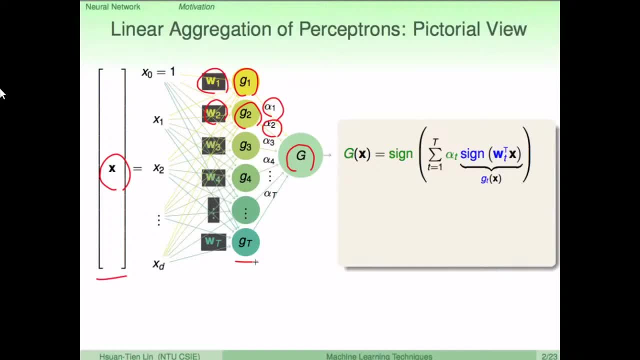 并且取正负号之后 得到一堆小G的输出. 再对这些小G的输出 乘上他们的票数之后 得到大G, 如果我们把它写成数学式的话. 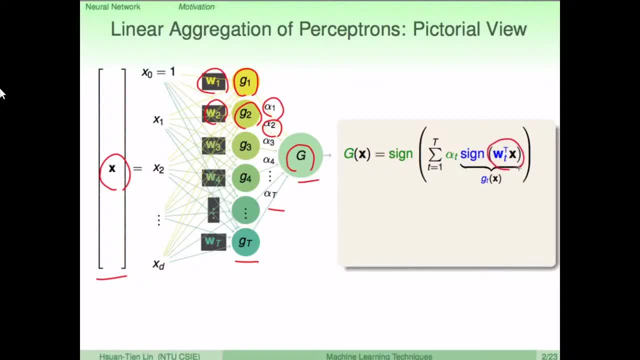 可能会长这个样子: 输入乘上各自不同的权重之后 取正负号. 这些输出就是我们的小G, 小G乘上他们相对应的票数Alpha之后. 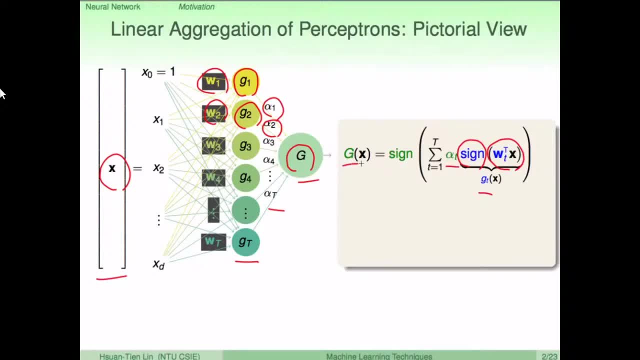 再取正负号 最后得到我们的大G. 所以现在我们看的是 这样的一个流程: 怎么从我们的输入 最后得到我们的大G? 我们注意到. 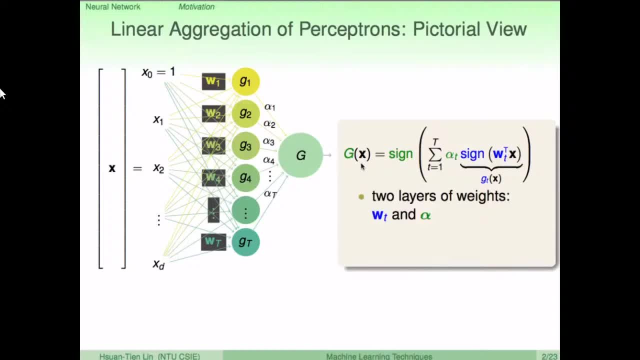 在这个过程里面 有两组的权重. 第一组的权重是在这一边. 我们怎么从我们的输入 进入到得到一堆的小G? 所以这些权重是我们的WT. 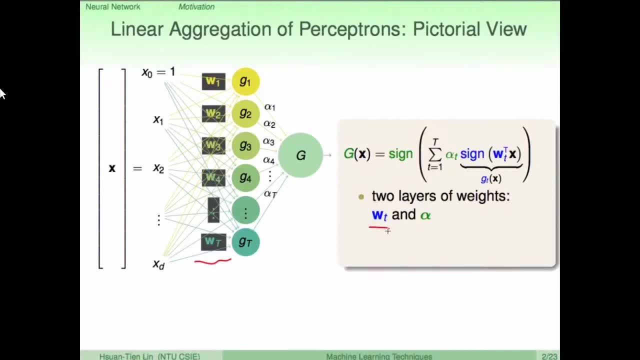 得到这些小G的结果 然后再来 有另外一组的权重. 是这些小G的投票的权重. 这些投票的权重, 我们说放在这个Alpha. 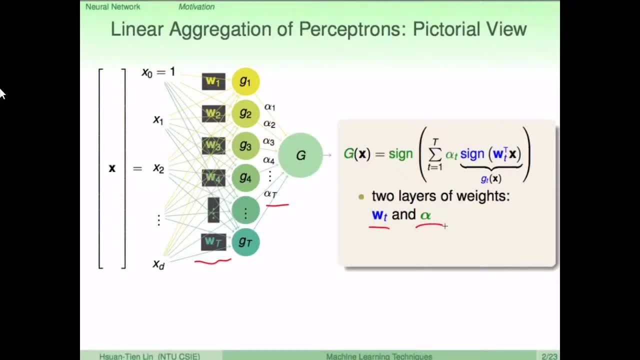 这样的一个向量里面, 透过这些权重, 这些Alpha, 透过这些投票, 我们得到大G. 在这个图里面, 除了有两层的权重之外. 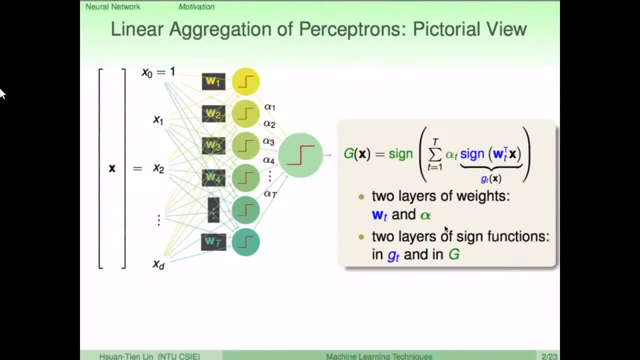 我们还有两层的什么呢, 在每一个小G跟大G里面. 他们其实都取了一个这个Sign: 小G里面取的Sign在这里, 大G里面取的Sign在这里. 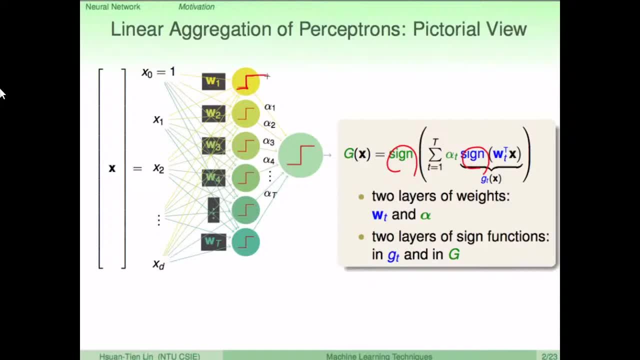 图示来说, 我们可以用这样一个, 我们这个Step Function, 就是这个阶梯函数来做代表, 说我们在这里做的事情是 算出分数以后. 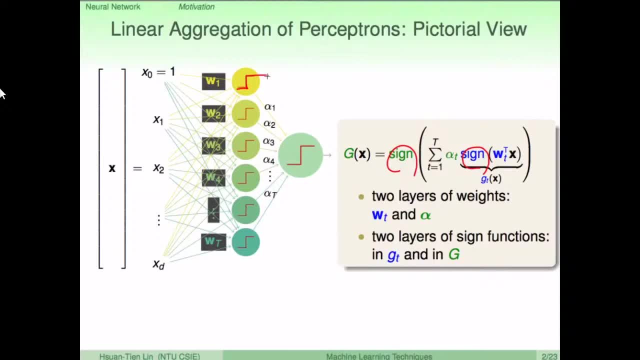 透过这个阶梯函数取的是正1还是负1, 最后把它输出去. 所以我们在图示里面 可以用阶梯函数来画. 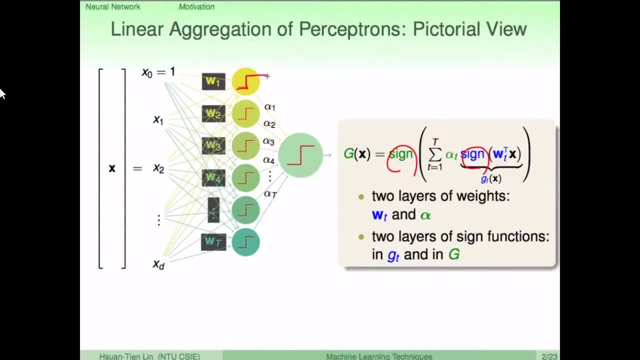 我们在这一个圆圈圈, 这个圆圈我们一般叫做一个Node, 在这个Node里面 我们做的运算, 算出分数以后. 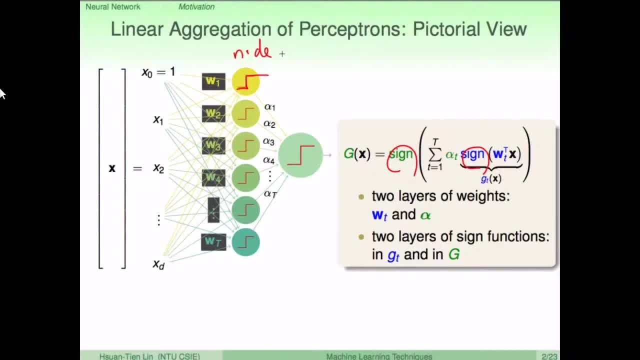 我们做的运算是取正1还是负1 输出去. 这是我们把我们之前所学到的Linear Aggregation. 如果我们搭配上Perceptron的话, 把它的整个作用的方式. 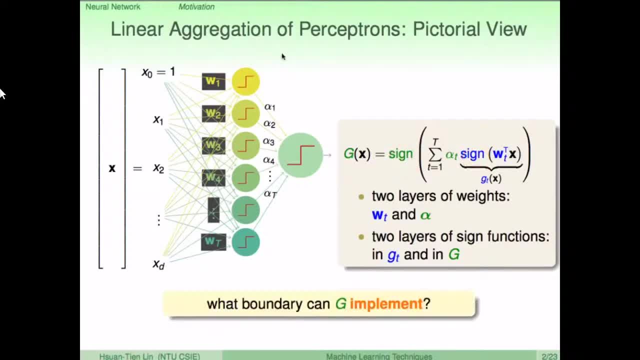 用一个图形来做表示. 那我们现在要探讨的问题是这样: 想像我们有一个这样的模型, 所以我们可以自由的决定 我们的这一堆的W. 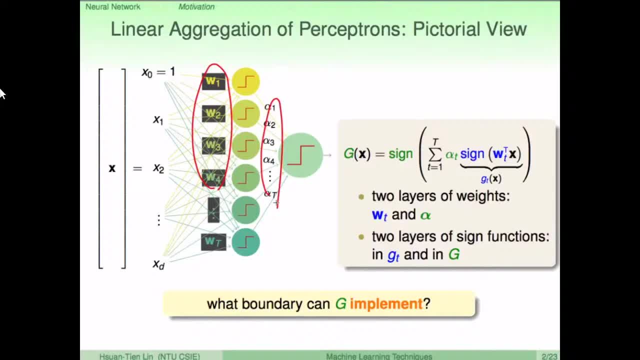 还有这一堆的α. 那么这样的模型 到底可以做到些什么样的边界? 它的边界的长相会是什么样子的? 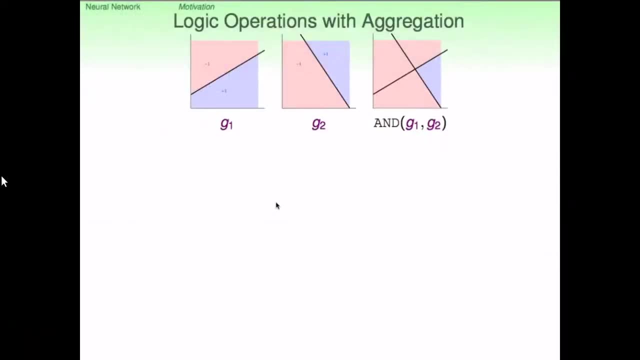 我们来看看这样的模型. 其中一个可以做到的是: 想像我们有一个Perceptron, 这个Perceptron G1. 这是一条分隔线. 它说蓝色那边是正1. 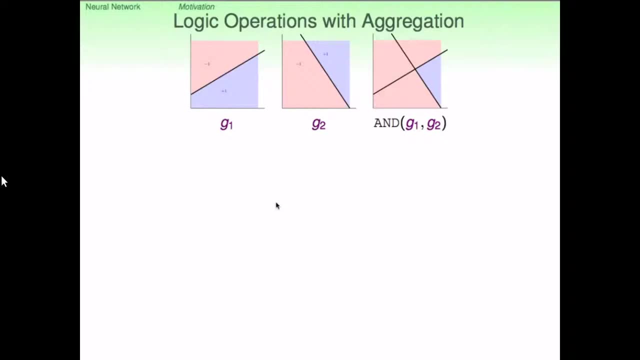 红色那边是负1. 另外一条分隔线 它是G2 一样蓝色地方是正1, 红色地方是负1. 我们来看看我们刚才讲的那样模型. 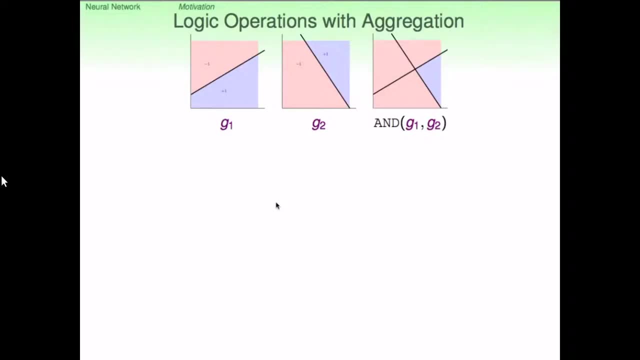 可以做什么事 那样的Aggregation of Perceptrons, 也就是说我把这两条线, 把它用我们之前讲的Linear Aggregation方式合起来. 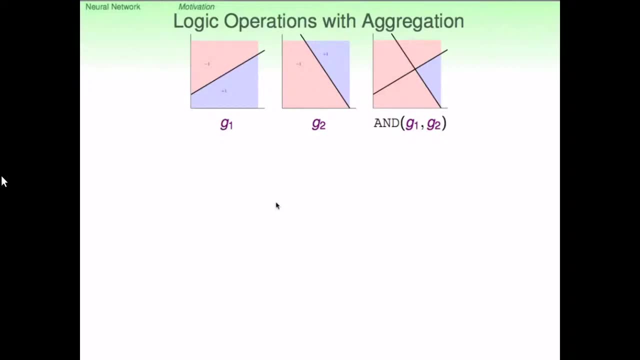 我们可以做到什么事. 我们说它可能可以做到. 右边的那个图, 右边那个图说什么, 右边那个图说是两个的End. 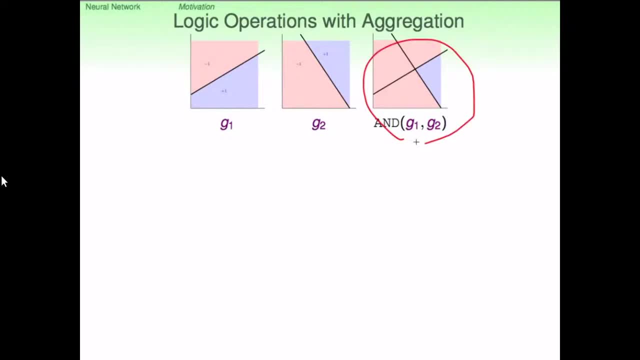 End什么意思? End是一个逻辑上的运算. 如果我们把我们的正1当作True 当作布林运算里面那个值 正1的当作True 那我们右边想做的是什么. 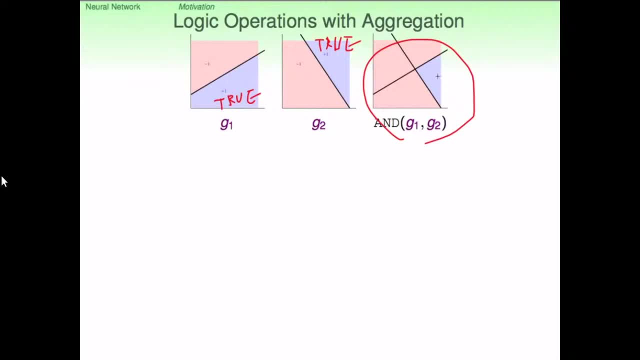 我们想做的是End, 也就是说要两个True 都是正1的, 成立的时候才会是蓝色的. 那其他的情形都是红色的. 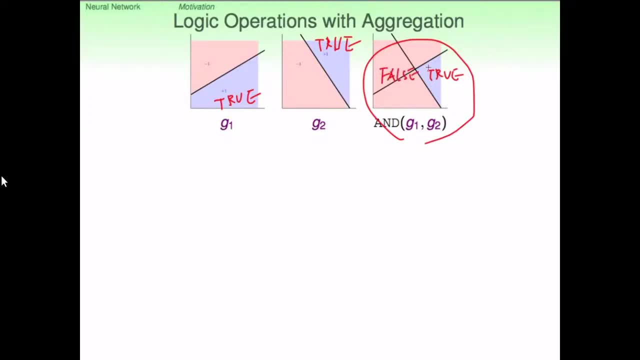 就是所谓的False负1的情形. 我们刚才那样的模型, 那样子把Perceptron做Linear Aggregation, 怎么做到右边这个End呢? 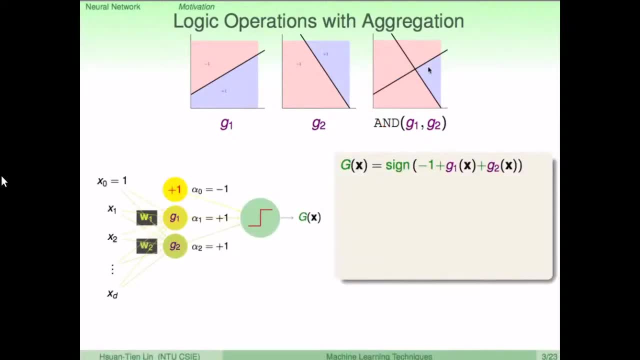 我们来看一看, 我们说可能可以做到的方式 是这个样子的. 我们把第二层这边的权重 这些α的值 设成这个样子. 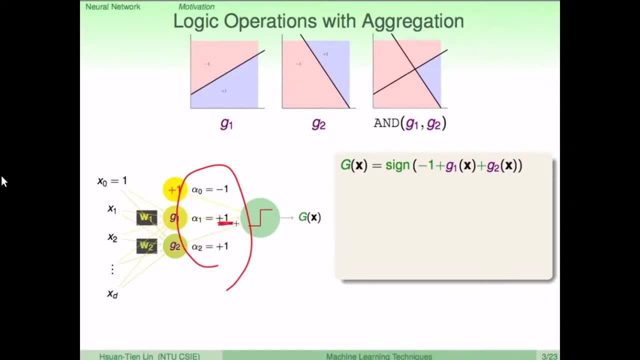 把G1的α值 设成是正1, G2的α值也设成是正1. 我们如果想像有一个G0, 这个G0是一个常数的输出. 常数的输出永远都输出正1. 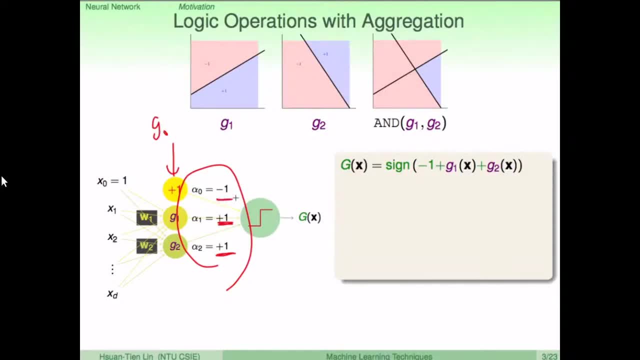 但是我们把它的权重, 它能够投票的数量设成是负1. 所以我们来看看一个这样函数: 我说我们的大G是把原来的小G1. 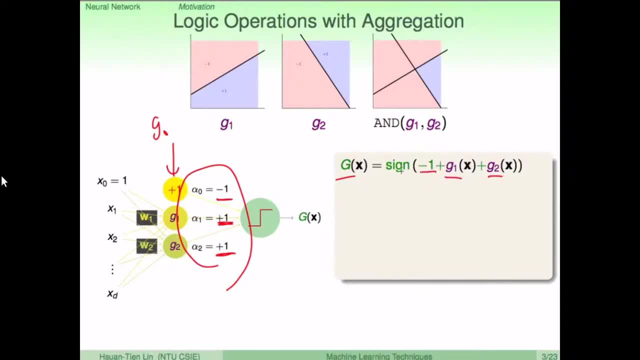 跟原来的小G2加起来. 以后减掉1取正符号再输出来. 我们的宣称是这样的大G 跟我们上面想做的这个End. 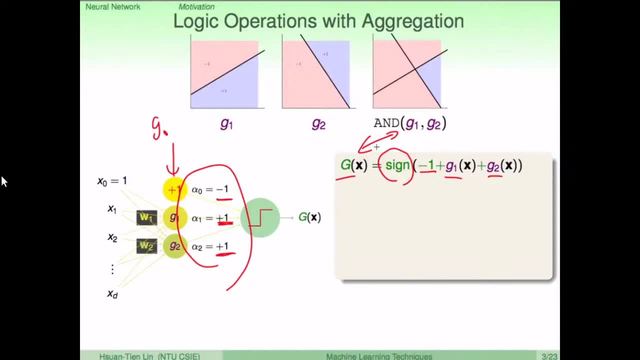 是一模一样的意思. 怎么看出来呢? 我们来看: 如果今天两个小G的输出 都是正1都是我们说的True, 也就是都在蓝色. 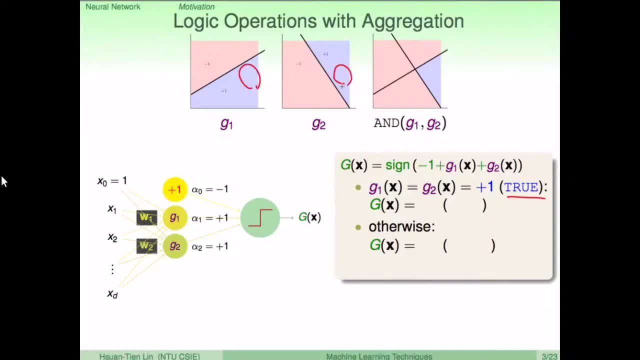 蓝色的这一区的话: 那反正什么事. 我们这边得到的是正1加上正1, 也就是说我最后得到sin的正1, 对不对? 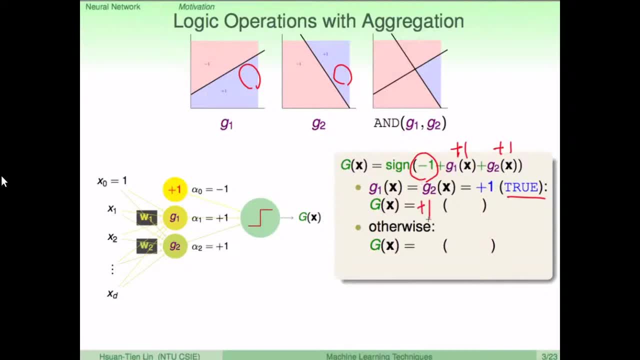 两票再减掉一票再取掉sin, 所以我的G是正1, 也就是True的结果. 如果今天两个小G里面有任何一个是负1呢, 那么两个小G的和. 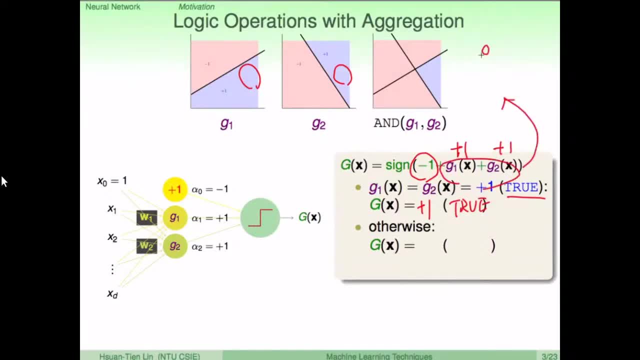 这两个小G的和 我要么就会得到0, 要么就会得到负2. 不管我是得到0还是得到负2, 我这边又有一个减1的结果. 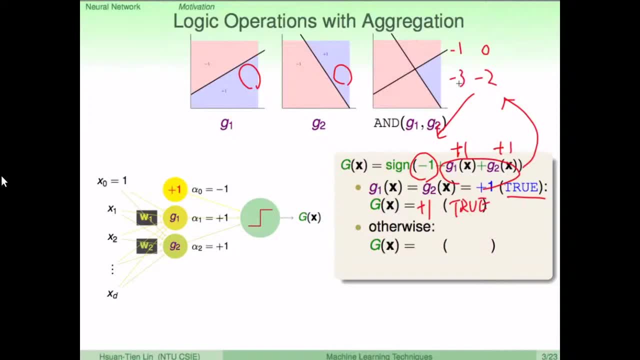 所以我最后会得到负1或是负3. 这负1或是负3取了sin之后, 我最终最终大G一定会得到负1, 也就是False. 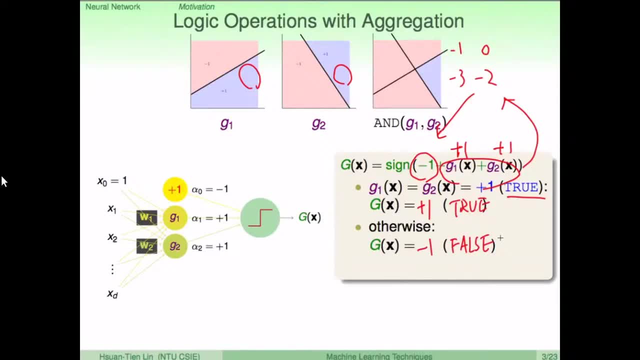 两个都是True的时候得到True 两个只要其中有一个是False就得到False. 这是什么 这就是End. 所以我们的大G其实做到的事情. 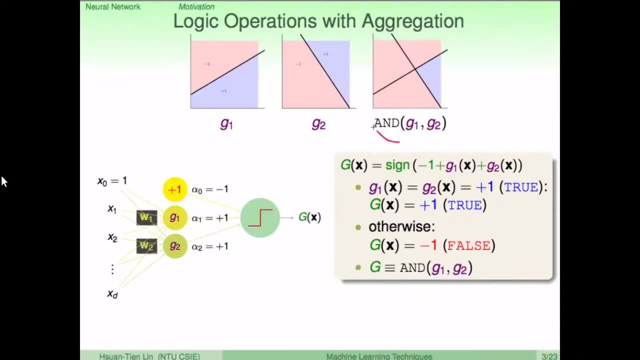 就是跟我们 右上角想要做的End是非常一致的. 所以这里说明了说: 我们如果用Linear Aggregation of Perceptron的话 我们似乎可以在第一层的Perceptron上面. 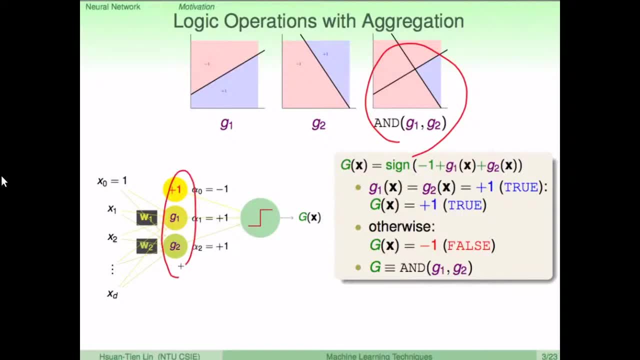 第一层的这个G1跟G2上面 做一些些逻辑的运算, 进去第二层的时候出来一个比较复杂的边界. 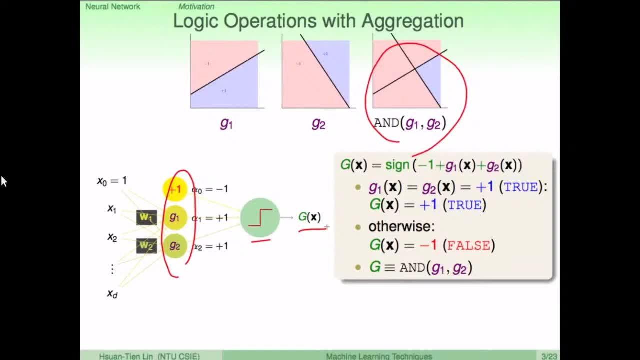 比较复杂的边界就不再是一个线性的边界. 例如说我刚刚这个End的例子, 它的边界是一个由两条直线组成的边界. 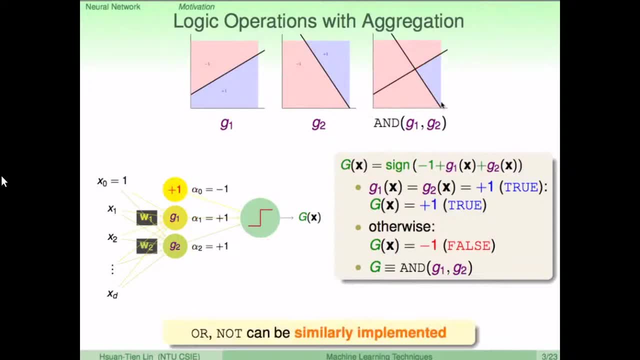 而不是单一直线的边界. 好那如果你有兴趣的话 你也可以推导看看 其实你在一般的布林运算里面. 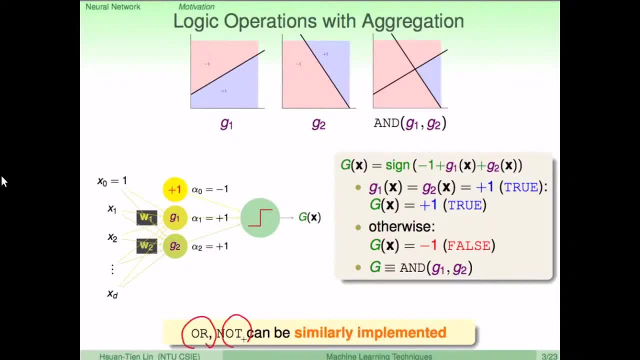 你如果要做OR或你要做NOT的话, 都可以用类似的方式来做推导. 那很比较简单. NOT其实就是把输出的部分乘上一个-1. 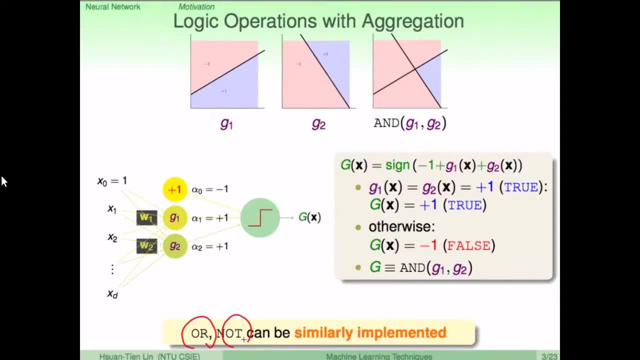 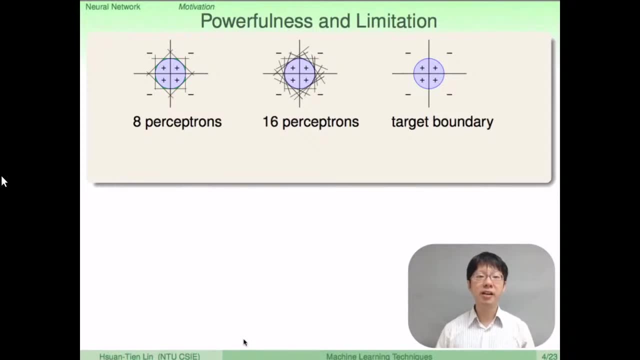 把它反向就好了. OR的部分可能稍微复杂一点. 这是参考End的方式. 你应该也可以推导的出来. 好所以这样的模型 我们刚讲Linear Aggregation of Perceptron. 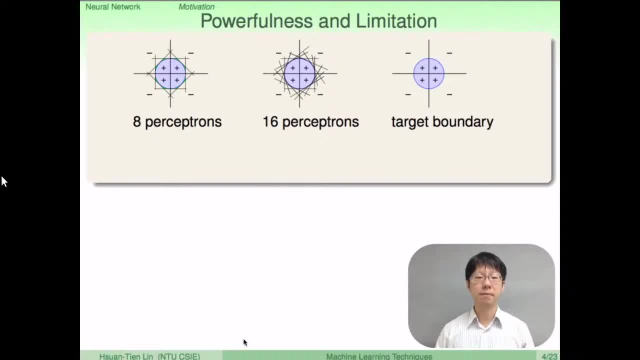 实际上是非常的powerful的, 非常复杂的. 怎么说呢? 我们来看看上面这个例子. 想象说我们如果在我们的目标里面. 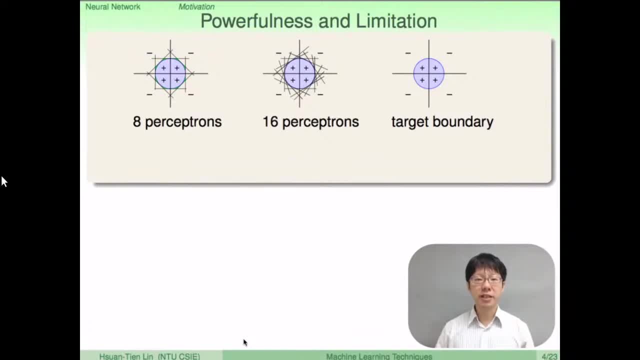 有个圆圈圈. 在圆圈圈里面是正1, 在圆圈圈外面是负1. 我们可以想象, 如果今天用单一的Perceptron. 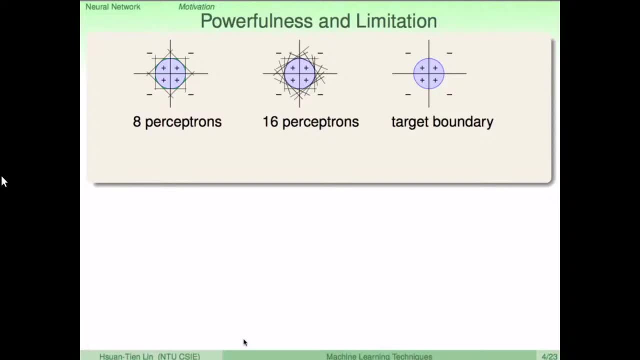 是没有办法做的. 但是我如果用8个Perceptron呢, 我用8个Perceptron, 把它用刚才那个End的方式合起来的话 我可能可以大概的切出一个. 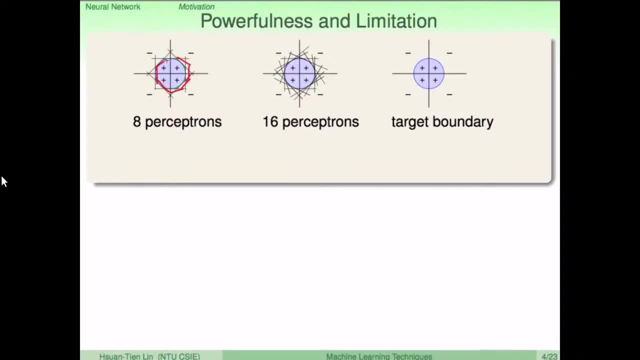 你看起来还OK的, 很接近圆形的边界. 如果我用16个Perceptron 再把它们合起来, 看起来可能就可以切的更细致. 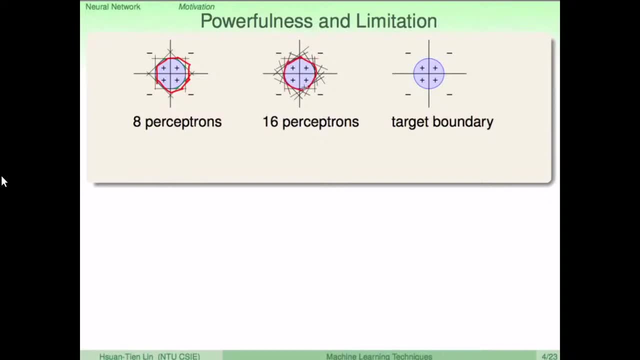 更好一些. 所以从这个例子看起来, 我们只要有越来越多, 越来越多Perceptron, 我们可以切出任何的Convex Set. 记不记得突多边形. 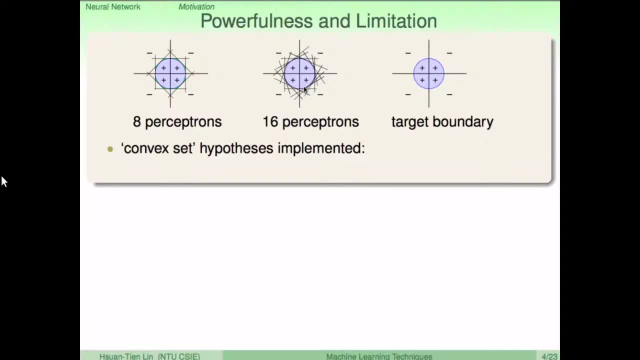 在二维平面里面的突多边形. 二维平面里面的突多边形. 如果所有这一类的突边形, 里面是正1外面是负1的合起来的话. 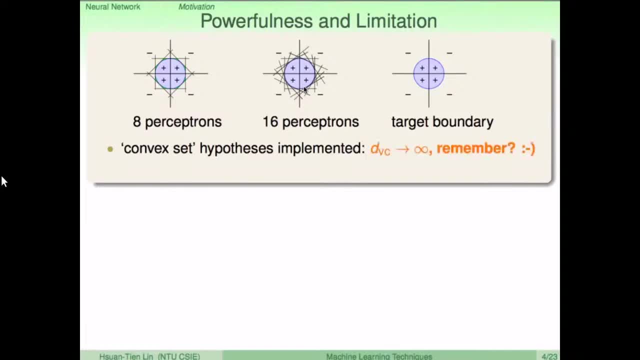 它的VC Dimension是多少, 记不记得, 无限大. 所以这里告诉我们说: 只要我们有够多的Perceptron, 没有什么做不到的事情. 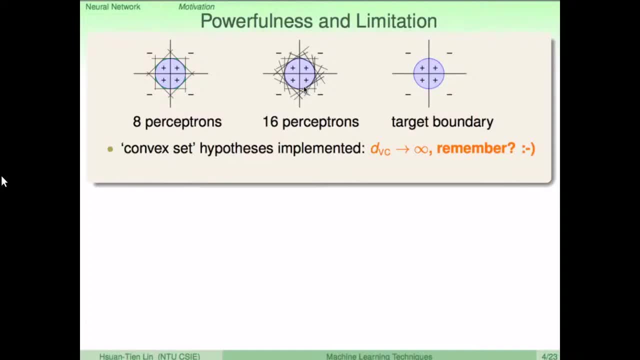 这可能是好消息, 代表说我们很多的Perceptron合起来 有很大的能力. 当然也可能是坏消息 如果这个模型太复杂, 把一堆Perceptron合起来太复杂的话. 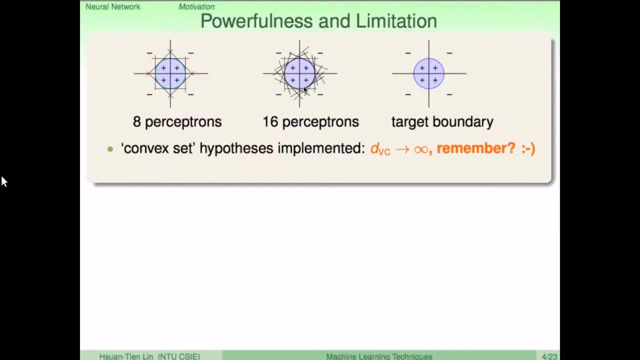 它可能会有Overfitting的危险. 它可能会有Overfitting的危险. 再来我们刚才在上面秀的这个例子. 再来我们刚才在上面秀的这个例子. 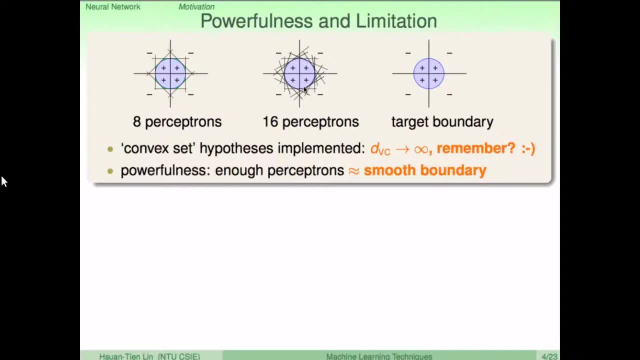 实际上是我可以用一堆的Perceptron. 实际上是我可以用一堆的Perceptron 来逼近一个什么, 来逼近一个平滑的边界. 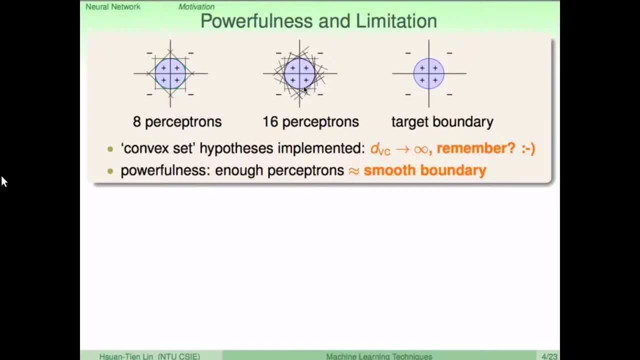 来逼近一个什么, 来逼近一个平滑的边界? 实际上我们之前在Aggregation 实际上我们之前在Aggregation 也看过类似的情形. 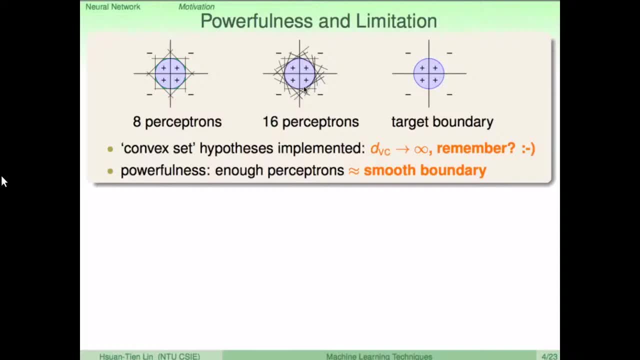 记不记得在Random Forest的图里面. 记不记得在Random Forest的图里面 说切出一些斜斜的不是很规则的边界. 说切出一些斜斜的不是很规则的边界. 说切出一些斜斜的不是很规则的边界. 慢慢合起来以后看起来会变成平滑的多. 慢慢合起来以后看起来会变成平滑的多. 慢慢合起来以后看起来会变成平滑的多. 慢慢合起来以后看起来会变成平滑的多. 这样的模型这样子把一堆Perceptron合起来模型. 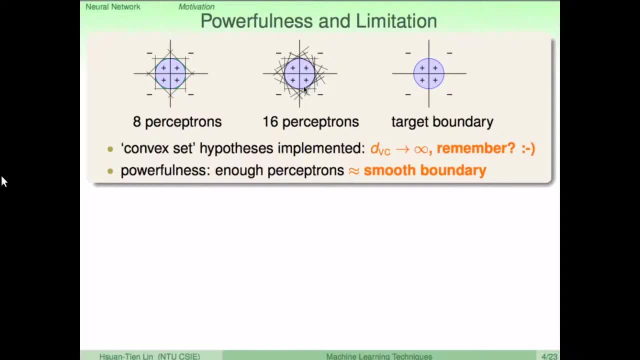 这样的模型这样子把一堆Perceptron合起来模型. 这样的模型这样子把一堆Perceptron合起来模型. 把一堆Perceptron合起來模型. 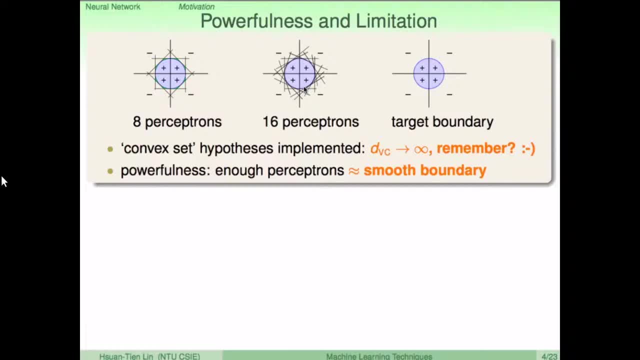 實際上是非常的具有能力的, 但是怎麼樣? 但是其實它還是有做不到的事情. 舉例來說: 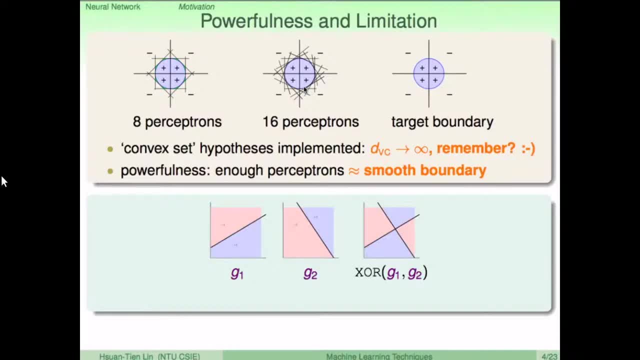 我們剛剛說AND好像做得到. 可是呢, 我今天如果考慮G1一條線, G2一條線, 我把這兩條線做所謂的. 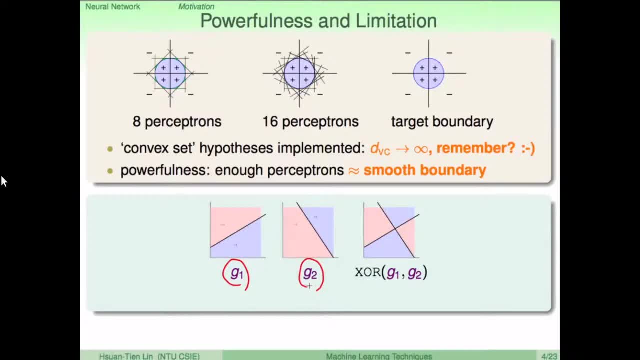 Exclusive OR Exclusive OR什麼意思? 就是兩條線裡面. 如果有一個是True 剛好一個是True, 那麼就是True, 也就是藍色的. 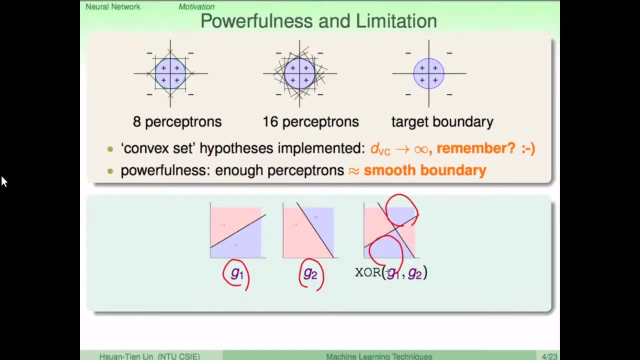 如果有0個或者是2個是True的話, 那麼就是紅色的, 就是False的部分. 這是一般的Exclusive OR這樣的運算. 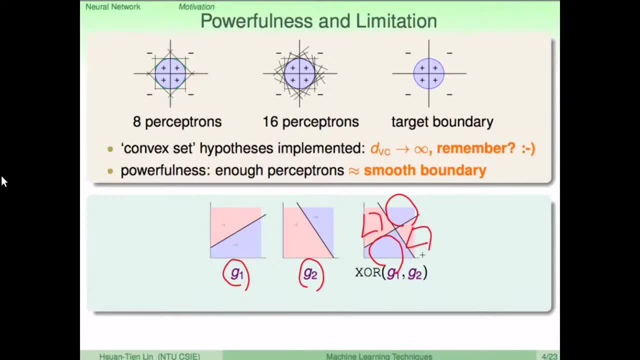 好我們的兩條線. 如果要把它合起來的話 做得到做不到這件事 經過一番的推導. 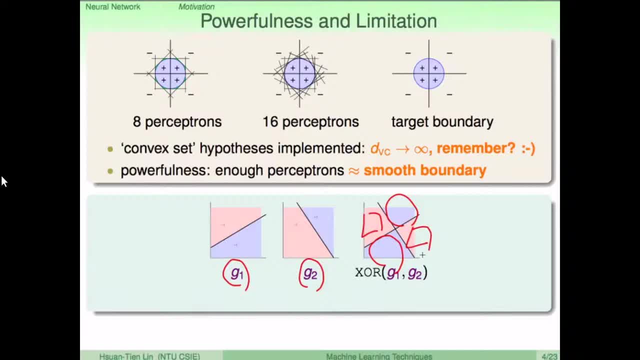 其實很類似我們之前在Perceptron裡面 我們想要證明Perceptron本身的複雜度的時候 我們就 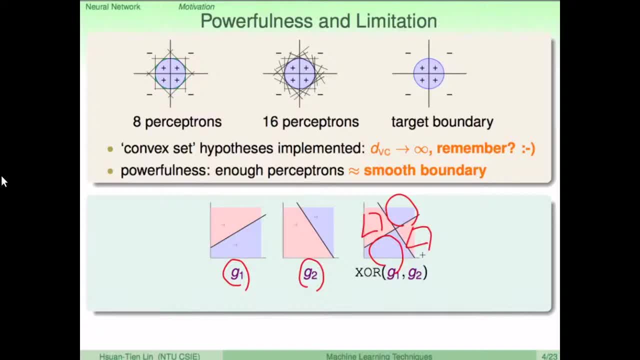 做事情. 你經過一番推導, 你會發現做不到, 做不到想辦法用Linear的Aggregation 把這兩條線合起來. 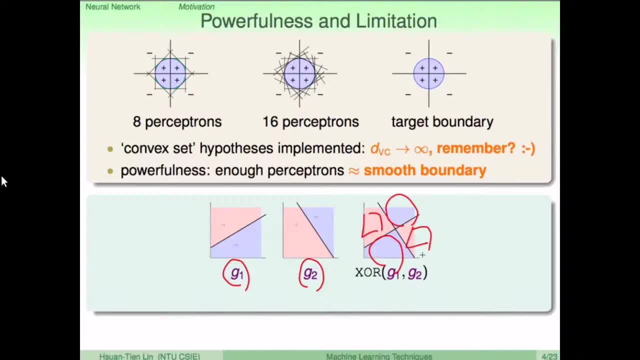 變成一個Exclusive OR這麼複雜的邊界, 也就是這是它的限制. 這限制怎麼產生的? 因為你如果把這兩條個別的線 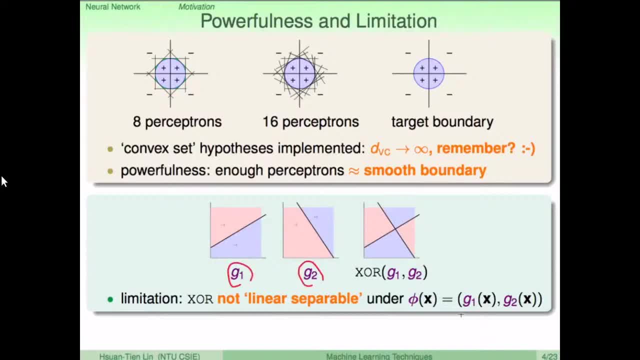 當成一個特徵轉換的話. 我們說的事情是: 轉換過去以後. 你還是沒有得到線性可分的資料. 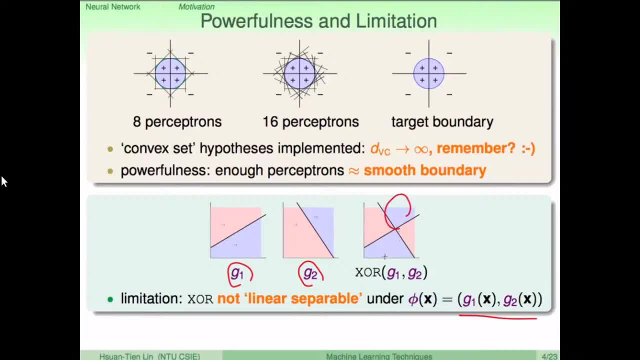 因為像右邊這個例子裡面 你的藍色要集中在好像一個雙曲線的兩側, 紅色要集中在雙曲線的另外兩側. 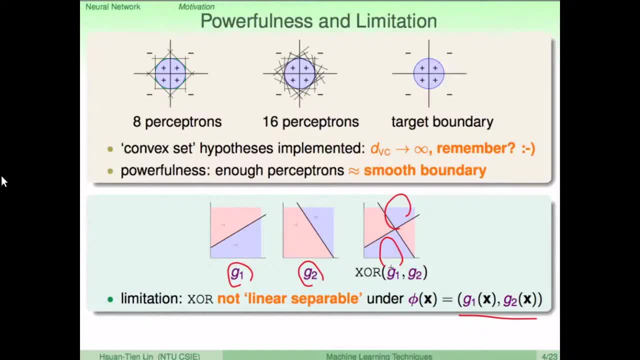 這並不是一個線性可分的資料, 所以在那個空間就算你轉過去以後, 你可能也沒有辦法輕易的用Linear Aggregation. 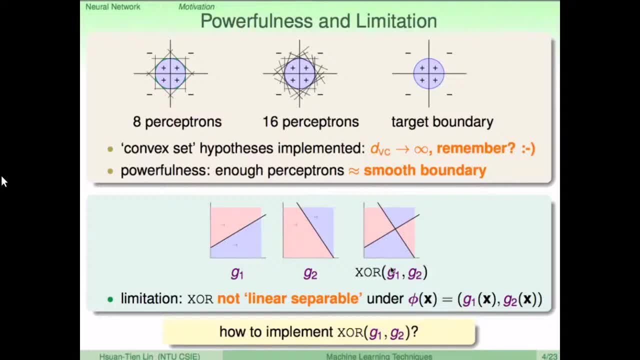 來得到一個適合的邊界. 好所以我們剛才講到的Linear Aggregation of Perceptron. 這樣的模型它的複雜度還是有限制的. 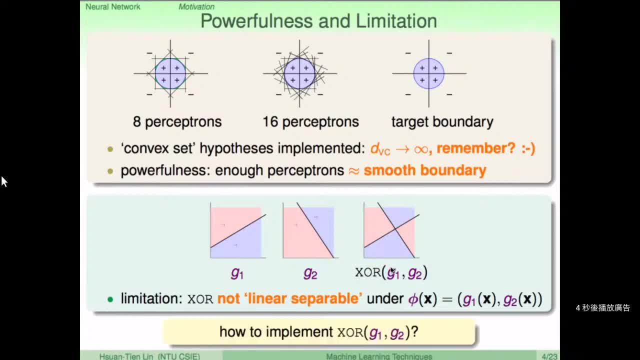 我們現在要問大家說什麼呢? 其他事情就是這樣, 那好? 那我們要怎麼做到Exclusive OR呢? 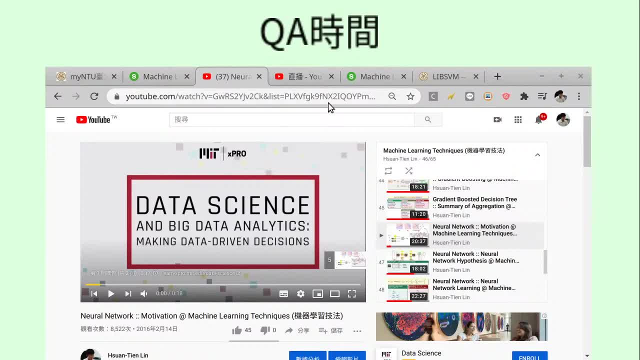 OK, 那這一段的課程呢, 我們給大家看到的是 Neuron Turk的開頭是: 那我們知道說其實我們沒有正式的上過Aggregation. 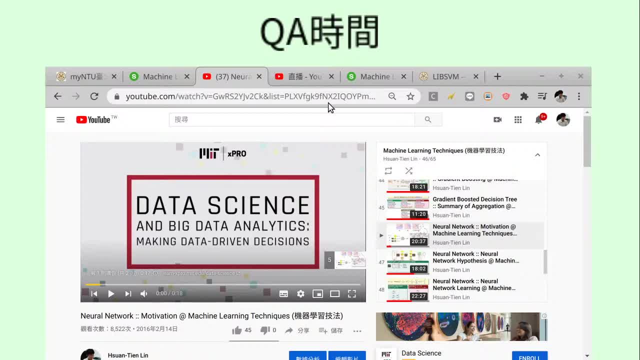 OK, Aggregation的意思呢? 其實就像是把你學到的一些Hypothesis OK, 當作輸出, 然後再接到下一個輸入. 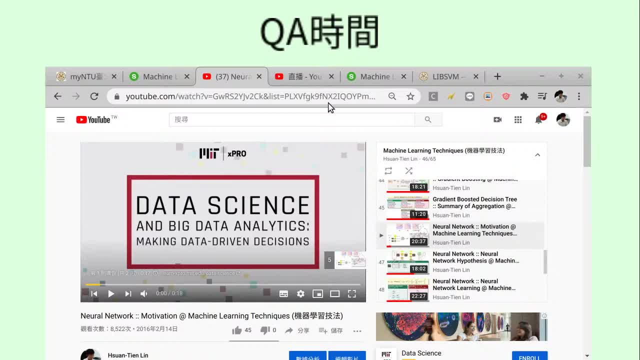 OK. 所以我們剛才看的有點像是 從Perceptron的輸出再接了一層. OK, 再接了一層. 在後面再接一個Linear Model. 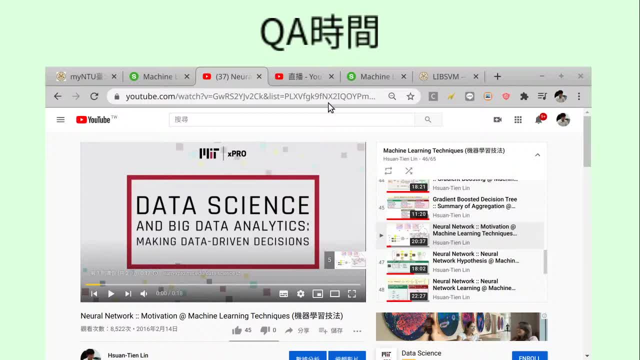 把Perceptron的輸出接到Linear Model的時候 我們給大家看了說我們可以做AND 我們可以做OR 我們可以做NOT. 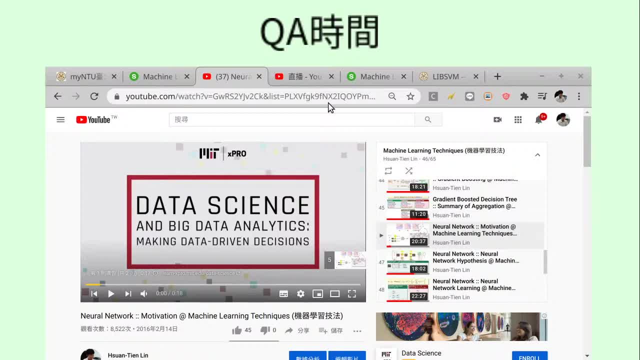 我們好像還是不能做Exclusive OR OK 然後那 所以這個我們再想想看要怎麼辦. 那當然這個下一次上課. 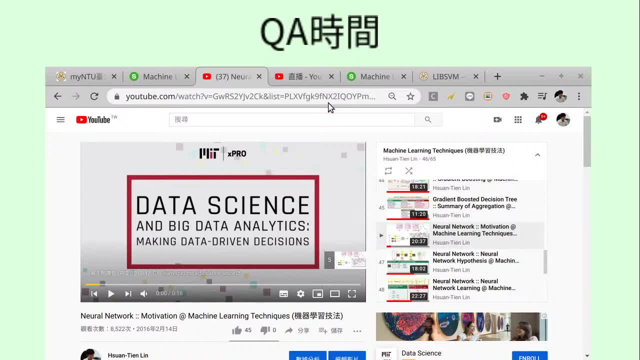 我們會給大家看到的事情就是: 那一層不夠你就接兩層嘛. OK, 一個便當不夠你就吃兩個. 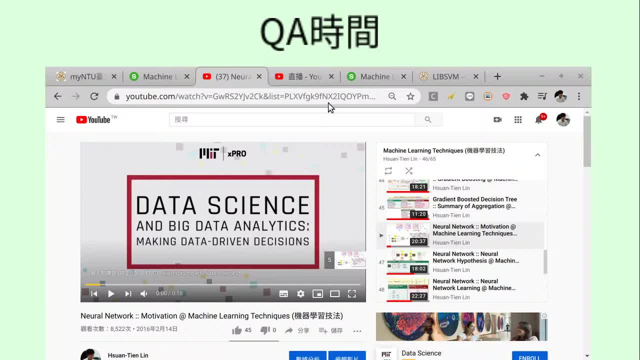 OK, 然後所以就是一層一層的接下去. 那這是我們給大家看到的所謂 類神經網路的Motivation. 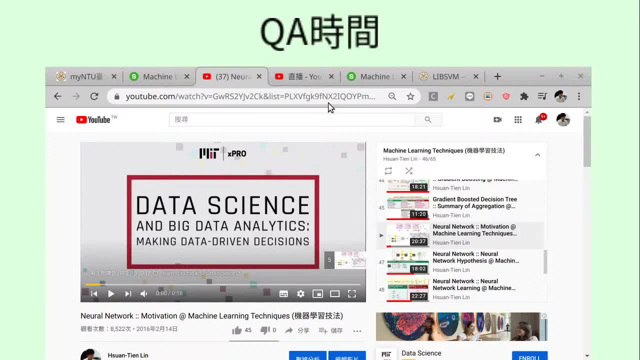 OK, 就是說你單一的Perceptron, 你如果覺得它能夠做的事情不夠, 那你就再接一層, 再接一層看起來變複雜了. 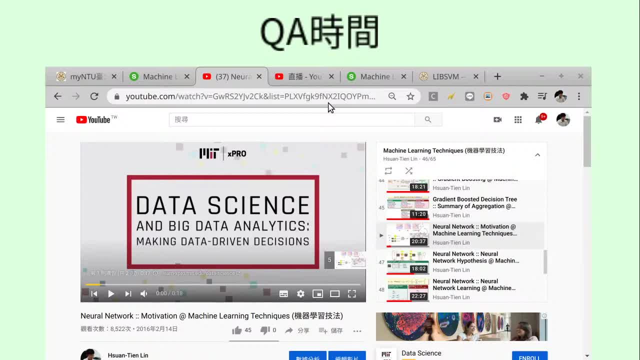 比如說你剛才已經可以做到Convex Set OK 這一類的事情, 那但是還是不能做Exclusive OR. 那怎麼辦? 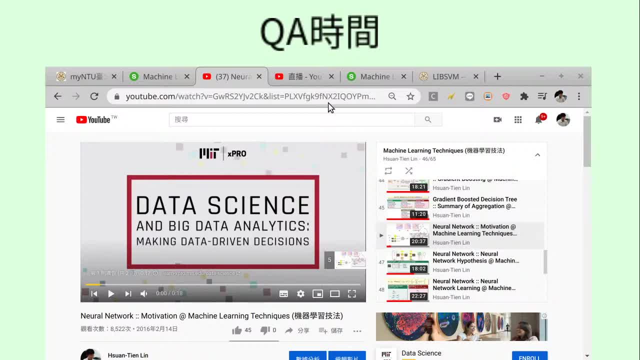 那就再接一層. OK, 那如果接到很多層的時候 就變成這個我們現在很流行, 很聽到的這些Deep Learning. 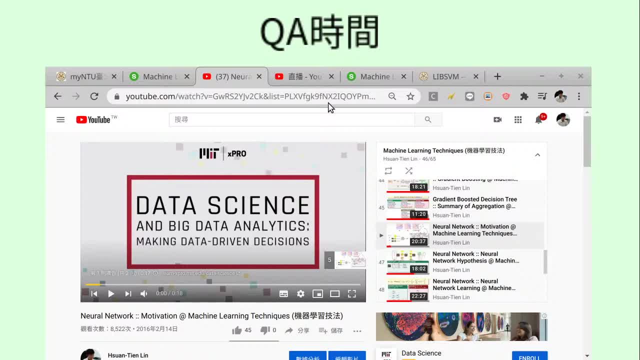 OK, 那當然這是開始. 真正要從層層的Perceptron- OK, 真正一路講到Deep Learning. 然後Deep Learning為什麼會動? 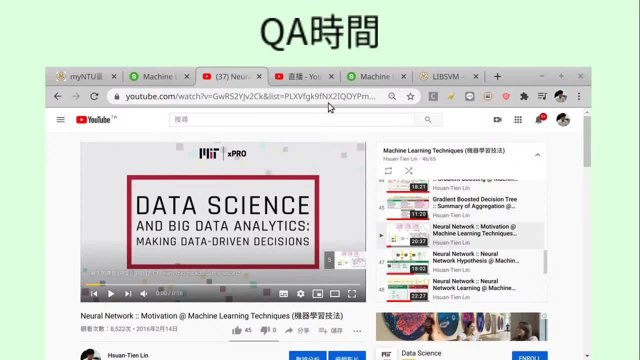 Deep Learning裡面要怎麼動起來. 裡面還有很多的技巧可以講. 那至少我們希望. 今天先給大家一個很淺的出發點. 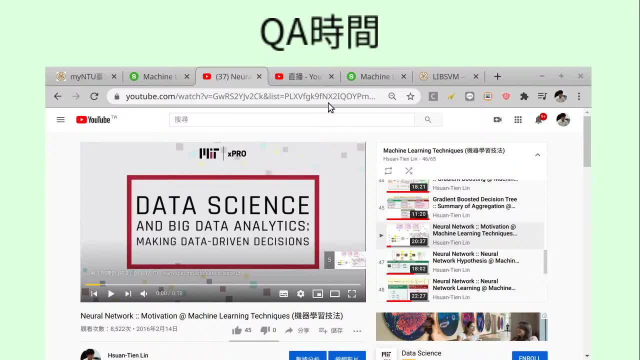 OK, 那下一次的時候 我們講一些些Neural Network, OK, 用它來帶出這個Metric Factoring, 這一類的所謂Recommendation的模型. 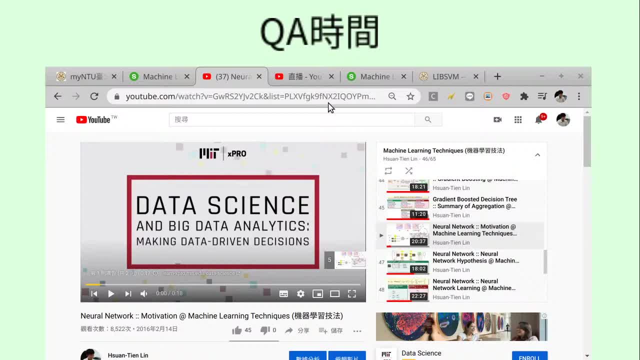 可能可以怎麼樣子想, 可以怎麼樣子做. OK, 來當作我們的一個 想像成大家一個興趣上的影子這樣子: 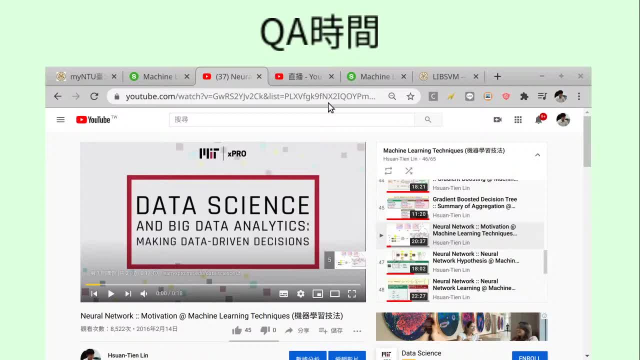 OK, 好, 那有問題嗎? 請說, 這樣會有廣告收益嗎? 大概我不知道, 因為其實是這樣故事. 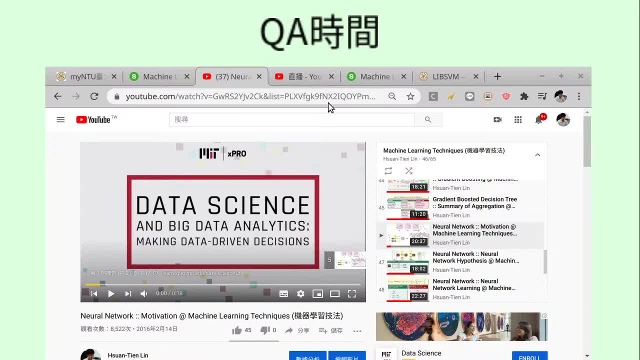 這個曾經有一陣子 我有把一些影片設成有開放這樣子 然後設成有開放以後. 這個好像會發生的事情就是若干個月. 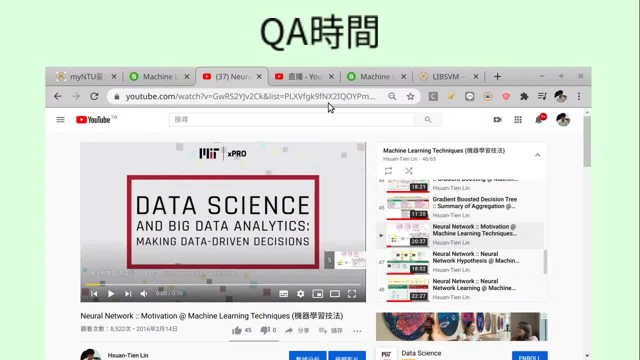 OK, 然後他們就會 Google就會給我什麼幾十塊美金那一類 非常非常非常少. OK 就是然後少到我也忘記到底有或沒有. 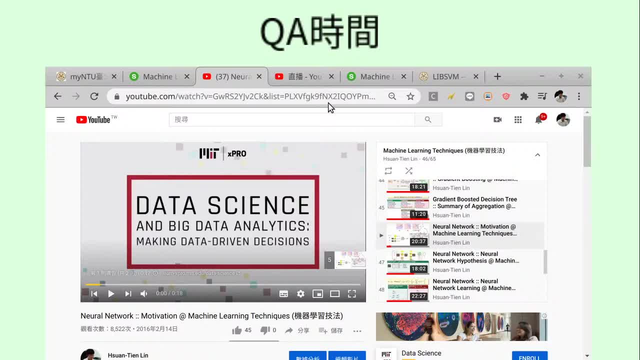 然後所以後來我就這個: 有的時候我就會把它關起來, 然後有的時候會怎樣. 所以我現在也搞不清楚到底哪些有開放. 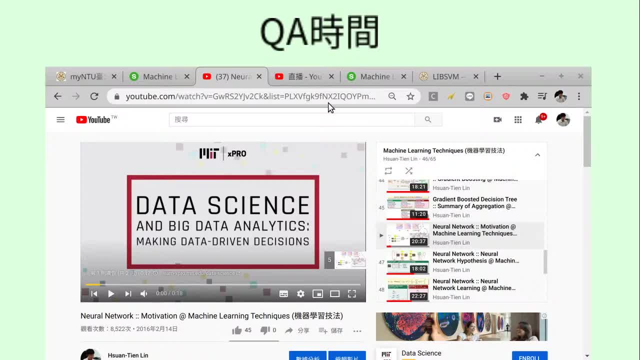 有些沒有開放的這樣子, 但是 in any case 我們現在還在直播世界裡面這樣講. 所以呢如果以後你們要反對我選校長的話. 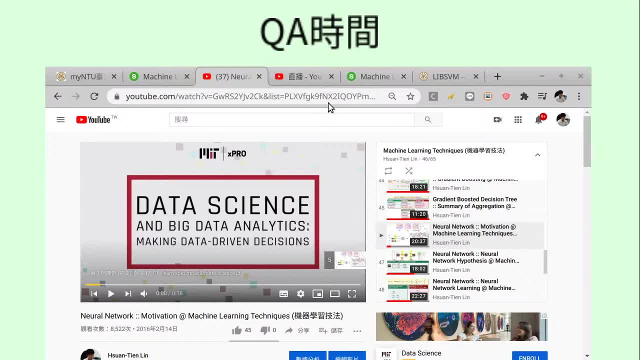 OK, 請拿著一點去檢舉我. 再說顯然我有不太正當的業外收入 還是什麼鬼的一類的. 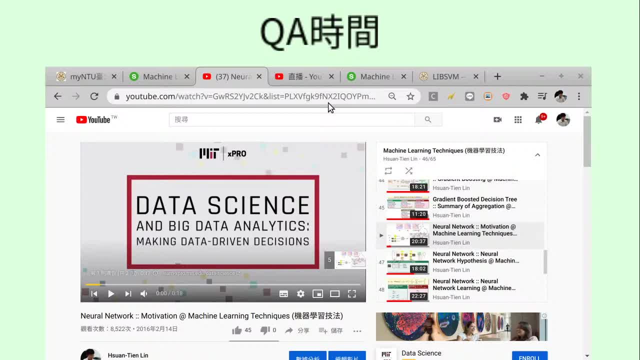 但是我也接錄影的機會慎重澄清: 這差不多就是一個幾十, 就是幾個月有幾十塊美金那一類的東西這樣子. 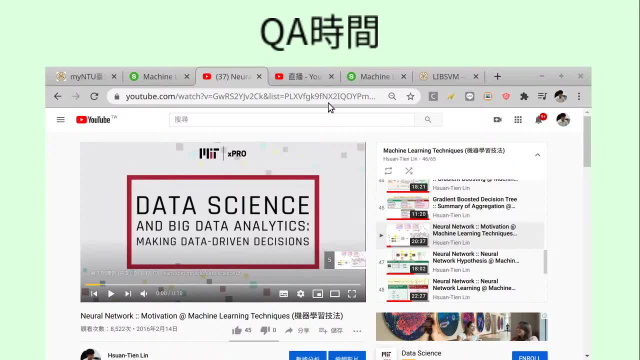 那這個我通常記得的時候我就會把它關起來. 有時候有些沒關到的還是怎麼樣子. 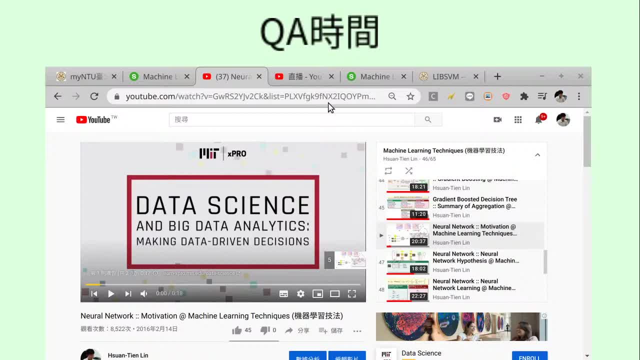 然後就會放出來這樣子 OK 好, 不過我才猜是這樣. 我自己放的應該沒有. 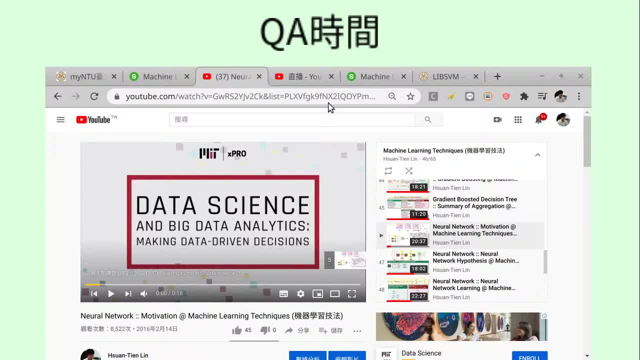 因為 Google 應該有一定的條件說 你不能自己去狂放自己的廣告. 這個顯然不是太幸運. 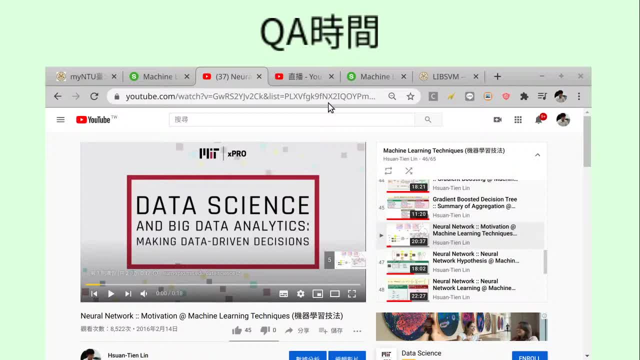 不過我如果跟大家宣傳的時候, 如果大家真的很想要贊助我的話 多多看看影片 然後多多按按廣告. 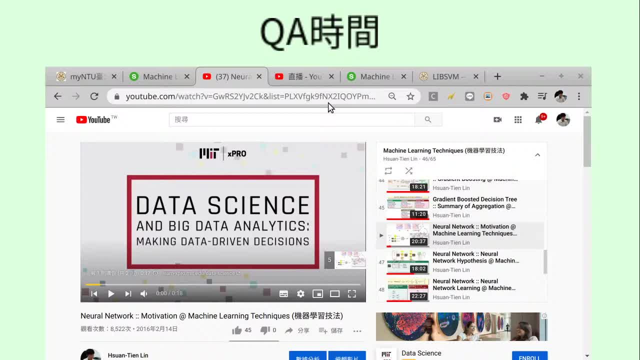 我不知道. 我其實不知道這會不會真的比較多, 因為你知道, OK, 就是已經有點嚇到. 我們先看有沒有其他問題. 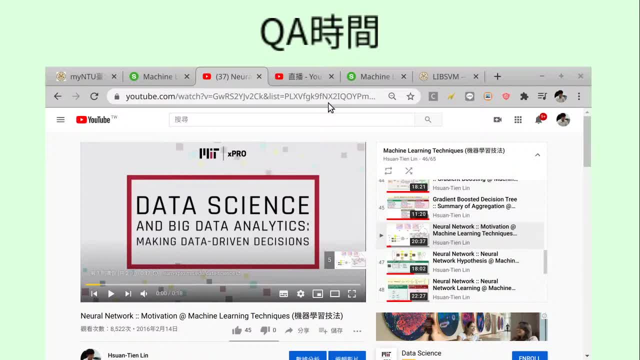 然後如果想要聽聊天的 這個我們可以下課之後再聊天, 沒有其他問題. OK, 好, 那我可以結束直播. 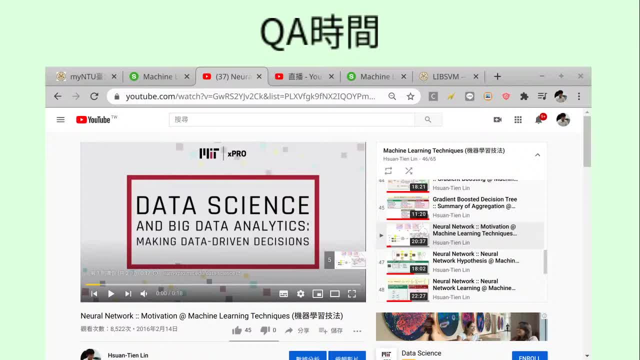 然後結束直播以後就可以聊天說: 我這輩子廣告收入最多的是什麼東西? 好, 我們先把直播關起來.